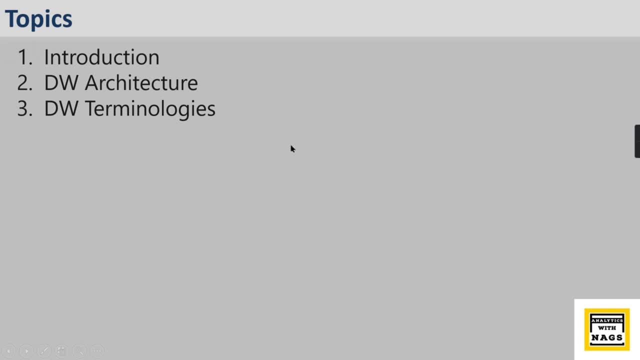 will not be a good flow or learning cycle. So I will cover some of the terminologies in Data Varo's- and there are lot more. I will cover it while I am demonstrating And we will discuss one business case study. That business case study is like explaining the OLTP system, and for that 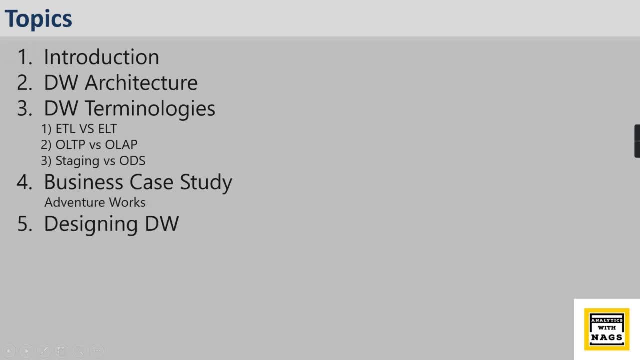 business. we are going to create the Data Varo's and that is the main agenda. and you see, that is business. case study is AdventureWorks. It is freely available and that OLTP system is available internet. We can download it. I will walk you through this. 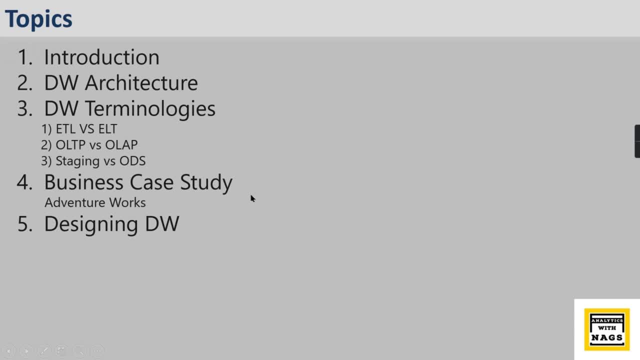 In Data Varo's. we have 3 steps. Finally, we will discuss about the steps, How you can do that as well. if you are not familiar with database technology, Then we will begin with designing Data Varo's. So it's not as soon as you understand the source system and Data Varo's, you will keep. 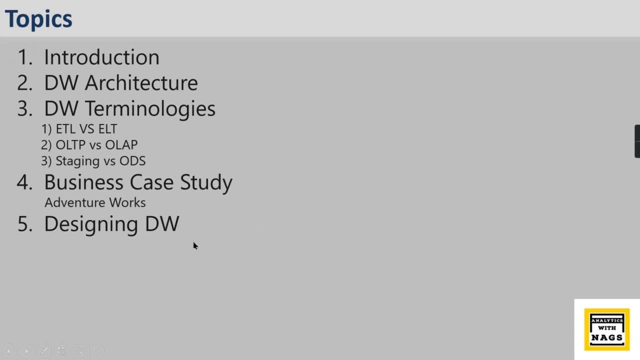 Implementing it, You need to properly design it. So what are the things present, How you can design. Who will design All those things? we will discuss there. So we will consider staging layer dimension modeling, how to identify fact dimension. what is the? 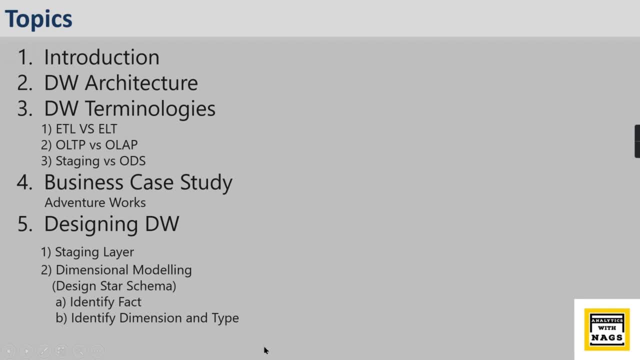 does it mean? are the different types. those classifications will comes under designing, so these part may be at least half an hour to one hour. we will talk about the data virus concepts as well as designing part, and after that we will start actual implementation of data varrows. that involves creating data. 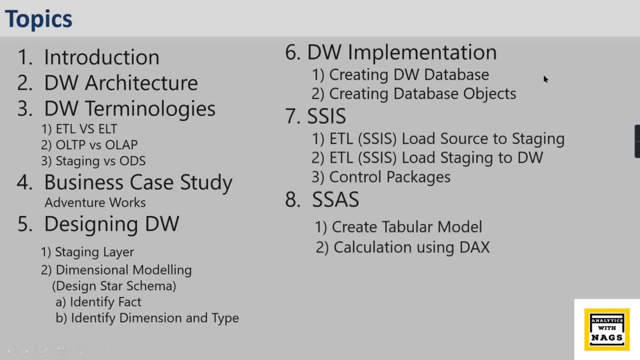 varrows objects, creating database objects like staging objects, then creating SSIS packages, then cubes right. so only till this point, SSIS, you are done with data varrowsing, but as a complete, what is the main purpose of data varrowsing is to build reports and make the business self servicing BI. 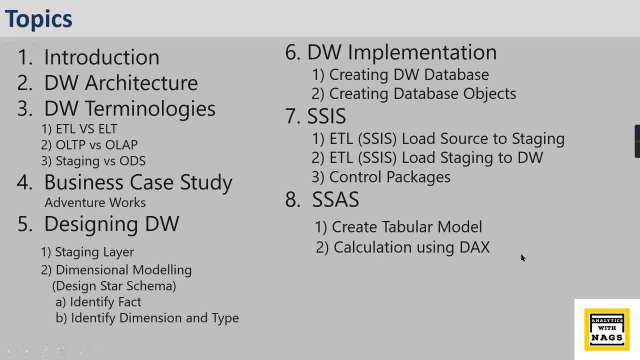 right, this is a part of BI. so these are the some of the add-ons I will add. so I will create some SSIS cubes in tabular model and, if time permits, we can create DACs and then we will schedule the jobs. so there are scheduling. the one flow is: 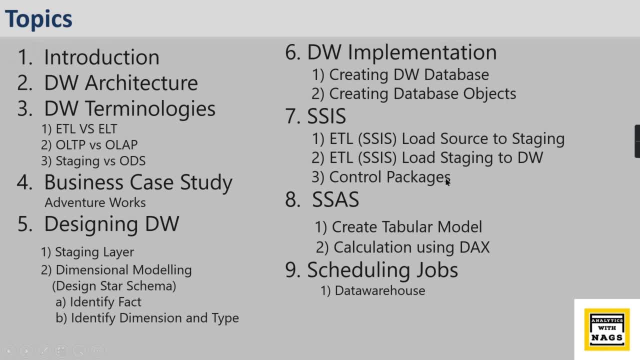 like schedule. whatever we have implemented, we need to schedule it for the data varrowsing and the scheduling. there is some the power BI scheduling is different, so we will talk about that once we come across this session. then we will finally summarize what we have seen in this video. this is the main. 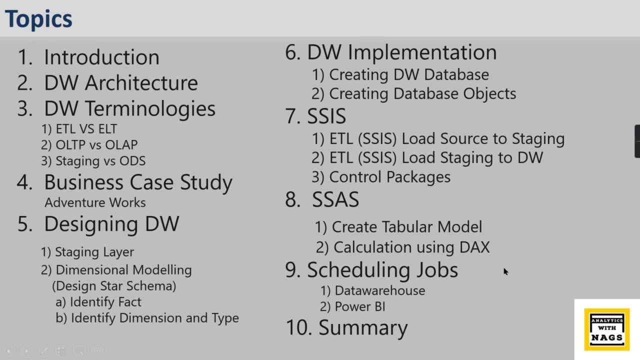 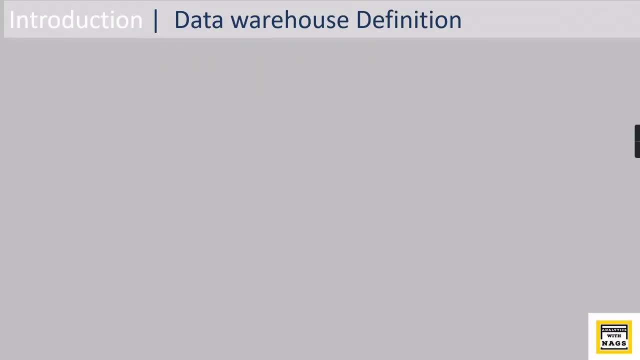 agenda. that is what I will walk you through in this entire video. if you are new to this channel, hit the subscribe button and press the bell icon for notification. let's begin. let's begin with introduction about data varrowsing. so the definition says: data varrows are central repositories of integrated data. 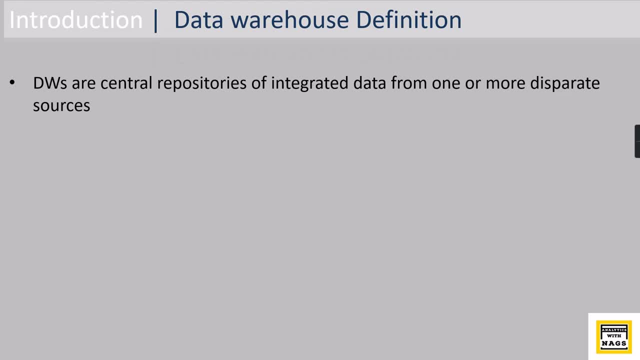 from one or more disparate sources. basically, this is the fundamental definition of data varrows: where you have a data in different sources- it can be Oracle, Excel or different application mobile applications- and you need to integrate into a single place. that is what a data varrows is meant for and it 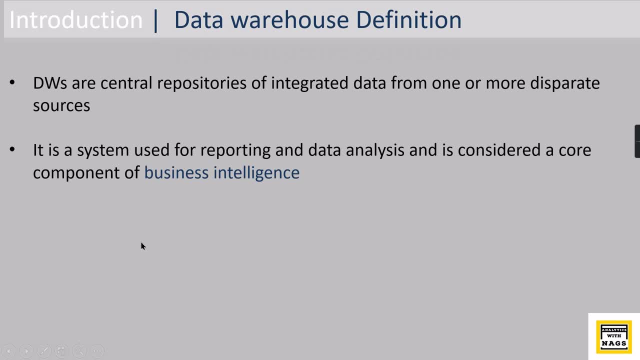 is the system used for reporting and data analysis is considered a core component of business intelligence. so with this we are introducing new terminology: business intelligence. so business intelligence and data varrowsing interchangeably used. basically, it is a system that is used for reporting and data analysis. basically, you are creating a BI solution. what it means is like you need to create. 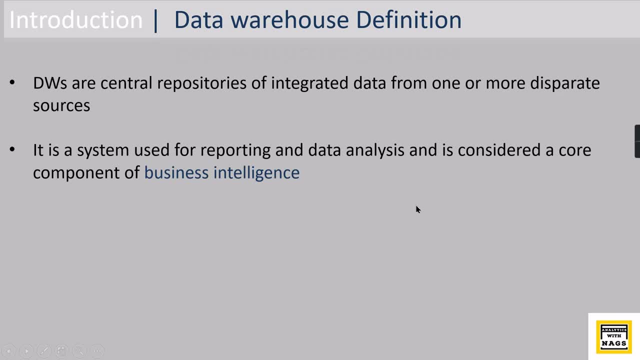 a data varrows so that your business intelligence solutions will be on top of that right: creating reports or self servicing, self BI, those things. so, basically, if you are creating a BI environment means you are creating a data varrows. that is what it is. so let's try to understand what is business intelligence is. 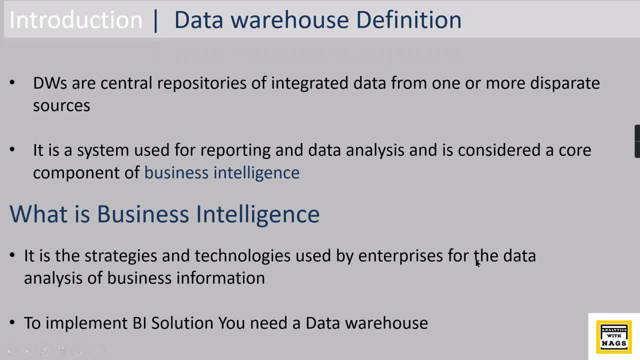 it is a strategies technologies used by enterprises for data analysis of business information. so all the big companies, most of the companies, those who use BI solution, right, they use this solution for data analysis and for the business information, data analysis of business. what they will analyze, whatever their 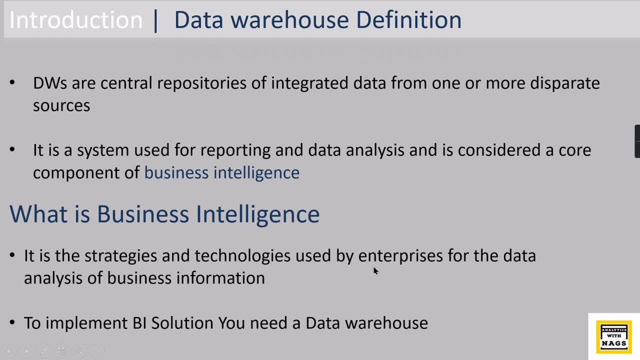 business generate the data. that thing they need to analyze and the technology they implement is BI and how they can implement. once they build a data varrows, they can implement a BI solution. so to implement BI solution, you need a data varrows. this is what a simple terminology or introduction about data. 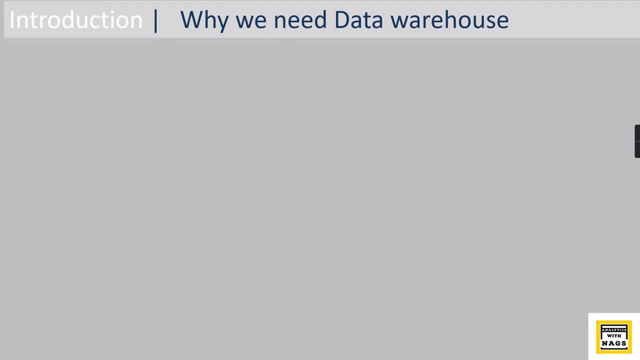 varrows. so why we need data varrows? and there are a lot of reasons. one is, as we discussed before, to integrate from many different sources of data. avoid users running reports directly against operational system. these are the important aspects, just. I will take a couple of minutes, like you have a. 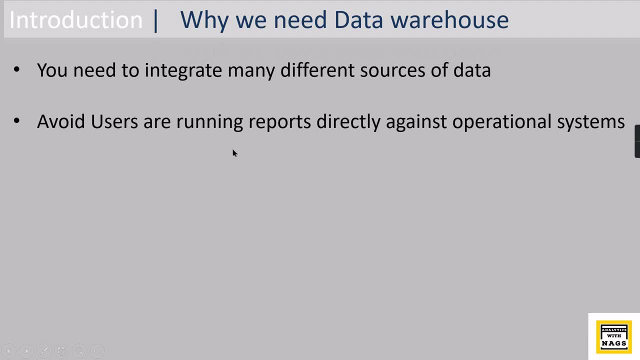 different sources here and your operational system. that operational system- maybe I am saying banking system here- is you nationalized bank in India having 10 million or 20 million customers, right? so at least a hundred thousand people log in in their system. so their system should be optimized in a way that 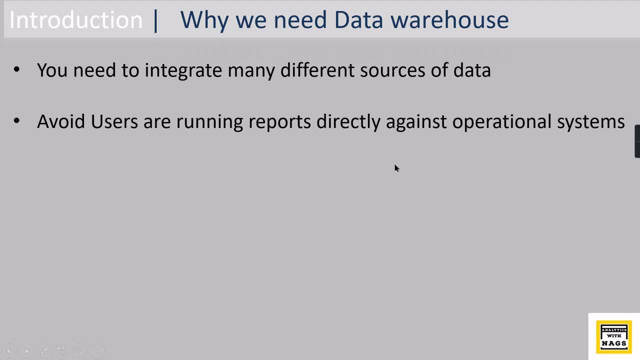 they can run the data. they can run the data. they can run the data. they can run it in a way that the bank knows that accurate and they know that their there will be dedicated system meant for reporting. that is what a data varus, and also having a single. 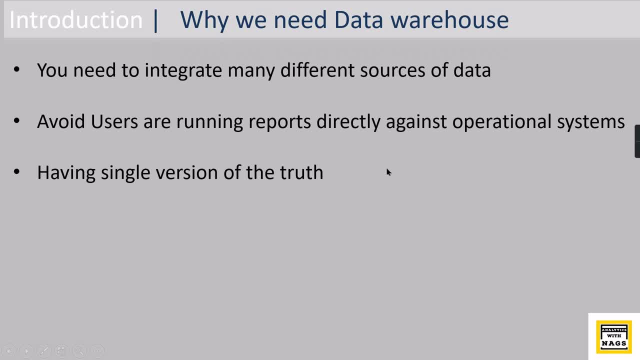 version of truth. meaning like people will maintain the data in different places, so there will be different versions of the meaning. like a customer information is maintained in two system and one system says the customer is from india. another system says like he is from another country or you can consider within india. you say like customer belongs to chennai and another system. 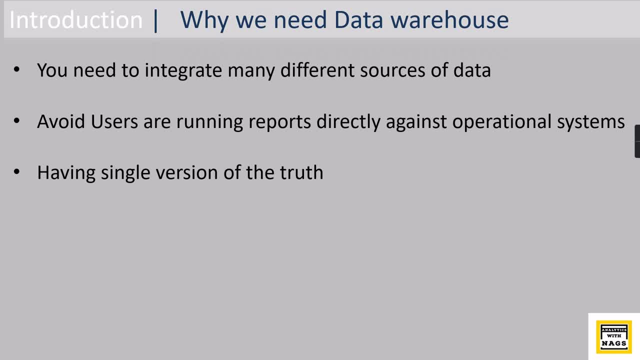 says customer belongs to delhi. so how you will promote or you will give some promotions based on different locations, right you, without knowing where is actually is right currently, then you cannot give a correct solution and whatever you give, that will not be much effective. so it should. 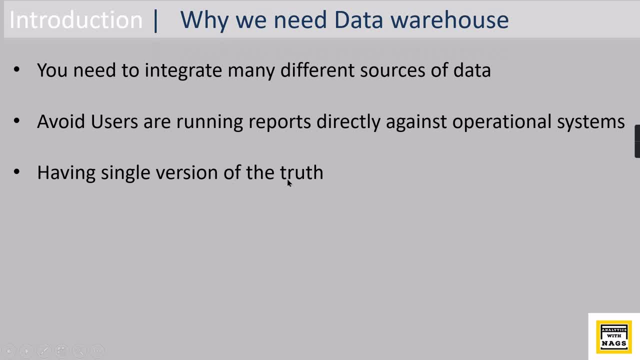 be. i'm saying a simple example. what is a single version of truth? right? so everywhere it should be. whatever the data, it should be a single version. there won't be multiple versions of your data and you have tons of historical data that you need to gather. basically, 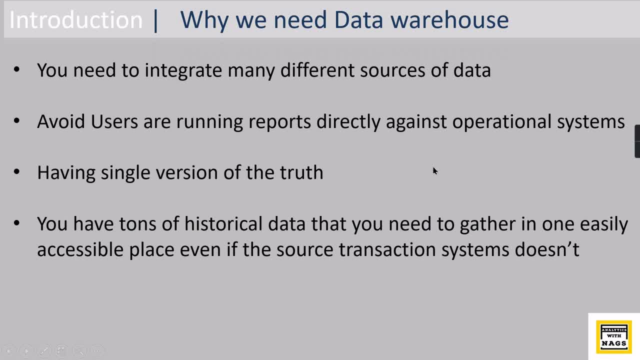 your operational system. it should be functional, for operational system means, if you are not aware it's like consider a banking system, your core banking system or your e-commerce website. those things are operational system to what is the main purpose? to run the business, to do a transaction. 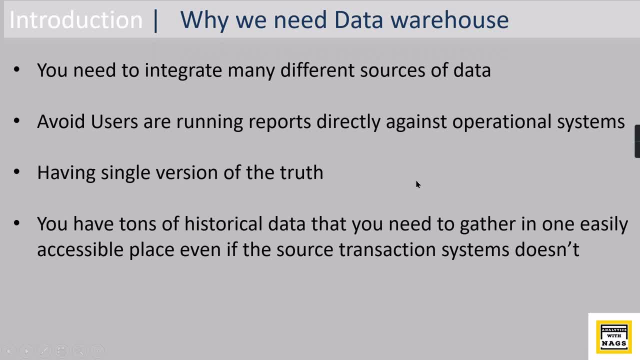 you want to send money from one person to another right. that is operational system so it will keep on generating the data around 10 to 20 years. right, and you store the same data and for your operational system, also hold the same right. it will slow down so you can move the old data in. 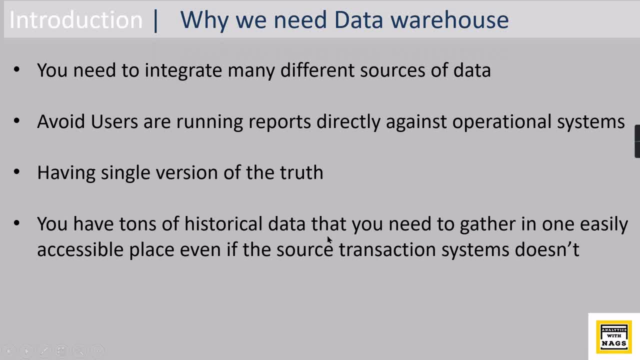 the operational system. you keep only two years of data and later two years you can move that all the data with some other system. so till now they use the name called data warehouse. so historical data will be stored in the data warehouse. this is the another purpose will go for data warehousing. there are some other reasons as well. we will quickly walk. 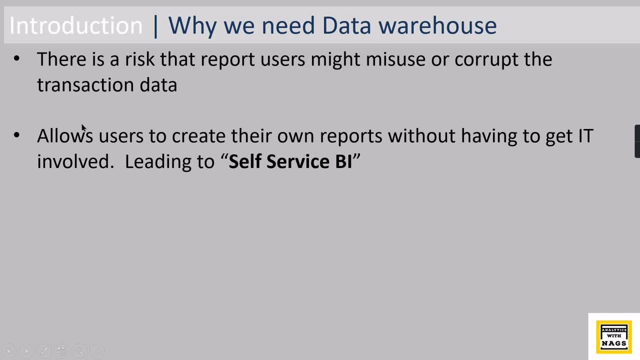 through the risk of report users might misuse or corrupt the transaction data. your transaction data is very important. again, it is same point. we can move on to next, the data warehouse system. you search for the data warehouse system and when you search the data warehouse system, you can access the data warehouse system. it allows users to create their own reports without 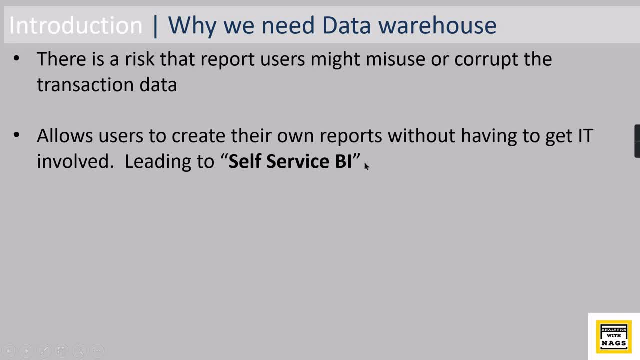 having to get it involved. so this is what very important aspect of data warehousing or bi solutions basically like: when you have all your data in a transaction system operation system, typically it's stored in the database. so for a manager are non-technical people, they cannot go and query the database. they don't know the sql or the programming languages right, so they just need a ui to be able to create a data warehouse system. so you can view it as your own data warehouse system is a bit complicated. there is no need for each of the data DieR or data warehouse system. everything can be created and when we come back here we 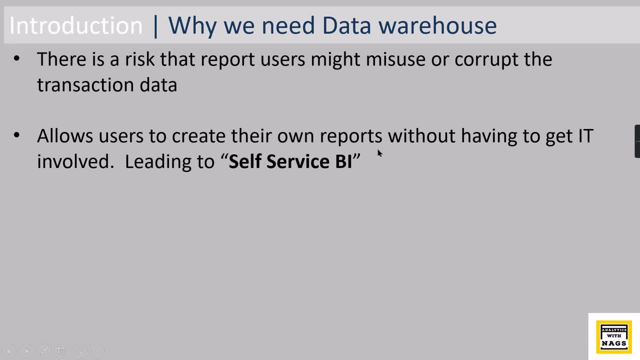 languages right. so they just need a ui to drag and drop certain things and ask the questions with the ui only so, in order to enable the self-service bi, you need to create this bi solution using a data warehouse. then the executives they can drag and drop how many. 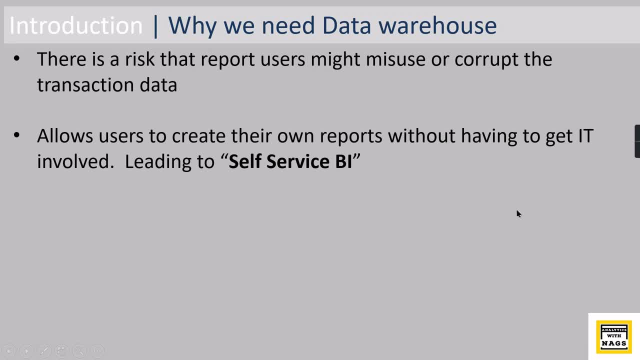 cells happened in this location, or what is my top sales? what is my bottom sales? those things they can do, play around with that. for that you need to build a proper data warehousing- this is another important aspect- a convenient place to create store metadata and business logics. so basically, you have logics or calculations you need to do to compute your 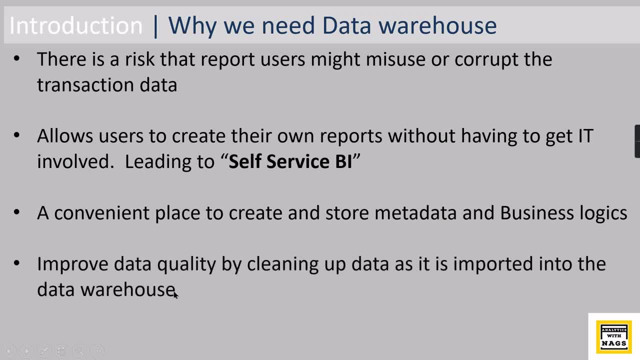 core business logics- this is the place where you can do that- and, more importantly, data quality by cleaning up the data, because for reporting you need the clean data to be displayed right. so you will get some comments with some kind of spelling mistakes. for different locations, you will get a short forms instead of giving a proper name. like bangalore, people say bank or 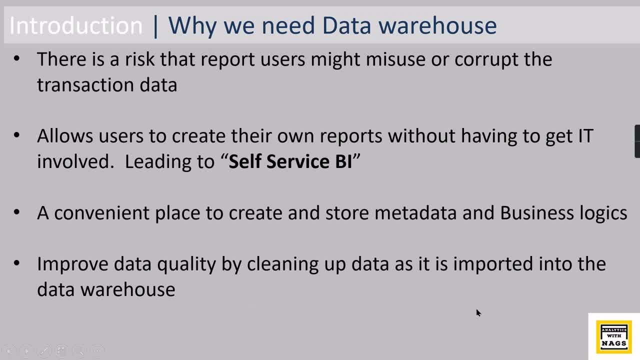 some hyderabad they will say: hide something like that, right with its short characters, so those things cannot be reported as such. you need to do some cleansing exercise or improve the data quality, so this is the place you can do that. then it is the proven technology where you no need to do anything. i mean to say like: 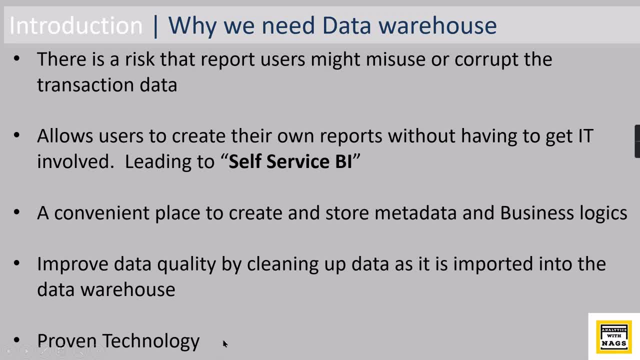 whether you need to invest or not. yes, you can invest because most of the organizations- those who invested in data warehousing and bi solutions- they have gained a much. that is what it is: a proven technology. so these are the reasons why we need to go for data warehouse. let's start discussing. 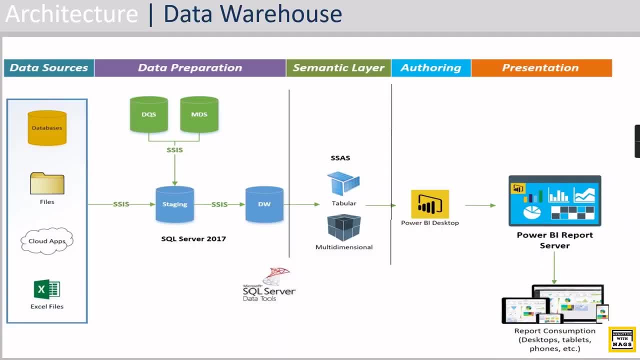 about architecture of data barrows. so this is a typical architecture where on your left hand side you have your data sources and this is the layer we will call it as data warehousing layer. once you build your data varrows, we will create a ssas tabular model that can be a possible right earlier. 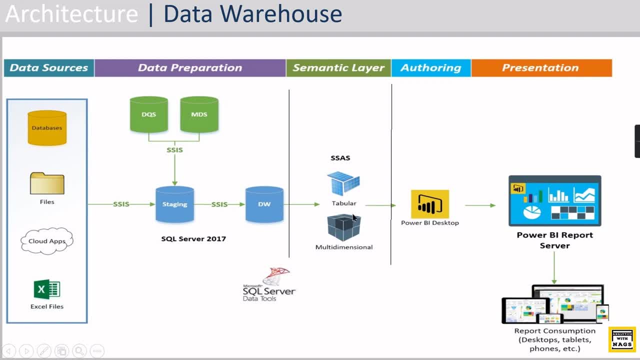 we used to create a multi-dimensional model so you can create a regular image from that. you can also- and surely microsoft is not recommending and those who are conventionally using they still maintain it- but most of the things you can achieve it in ssas tabular itself. this is what 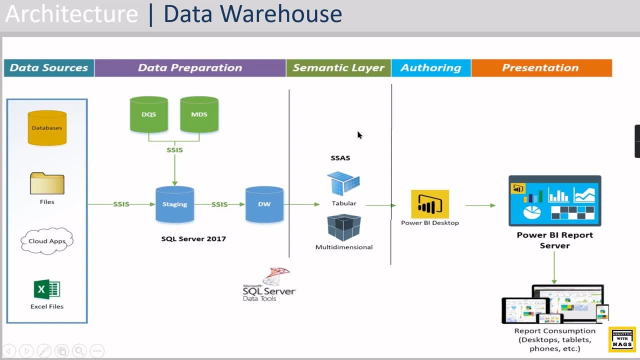 microsoft currently recommending. this is a semantic layer where you will apply all your logics and measures, calculations, where you want to create ytd, mtd and kind of. some time intelligence functions on top of it, right? so those things you can create it here. then there comes a reporting. 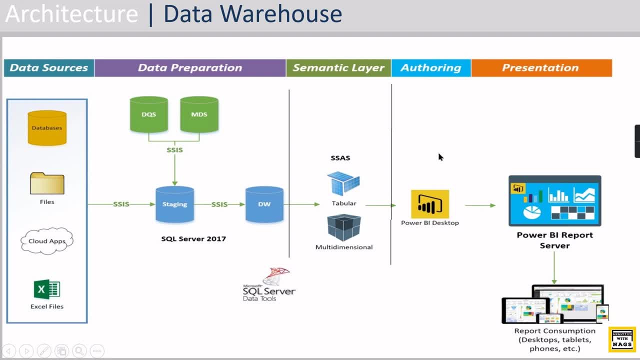 layer. either you can use power bi desktop or your custom build applications using dot, net or any other tools. typical people, most of the people, use the excel as the reporting and recently people are going to power bi as well because it is so famous, user friendly, very interactive right. so for those, 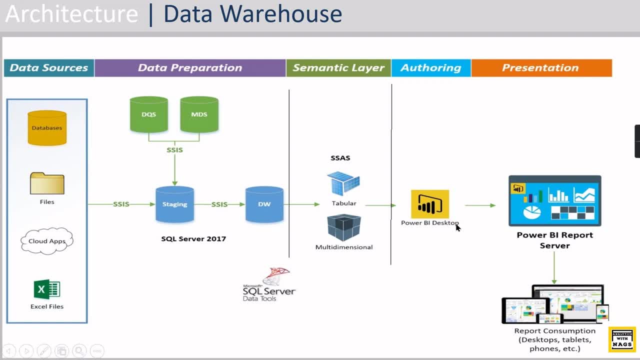 reasons, power bi is a very good way to create a reporting layer, and you can create a reporting layer here now. that means if you we go to our web browser and you can create a report on this report and then you also create a service on your web browser and you can use your data warehouse. 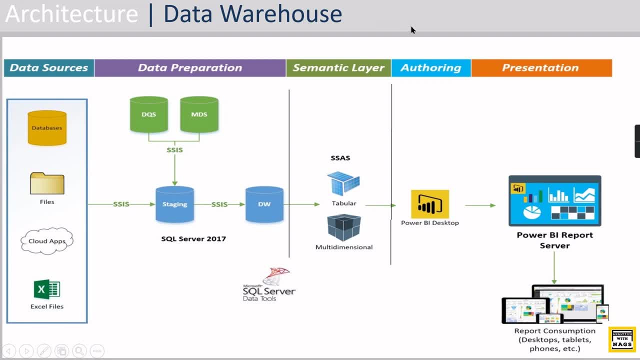 for it, and so power bi is successful. now then that is so. there is no different things. i mean the flow it is showing. once you develop your report, you deploy it in power bi service where you can. data warehouse is to build your dimensional modeling. dimensional modeling is nothing but. 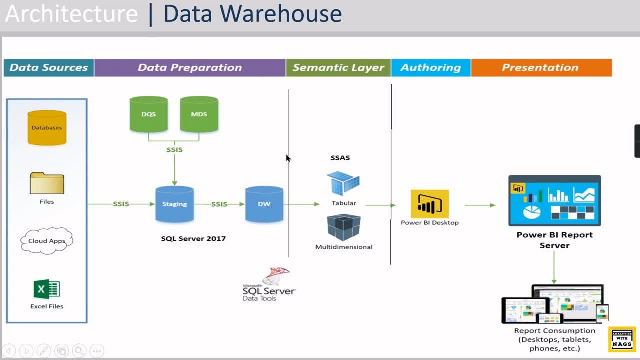 you create your star schema, you have a fact surrounded by your dimensions. so inside data warehouse you have different data marts as well. what is data mart? you have a sales data mart where all the elements related to sales fact and dimensions will be considered as one data. 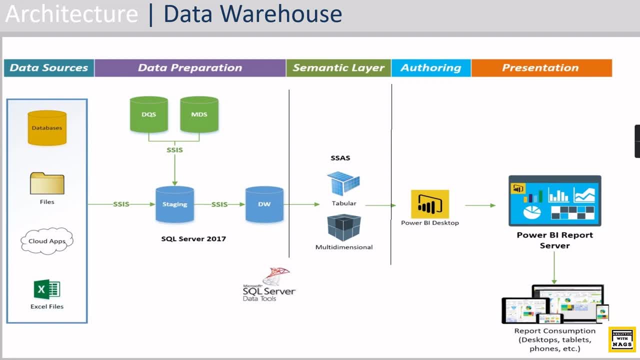 mart, that is, sales data mart. you can also have another data mart called the human resource right, so human resource will have its own fact and dimensions. then you can create that as well, so there can be a common dimension between sales and human resource data marts as well. so your data. 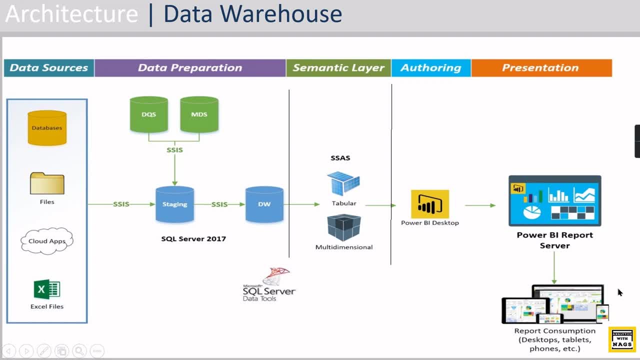 warehousing ends here. the entire architecture is your bi solution, business intelligence solution. so bi and data warehouse interchangeably. people use it. so bi is nothing but implementing your solutions like data analytic solutions on top of data warehouses. we can say like that, right, we have already seen the definition, so 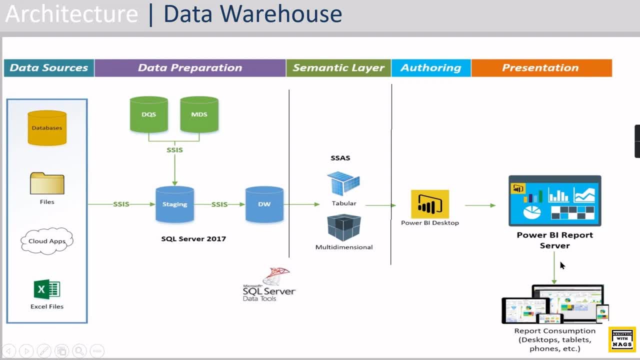 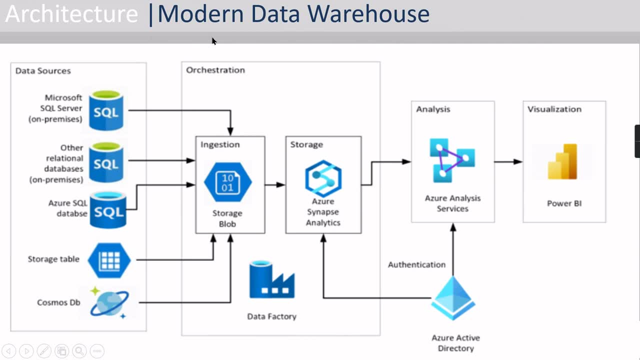 this is what a typical conventional architecture is. and now, with the modern data warehousing approach, like the data are mode changing right, different varieties, where you see here a model of a table of data, where we have a different type of data warehouse and we have a different type of data warehouse. so this is what we are seeing here. so this is what we are seeing here. 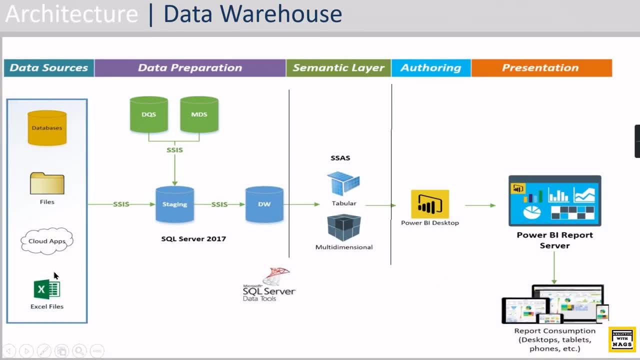 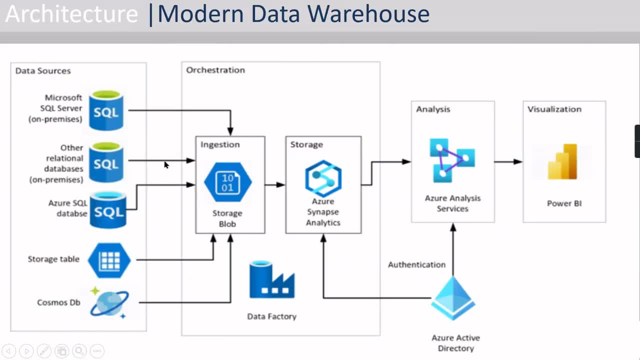 this is typically like structured data. so those who are having a structured data, then this is the approach. till now it's successful, unproven technology where in our modern data warehouse architecture you can see here datas are coming in different forms right, different varieties it. it is not only a structure. you will also get unstructured data and semi-structured data as 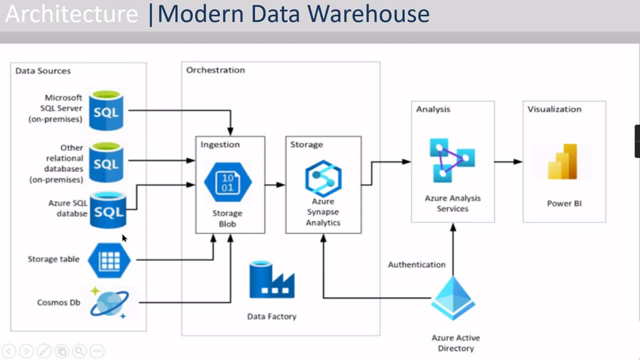 well, so those things to handle it. it is not enable. i mean, the current on-premise ecosystem doesn't support much and the storage cost is more. so people go for cloud technologies, right, and whereas from your this is not very different: architecture: the storage part and the processing. 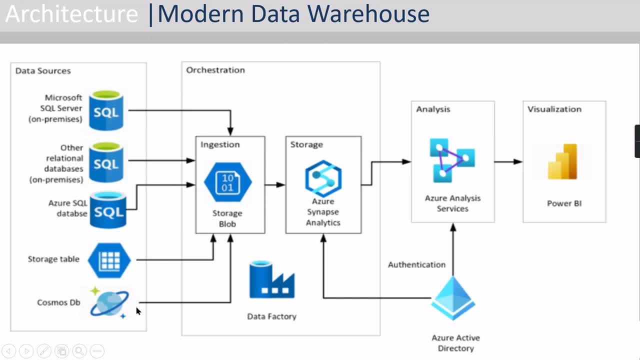 part varies where you can see same, like you have different sources and you can ingest information from different sources. and you can ingest information from different sources into a storage blob called azure data lakes- right, that is how to compatible data lake storage- okay. and using etl tools called data factory- right. this is the flow and you can also process it using 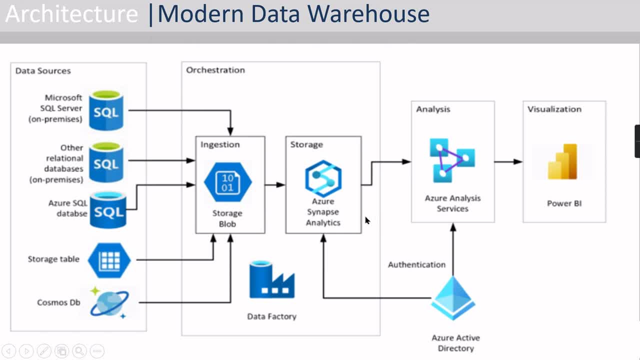 azure, synapse, analytics, creating a warehouse, and then on top of that you can create the analysis service, then power bi, the flow remains same, where your the usage of tools will vary. that is the only difference between the data warehousing conventional and the modern data warehouse. we will touch upon these things if time permits, but mostly we are going to implement this. 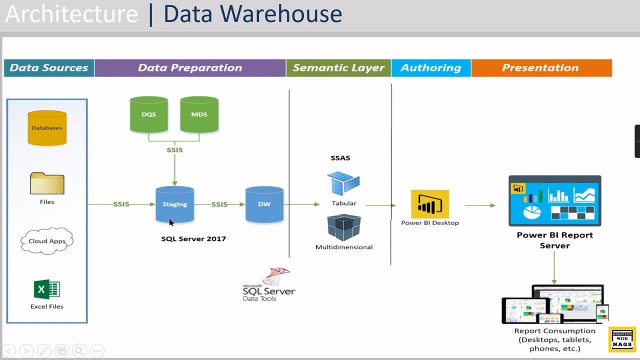 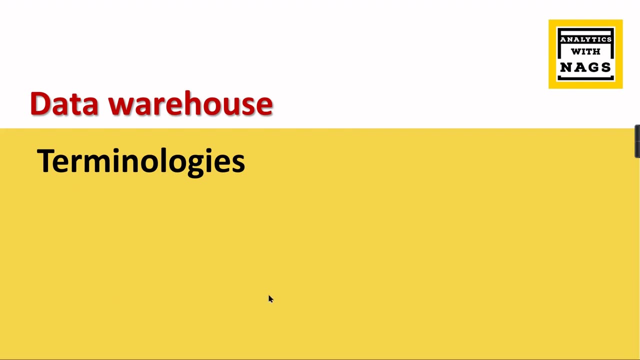 data warehouse architecture end-to-end from the creating of staging data warehouse. we will create ssas, then we will create reports in power bi and publish it. that is what the main agenda of this video. there are a lot of terminologies available in data warehousing. i have covered that in the data 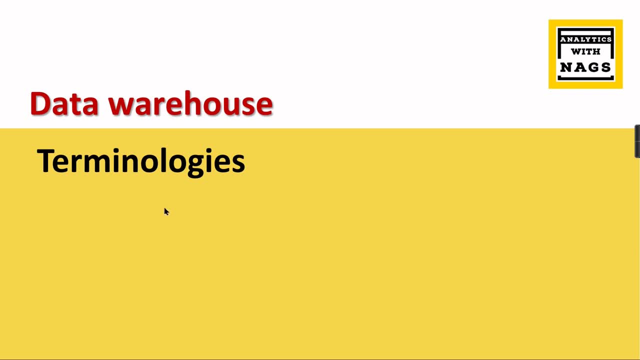 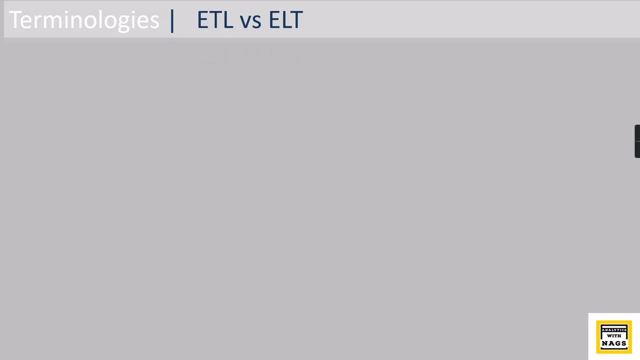 warehousing playlist. i strongly recommend you to watch that playlist. i didn't cover much of it. i whatever i feel that people should know before implementation. i have touched upon that in this session. let's start understanding what is etl versus elt? etl stands for external data warehouse. 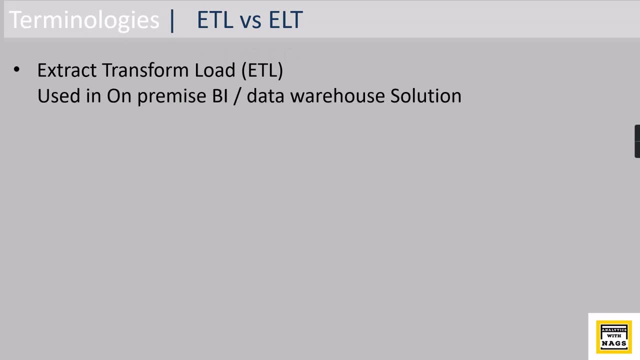 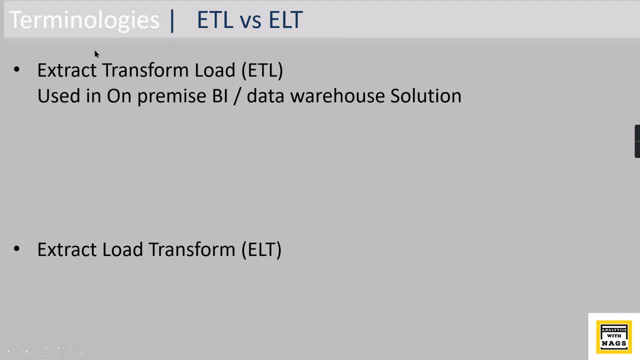 pure and extract, transfer and load used in on-premise bi and data warehousing solution exchange. and what about elt? ont enters for extract, load and transform. so just swap between the words, meaning like you will extract and do the transformation and load into a data warehouse. that is the main purpose of etl and 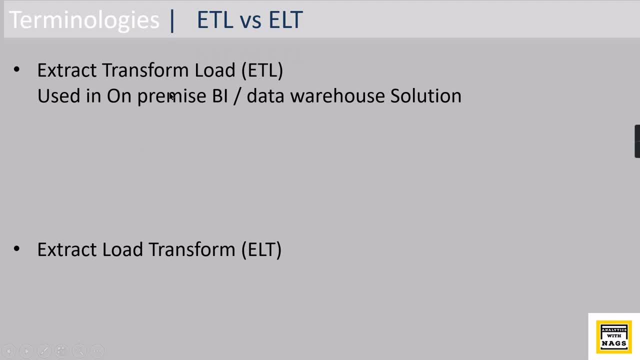 also in transform, you will do the cleansing exercise, all other steps as well. this means that this is typically used in the on-premise BI data warehouse solutions, whereas the extract load transform, that is, ELT, used in the cloud technologies. basically, in data lakes, you will store the data in a raw format. so those who has worked in 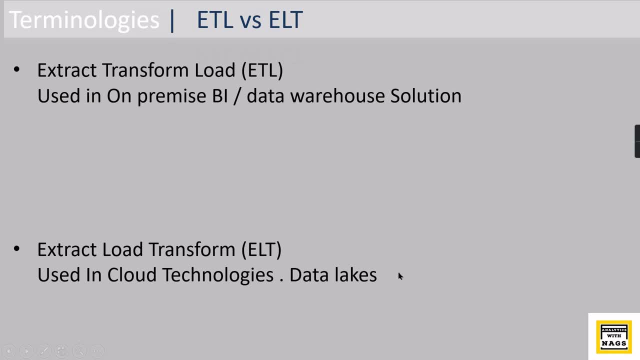 the data lakes they will have had, like how they will store the data. it is just like a text format or in a table format. you will store it so that is why it is called as ELT and mostly it's used. when you use the data lakes, they will call it. 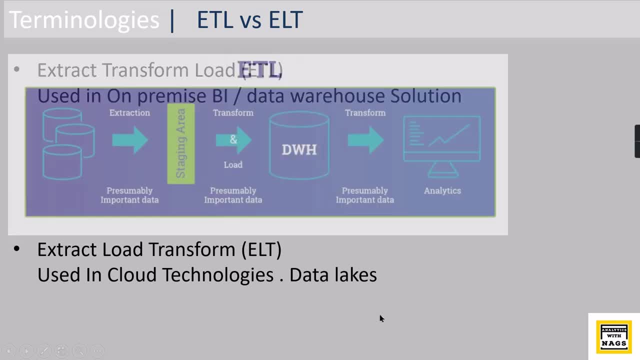 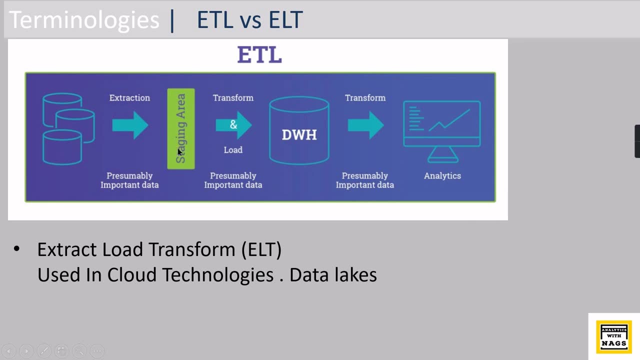 as ELT. okay, and to understand it better, you can see here: this is the typical data warehouse architecture where you will extract it and load it. right, I mean to say extract, transform and load. the end objective is data warehousing and you will extract and then transform and load it. okay, there will be confusion, like you. 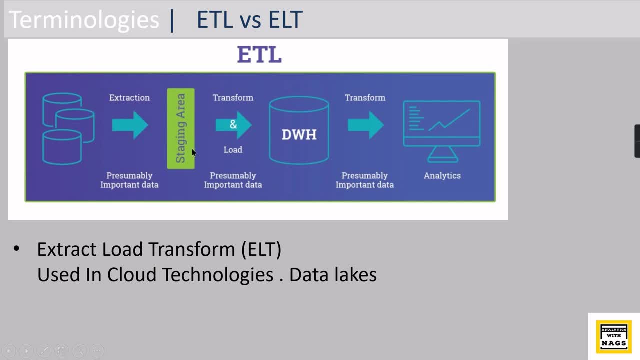 you say. you say like as soon as you extract you are loading it in the staging, but in this transformation it so I mean loading itself. you will do certain transformations as well: changing the data type, removing some columns, those kind of cells also considers transformation, and you will do that one. 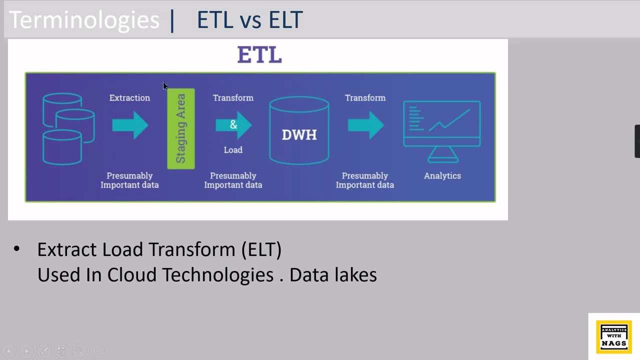 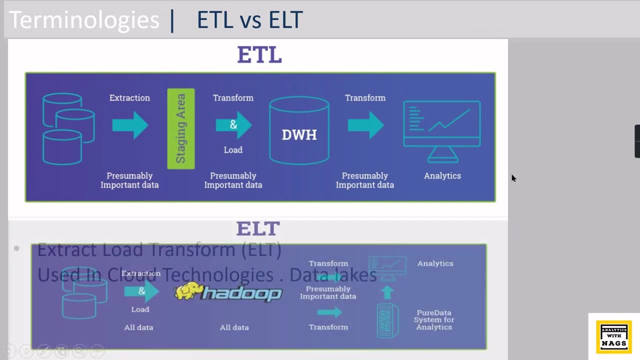 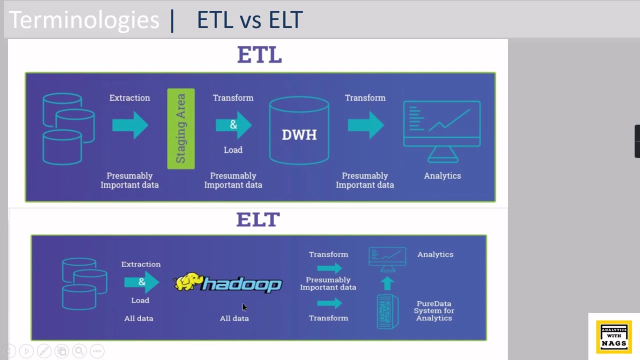 as well. okay, that is why ETL is mostly related to on-premise, and you will work while we work on it. you will understand it better. in case of ELT example, for instance, we will do an instruction, that is, πάng file and write. here we have a file called lsd, which is the one that will be used to create the 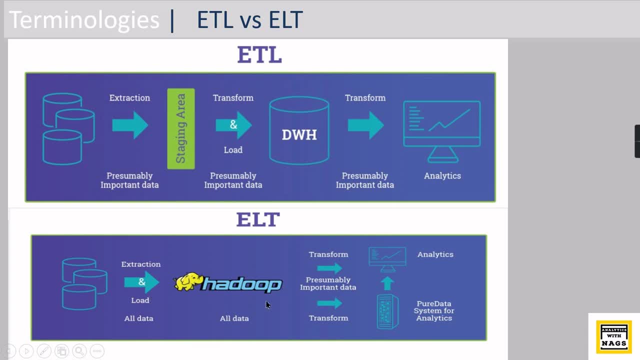 information for the files to be saved. that is called the lsd, and you will have two files here. you have the first file and the second file, and the third file and the third one and then the last. first of these is the next file and the folder. so that is why you extract loading. you are loading the data then, based on the requirement. 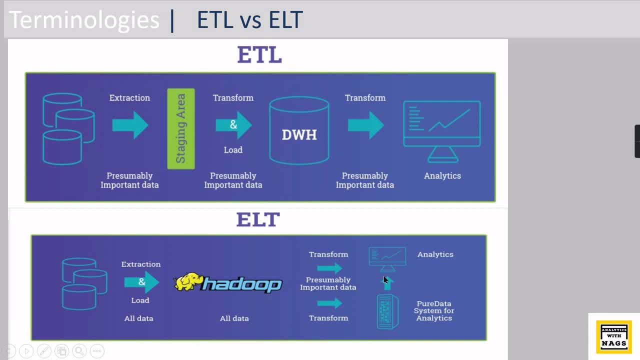 as and when required. you can transform any form right either. if you want three columns for one report, you can do it. here you want only four column, you can do it. but here it is very like. only you can consider as standard. you will design it prior to this. then you will create the standard. 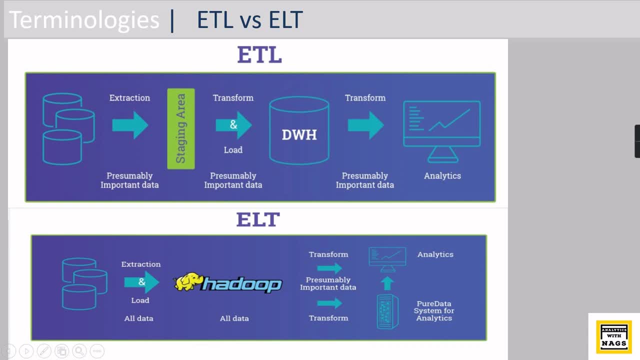 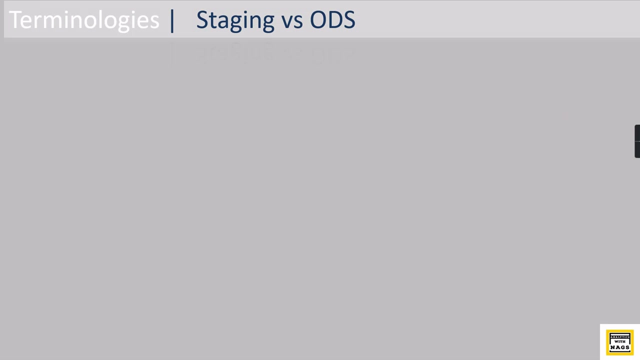 structure. you cannot keep transforming your data here. okay, that is different story, but to understand it in a single liner: etl- extract, transform and load- used mostly in the on-premise environment, and elt- extract, load and transform- used mostly in the cloud solutions. let's talk about staging versus ods. we all seen what is staging is. let's again discuss about it. 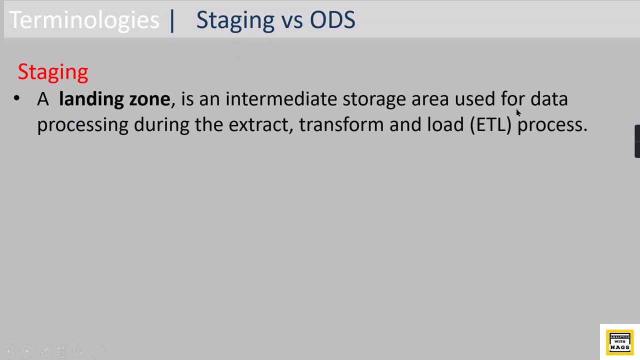 a land. land, the landing zone, is an intermediate storage used for data processing during extract, transform and load process, correct, if you remember the architecture. once from the source in the staging area, we will load it and do the transformation. i will explain it once again in the as soon as we complete this definition. so the data staging area sits between data source. 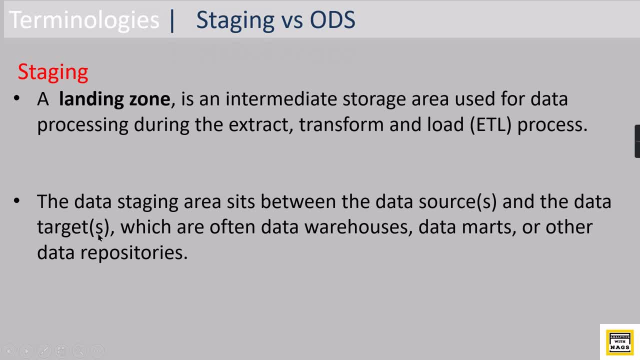 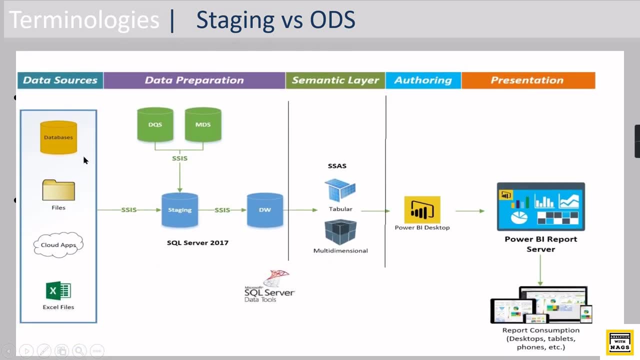 and the data targets. there are targets, in our case is data arrows, which are off in our data arrows, data marks, another data repositories, correct. so here we have our architecture, again, what it mean by staging. so this is the layer and in order to understand Nanodias, how the data processing happens, that is what we need to. 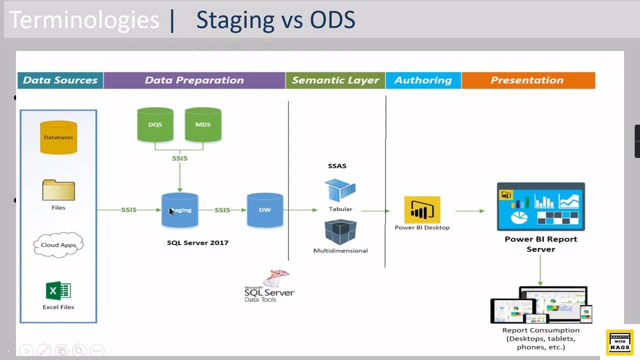 understand. so, once so the data has been extracted and loaded in the staging, you can apply some transformation, meaning, like you need to pi-jat your table, you need to pivot your table. and head up stage. meaning, like you need to pivot to a table, you need to unpivot your table. and now, when you put down your data совсем, in order to construct the setting like: so this is how it works, because once the data has been extracted and loaded in the staging, you can apply some transformation, meaning, like you need to pivot your table, you need to in place. 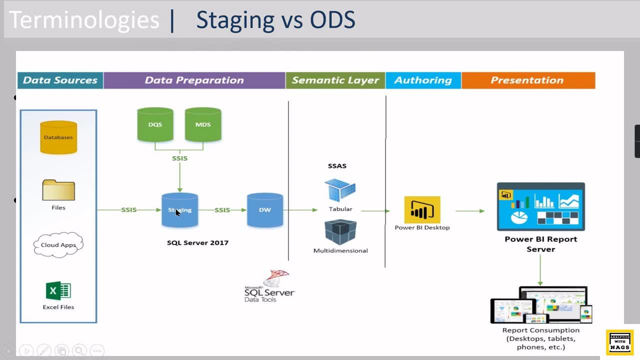 table. you can remove some logics. you are getting some duplicates in this data. you can remove it, right and you need to merge two to three tables and then get the desired results. so these kind of transformations, after you load it, you can perform it and then loading into your data. 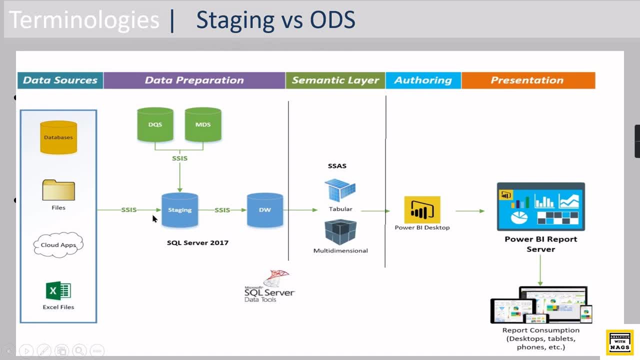 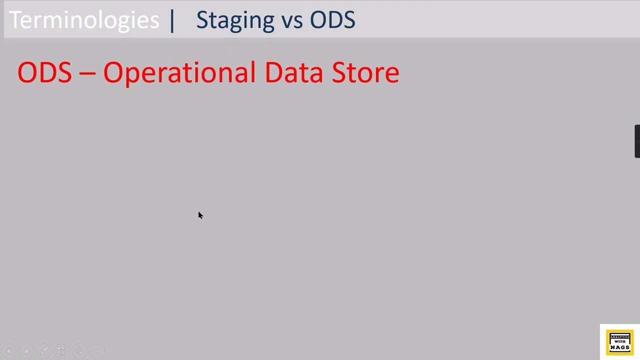 arrows. that is what your staging is. once you process, you can clear it. okay, clear means you can delete these records. staging, as the name indicates, temporary storage you can hold to while the processing happens, right until the processing happens. this is what a staging is. then. what is the ods? where does this ods comes from? when people use it, ods stands for operational. 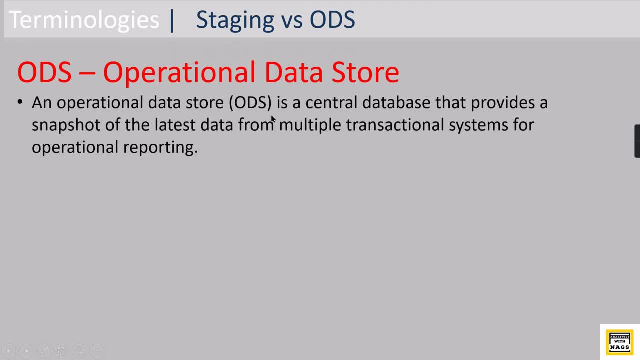 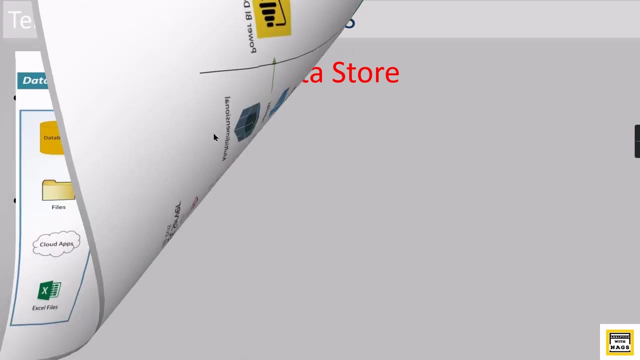 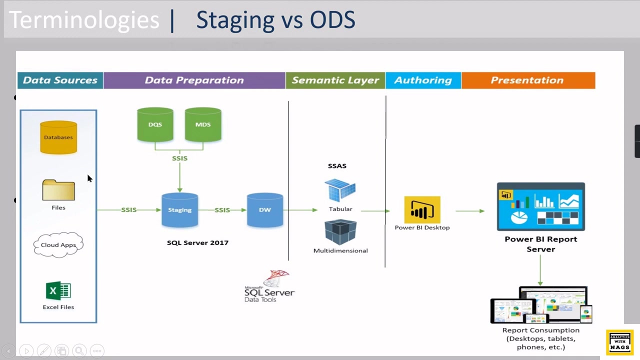 data store and other definition says like is a center central database that provides snapshot of the latest data from multiple transaction system for operational reporting. basically, like as we said before in the previous architecture, right, so you should not disturb the the we when you talk about why we need data arrows- we already discussed. like you should not disturb the databases. 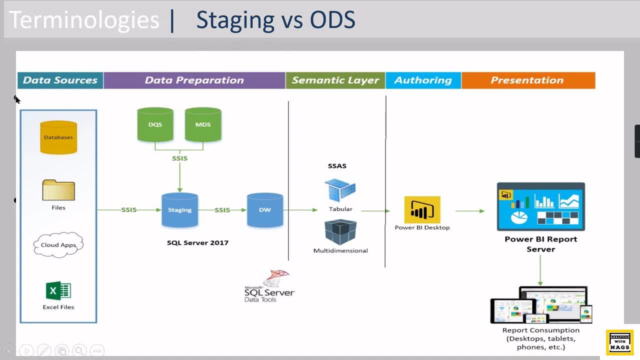 or operational system. because, for the reporting, because your operational system keep on inserting a data, someone is doing a transaction- sending money in case of banking, right, so sending money or purchasing from the online orders it in case of online shopping websites, then you, while for reporting, you should not disturb this database, so you need. 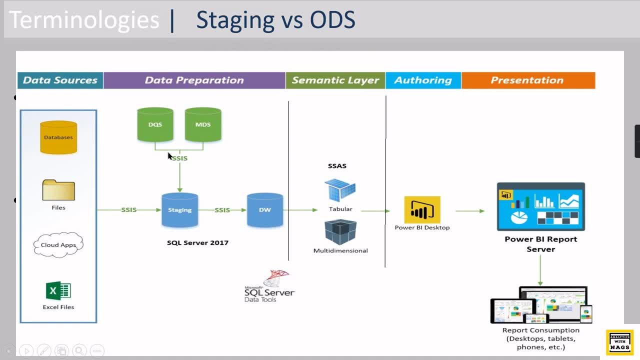 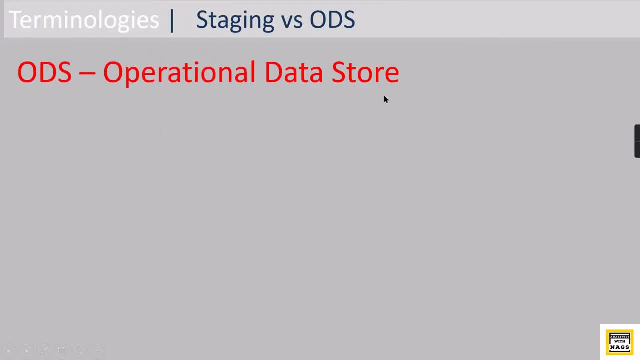 to have a separate system. that is why we are building it. so instead of touching this one, you can have a replication, one more copy. right? that is what operational data store and that is what you can see here. multiple transfer: it's a snapshot, okay, snapshot of the latest data. 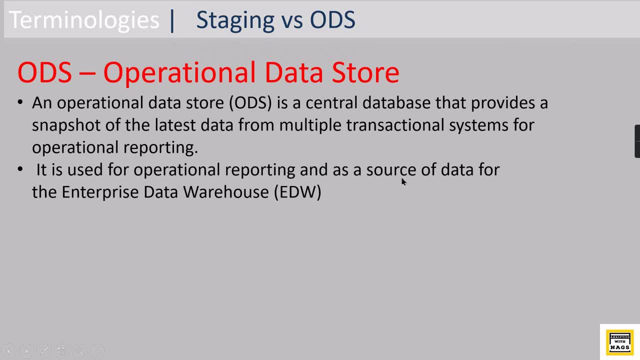 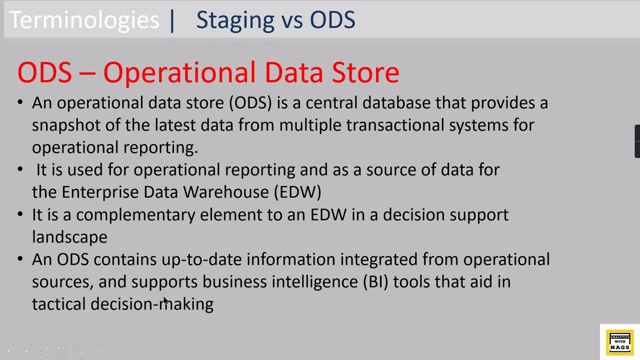 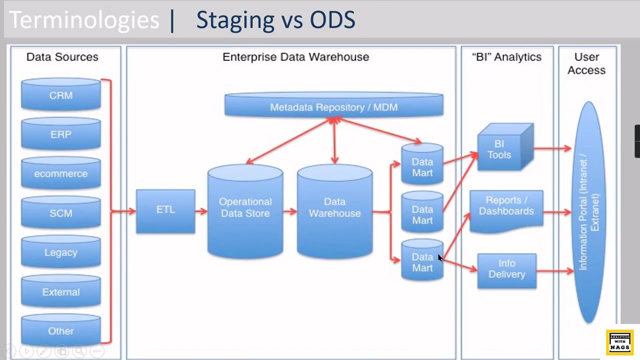 stores. it disuses some, the data from east to west, right, one more copy, more copy of this, one later. okay, so this is the data transfer method is like: okay, this is what I send. okay, I can go to this other side. okay, as same definition, the main difference, right, let's let me summarize this. so you have data sources. 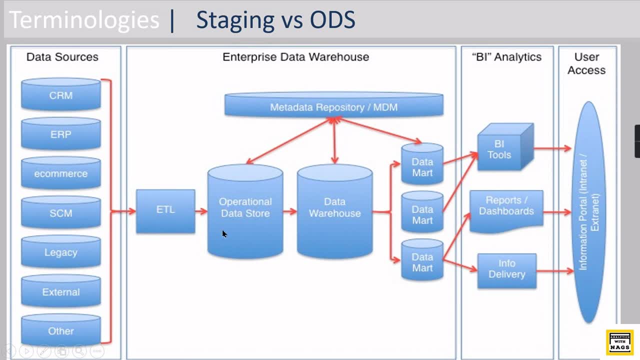 we have seen a staging here. using etl process you can store the same copy, the crm, erp, e-commerce, everything. you can store one more copy here. so whenever you want to reprocess your data warehouse, okay, you no need to touch this crm. say, for example, the the main purpose. okay, i'm saying when 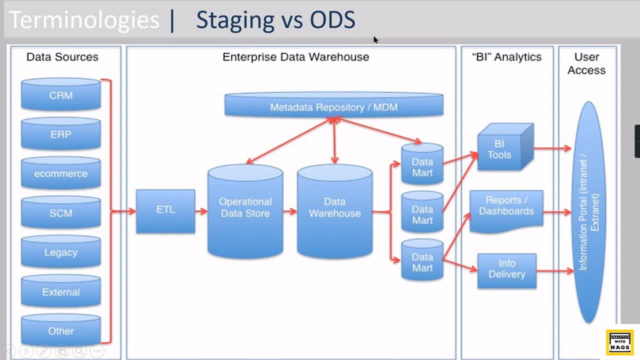 you can go. for people often confused with staging or ods: okay, staging is different staging. once you process the, you can clear it and then, once it is loaded in data warehouse, it says temporary staging area, whereas ods it's a copy of your source system. when we'll use it once you process, when. 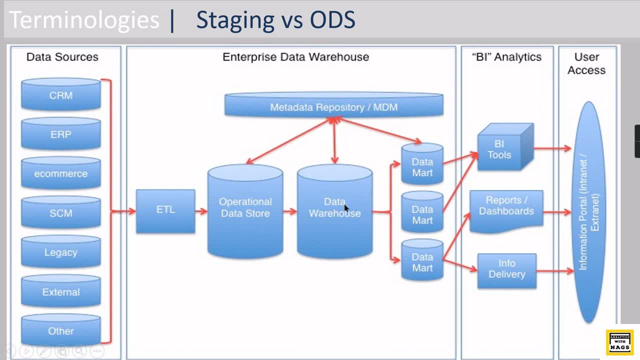 you want to rewrite your logics. you process this for 10 years. there are some times you need to reprocess your logic. for that you need to extract the entire source data. at that time this operational data store will be huge. but assume, like you are copying our entire. 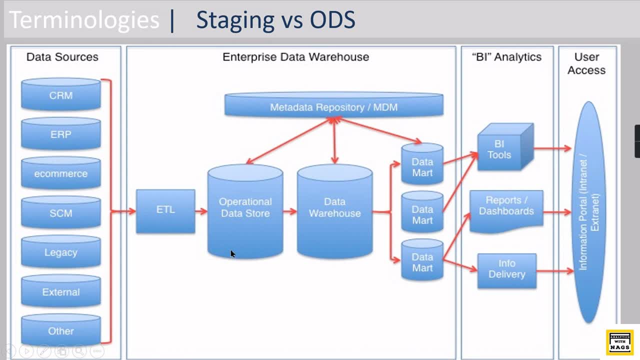 store here, then the cost will be another concern, right? so this is what ods is. this is optional. mostly people won't use it and they interchangeably use this staging as well, so in staging itself, they will use it. i mean, it's like the people often confused with it, whether whatever, they maintain it. if they maintain it, they DNS. it's the case like, for example, data storage is going to predict which and which one, and so on, forERS and so on. so previously we reviewed 19 że data storage, data storage options in the development document bottom of80, Wherever you are running a. 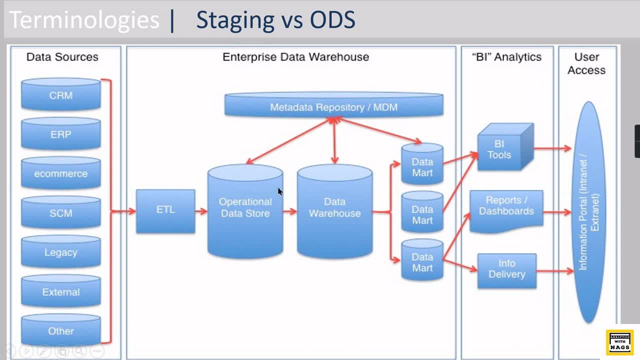 Web ran areations. if you use this as a open shroud, just do a login first here. when you click and maintain it, it is ods. if they are not maintaining, it is staging. that's it. it is as simple as that. and also people, some people, a proper implementation, they will also have operational store meaning. 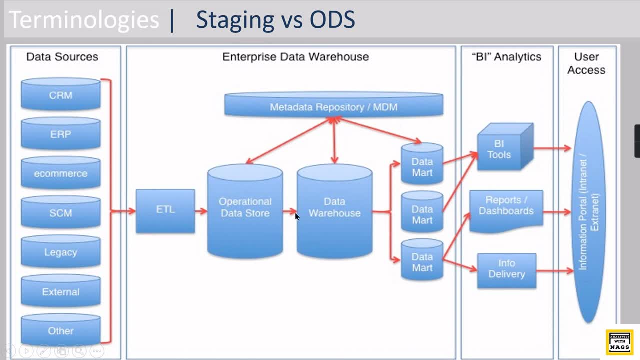 they will maintain the data, the copy of your source and also a staging to temporarily process. that is the proper implementation. but for now, because if you maintain or copy your data it will be to 2ds, we will ignore this. for our implementation, we will use only the the. 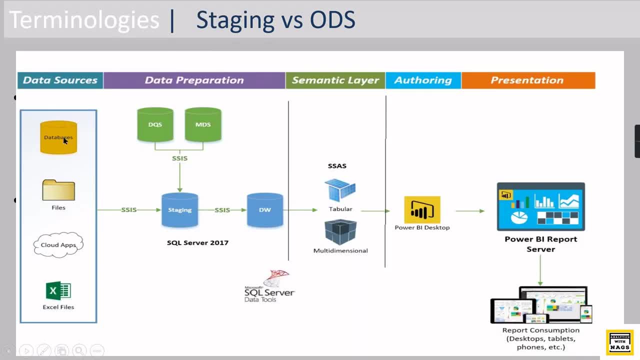 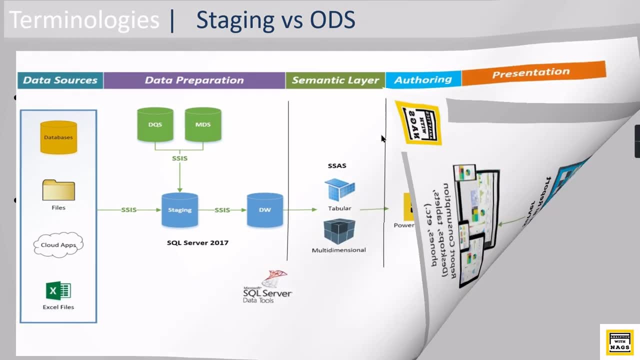 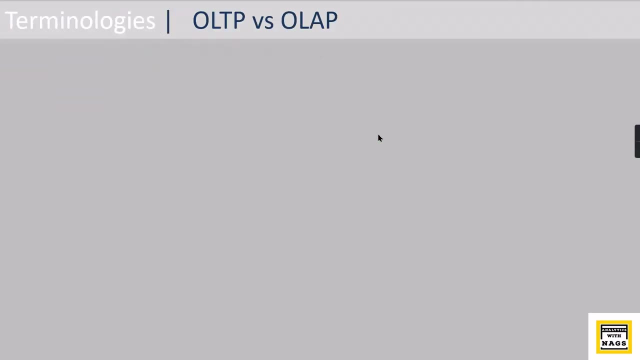 conventional, the architecture here, whatever mentioned, we will get this data, temporarily, store it, then we will process it. then, once it's loaded, we will clear it. that is what we are going to see in this demo as well. i hope you clear with staging and ods. let's move on to oltp versus olab. 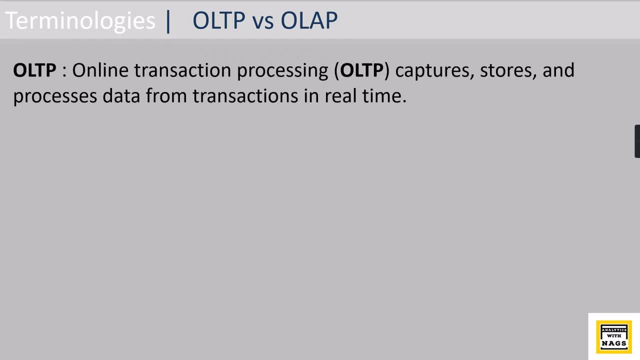 all tp online transaction processing that captures, stores and process the data from transactions in real time. as we mentioned, whatever the source systems we have discussed- erp system or banking system or websites that use it to process your um datas- are called oltp, right, so that captures and stores and process the data. okay, that is what oltp system and overlap. 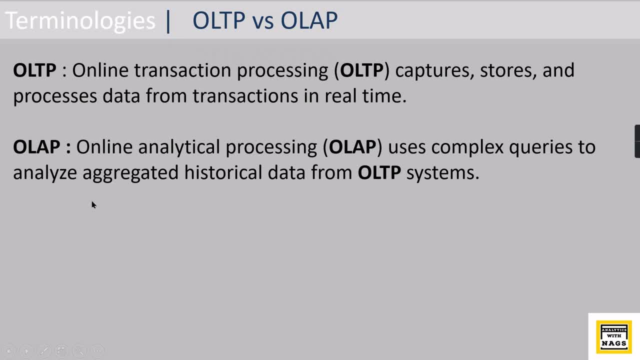 is the analytical um processing uses a complex queries to analyze aggregated historical data from OLTP system. OLAP system can be created only if you have generated the data from the OLTP system, which is nothing but a analytical processing. okay, that's used to process the or query the aggregated. 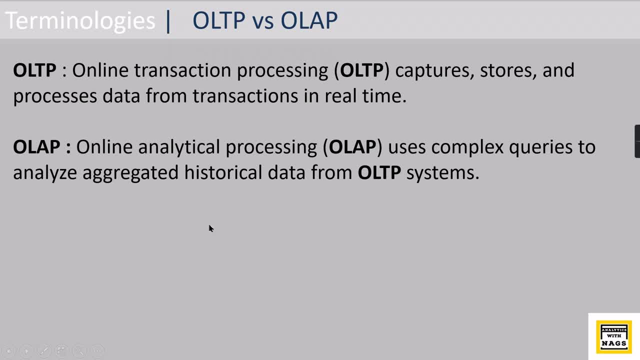 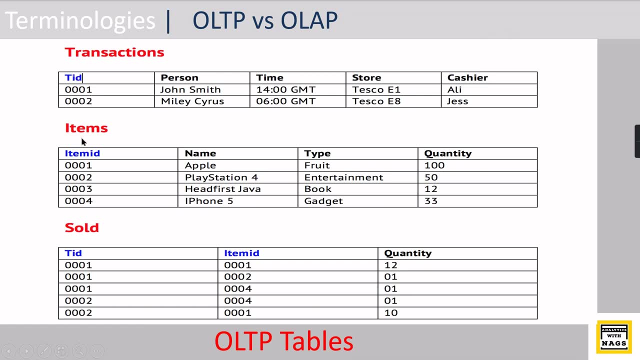 historical data. this is the code difference between OLTP and OLAP, how data looks like. in OLTP, data will look like this. you see here: transaction item. it is a two-dimensional data where you have rows and columns. okay, this is what a OLTP system. you can store the data over here, whereas the OLAP 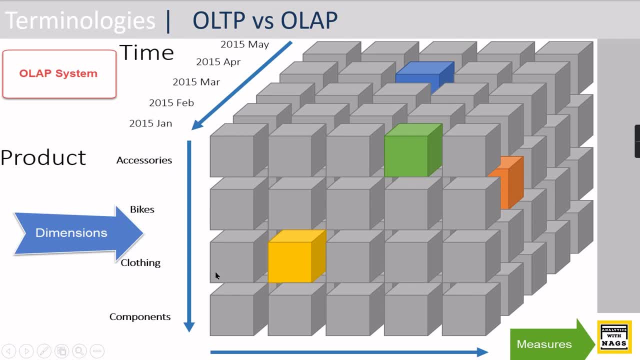 system which will store the data in the cube format. okay, this is three-dimensional cube. similarly, you will not understand you better. okay, the data will be stored in the OLTP system, which will store the data in the cube format. okay, this is three-dimensional cube OLAP system like this. okay, in order to create a OLAP, you need data varrows and how the data is. 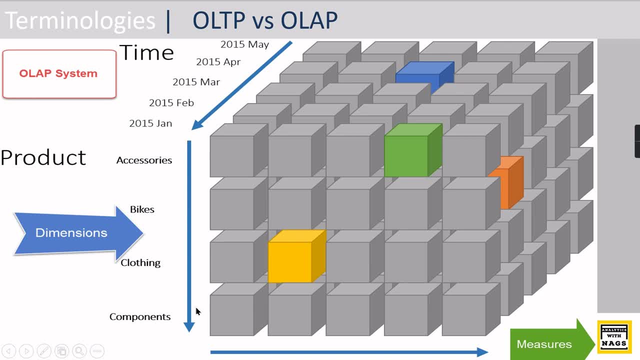 stored here. you can see it's a product right, one dimension, and you can consider this as another dimension or customer location. then the data is for time dimension and your measure will be stored here, meaning like what is this box indicates to me in accessories in this customer location, Chennai? 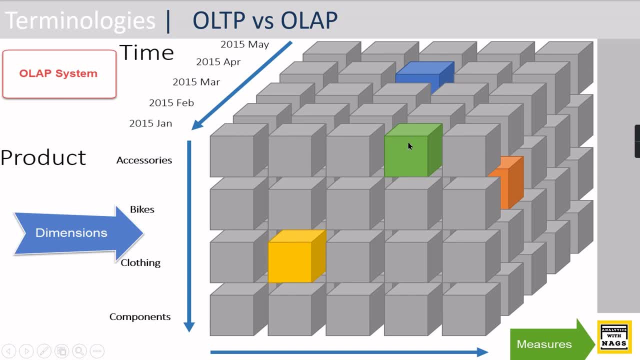 and 2015, Jan. this is my amount, right. so this particular dimension, this is what the how measure is analyzed in different dimensions for each possible combination of your dimension. right, there will be one cell. in that cell, the measure will be stored. right, because how, how, you can. 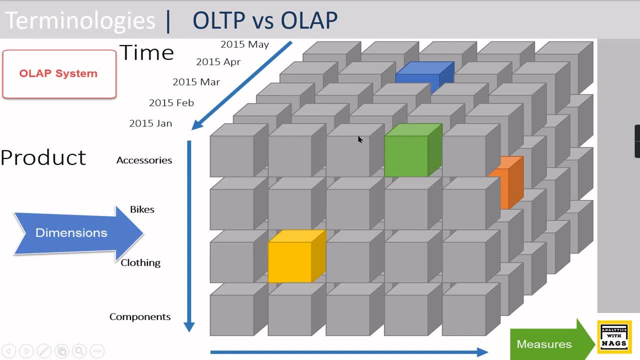 understand. this is like you in a at as a total of sales of your organization. you can understand this by using the data set, that the data set has a value of 1 in M, that you can actually see what this is and what is the value of this data set and what is the value of this data set. 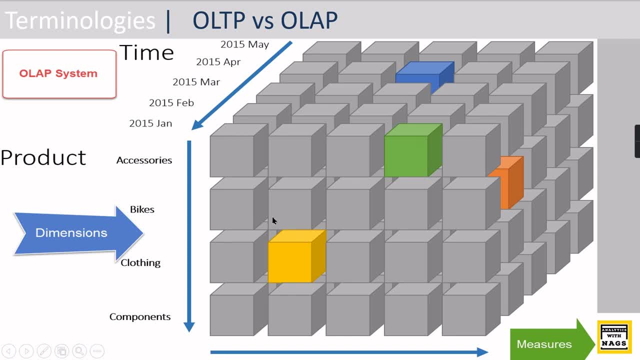 this is the value of. this is the value of 1 in M. that's exactly what you need to know. okay, what is in the data set? this is a value of, which means that you can see that here is a value of what your data set is currently considering for the entire organization, for. 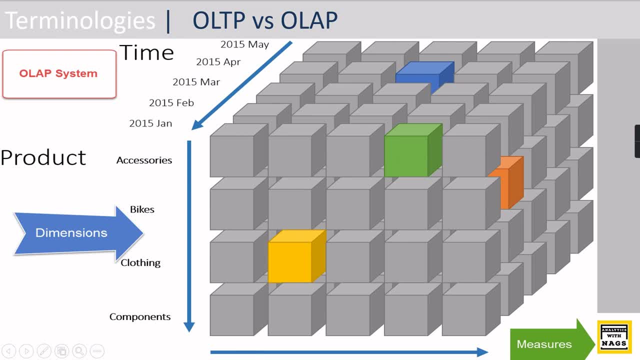 two. those I mean consider for entire organization from the beginning till this date. it is 1 million dimensions. for each possible combination of dimension, you will have one cell that will be already processed and stored. so when you ask a query like in this- accessories in 2015, what is? 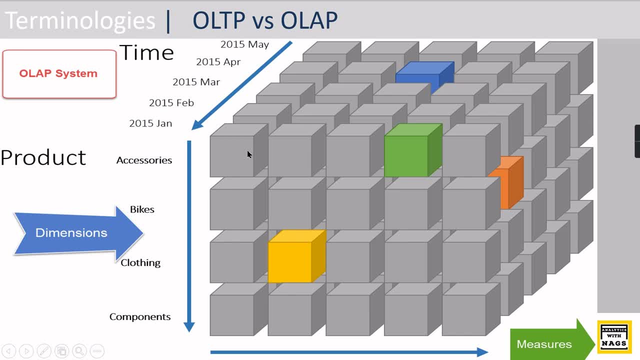 my sales. it will go and check the index, this particular cell, then give you the results. that is why your this olap system is meant for querying. it will be more faster than your typical two dimensional table queries. okay, with this note we will stop. this is the main purpose of oil all up. 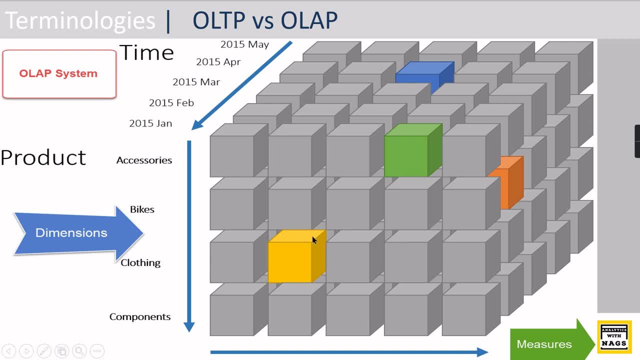 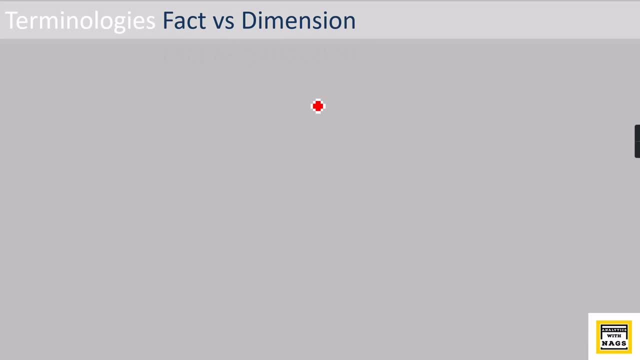 which is meant for responding to the queries quicker. let's try to understand other terminologies, facts and dimension. so ultimate aim of data warehouse design is to build a dimension modeling. a dimension modeling is nothing but design your fact and dimension for a particular data matter. so, without knowing this definition, it is. 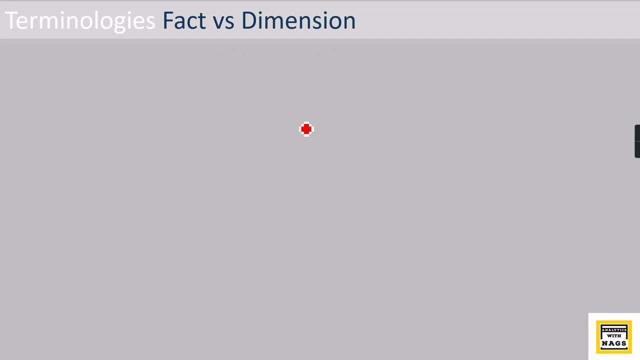 no use of designing your data warehouse, so try to understand its definition first. so, fact, how you can analyze is like what you want to analyze is your fact and fact table contains a measure, along with foreign key references, of your dimension table. so basically it contains your numerical values. it can be sales amount, quantity or it can be a production defects. 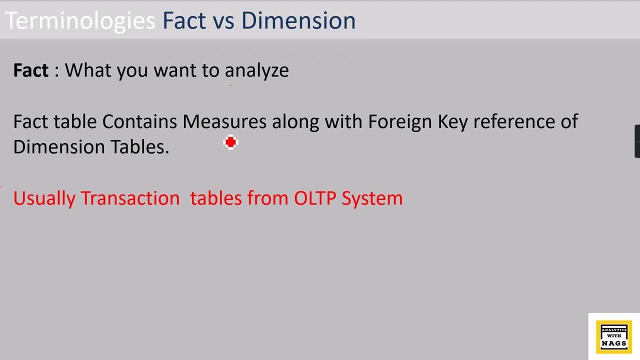 number of defects. those can be considered as your fact and it will have the foreign key references of your dimension table. this is what your fact table is. usually. a fact table will be a transaction table from the OLTP system in case of banking system. whatever you do transaction, sending money or 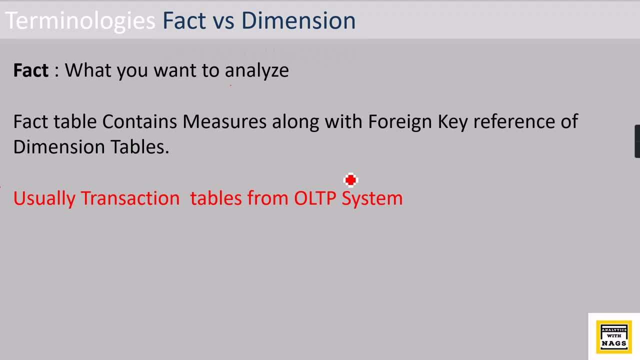 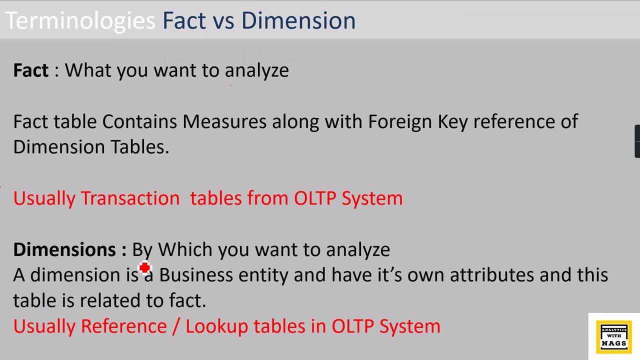 POS point-of-sales right. if a customer is doing one billing, that is considered as your transaction table, so those tables are considered as your fact tables. what about the dimensions? so dimensions are nothing but by which you want to analyze those facts, meaning like you want to analyze the fact. 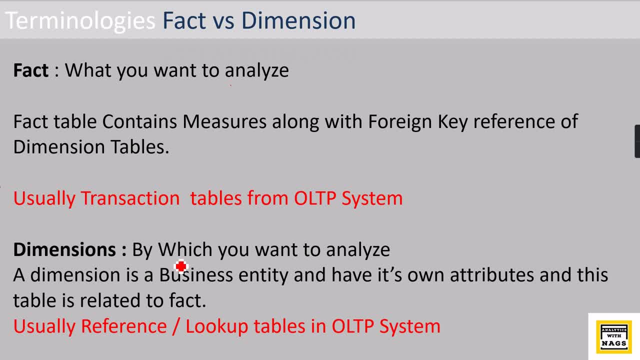 let's say some out by customer location, by store, by which time it has been done or which year it has been done, right so, by which you want to analyze the fact, it becomes your dimension. basically, a dimension is a business entity and have its own attributes, and this table is related to the fact table, why it is mentioned like it has its own. 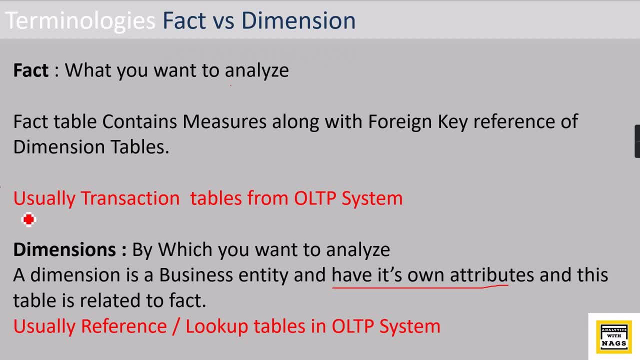 attributes meaning like: if you see a dimension table, consider customer, it will have a gender and it will have a maritial status, all those things. in case of location, it will have a region and group right, so it has its own attributes that is not related to other dimensions. that is why it is mentioned like that. so this is the typical. 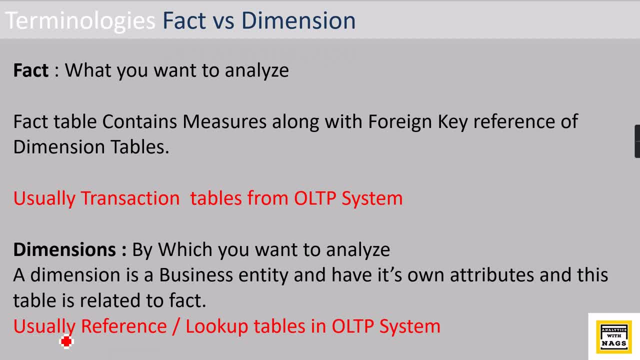 definition and usually your dimension will be like a reference table or lookup tables in the OLTP system, meaning like you have a customer master, when you have something to drop down and you will filter it, then those things are considered as your dimension tables. this is how you can. 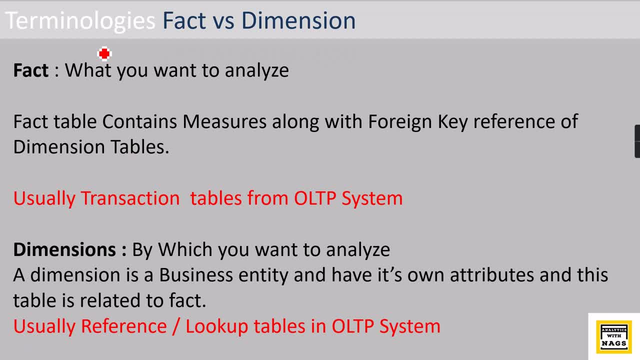 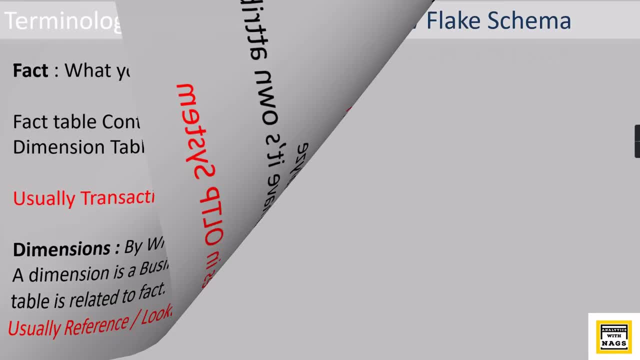 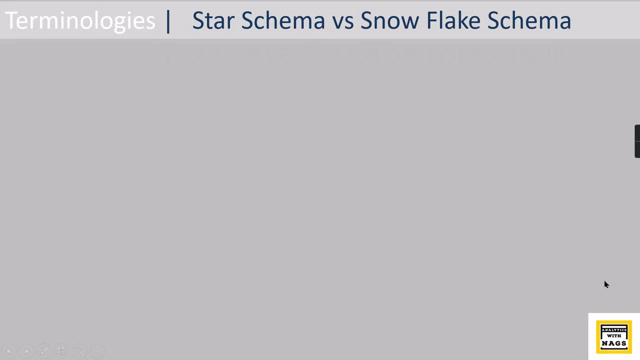 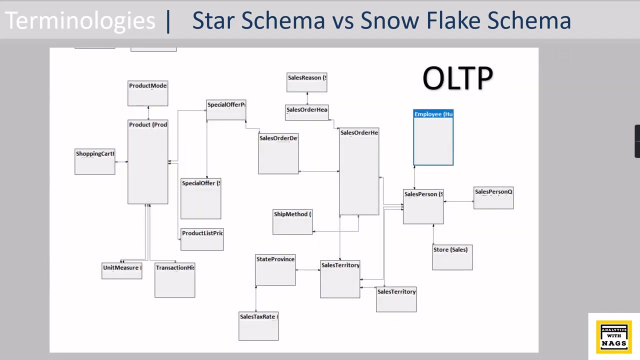 classify tables from the entity relationship model as a fact and dimensions. this is what i want to highlight. let's start understanding about star schema. i have talked more about star schema in various videos, either in power, bi and data browsing concepts or in ssa as well, but to understand it better, i quickly walk you through again in this video. so typically, 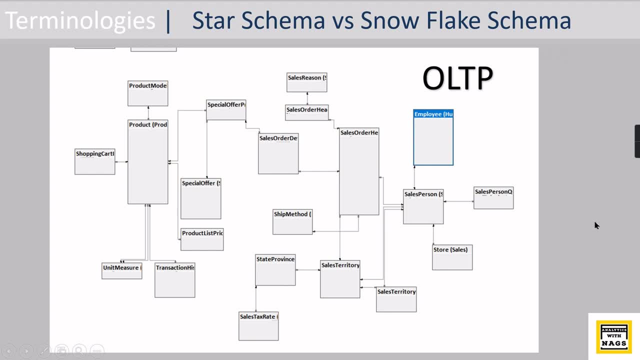 the ultimate aim of star schema or data warehouse design, is to build a dimension modeling. so this is the entity relationship model available in the OLTP system and from where you need to convert into a star schema. so what is the advantages of it and why you need it? 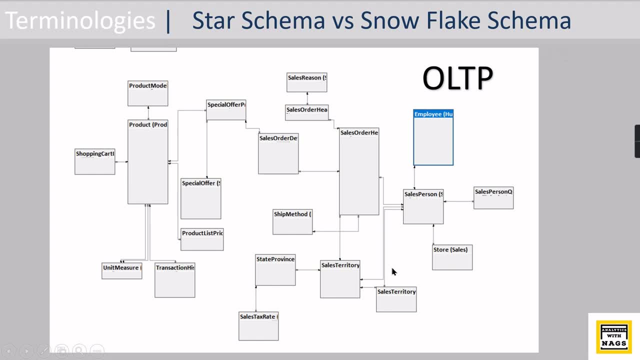 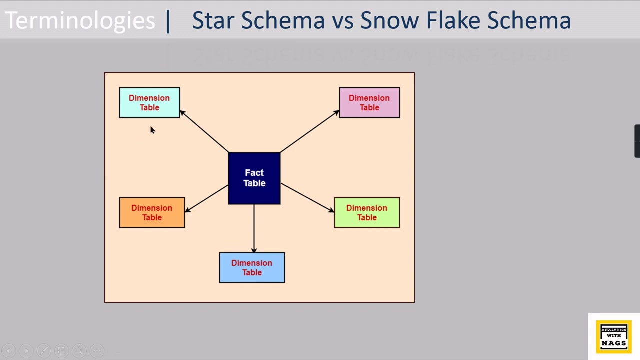 and where you can build your own волtthis model from the origin, or if you have a kernel Network where you need to build a study, and if so, what are the advantages? it is the main purpose. so the for me to say is we have entity relationship model that is meant for ol tp. 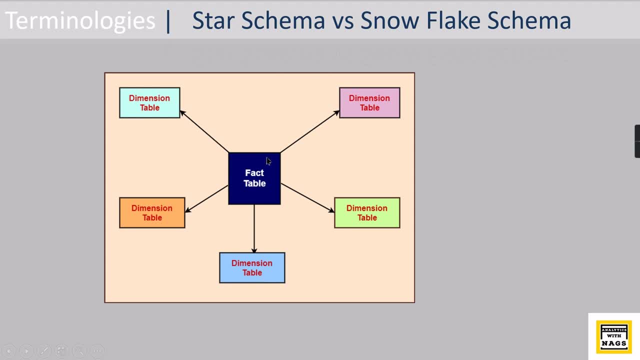 that. i want to explain it clearly so that that is the main purpose. basically, what i am trying to say is this: we have star schema, a fact table surrounded by a dimension table- so let me take a pen here- and this is considered as a sales, as we seen in our previous slide. whichever a transaction table is considered, 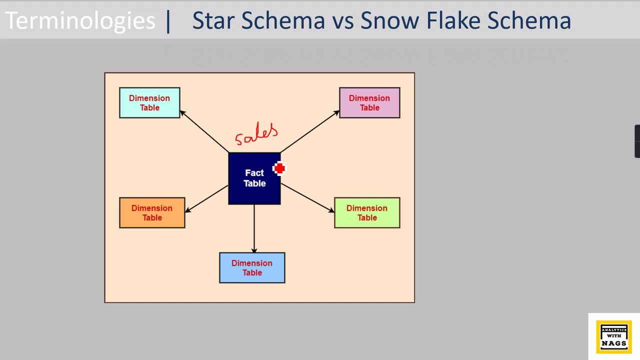 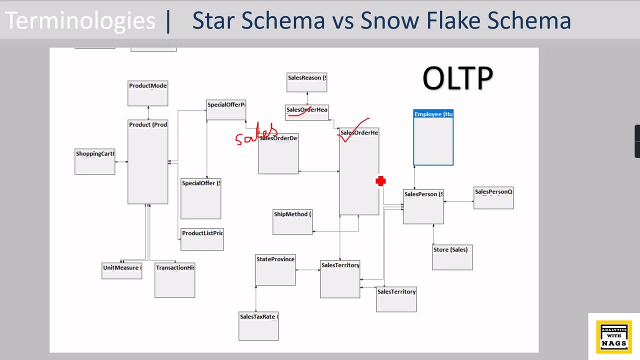 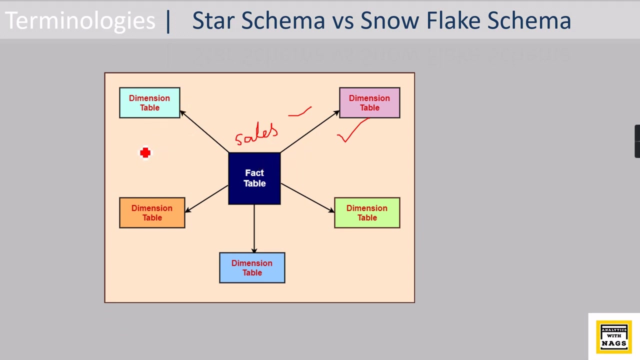 as your fact table right. so in this case you have a two transaction table like sales header and sales header detail. okay, while i am demonstrating these tables in the implementation phase, you will understand so how we can merge it right. so this becomes your sales table now. so from this, what are the different reference table? this understanding will come from business. 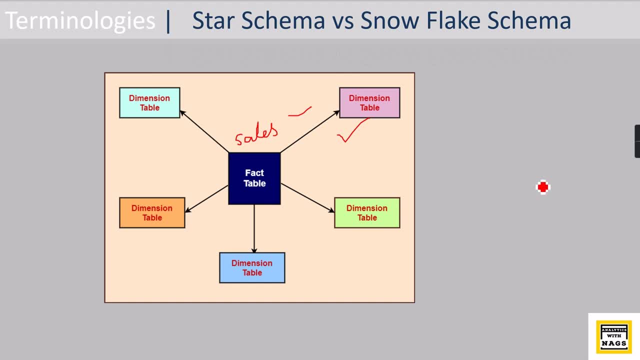 like what they want to analyze, what are the things they do not wish to analyze? right, those things comes from the business. so here you need to decide. from the transaction table you will create one fact table and what are the attributes that is related to this fact becomes your dimension table. so this can be a product, okay. 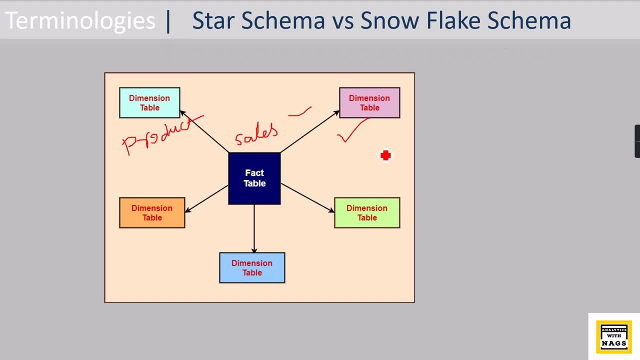 and this can be a customer, and this can be a date, okay, and this can be a location or geography, whatever it can be, and this can be a promotion. so there are different dimension you have decided, then, from the entity relationship model. you cannot have the product table as such simple, as such available directly. 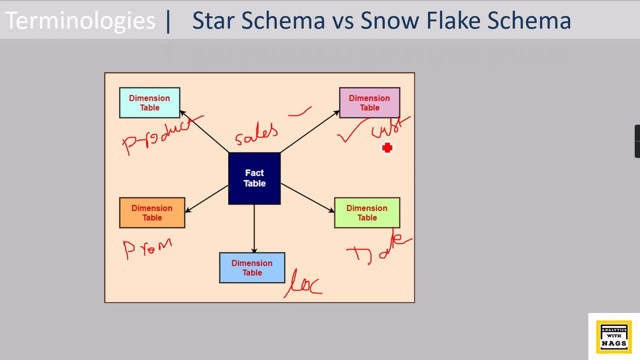 over here. it will be product, product type, or it can be a customer, can be entity model. while i am showing a demo, you will clearly understand you. in the entity relationship model, these tables are not straightforward available, so your task mainly focuses on bringing those tables into this dimension. 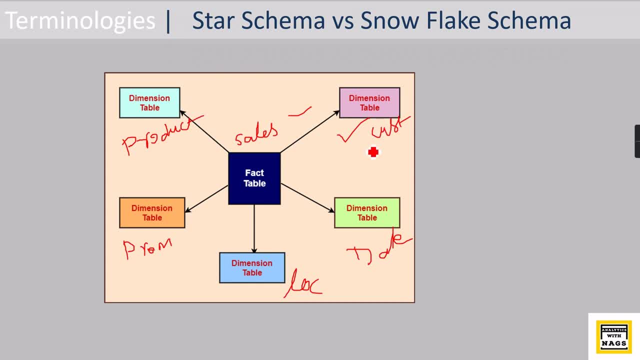 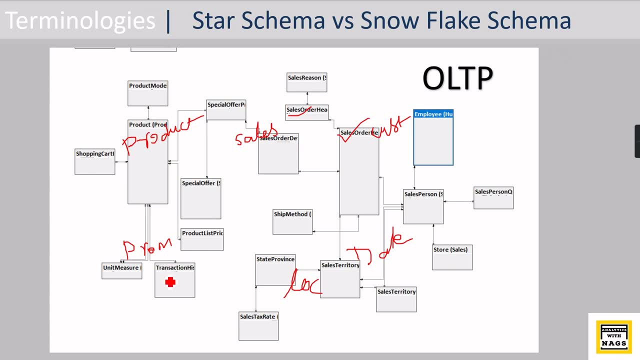 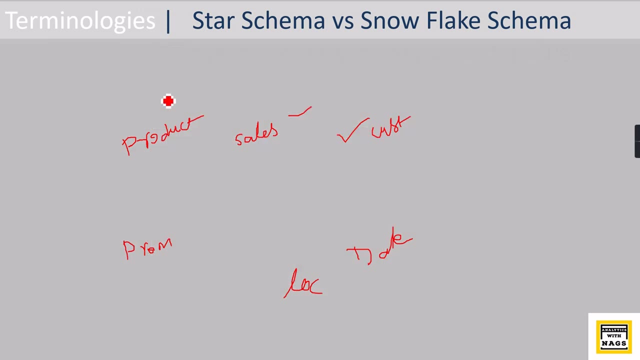 modeling table. right, so lets start with costends. so what can you do to attack and – so let us take one such example: uh – like uh – product, you have a product over here, product and uh, you have a product, uh, umm mode. you don't have a product subcategory here. 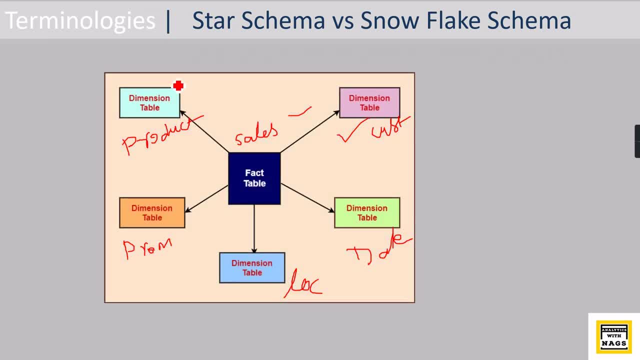 maybe it will be disconnected somewhere – so you will need to combined from that 1,, 2,, 2,, 3, 4 – 4 tables. then you need to bringing it into a single table. this is the very challenging part, okay –. 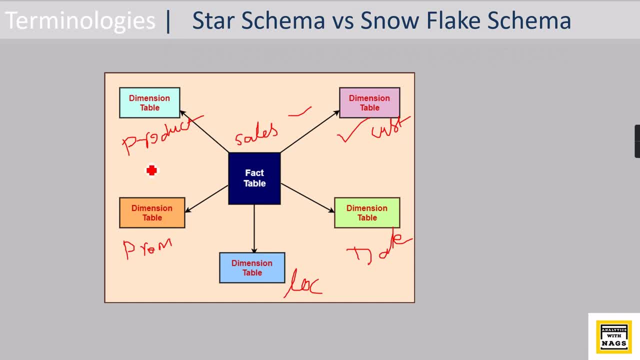 so once you decided these are my fact and these are the dimensions going to be act in this star schema, then you will implement it correct. then what is the advantages of your star schema? so basically, like we have seen, the OLAP system. the OLTP is entity relation. OLAP is meant for 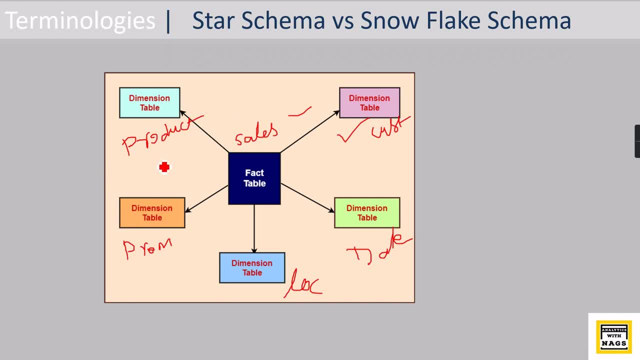 querying how. this star schema is very quick and fast. that is what you need to understand now. assume this product contains this. as I said, the I'm going to demonstrate one business. this business is having hundred products and there are around thousand customers and they are running the 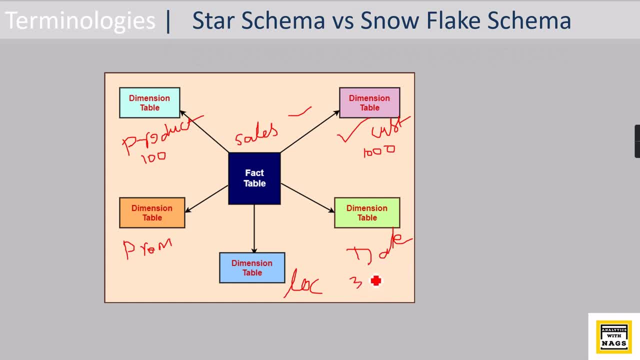 business for three years. so 365 into three, it's around a thousand eighty, okay, something around that, and you have a location. they have four, forty location, I think ten location, let's say ten locations. then they have two to three promotions they have so for each dimension table. 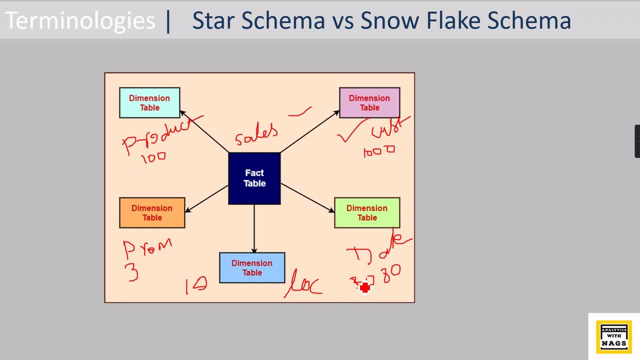 you have hundred products and thousand customers, and there are one thousand eighty days, right, and there are ten locations and three permissions happen. so based on these combination, only your sale is going to happen, right. so in your fact table there can be a transaction for this product and this customer. some one of the customer has brought on this particular date and this location. 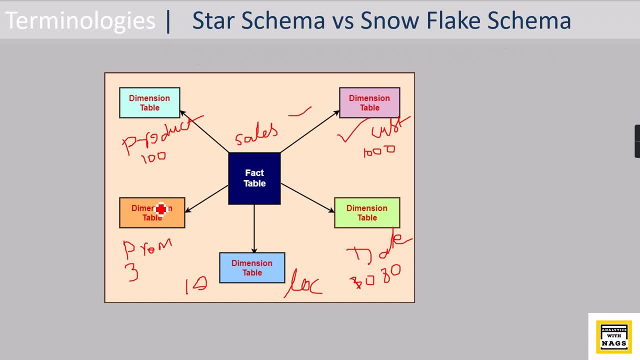 and is done this transaction using promotion? okay? so, basically, all these questions are all this. any questions will come from only these dimensions and combinations. so how we need to calculate is like: so, hundred products into thousand customers, into three promotions, into ten locations, in two thousand eighty, okay it, these combinations may come around. one point two. 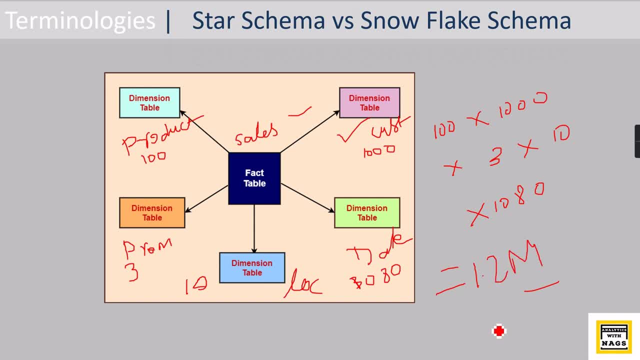 million combinations are more than that. I didn't calculated it will be more than that. okay, so these possible combinations are pre-aggregated. okay, this particular product, this particular customer, this particular date, this particular location, everything is pre-aggregated and can be stored in a cube format, not to cube. to work properly, you need to. 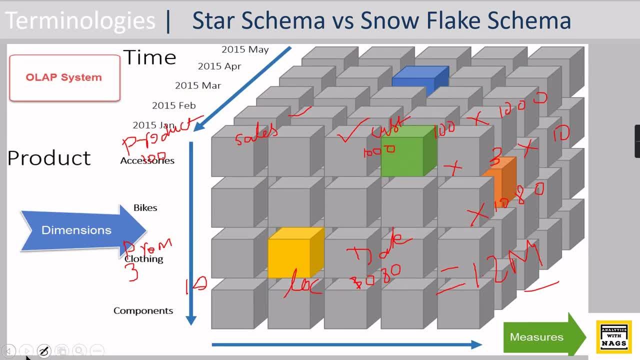 have a proper star schema you can see here. let me clear it out: this highlighter- sorry, there is all kinds of this. so now you can see this is what I said. so there are four products here. I mean this can be category and the time dimension is. 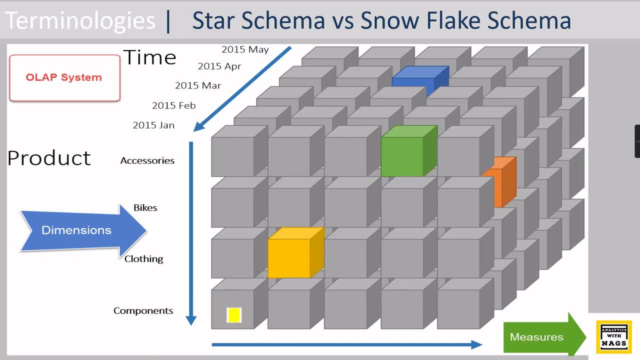 over here and this can be another dimension. so, as I said in the OLAP explanation, so this component in this particular location in this January 2015 sold, or how much this will be pre aggregated right say, for example, it is 50 sold here and this is sold as 60. so when you click on and click querying the 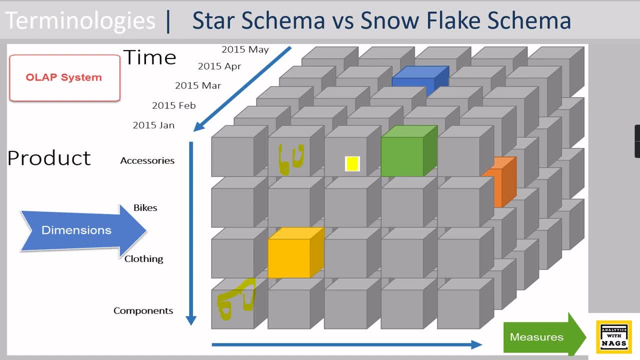 OLAP or star schema right, the accommodation will be very quick. the the main purpose of star schema is that you're able to build a cube on the edge of the point. that is why it is important that you build a cube on the edge of the point, because if you build a cube on the 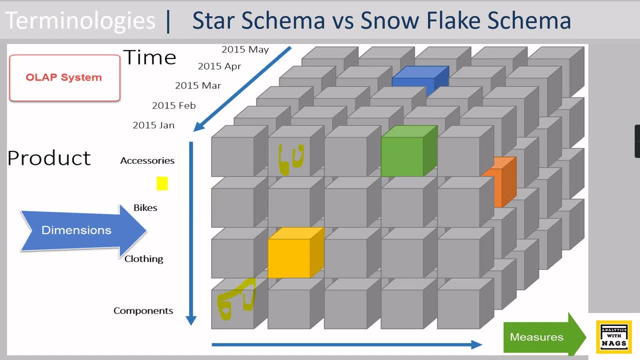 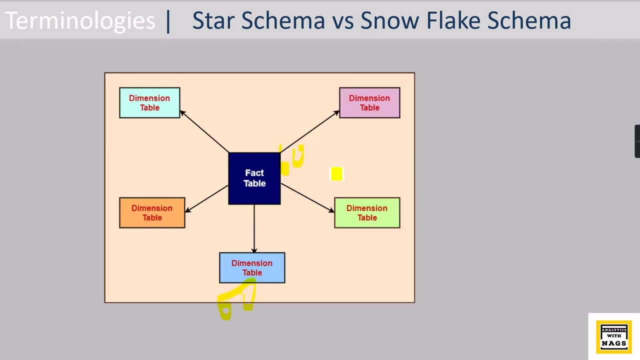 edge of the point, the boundaries will be too fast in responding, because you have a proper relationship between fact and dimension and once you build a cube it will be super fast, big. why? because those combinations are already computed and stored here, so you just need to reference to the pointer. that is why it. 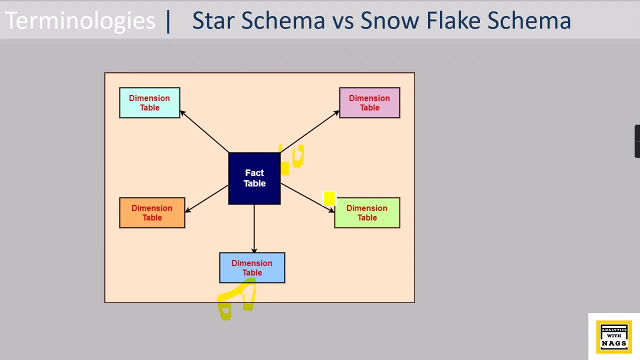 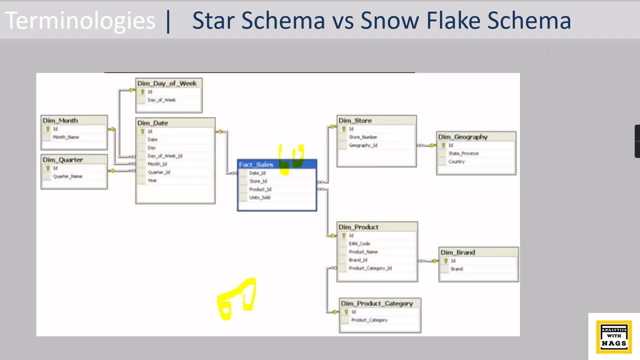 is fast entity relationship OLTP system to your star schema that I am going to demonstrate in couple of minutes. so next thing is all about snowflake schema. so there is no much difference. the snowflake schema, the fact table, is indirectly connected to a dimension table. you have this dim brand. 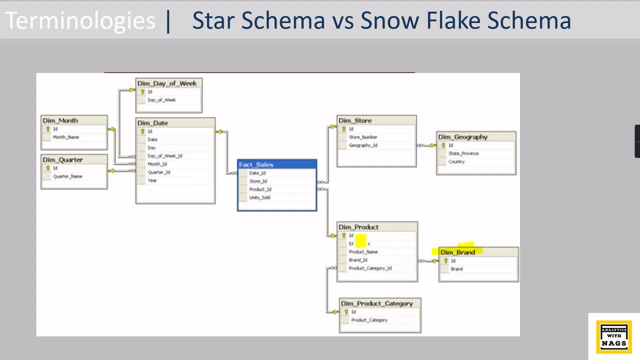 it is not directly connected to fact. instead it is connected to a dim product. so there are some dissonance. I mean design requirement, where you have this brand, description is more and you have a lot of products over here, right, 10,000 products- and this brand is three to four brands. 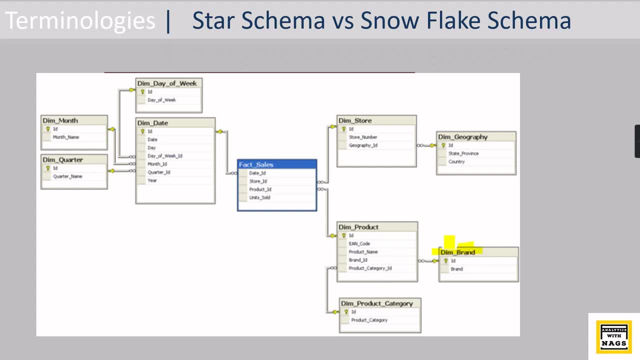 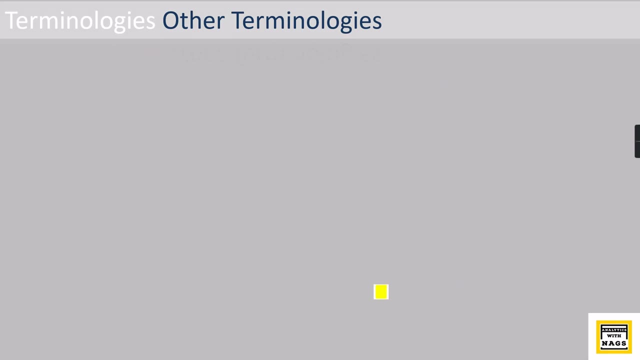 only that is, keep on repeating. so in order to avoid that such a things, we can go for a snowflake schema. so this is the another terminology you need to aware of. so there are other terminologies where I'm not going to cover these things in deep. 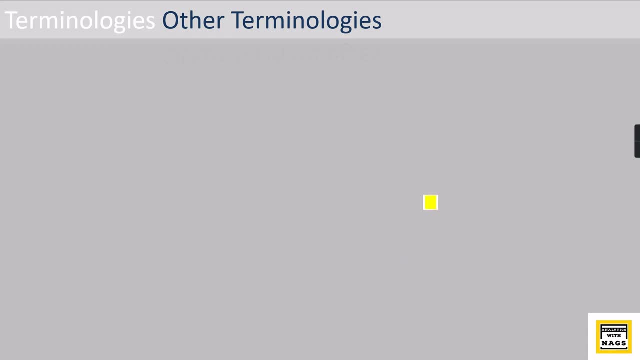 because if I keep covering, we will it will be taking more, much more time. as I already covered these terminologies in my data arrows playlist, just go and watch it and while implementing, I will come across one or two concepts here so that you can relate. so what are those conformed? 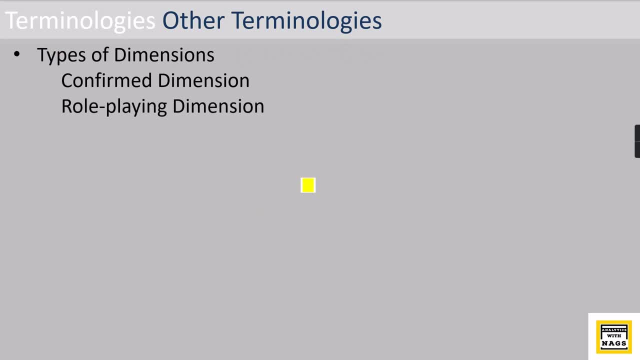 dimension. basically, I am going to show you how to do that. so I am going to show you how to do that basically, there are different. once you decide a dimension, right, fact and dimension. so these are different types you can classify: conformed, role-playing junk, degenerated, slowly changing. 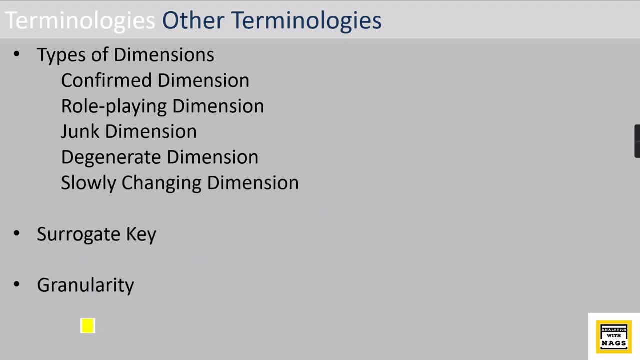 dimension and a surrogate key: granularity and cardinality. so whatever I said before, the 10 products in 200 customers and into some three promotions. this is called a cardinality. what is the? how much the cardinality your dimension is meaning? how many rows it contains. right, that becomes your. 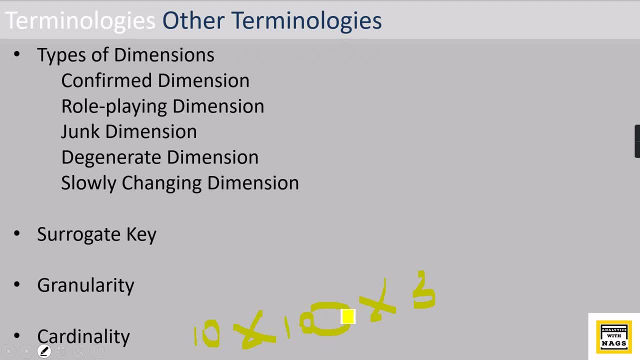 cardinality. basically, based on this, if your customer dimension is huge for online transaction portals like Amazon or Flipkart, you have millions of customers, so, cardinal, it will be very much right. so, based on that, you need to properly design- and what do you mean by granularity, like I am doing? 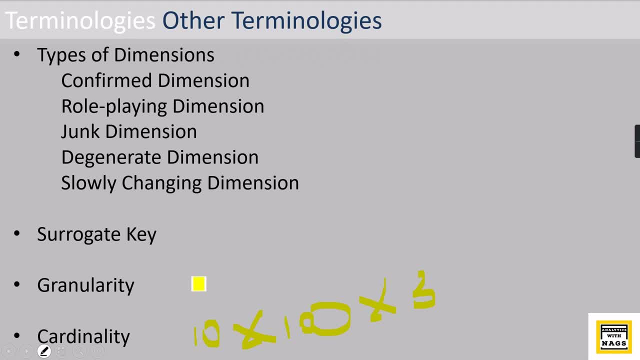 the transaction at the every minute. so in the form of transaction in a transaction at the every minute. so in the form of transaction in a transaction in a transaction at the every minute, so in the form of. So instead of maintaining my fact table at the minute or seconds level, I can skip those minutes. I can have only the date right. that is your granularity. the least level you need to maintain is your granularity. 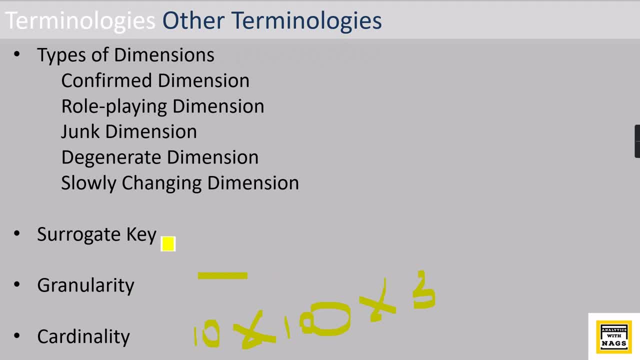 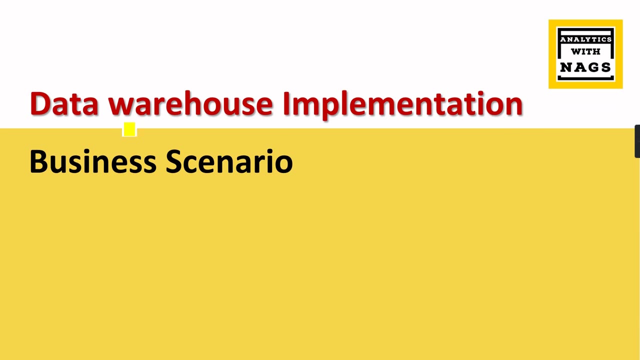 So this I want to make you very clear, And while I'm implementing data warehouse, I will talk more about surrogate key. So these are the some of the terminologies. you can learn more in my data warehouse playlist. So let's jump into understanding the business scenario for which we are going to implement a data warehouse. 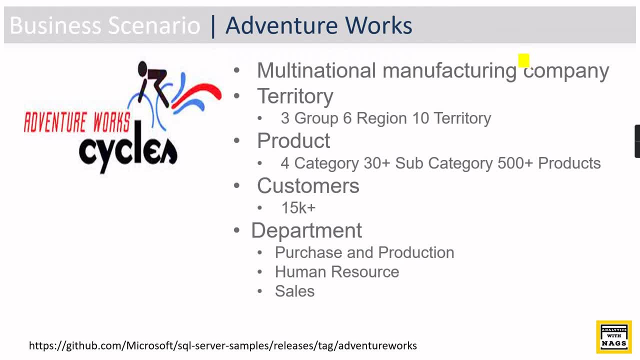 So it is not new, some of the people who are already familiar with AdventureWorks. So AdventureWorks is the Microsoft fictional OLTP system And for that they have designed the data warehouse as well. So this is readily available In the GitHub Microsoft SQL Server samples release tag: AdventureWorks. So this is nothing, but in this you can go and get the AdventureWorks OLTP database because we need a source system. that source system you can get it from this GitHub link, OK, And from there you can download it. 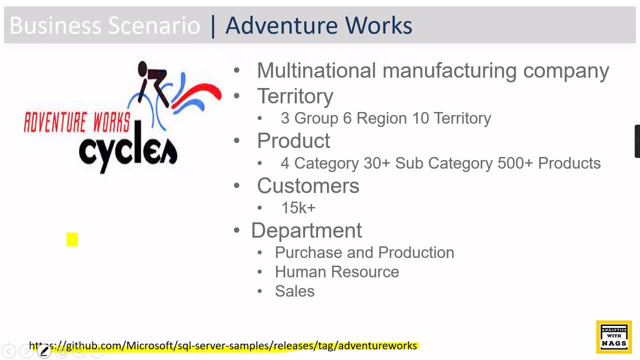 And then you can install the OLTP system. ready for that OLTP system, we are going to build a data warehouse that. I will walk you through this implementation step. let's try to understand this business. so this is adventure. works a manufacturing company? right, it is a multinational manufacturing company. 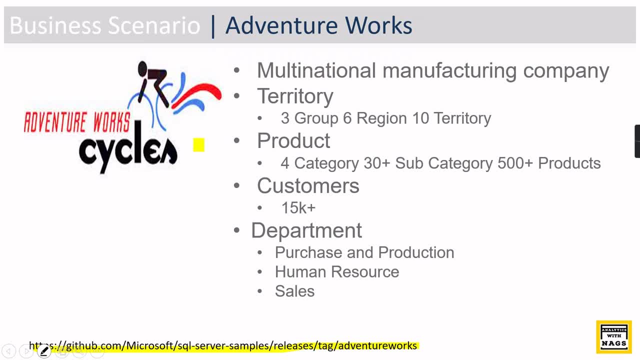 and they manufacture cycles and that's related products. so they have a three group, six region, 10 territory, and they sell products across four category, 30 plus subcategories, 500 plus products. the products can be a wheel or handle or pedal or entire complete cycle or mountain bikes. 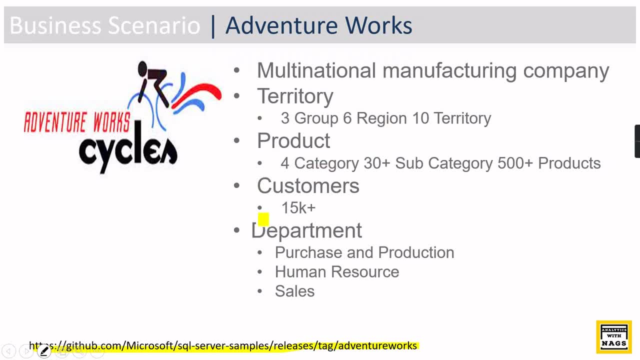 something like that. okay, so anything considered as a product, they have 15k plus customers. they have different departments- purchase, production, human resource and sales. so they do not have any data warehouse yet, assuming and we are going to build it. so what we are focusing on? we will focus on sales and human resource, and they have finance department. 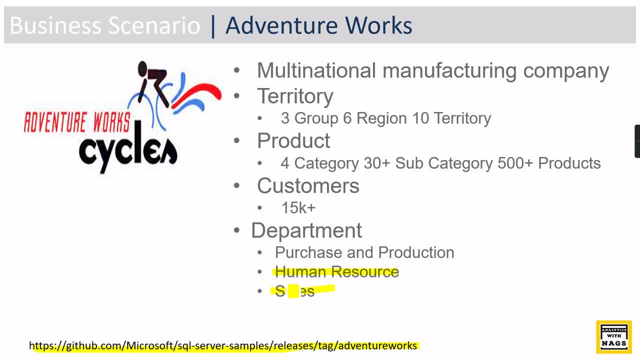 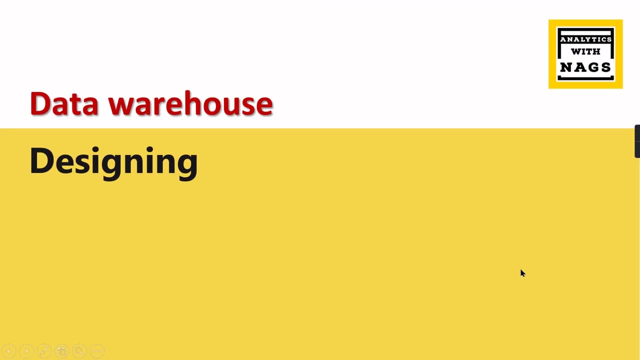 as well in the OLTP system. we will focus on these two and we will create the two facts here and human resource. one fact that the main objective of this implementation session. so we have seen our business scenario for this business. we are going to do the design of data vow. and we are going to work on adding and removing surveillance cameras are doing now, assuming that the day there is no data arrows has been designed prior to this particular adventurfoworks business- we are going to start from the scratch, right, so right from a how a data can be designed, those things, i'm going to cover it. the first third is covering it. the first three. 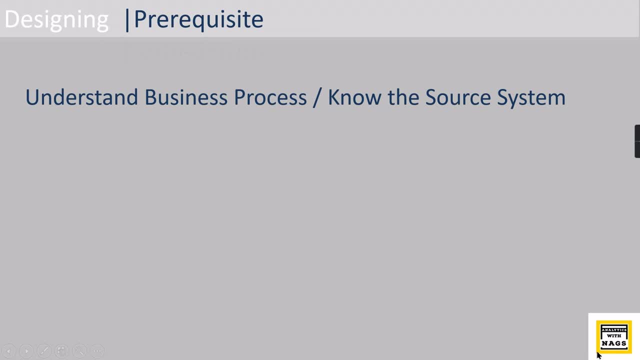 prerequisite is stood for the design for the data warehouse is to know the business process, that is, OLTP system business process, and know the source systems. what are the data coming from, where it comes from, what are the different systems they use, right? so this is the main prerequisite and for that 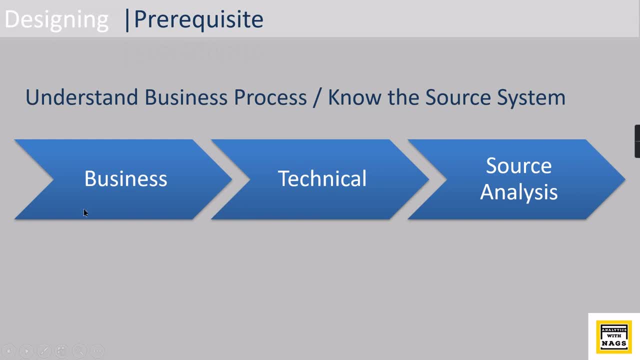 there will be different discussions happens like it. it is from the starts, from the business. they are the initiator of this process and they will explain their OLTP system and there can be some people that they have a requirement for the data arrows. what are the expectation from the business for the data arrows? 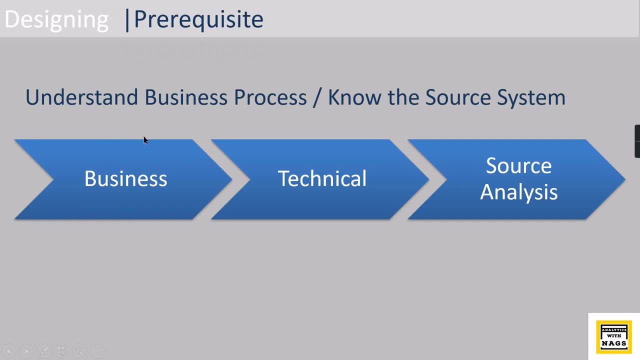 both the things can be done from the business side. then, from the technical perspective, there comes the architecture of the OLTP system. they will explain that the data is coming from where it is coming from, where it is coming from and how their business process works. they will show the tables, they show the 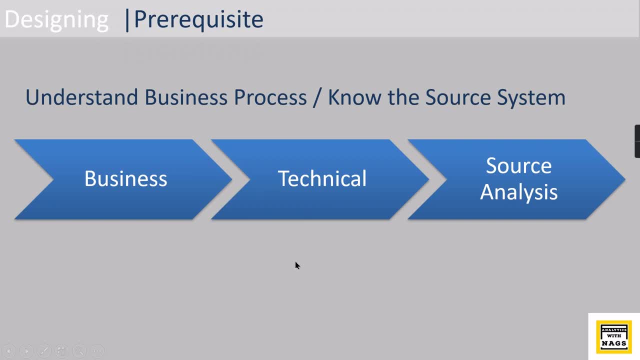 applications and with some current problems with applications, those things, so that only a proper data warehouse can be designed. then, if there is some chances, some people will provide access to source analysis, meaning like they give access to the databases so we can explore those who are designing so this 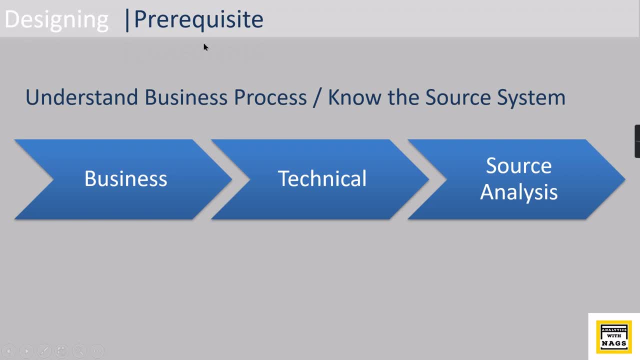 is basically the basic structure of the OLTP system. so this is basically a designing phase. this is not for the early starter of the data warehouse people. this is for the senior level people who can be a five to six plus years of experience in data warehouse design- how they can design the data warehouse. basically, there can be a 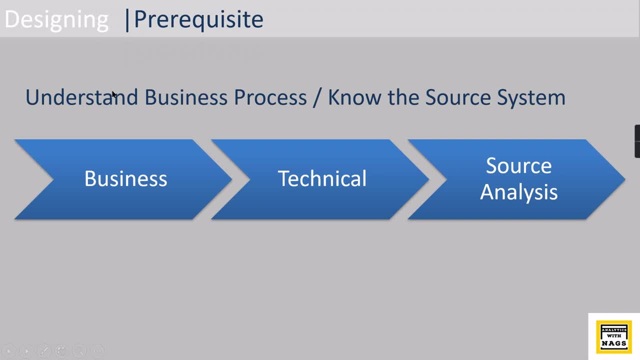 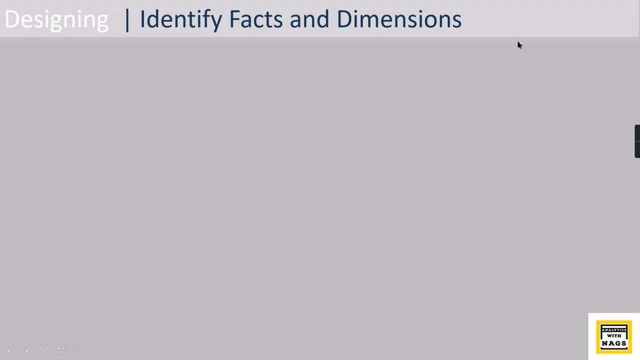 architect or they can be a team lead or consultant role. so the ultimate aim of designing is like this: like we identify the facts and dimension right. so how you can identify it's based on the subject area you can. first you need to classify a subject area. what are? 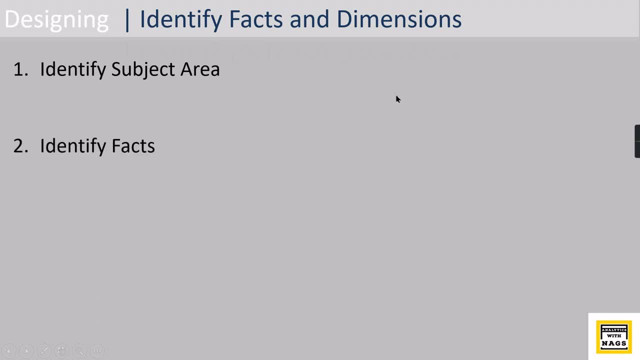 different subject area a data warehouse is going to have, and then we will have how many facts in that subject area and you have to identify dimension and its types. then you can set the granularity. so, as we said in our previous slide, it is business process, technical analysis and 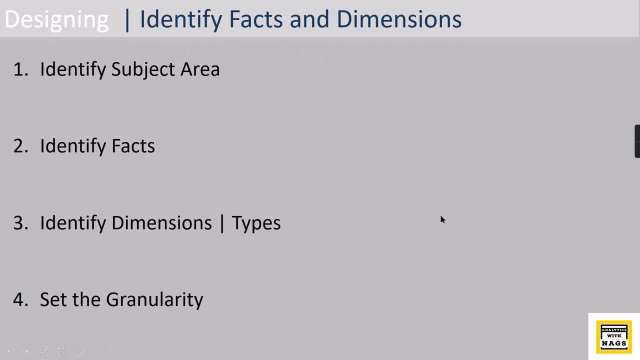 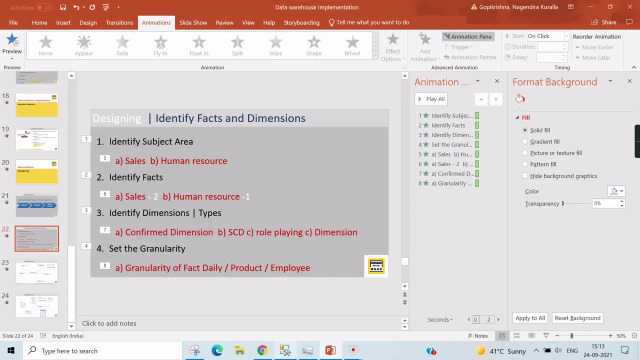 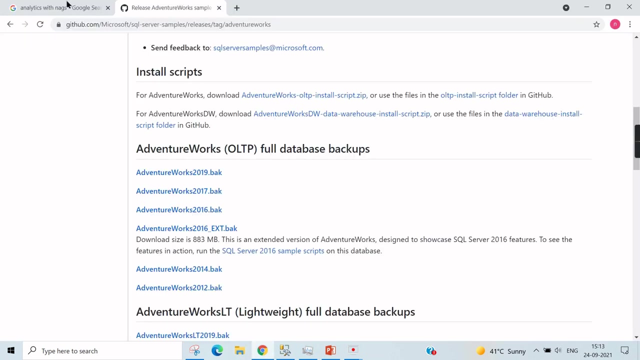 source analysis and let us try to go and see the adventure works business database and we will do some technical and source analysis. then we will come here and identify what we are going to do now. so I am in adventure works. this I already explained, as I provided in the link, the Github website. 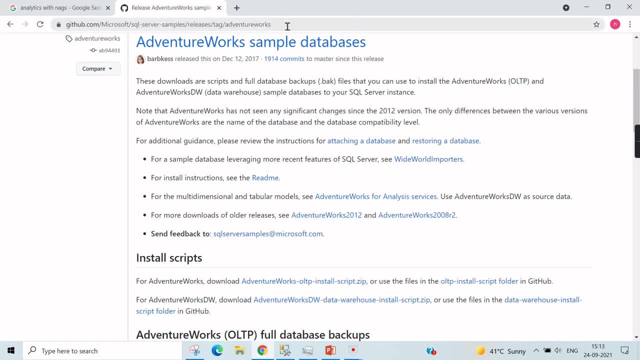 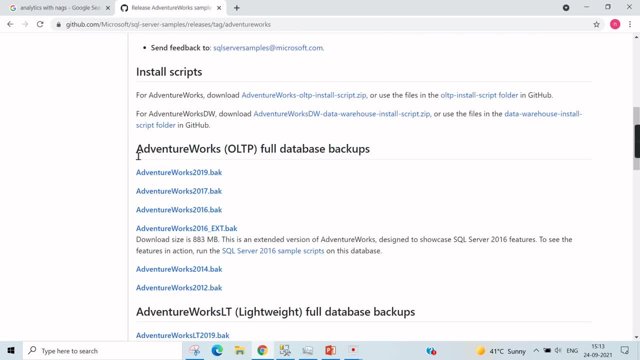 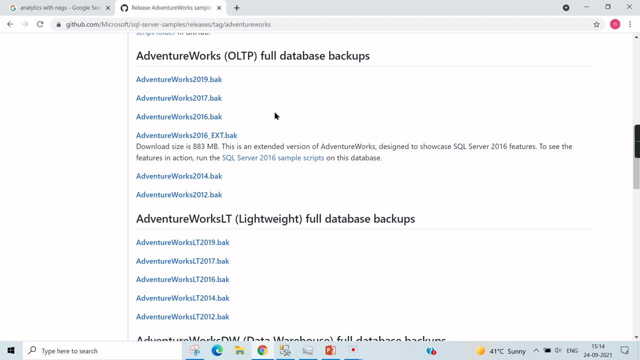 dot microsoftcom. i mean microsoft sql server. samples. release tag: adventureworks. this is the url. i will provide it in the description as well. just go here and do the adventureworks oltp system where they have given the backup. okay, oltp backup. then there is a data warehouse as well. this we are. 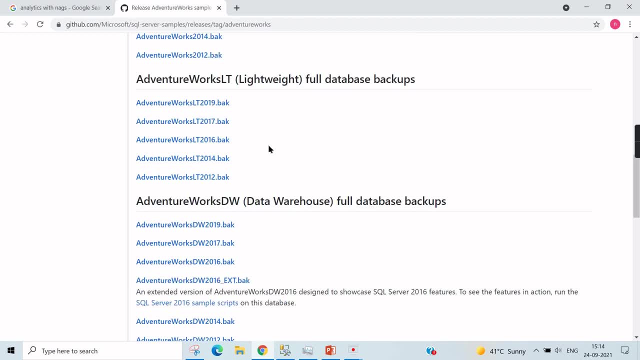 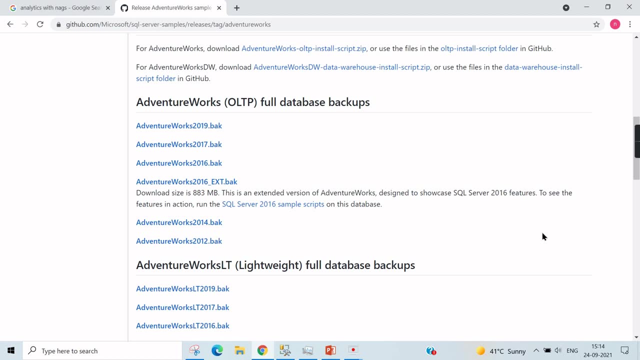 not going to use it because we need the source system. this is oltp system, and then from here we will build our data warehouse, right. so that is the ultimate aim of it. so for this demo only this is enough. but you want to explore how the data warehouse is built, and there is no relationship. 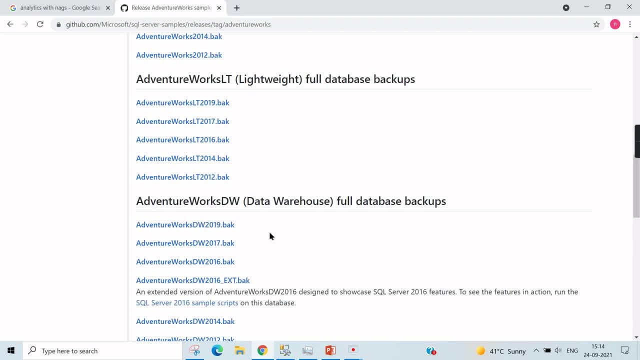 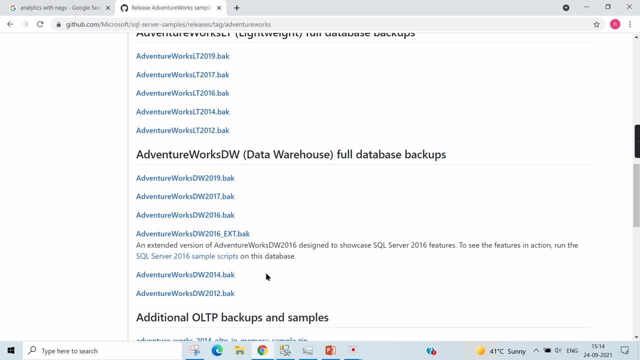 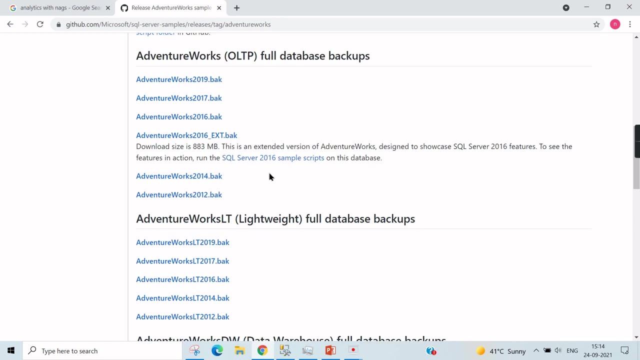 for your information: the data warehouse you cannot directly build from the oltp to here you because that is some conflict or there is no much data provided here. well, some of the things you can create it. so for this demo, only if you download it and keep this one adventure works 2014 backup. 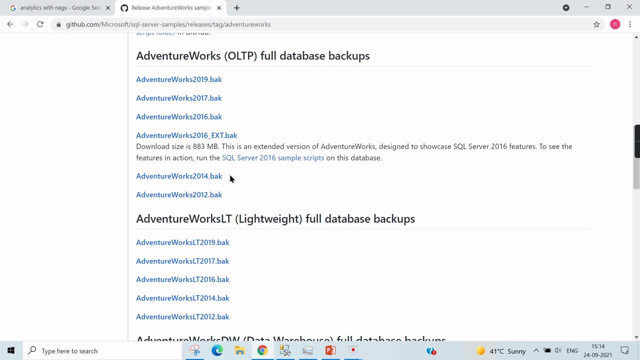 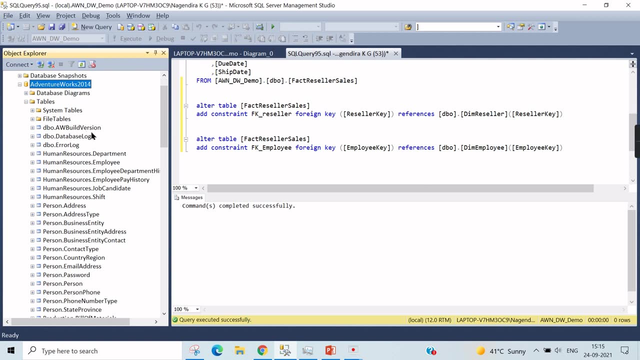 that is enough, because i'm using this version. that is why i'm recommending, if you have a latest version, you can go for any of those. that's fine. now we are in adventure works db. let's try to understand this. like we have a sales and purchasing production and person human resource. 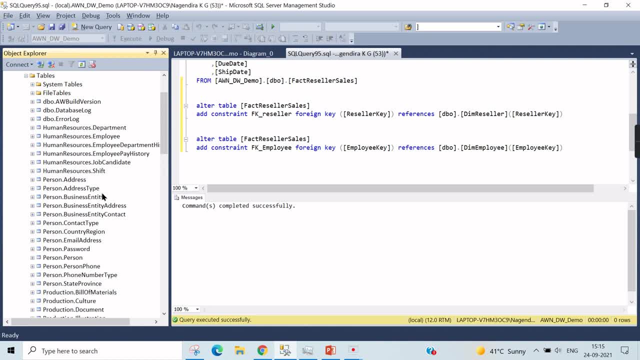 these are. the different departments are different way they have handled it. so where this transaction happens, right, so we can classify similar to this, data marks like sales and purchasing, production- we don't know what it meant by it- and human resource. so to have a very simple um. 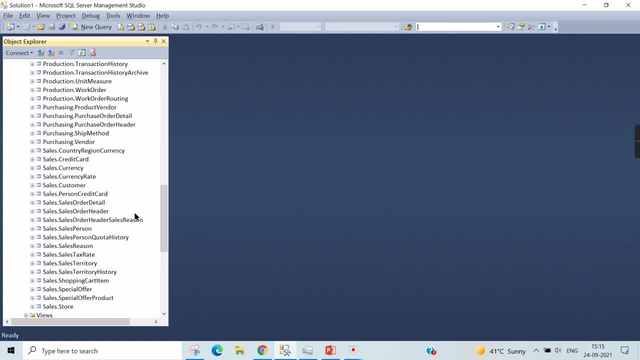 case, we can start with creating a sales data mark, then we will have a human resource data mark, two data marks then going forward as the business evolves, they can keep adding the data marks. that is the flow. it is not always. you design the entire data mass initially and then you can design. 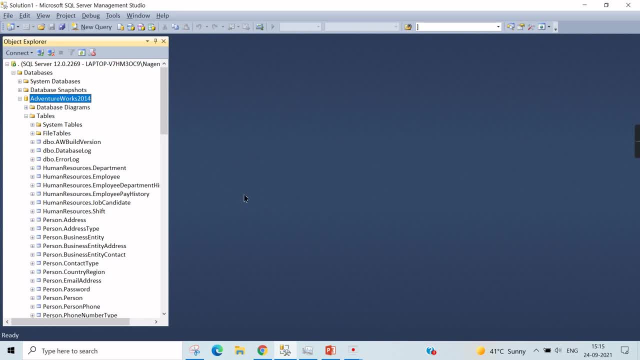 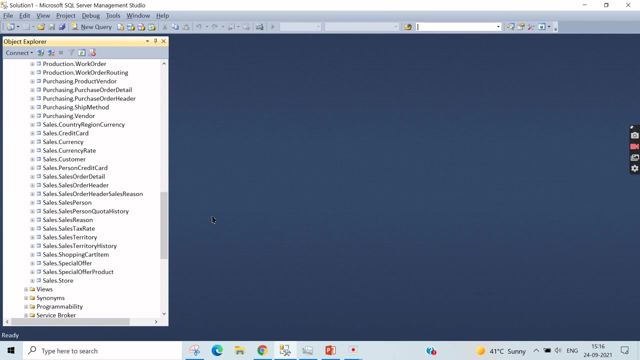 implement it at same time. the design can be. you can design different data marks, right to sales, human resource, other things. design can be done at the initial level. for the entire data arose, the implementation phase goes one by one, all right. so we are going to follow the same approach. we are going to design right the sales data mat first. 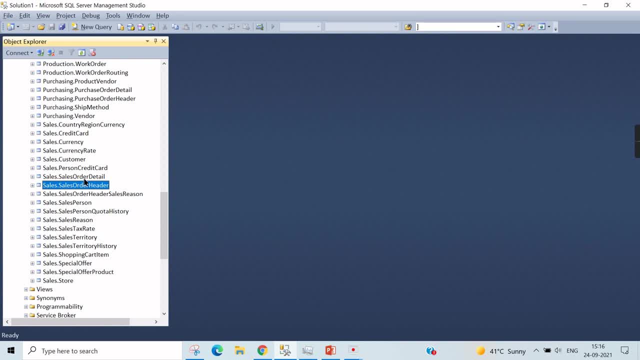 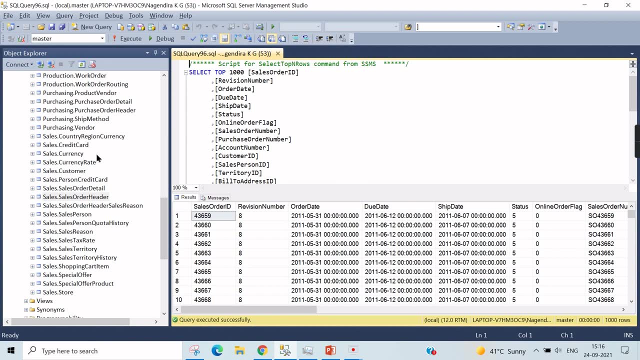 now for sales data mart. this sales order header detail are the key information. so i have pre analyzed that i'm not coming directly here and understanding this. i have pre-analyzed that for time saving purpose. i'm trying to explain what i understand. so this is a header, what it contains. 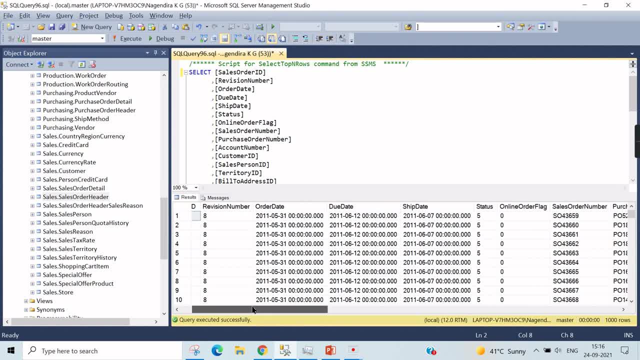 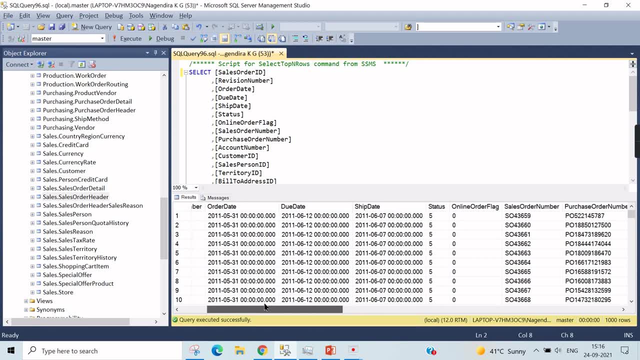 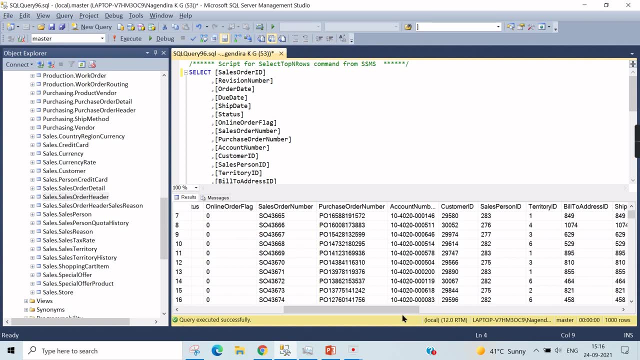 this contains the sales order, order date, due date. as you understand this business. this business is selling the uh the bike products. adventure works. bikes are uh, that cycles right. so this is order date, due date, ship date. and there is a sales order number, purchase order number. which customer has brought it? salesperson, id, territory, id bill to address credit card. i've got. 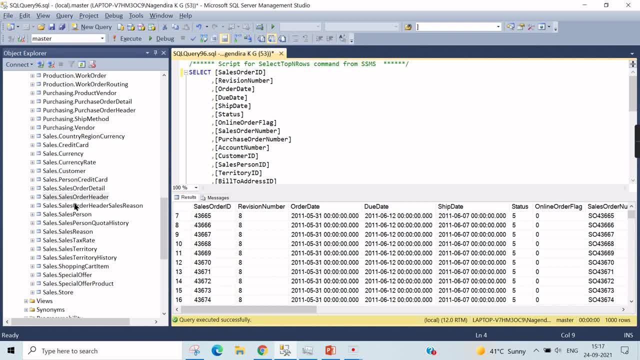 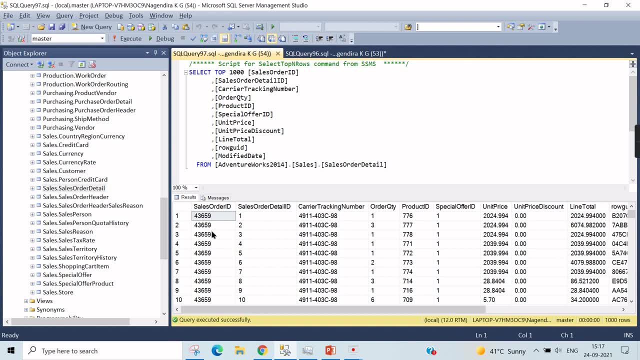 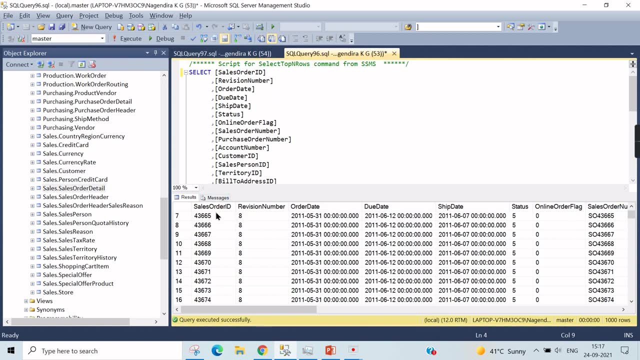 credit card are all those things. This is your transaction table. So what is there in the sales order detail? Let's go and check it out here. The sales order detail contains the actual line number, because you can see for this single order right: 43651. that is only one record here and when. this order has happened and this 659 has sold 10 products. 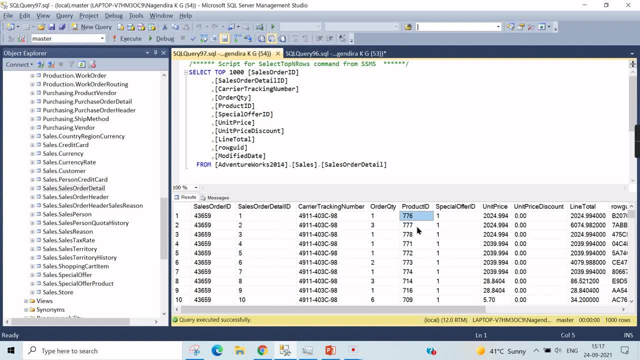 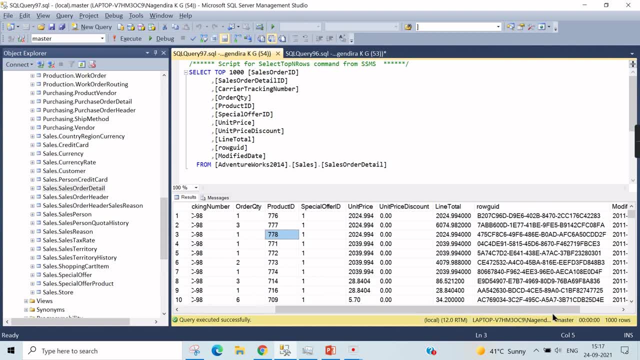 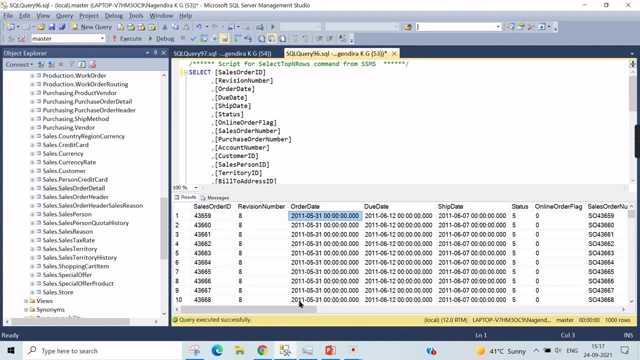 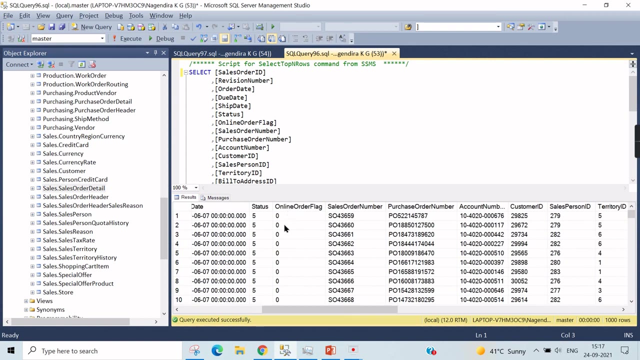 I mean this: 10 items, which is nothing but 776777778.. So these products has been sold. Then this is the unit price line item, all those things right. So this is like line item number wise and this is like a sales item number wise. So this is what you understand from here. This is how entity relationship model is designed. Another important factor here you can see in the order header is: like you have: 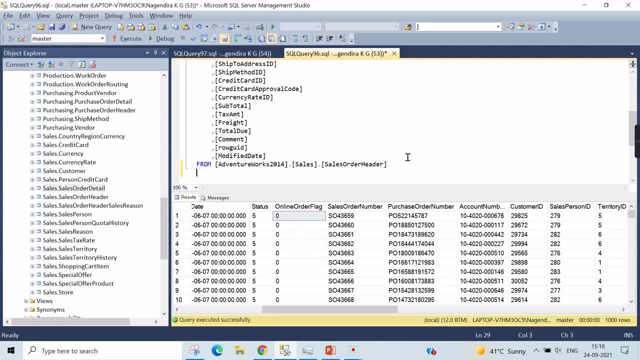 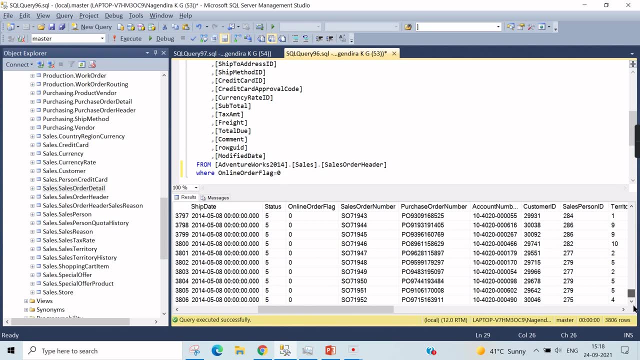 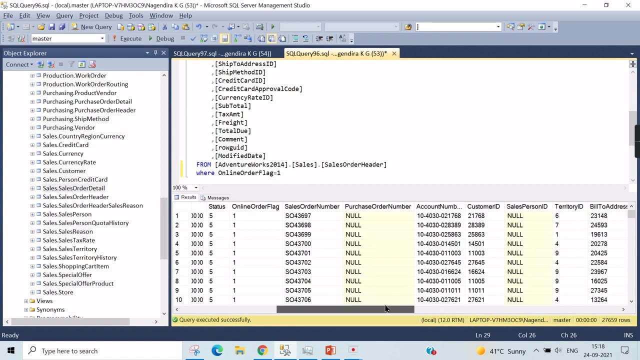 a Online order flag. What is that? So when we try to query it- online order flag- Okay, Online order flag- equal to 0. When I see 0, then you have 3800 headers. When I query it, equal to 1.. When I see 1, there is no purchase order number and salesperson meaning like. 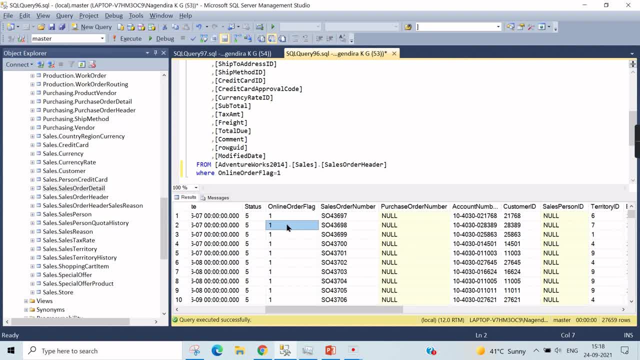 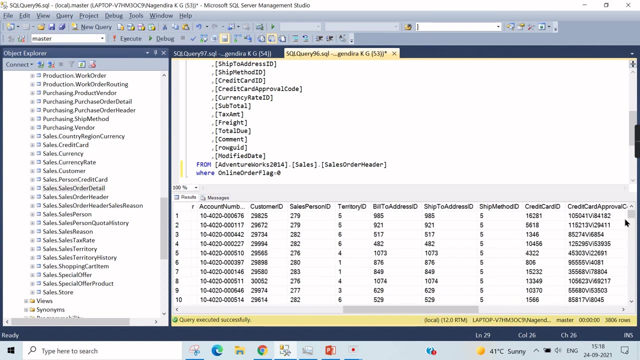 this online order, right, There is no salesperson involved. That is obviously correct, because the order is made on the website, So there is no person involved in it, right? And there is no purchase order as well. And when it is comes to 0 online order, flag 0.. Let us see. anything is missing here, Nothing. that is fine. So this is another important factor here. 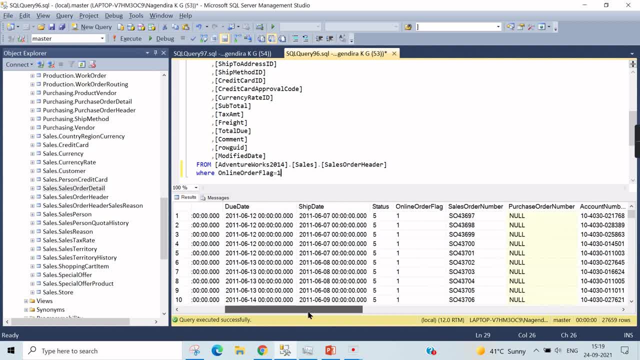 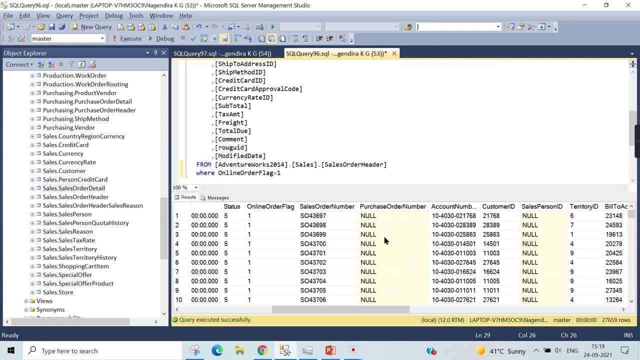 Another important factor I have identified. So they are keeping the online order as well as the offline order. Okay, The offline order is nothing but something that is happening at the store. Okay, That I will explain it shortly. There is no salesperson involved. This is one key, important factor we have found, Then: who is the customer and who is the salesperson? What I am trying to say here is like: in sales header, you have customer. This is another important factor. 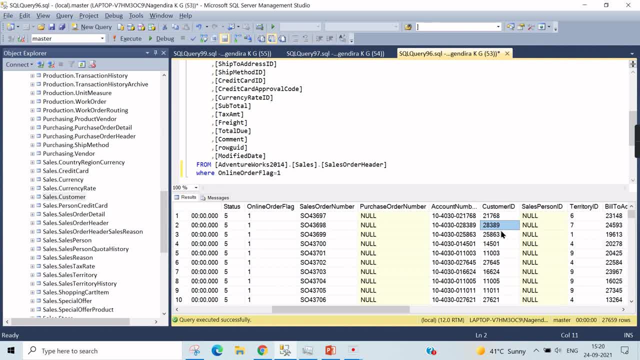 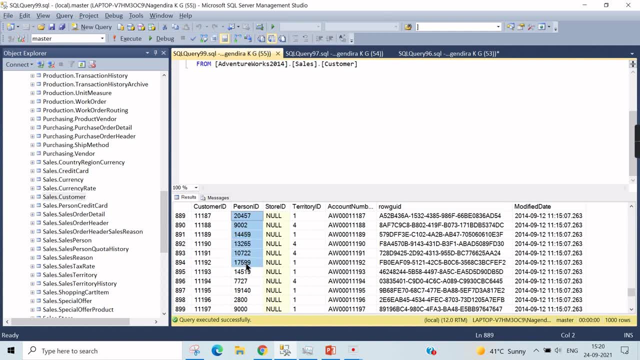 customer can be individual person or another store. so here you can see, the customer is whoever having a person ID right, he is considered as a person. I mean person ID is not null, is considered as a human or individual customer. then the customer ID of our person is null, he is considered as a store. so this is how. 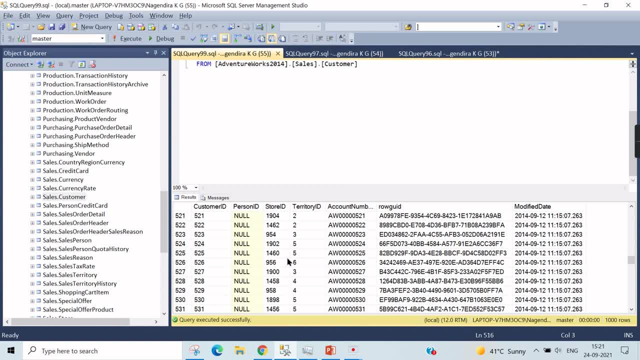 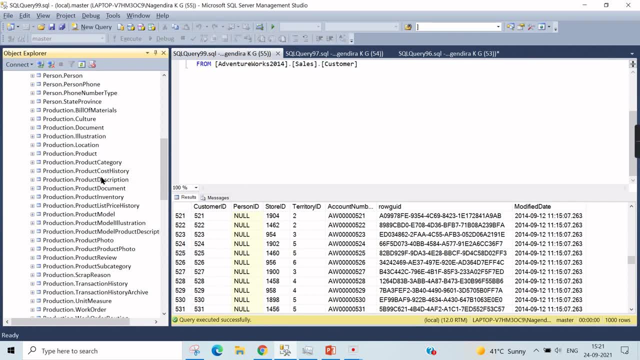 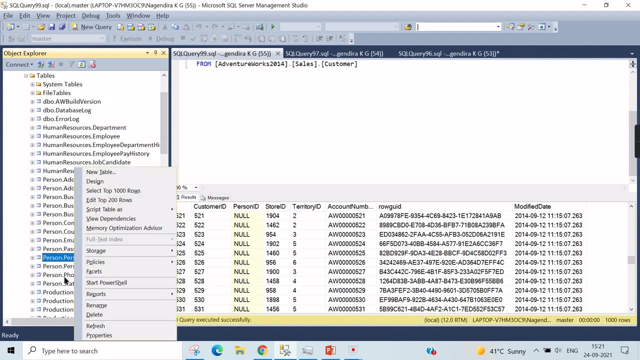 this system is architected. so this is what I want you to understand: how this system is architected. then again you can see. so everything is business entity, okay, and for that you have this. if it is a he fees a person, that information is stored. 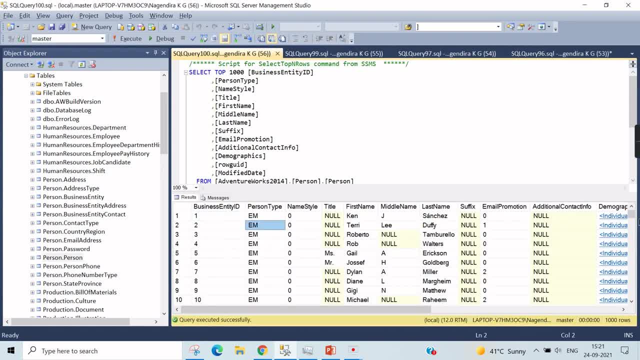 in the person, that person ID, whether he is employee or he is customer, sales customer, say, SP, means salesperson, so something like that. so the source system is very difficult to understand, so that how this will become your dimension modeling right. so how, from this entity relationship model, the how you can create the dimension model, that is the. 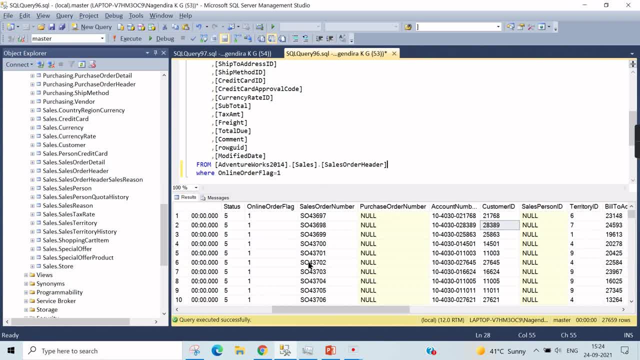 very big question now. okay, basically like this is what a complexity I want to explain. so, customer cannot be directly a customer. it's available in the customer table. he is can be a customer, he can be a store. so these informations only a source system can provide. and where is his? 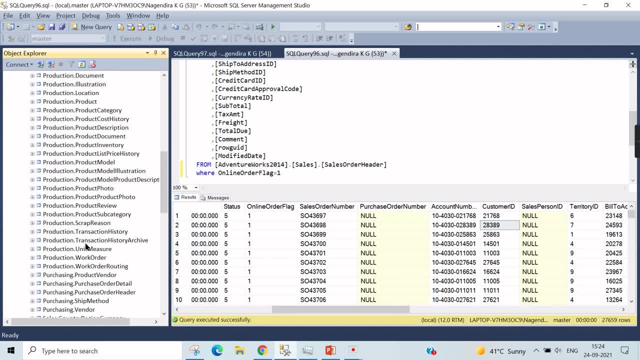 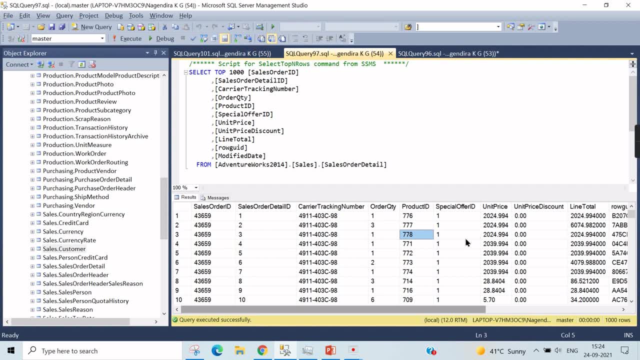 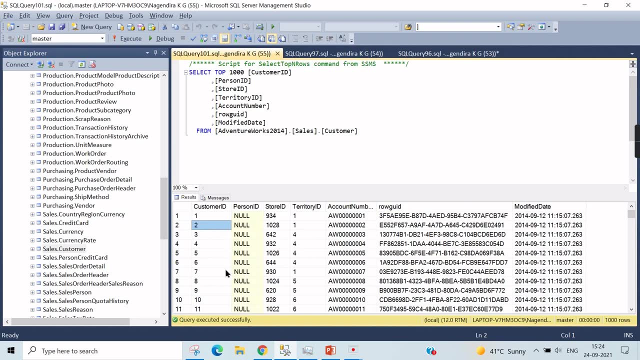 other information. he is the entity. so if we want to know what is the name of the customer, right, he is only having customer ID. we assume like customer in the header table. in customer table you should have a name address, but there is no address, our name here. in turn, again, it is referred to another table like person. 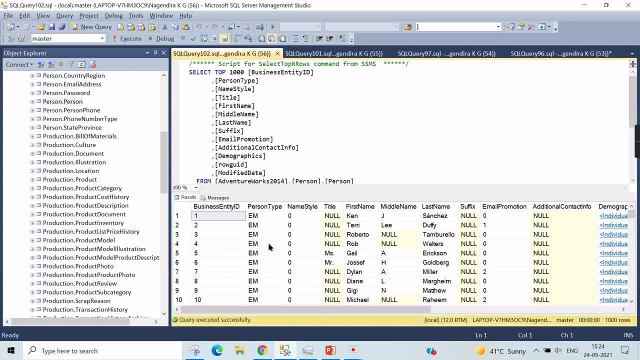 person dot, person ID. so here you will get his name, last name and what is his other informations, right? and even you have a person dot phone number, person dot address, email address, country. so everything as a separate table. so this is how you need to correlate the things. 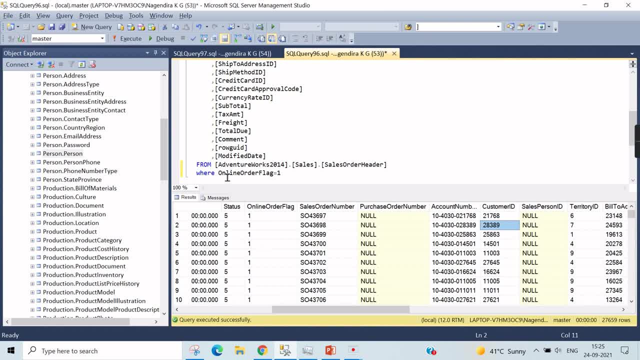 you need to understand the source system. after understanding the systems, then you will come and design your dimension and facts. and one point to highlight here is like: this is: online order is something the customer is purchased, and if it is offline order, it is called reseller. okay, so the thought. 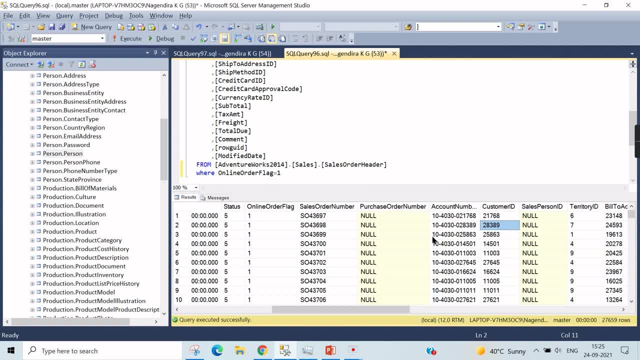 is like you can have your online order in your online store. then further, the relationship between the four subjects will be higher than in the other customer websites. it in the other образом now, when a two separate fact for the, because if you have customer and reseller in the same place, 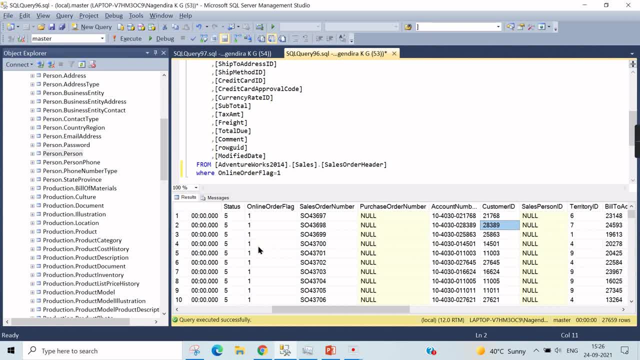 you will not have a salesperson, right see? because in online there is no salesperson, but in offline you have a salesperson. so you cannot have such a design in your data warehouse, keeping one field empty for some records and keeping empty for another records. so you can divide this particular. 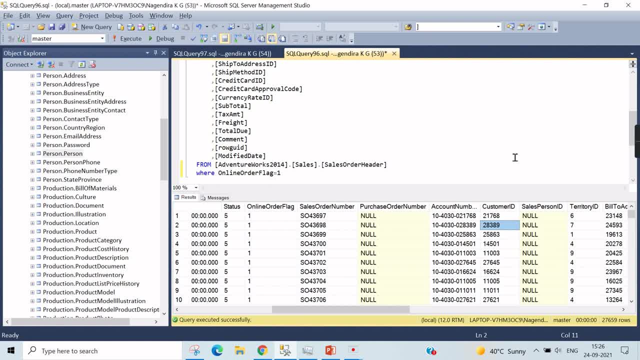 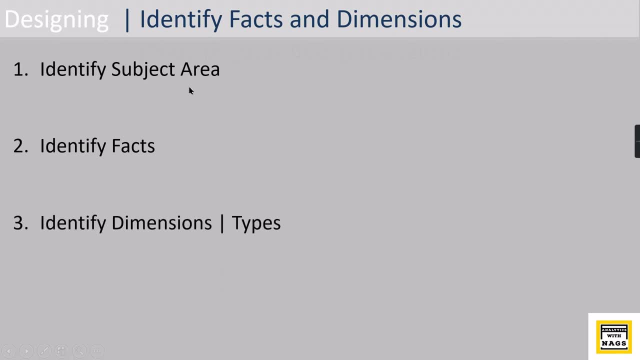 table into two tables as a fact. table one is internet sales and another one for reseller sales. let's try to walk through in the presentation once again, so as we have seen how to identify subject area and five facts, and let us discuss this again now. so for this demo, let's keep it. 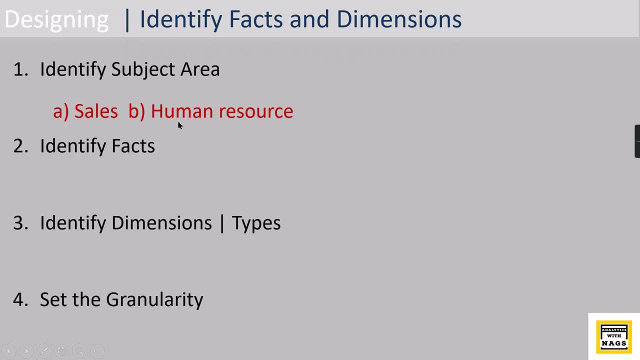 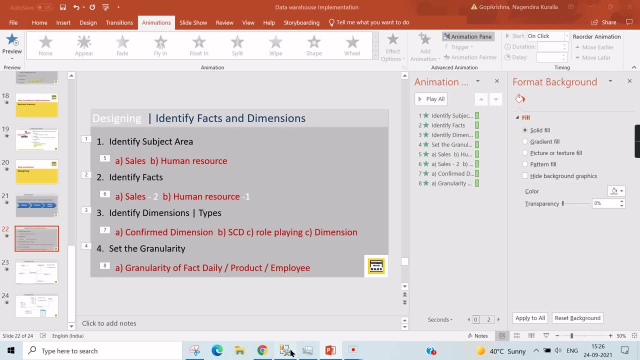 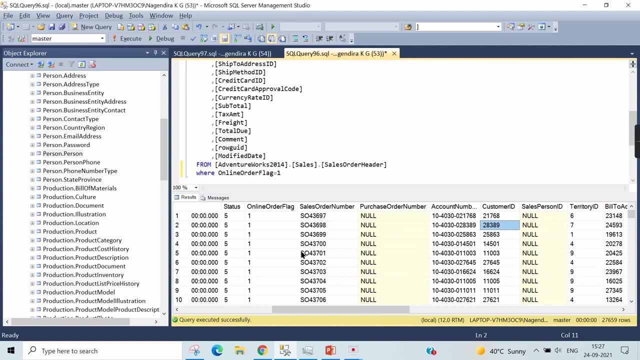 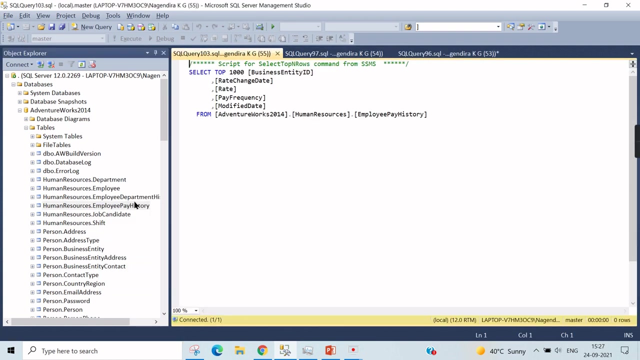 simple. we can have a sales and human resource. we didn't say anything in the human resource table, i will so. so in the sales table i mean sales subject area- we will have two fact tables. one is internet sales and reseller sales, and another subject area. what we are going to do is, like human resource, where we have a 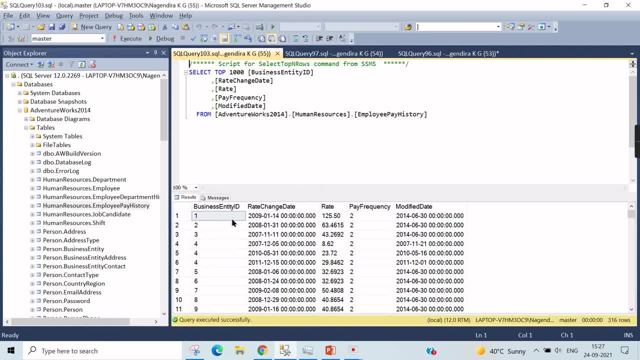 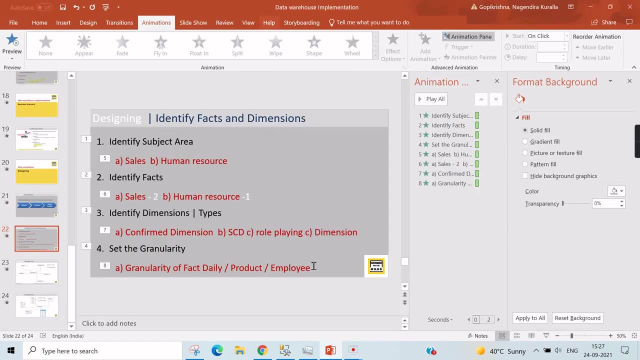 pay history right. so for this subject area we will try to create one fact table, simple fact table, after once we create the sales subject area, the proper implementation. once the time permits, we can also check, like this particular human resource subject area. so let's move back to our presentation. 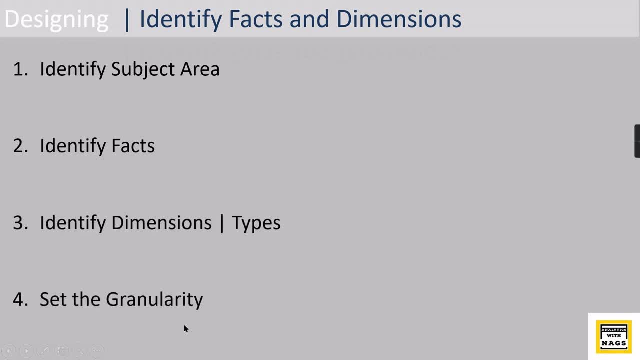 so these are the things we need to identify, as we have seen. so identify subject area. for this demo. we are going to decide on sales and human resource, two subject area we are going to start with then. in sales, you have two fact tables: one is internet sales, another reseller sales. 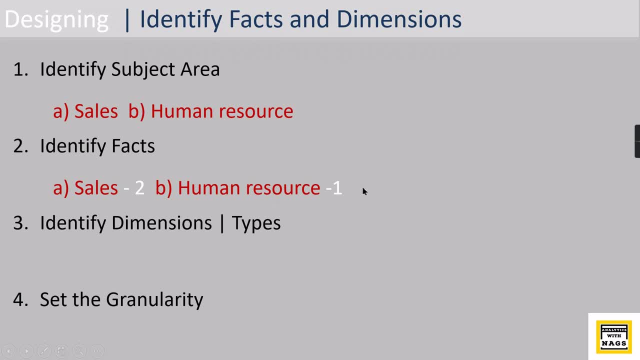 and in human resource. we will create another fact table then. dimension is related to confirm dimensions and scd role playing dimension. so how this can be classified is like a confirmed dimension is something it is came across all the subject area. so date is your confirmed dimension? it will be used in sales, a human resource, any other? 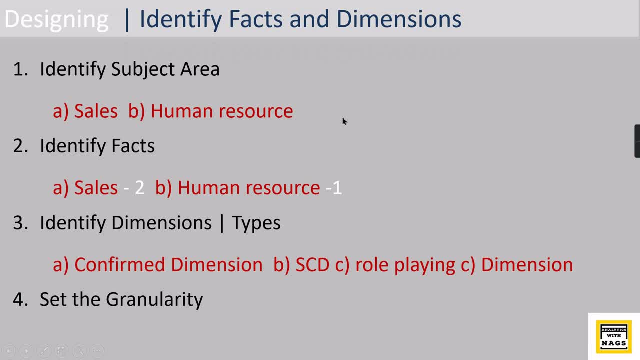 subject area you decide date will be there, and something like um, your um location. okay, that region can be available in all the subject area also, so that becomes your confirmed dimension, okay, so these are some of the things i am saying, and scd like um, slowly changing dimension. 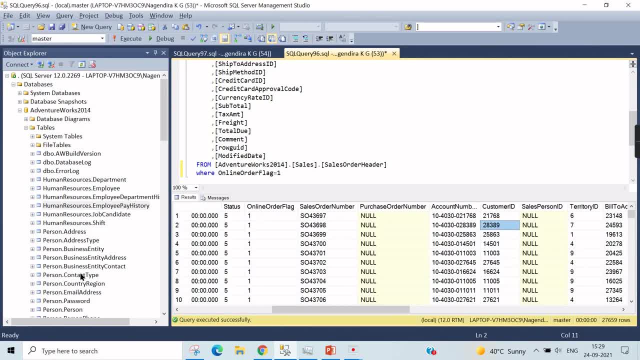 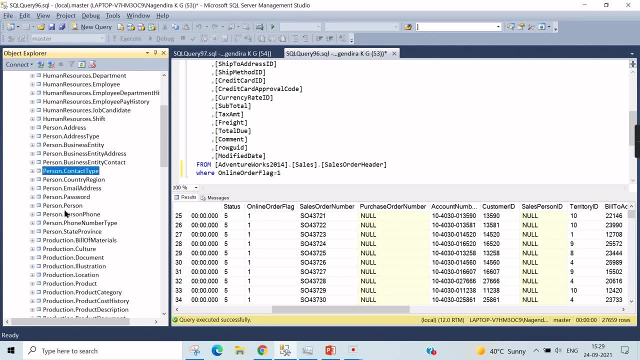 um, i have see, i have shown you like, um, this particular employee, right, he is a salesperson and he can change the department. so we need to track the history. so those are the things that becomes your scd. so if you do not want to track a history, 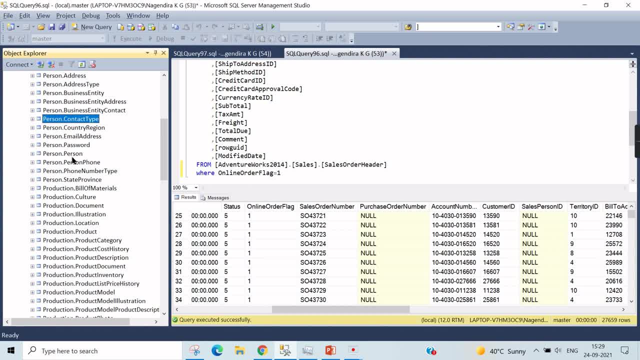 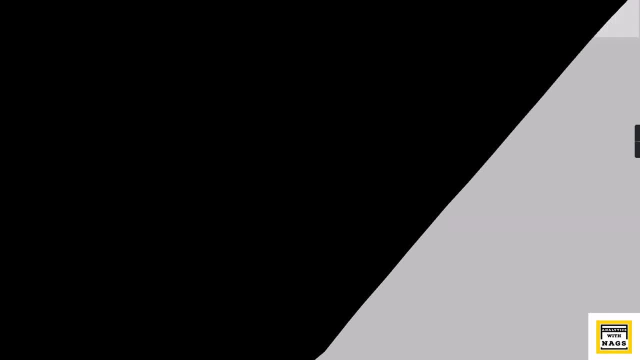 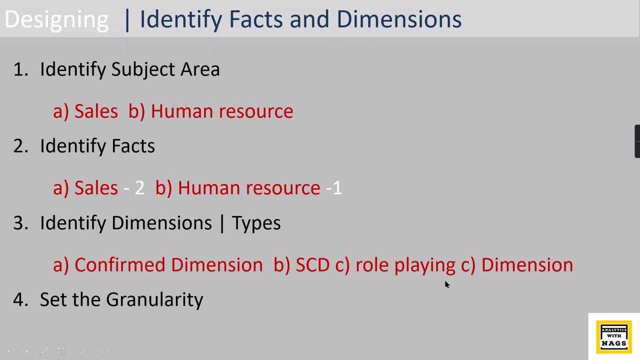 even this particular person changes. then you can go for scd1. uh, we, we can discuss while implementing more about scd concepts. okay, that i will come to that later. so employee can be a seri. then role playing: date dimension is role playing and other dimension that is related only to that. 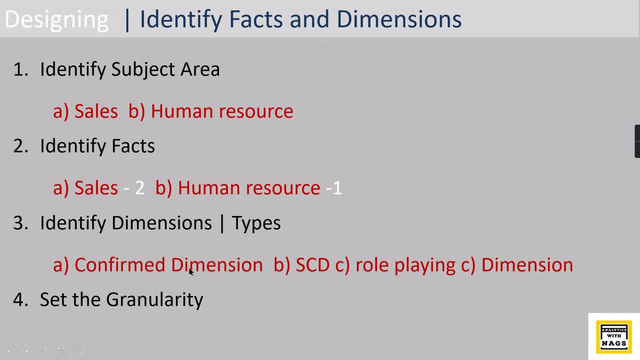 fact table. so these are the different types we will decide on. for each fact and dimensions, I mean each fact, we are identified. so set the granularity and this sales, it's now, it's again, already, it's daily. we can creep it and we can do it by product and then for the reseller it will be employee. so these are the. 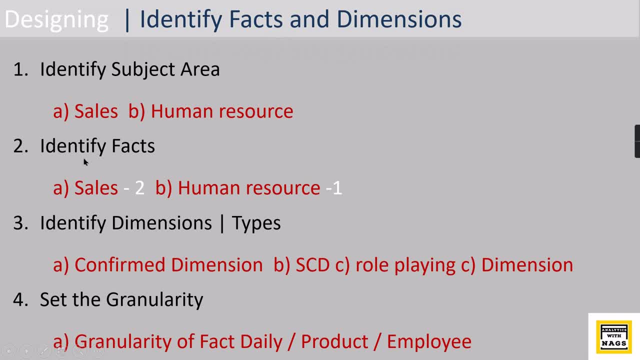 some of the things you need to decide on right. you need to identify subject area, identify number of facts and then dimension how you can do it? just by analyzing the source or keeping iteration. so this video, just a single video, is not enough, just giving you an idea how people will design the facts. 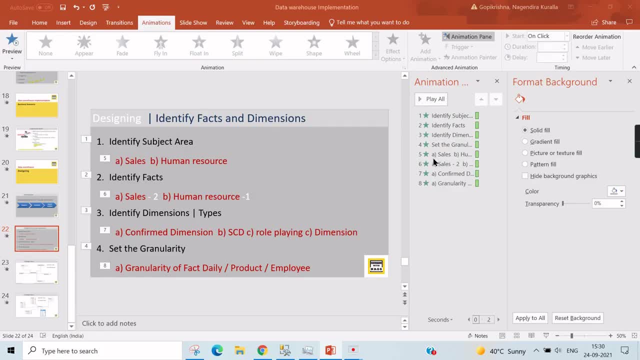 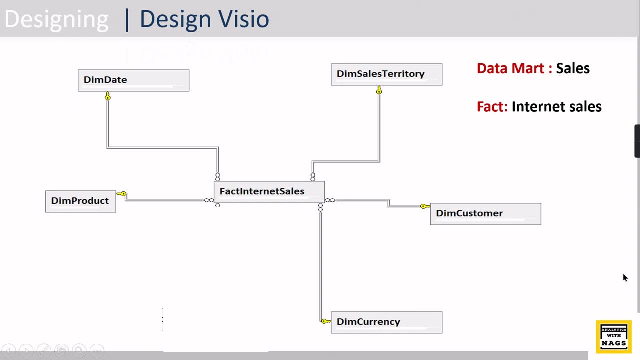 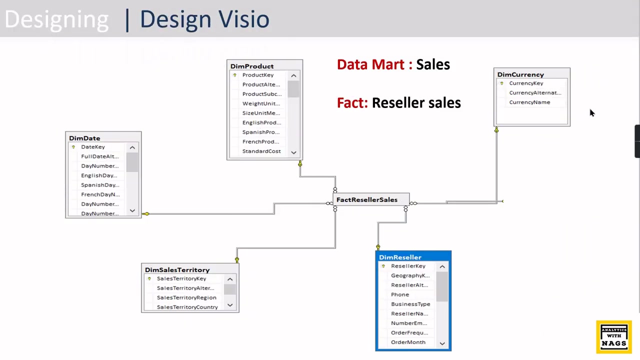 and dimension based on different things, right? so by deciding all these things now we have came to this design right in the initial. you need to set what are the your fact table fact and these are your dimension tables, and this comes under the sales data mat sales, internet sales. then you 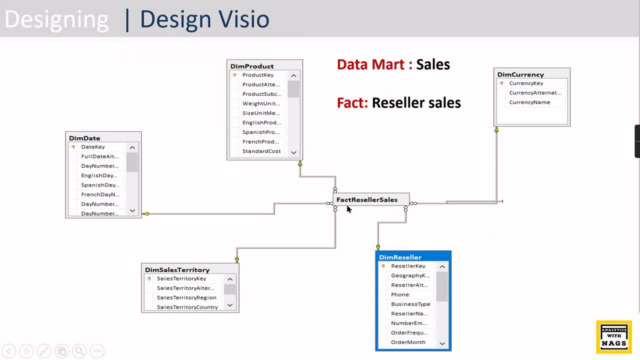 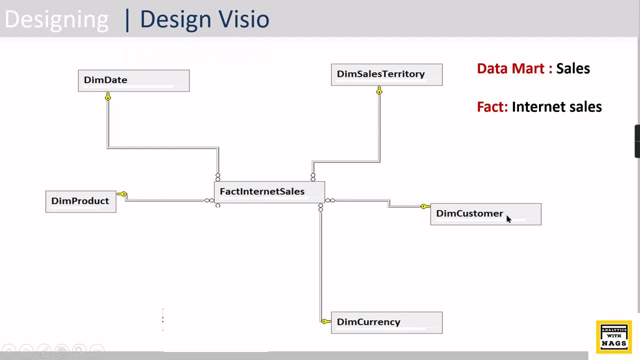 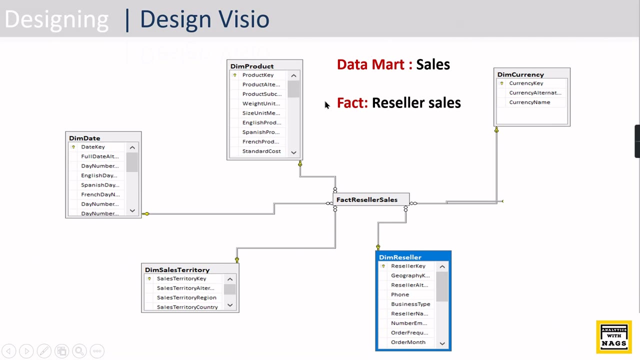 have similar thing like fact reseller sales and, as I said before, the customer here becomes the reseller. okay, so only between these two. data mat is like in terms of customer customer is not there, instead he becomes the reseller because it is the stores. okay, so we have created. 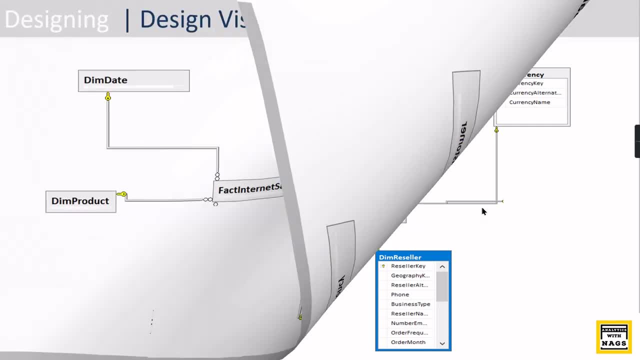 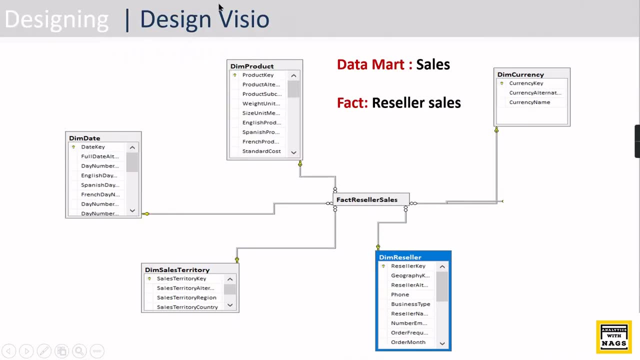 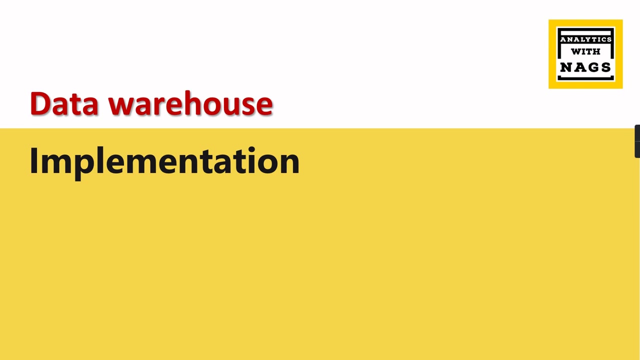 the another fact table. so two fact tables right, one for internet sales, another for reseller sales. then we will have design here, right? let us start the actual implementation of data varus. the actual implementation requires some steps. that is sequence of steps to be followed. let us talk about that and then we will jump into real implementation in 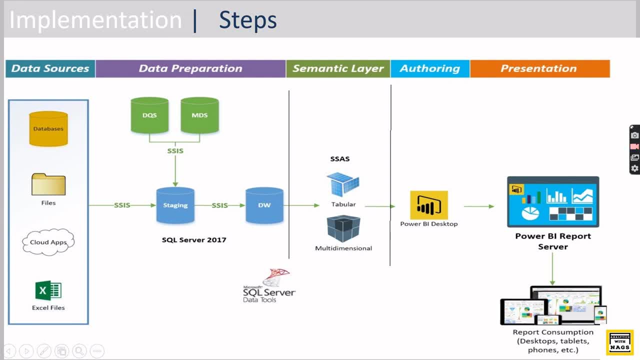 a demo. so this is a typical architecture and we cannot create a data varus in single. some slips- I mean single click, or it is not a quick way to do it. there are certain steps to be followed in a sequence. that is the proper flow. that is what I'm going to explain it with this diagram and once we 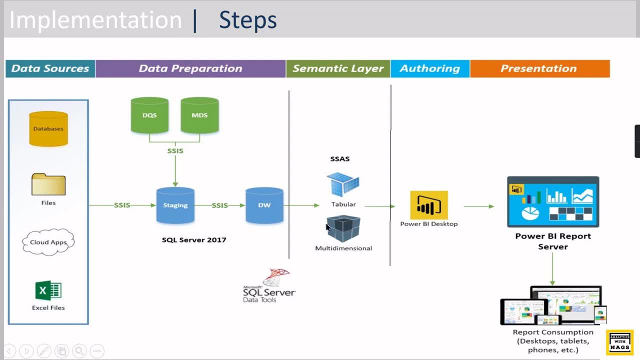 complete each step will come here and color it out. where this step is completed, you will be aligned with that. so what are the steps? so first thing is like creating database objects, so you need to create this staging database and data varus database. so, staging database, what things you are going to have you? 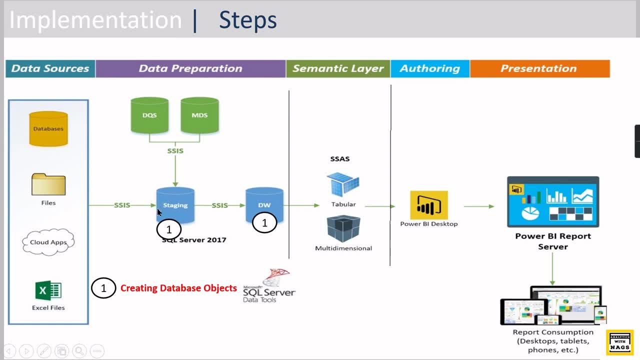 will have a same schema here. whatever in the source table, you will have it here and then you will blend it to have aligned with the data varus, right? so this is one database and this is another database and, deciding on where this databases should be, it should be in the same. 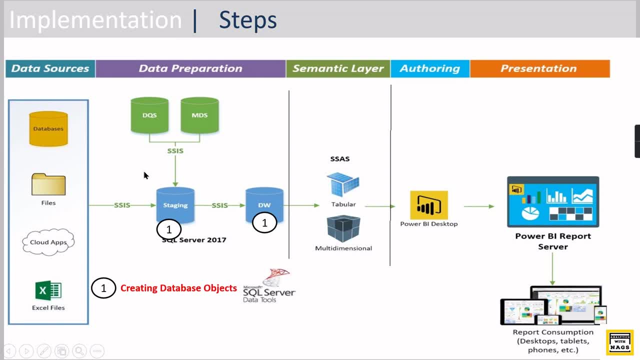 server or different server. so this is something like designing or architecting concept, but I want to explain it here now from my opinion. in my experience, if the staging and data varus is in the same server, right, you have a single server and staging is one database. 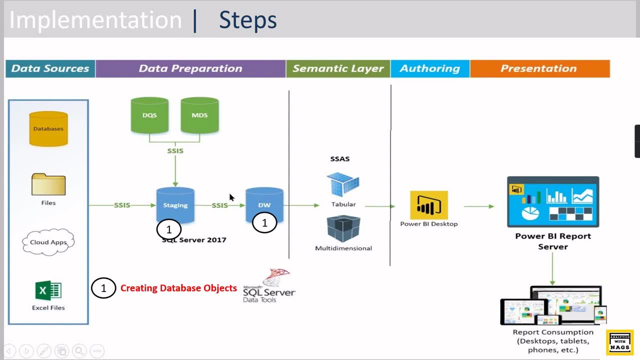 and data varus another database- then it will be very easy to implement because most of the time you will refer some of the objects from the staging and in order to do the incremental load, to check whether that data exists or not already and delete and improve incremental load the data you need the both database to be. 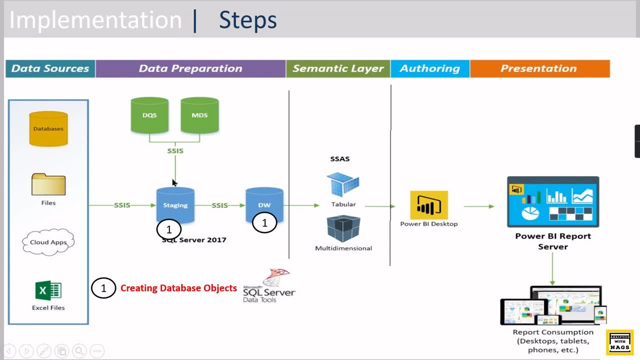 in the same server. that is my recommended thing and in case, if you are considering this as ODS, like you are not deleting anything in the staging ODS I already explained, so in that case it is fine. it depends upon your capability of your servers in that. 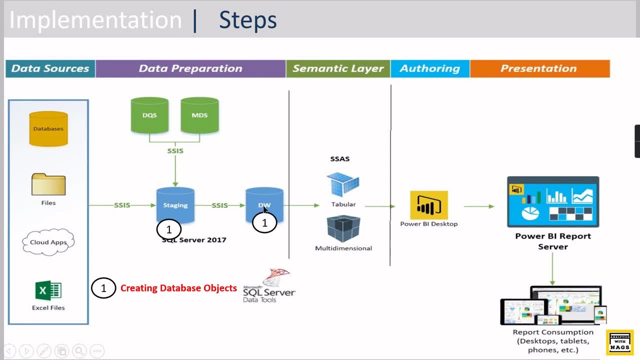 case you can have staging in one server, data varus in another server. if you keep both different servers, you will encounter some issues. you cannot write procedures to call. you need to always have SSIS to do it. I will explain while implementing. for simplicity, you need to create two database in the same server for this demo. 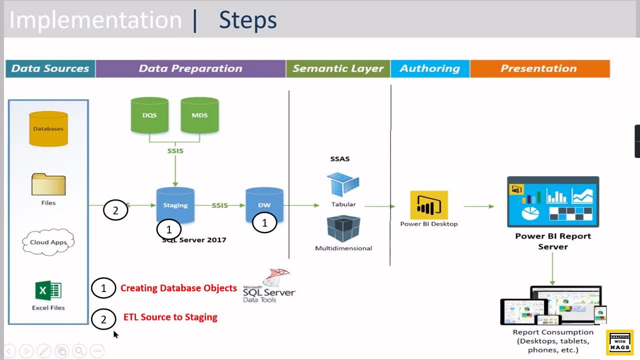 then next step is like: you need to load the data from the source into your staging. that is your second step that we will walk you through. then the third step is to ETL staging to data varus. once you are loaded it, you need to convert something, you need to merge some. 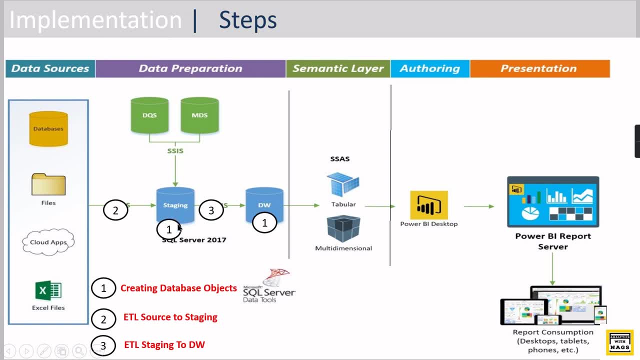 of the tables, those things, you will do it. then, finally, you will load it into a data varus. so there are three step process involved in building a data varus. so once we build it, we are not going to stop it with, as we are going to demonstrate the entire BI flow. after that we will create one. 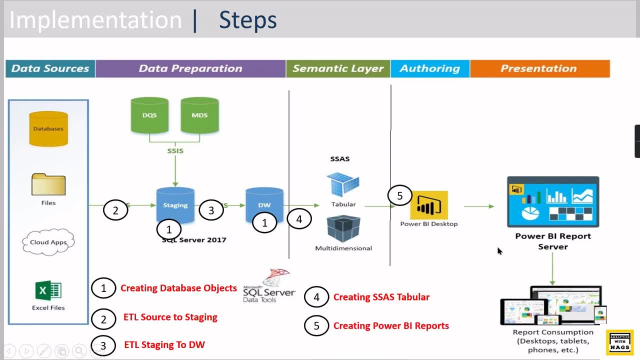 tabular cube, then followed by creating the power BI step reports. so while completing each step will come and color it out in green so that we will know where we are. now we will see the demos, which is the first step. then we will proceed further. this is: 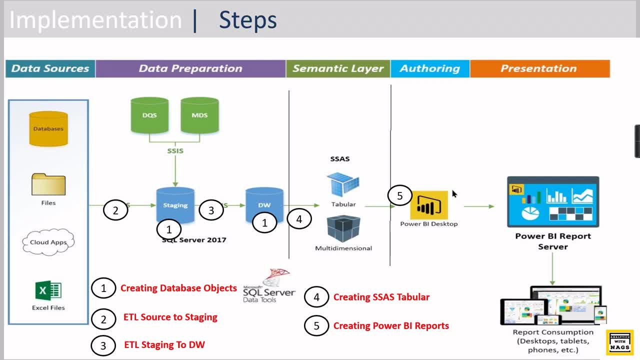 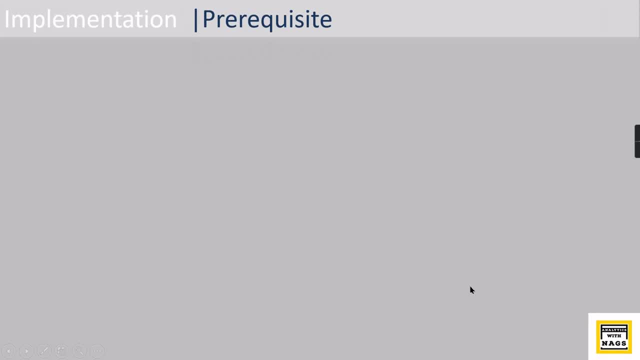 the plan. with this note, let us directly jump into demo. okay, now, if you are ready to develop along with me, what are the prerequisites you want to know, right? yes, that is first thing is like you need to have a skill server engine and you need to have a skills of a management studio that is for to work with KORIS. then, as I said, 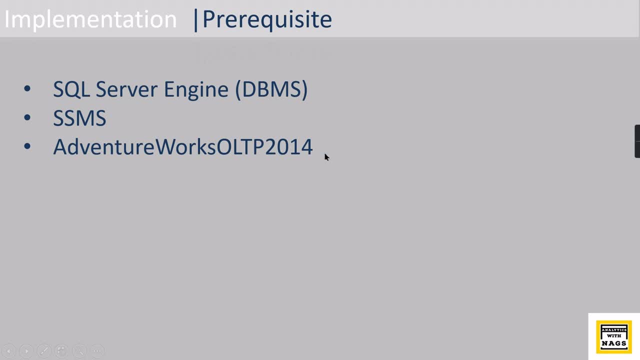 before, adventure works database that you can download from github and then you can restore it and keep it ready. then visual studio data tools. that includes SSIS, SSIS. then, additionally, if you want to explore all the works that we have done in powerful reporting tool, power bi is required. that I will anyway. I will demonstrate it is. 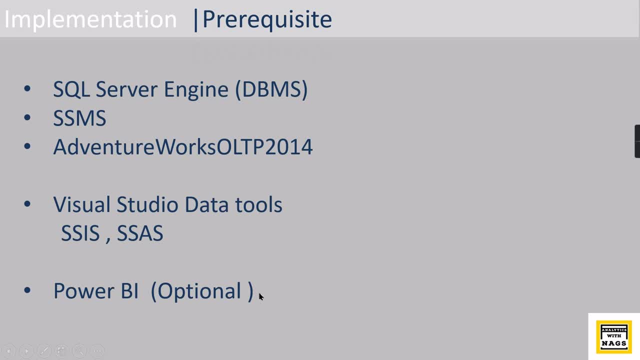 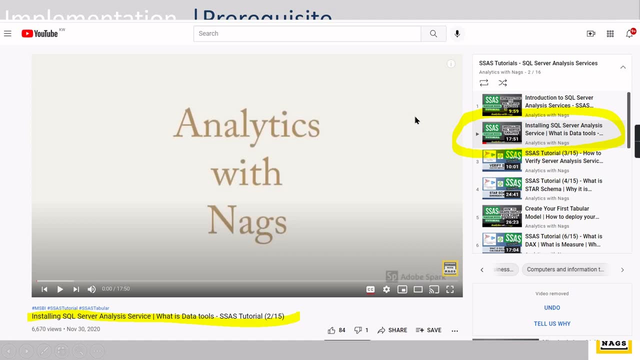 optional. up to you. you want to practice it or not. so these are the prerequisite and how you can install if you do not have anything about it- I mean, you do not know how to do it like over here. I have mentioned installing a skills of analyze service. that is in SSAS playlist. this is the video installing a skill. 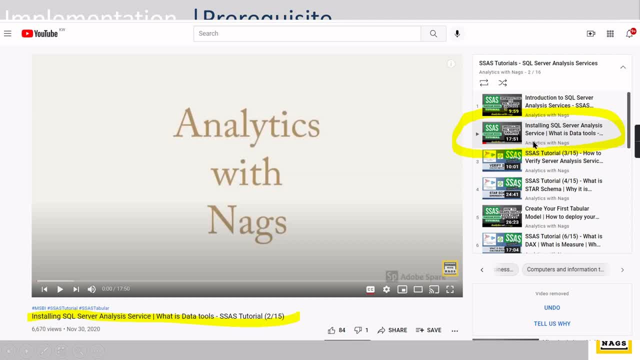 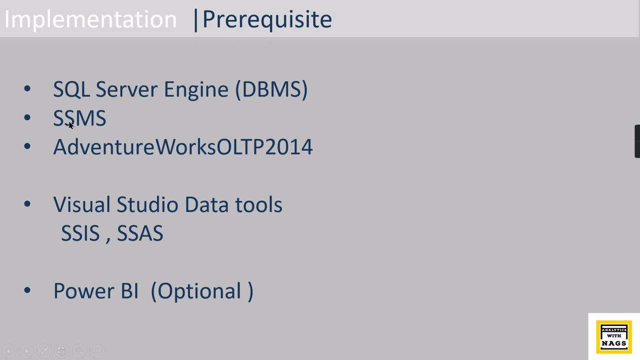 server data tools. right, it is basically- it's mentioned- only a skills of analyst service. basically it involves install a skill server database engine, SSMS, then visual studio. these three things you will able to do it in that. then adventure works. as I said before, you can use that github link. so 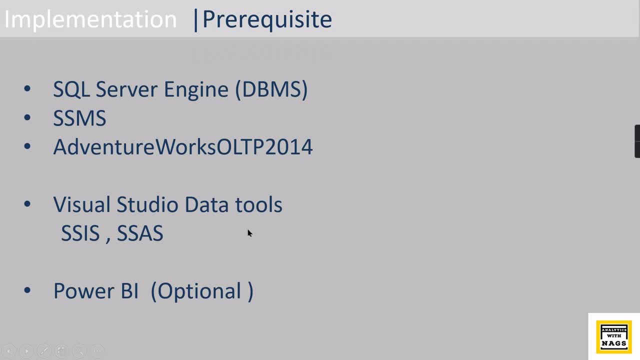 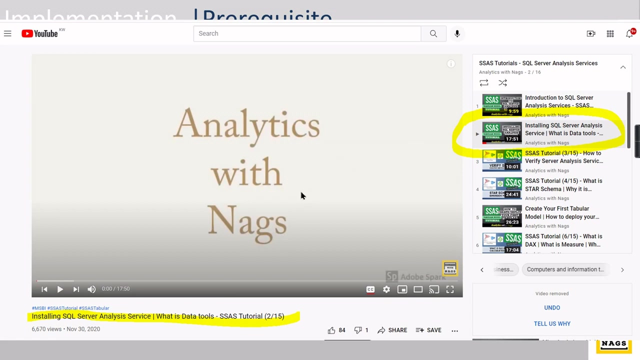 once you are done with it, before proceeding further, ensure all these things are done, then you can start implementing it. I will also provide a link to this video, as well as the link to this video. as well as the link to this video. I will also provide a link to this video, as well as the adventure works: DB. 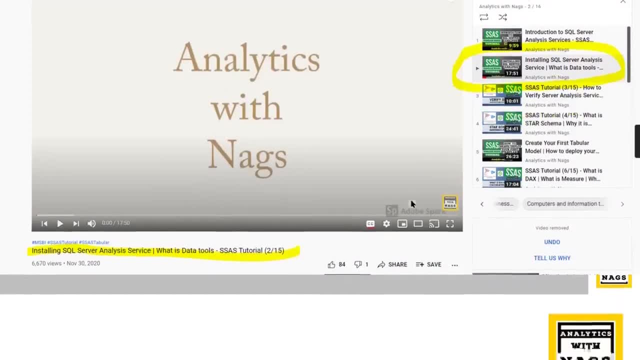 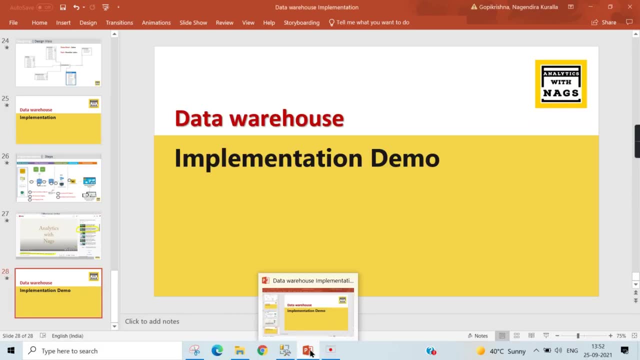 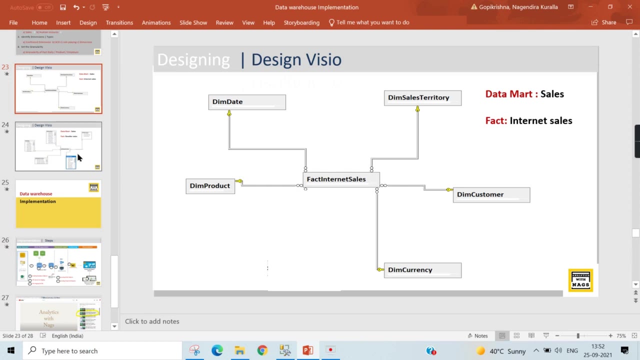 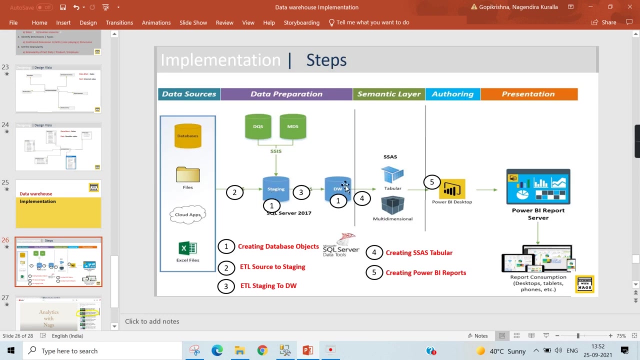 download in the description. let's start with the actual demo. so what we are going to do, like, as we said, in order to create this schemas here, right, the ultimate aim of datavirus is to build these two schemas, so for that you need to create a staging layer and data wearers layer. the staging layer is going. 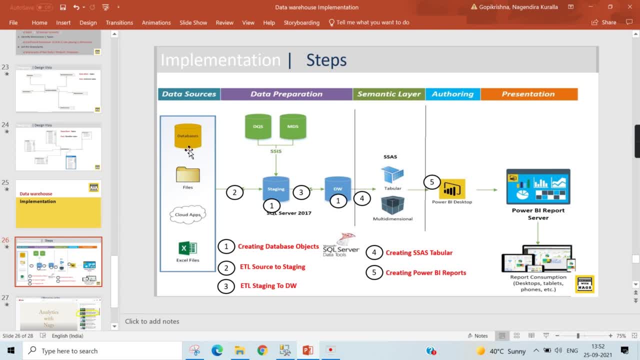 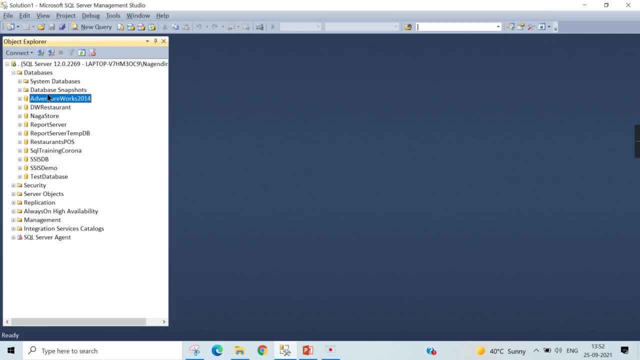 is going to have the exact copies of your tables from the source over here. okay, that is what we are going to do for the first step. so for that you need to have a source. correct this adventure work source. so those who are already working in database technologies, you might have a once you. 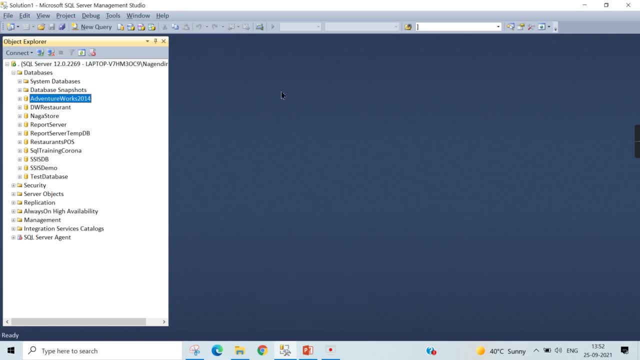 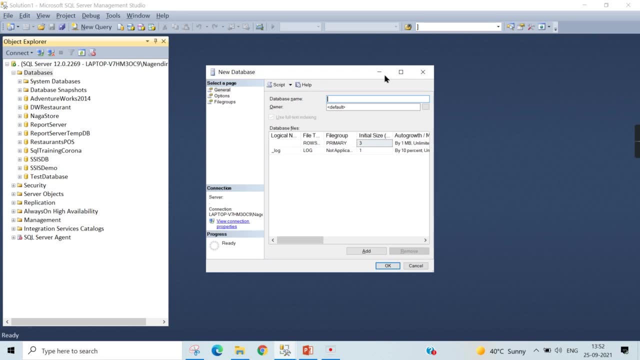 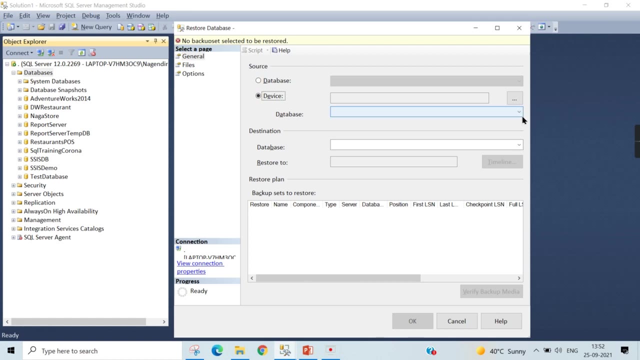 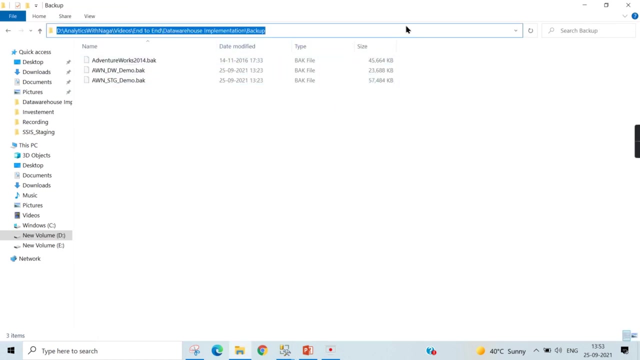 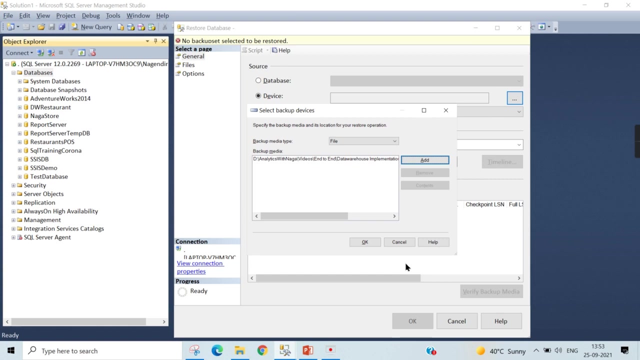 download that adventure works db from the link i have provided. then you can right click here, go to new database, not new database- right click and restore database, then navigate to device and you can choose that particular file over here. i have stored in this backup folder. so just paste to that folder, then click on this backup file that you have downloaded. 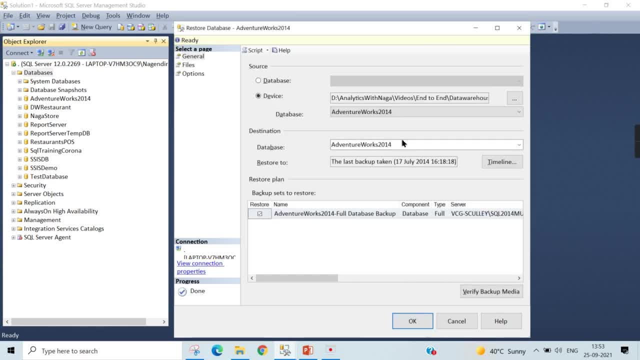 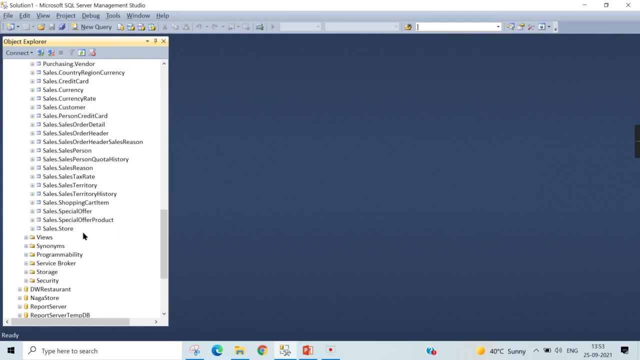 then click on ok so this will appear here. the name you can change if you want. But if you are following this, just ensure you are having the same name, because the SSIS package will point to this database. So once you have this, then click on OK. I am not pressing it because I already have this imported. So just press OK and ensure this is the source system. 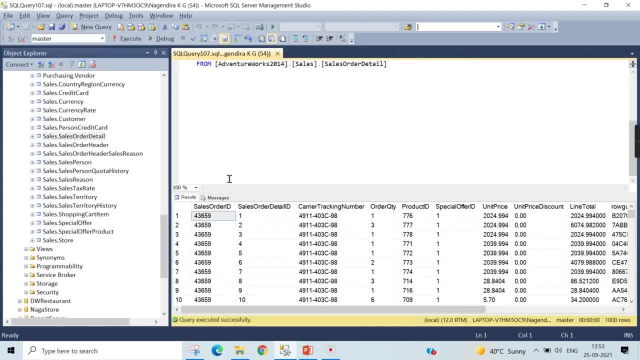 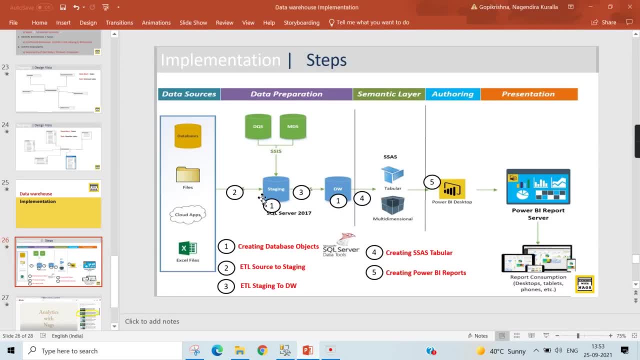 This is the OLTP system. Now you can query it over here, just check whether the data is present or not. It is fine. Now next step is to create this: staging tables for those whatever identified. You cannot bring all the database objects over here. What you want, you, but the initial development, how it follows, is like whatever required for a sales data mart, you will bring. So what is required you need to bring. 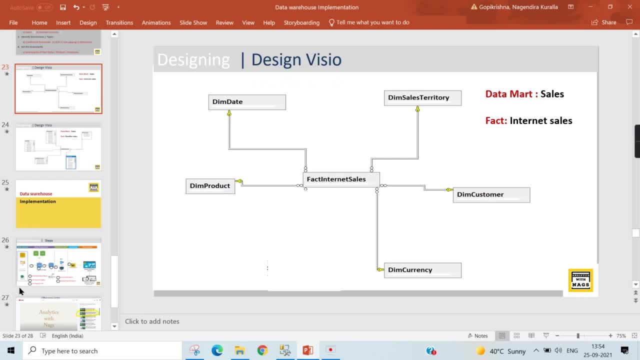 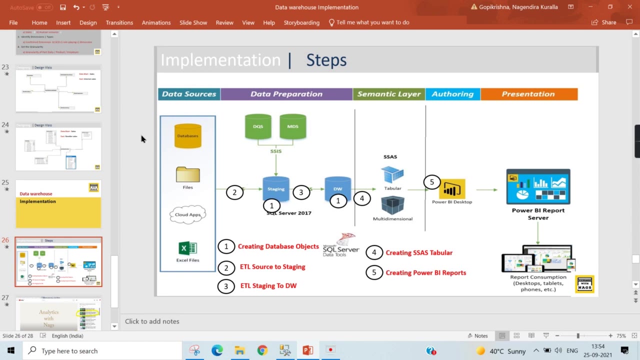 It says territory, customer, everything right, So only these objects. So these objects and its related tables, because in the data arrows we have designed customer But, as we seen in the one of the source analysis, the customer is present in different tables. So you need to bring all the related tables here, identifying what are the tables required. then bring all those things. So for that I have created the scripts. the AWN stage demo. 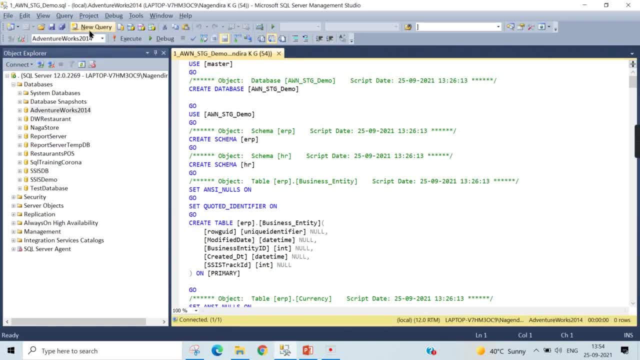 And we will try to create it here. Now you can see, this is the script that will create the required tables for our sales, internet sales and as well as the reseller sales data, marts. OK, That you are creating in the staging layer. So here is the script. you are creating the database. So I will create one by one to make you to understand. 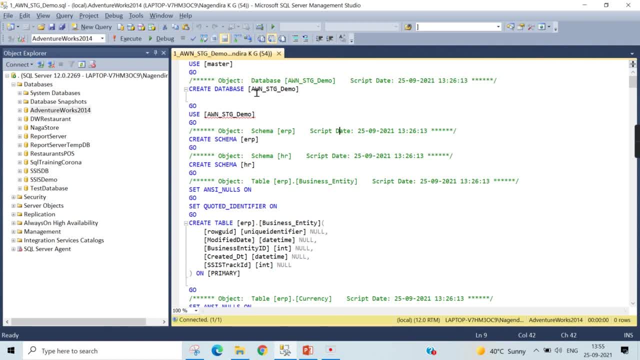 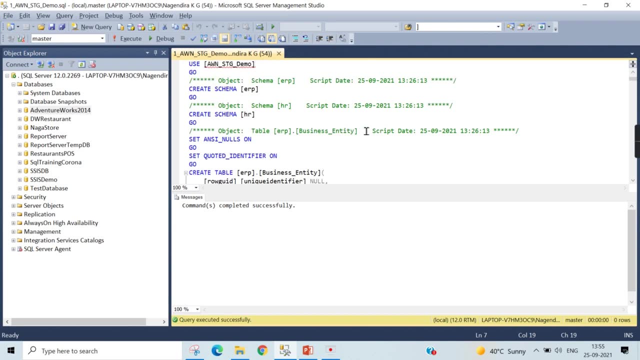 So that it will be easy for everyone. So first step is to create your staging database and for that run together in your case, just execute the script. I will anyway share the script to you. just execute it in a single step, So all the objects will be created. So here, once you go and refresh here, you can see a staging database created. There is no tables or views, anything over here, It's just a database. 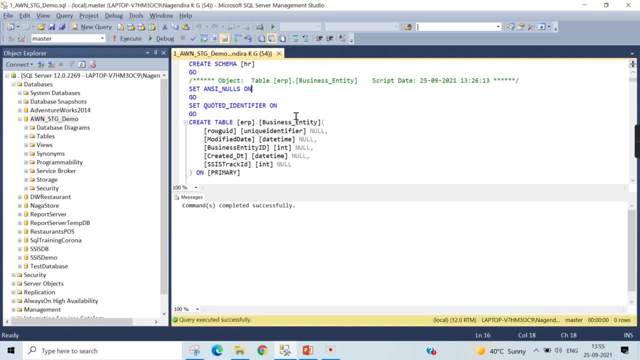 Next step is to create or bring those tables. So from here the table. what are the tables we identified is like: business entity, currency, customer person, person address, product. OK, Product category, product tables, sales header right and sales order detail. 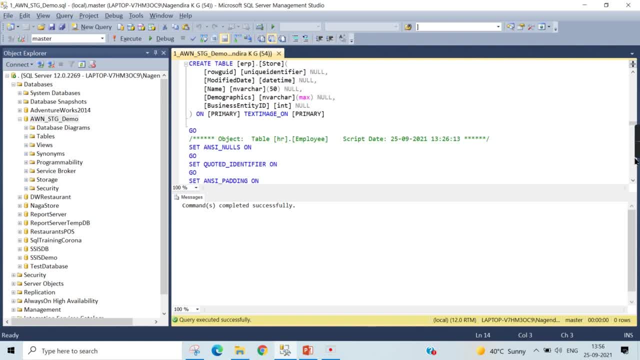 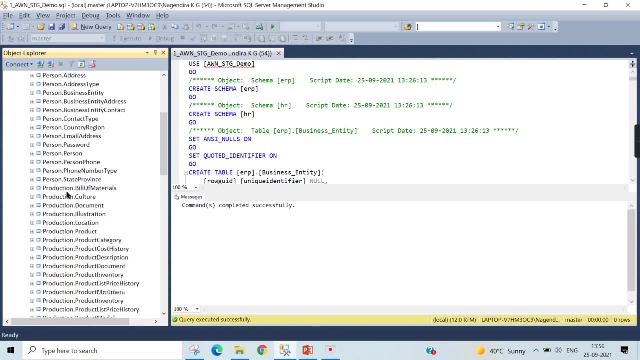 And territory, then ERP underscore store. One point to note here is like before executing the table creation steps, I have created a two schemas here you see the. in the source system you have different schemas. that is defined further specific to the business, correct? so in the staging database the data can. 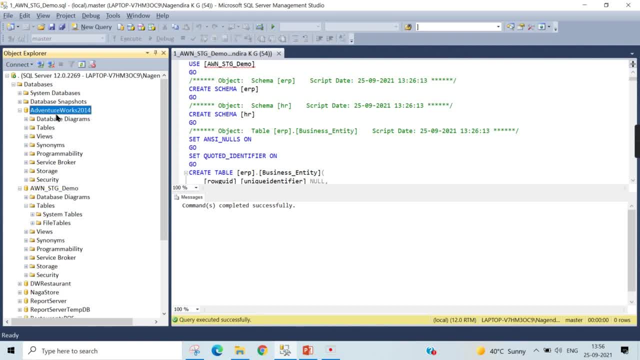 come from different sources. this is particularly especially for a ERP system and some other system can be a human resource, the employee related table. okay, so it is advisable in the staging area you can keep the schemas with the source system name so that you can distinguish between two. it is better because if the 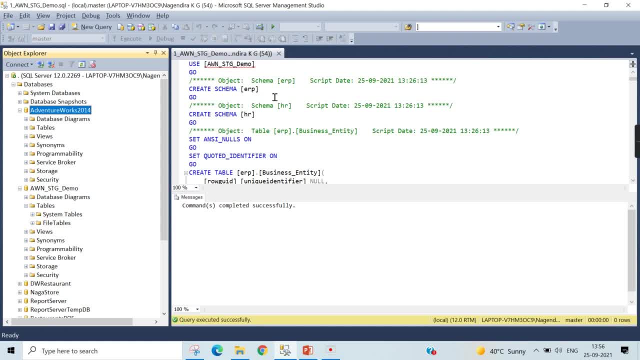 same entity if the customer is comes from ERP system and the customer is coming from Excel or manual sources. so it is better to distinguish between from which source this customer comes from and which source the customer comes from. it is good practice to maintain the source system name. okay for your. 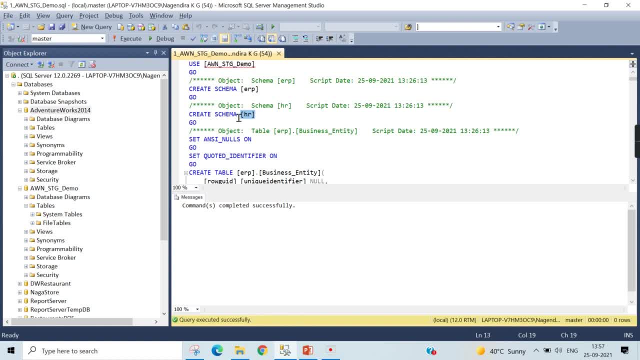 understanding. only I mentioned HR. now the employee details comes from this table only. okay, but assume that is another system having HR. that is why I created schema. so this schema creation is to distinguish the source system. so in the staging I have created the schemas now. now next step is to create. 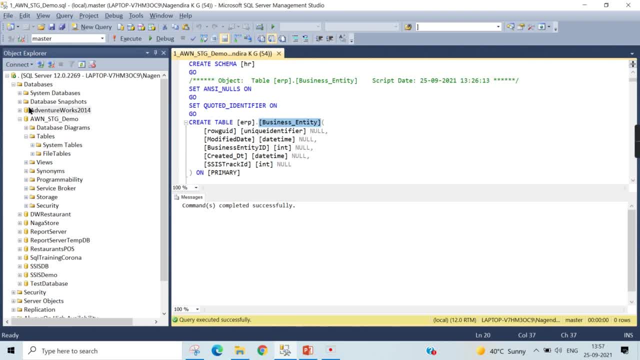 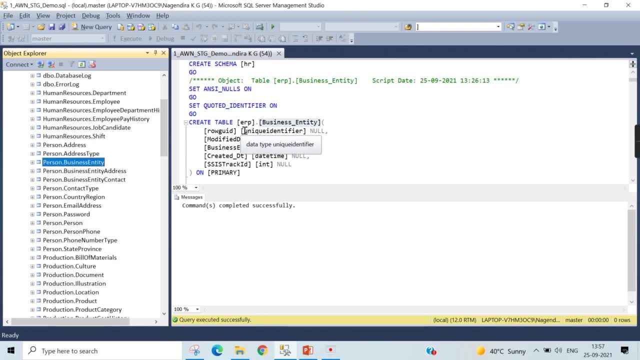 those tables. now you can see ERP dot business entity or that is nothing but this business entity. okay, this person dot national entity. I renamed it as ERP dot business entity, entire system I considered as an ERP. so next step is to create the tables. so let me select all. 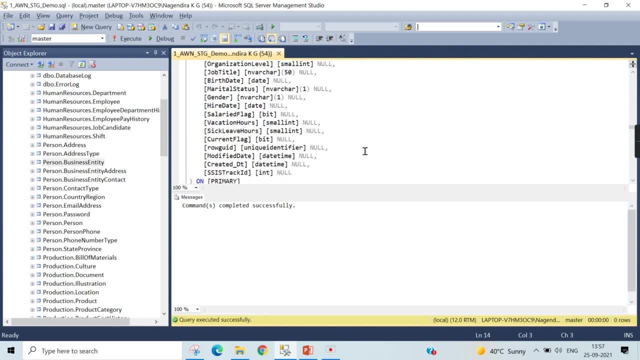 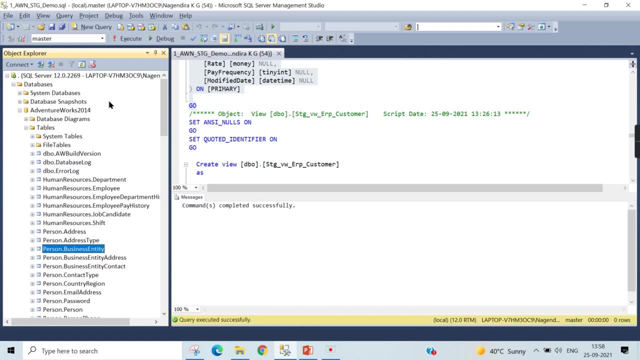 the tables required for this particular demo and then I will execute it. so this is the create table script. till this, it is a create table script and I will come to that views later. I just executed the tables. now the source tables have been created here. now you can see, not here in the staging database- refresh. 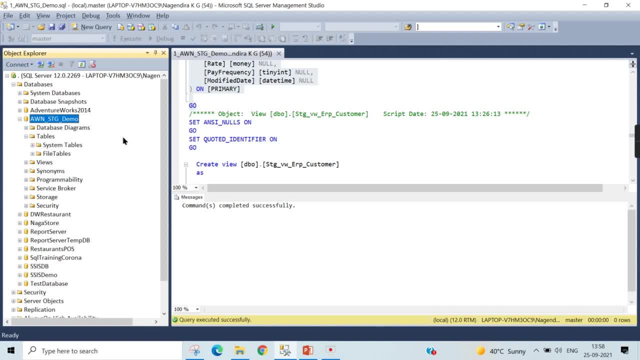 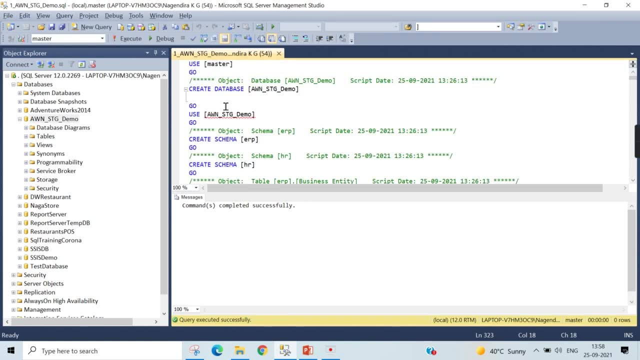 tables: refresh database and refresh the tables. okay, sorry, it's my mistake. I have created in the some other master database, so choose always the the respective database. then only you can able to properly do it. that's absolutely fine. this is how mistakes happen. we need to delete in the master. 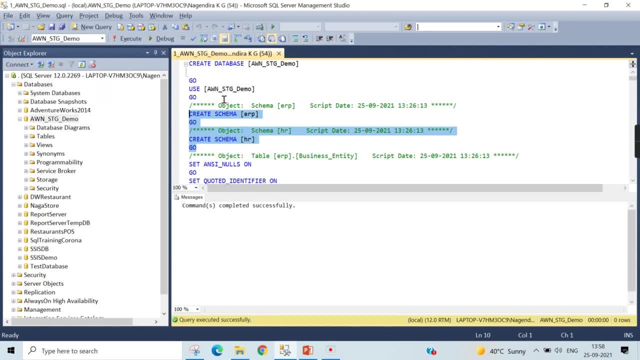 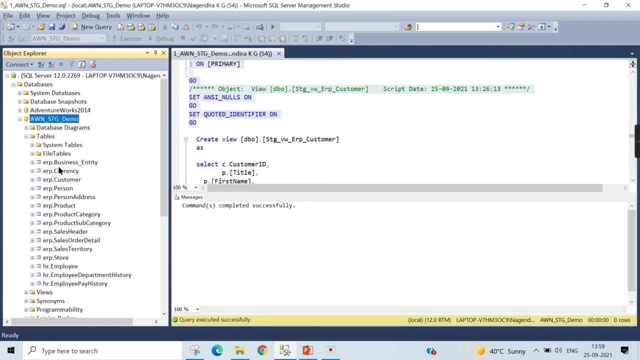 database, that that is fine. so I'm again creating it here in the use AWN staging database, AWN staging demo. then till the table creation, you select those tables okay, and then execute okay. so once you go and refresh here, then now you can see the tables are created okay. 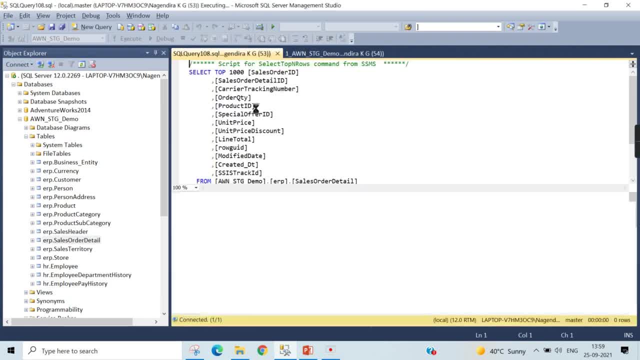 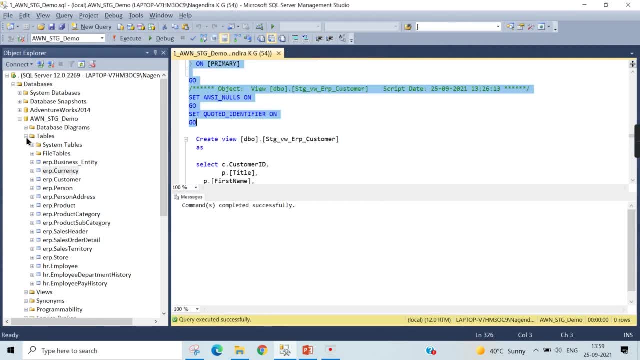 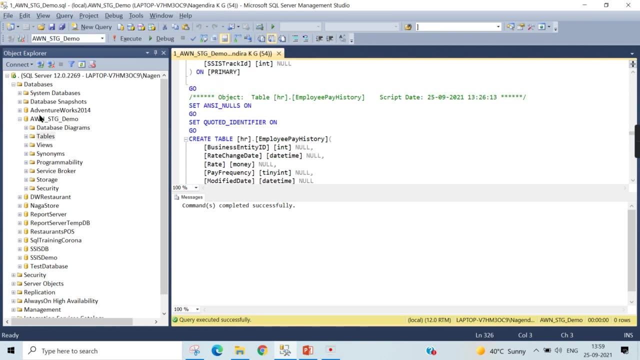 the tables are created. there is no data. you can just go and query it. there is no data and the data is empty, even you select any tables, because it's just a schema. okay, you have identified this. how you can create is how this script is created. you can analyze those source system and get the schemas from the 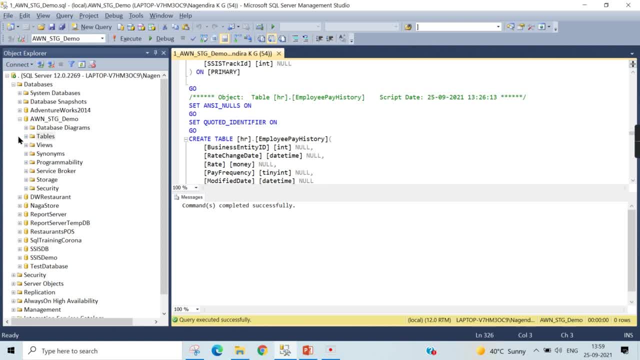 source system. okay, this is one method. another method: while creating the ETL packages from the source, you can create it. that is another way of doing it. okay, for simplicity, I have given this script. okay, now you created the required tables for the from source to staging database. 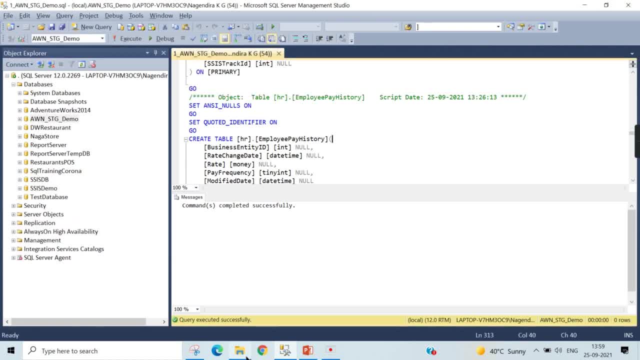 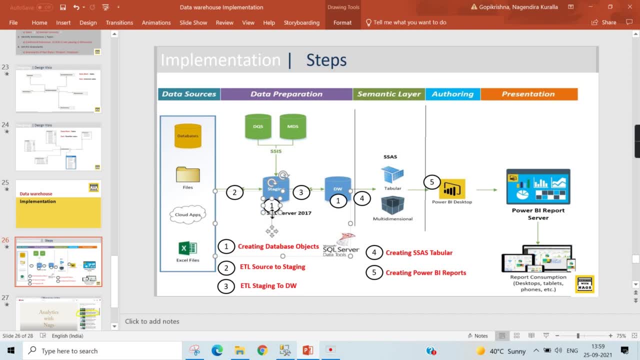 right now. next step is to create the. now let us make this particular thing as a table. okay, let me insert: fill the color as green, so we consider this as done. next step is to: either you can create the database objects as well. this can run in parallel because, in ideal scenario, there is no connection between. 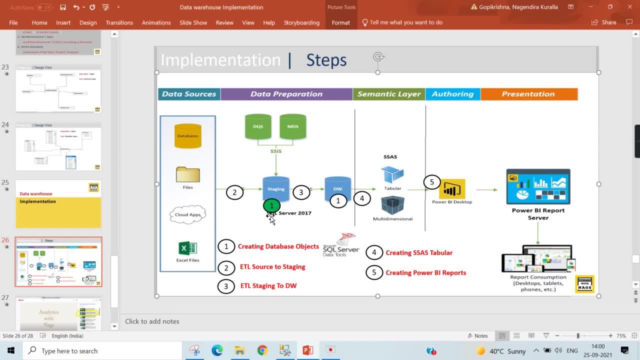 staging and data arose initially for creation of objects. one person can work on staging, another person can work parallelly on creating the database from source to staging and the first step is to create the data, whereas objects- that is how it can- you can easily creating, I mean quickly finish the data. 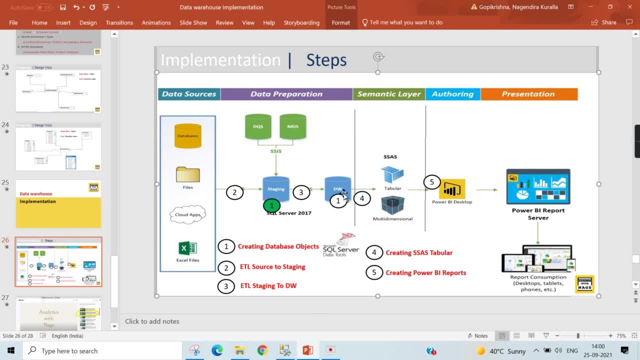 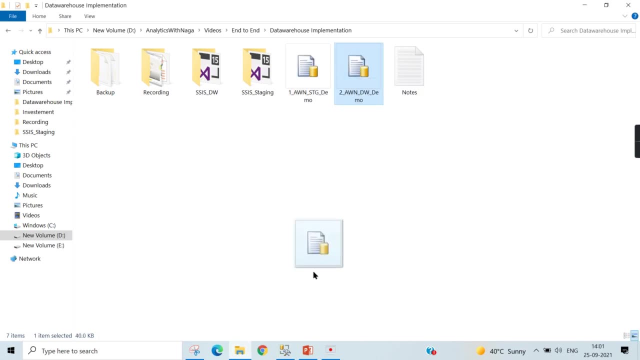 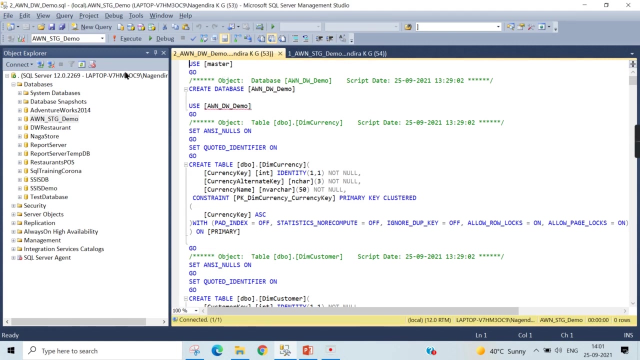 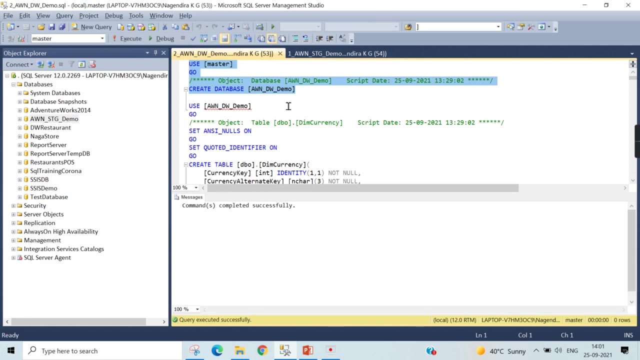 browsing projects. so now I will quickly create the data browsing schemas as well. right table objects. then we will move to populating from source to staging. now next step. it ready now, here again, you see, I am creating the data browsing, actual data browsing database, right? so once I execute the script, it created me one. 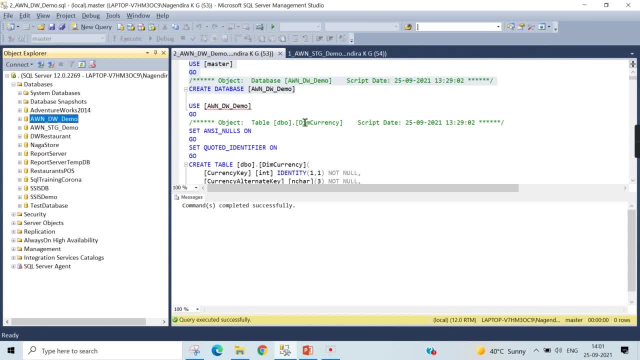 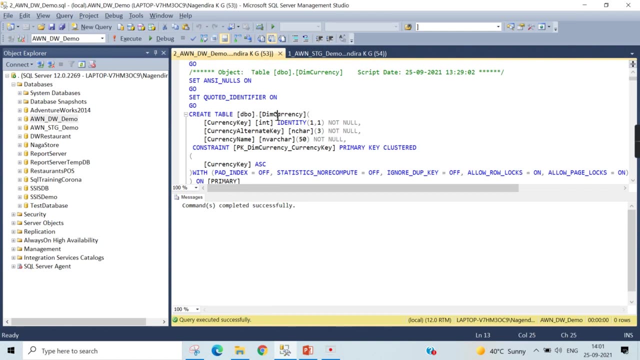 database you can see AWN data rows demo, then I choose this one. you should not make the same mistake: align. so I have used this database now. next, here you can see what are the objects I am creating. I need to create first thing. I need to create the dimensions. here you can see dim currency. currency key integer. 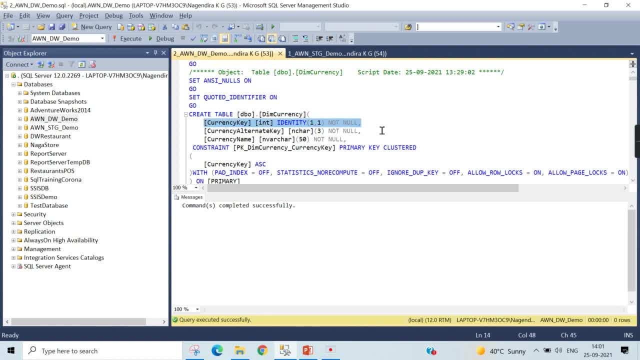 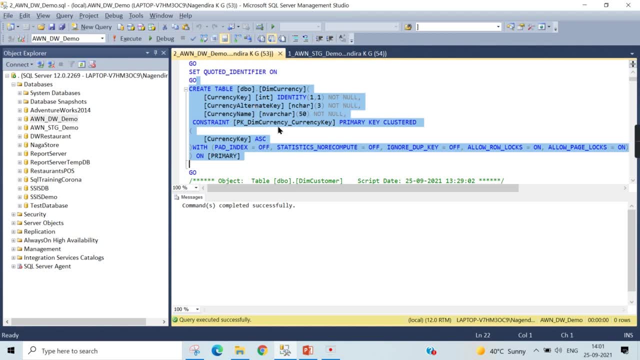 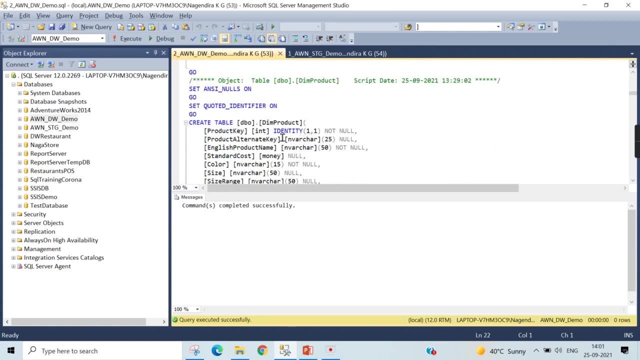 identity. this is called a surrogate key. I will explain it to you later, once I populate some of the dimensions. so this is how you will generate it. okay, this is one of the dimension. next customer: then you have a dim date employee, dim product. okay, so this is how you will create the dimensions and then you have a 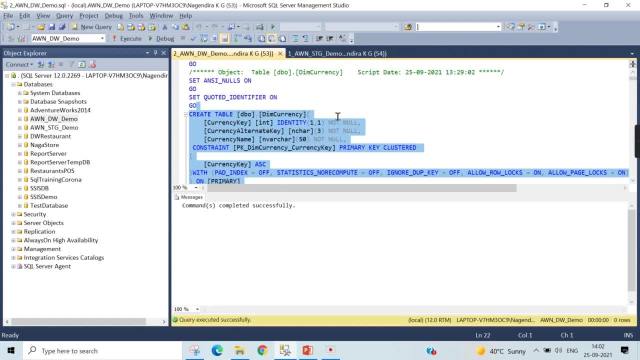 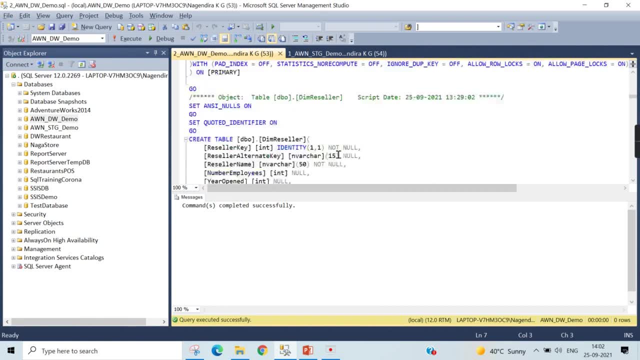 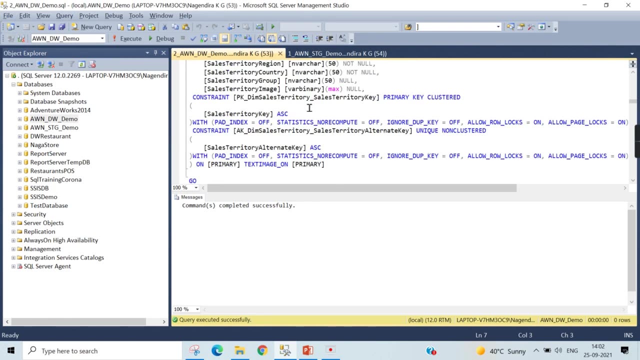 reseller. then there comes the sales territory. okay, so these are the different tables that we are going to create it now. so, in your case, no need to go through one by one, you just execute the script that I am going to share in the description. so till once. the first thing is, like you created the dimensions. 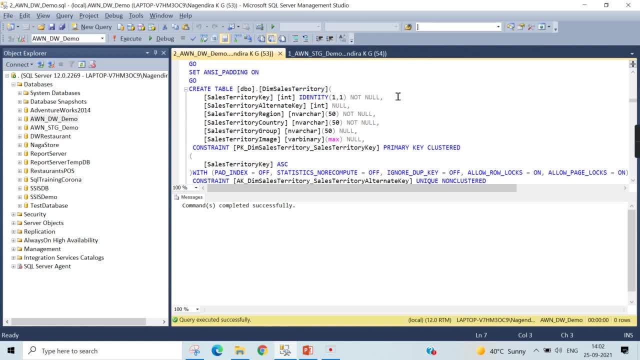 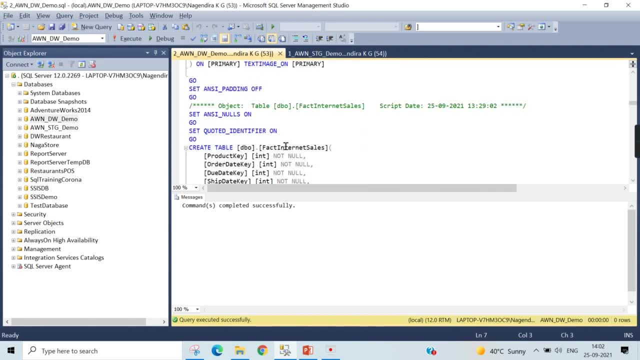 with its own primary key. okay, dimension, as we know, it should have a unique values and it will have its own attributes as well. right then, these dimension keys will be referred in the fact table. now you see the fact: internet sales. it contains product key, ship date, currency key, territory, everything along with the 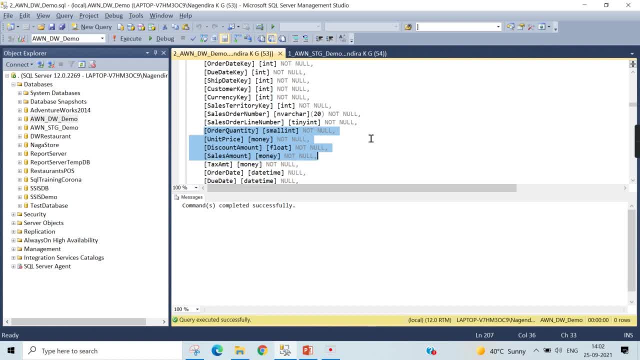 measures. we remember the definition of fact. it contains some measures along with the foreign key references of the dimension table. so that is what we are having it right now. then you can see, you will create some key combination in the fact table itself, in fact table, in this particular table. 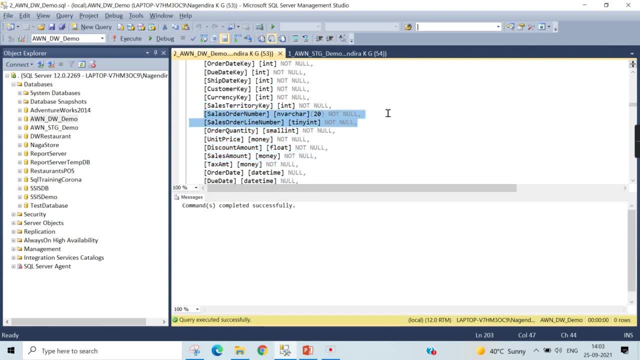 we have a sales order line and line number, which is not a key, okay, but you have this unique value for the fact. fact also, you need to identify unique record. that is, using order line and the order line number. so that is what you create: a primary key. then you create foreign key. right, I will show you the script and 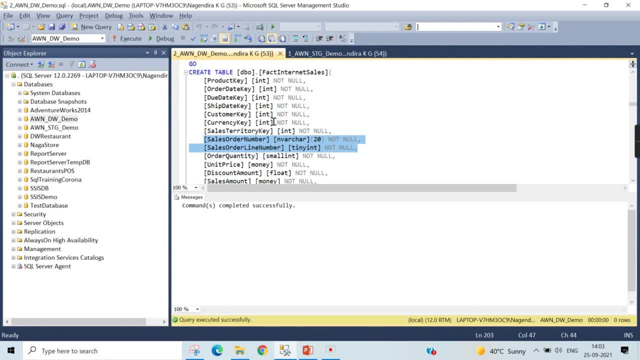 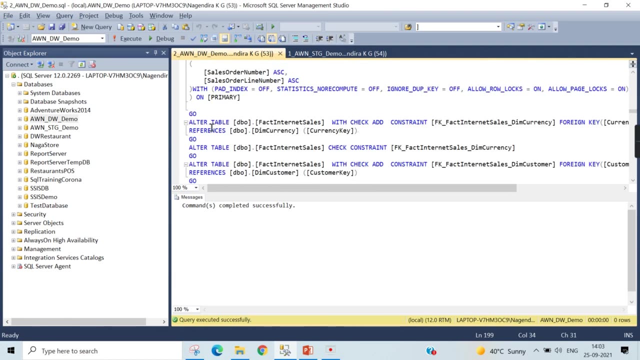 ah, for foreign key reference for these columns. okay, so the next table is fact reseller: similar values, only difference as we see, here it is a reseller, here it is a customer. so that is a difference. now you see the references. alter table. a check. that is the constraint. 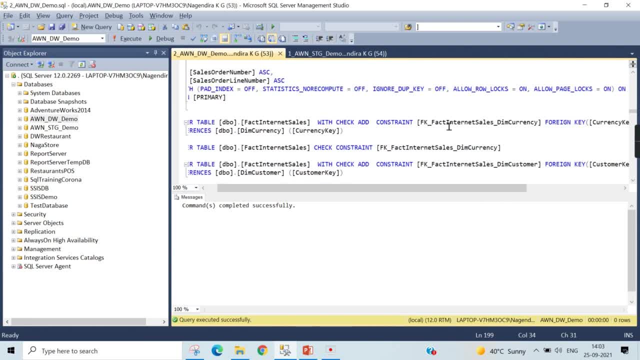 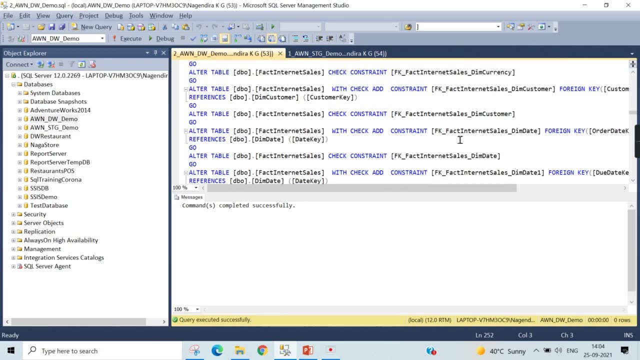 name: foreign key of currency key. in the fact table, the currency key is the foreign key. for which table it is the dim key. ah, so you can see that you have two key elements: your currency, currency key. so, like this, for each dimension reference in the fact, there are four to five dimension tables, for that you will create a foreign key. 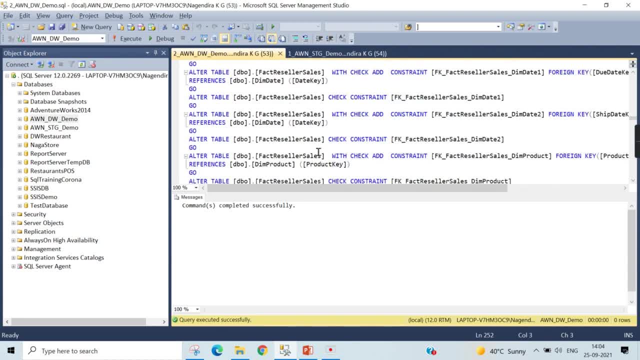 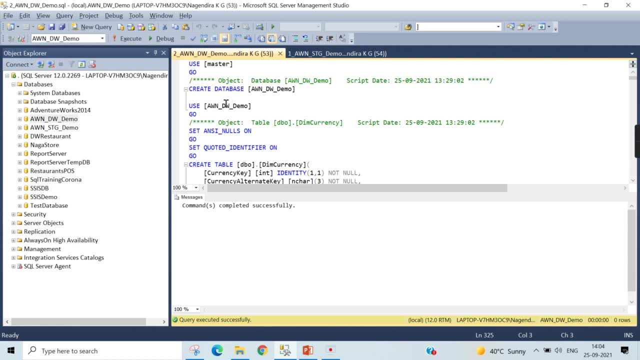 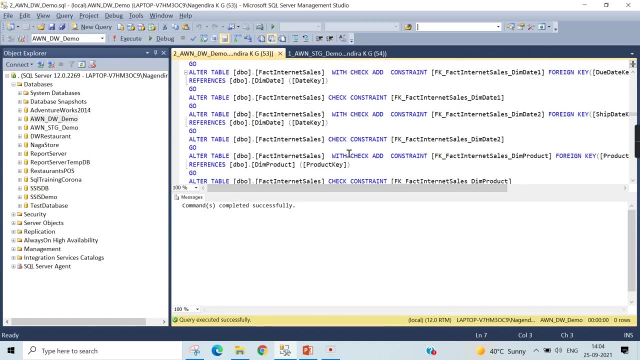 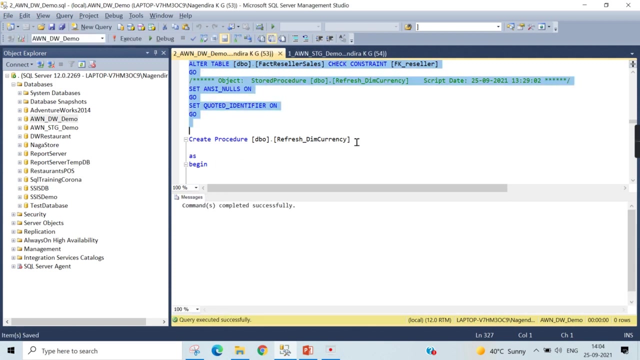 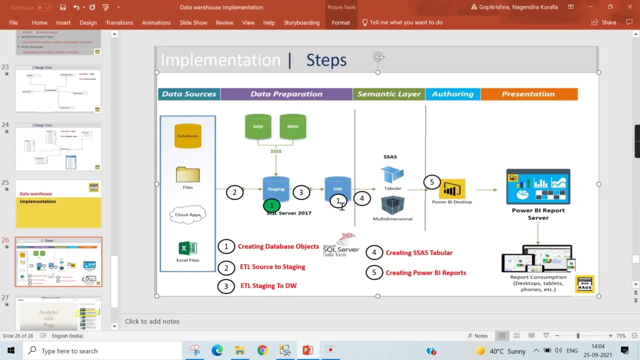 similarly for the reseller fact. so this is the script that we are seeing here. so this is what I want to highlight. let me execute this table creation steps so that we are done with our base, foundation or fundamental concept here. this is done. this is step 2. ok, I mean in the first step. parallelly, you can do: 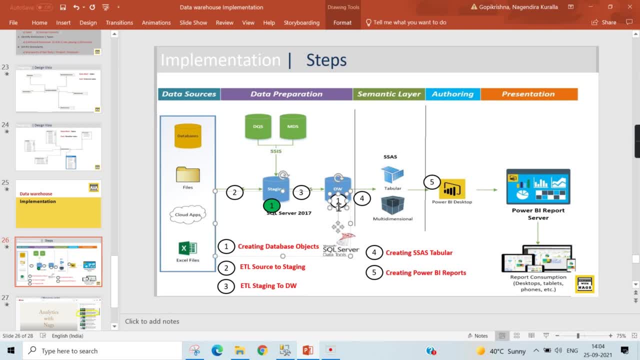 that is how I recommend, because you can do the work quickly. so now we have created staging database, as well as the data warehouse database, and we have created the respective objects. the next stage step is to load this source tables into staging. okay, so how you can load for. 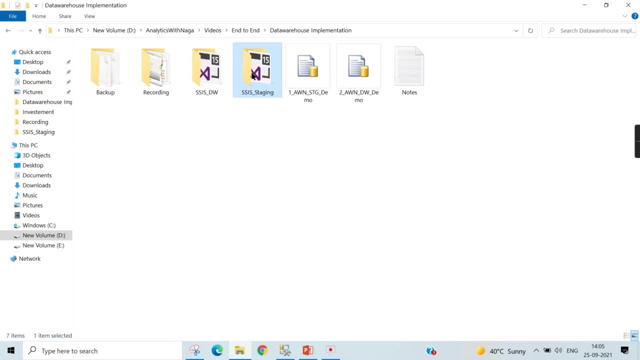 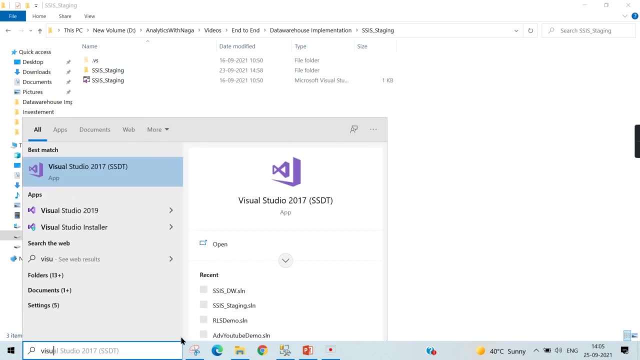 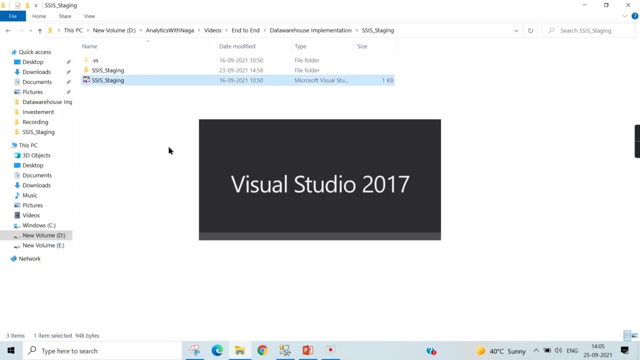 that you need to use the SSIS packages. so there comes a SSIS package. so how you can create- usually you can create. this is not meant for this demo. is not meant for how you can create. you should have a basic understanding about SSIS if you. 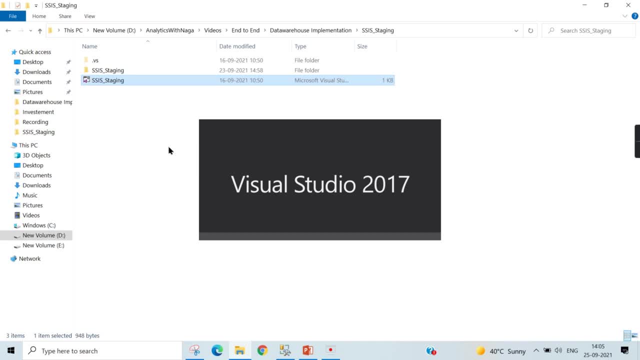 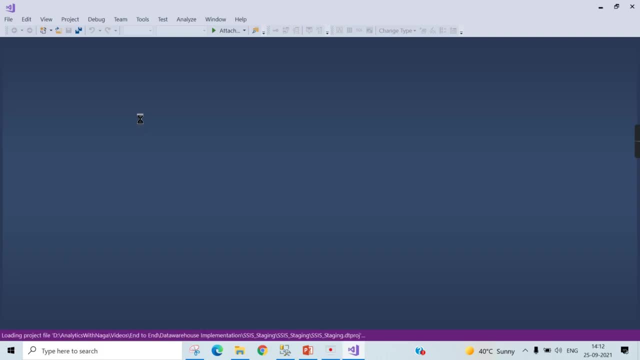 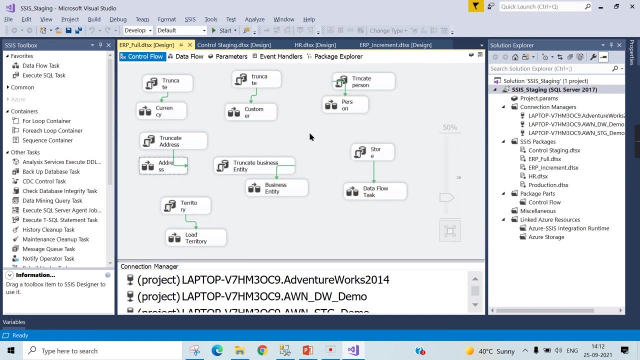 are not having. I have playlist for you you can refresh with the basics, how you can create a simple package. this SSIS packages are already created and this is not focusing on teaching you what is the basics of SSIS, for if you are not aware what is SSIS and how to use it, this is not video for you, I mean you just check. 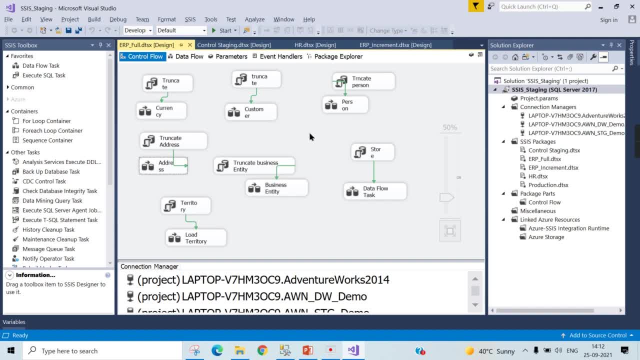 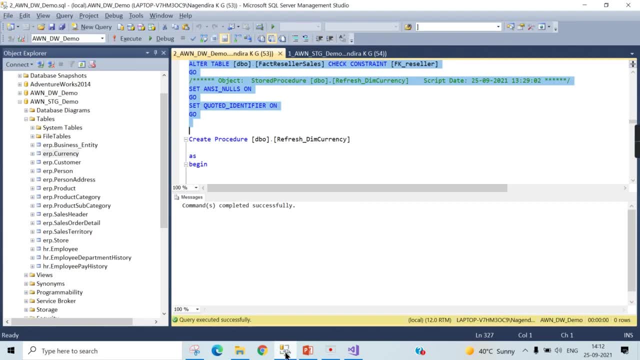 my playlist- SSIS playlist. you can learn it, how you can use it. this is not video for you. I mean you just check my playlist- SSIS playlist. you can learn it how you can do the ssis packages and here what, what we are trying to do here is like: 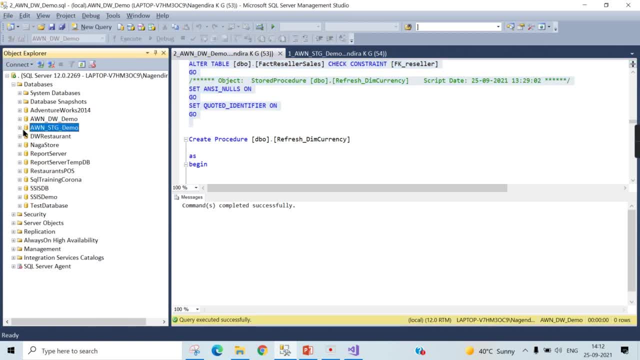 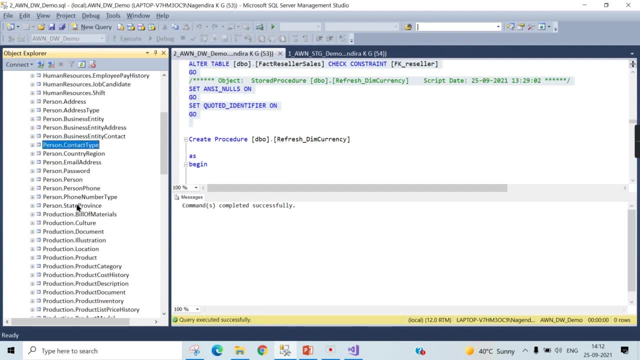 from this source. okay, this is the source. and then there is the staging. assume you need to load the table from. i mean currency table from here. the currency is in sales. okay, where is that? yeah, sales currency. this table has to loaded. the data in this table has to be loaded. 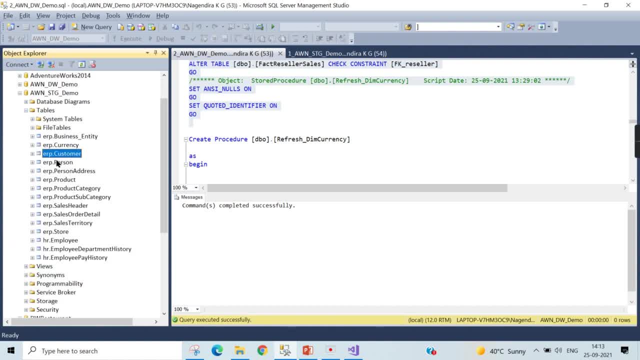 in this awn, staging database right, how it can be done using the some tools, etl tools. that is what these exercises meant for. and now the one more point to highlight is, like those who are not familiar with the servers and architectures, this source will not be in the same database. 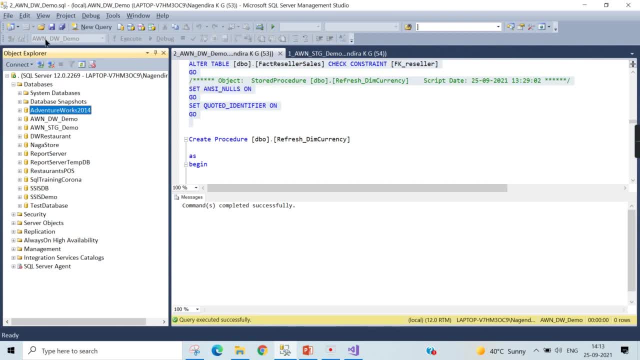 that is not ideal scenario. this erp will be separate servers. we need to connect and load it. okay, but i do not have another server because it the this particular server or database is maintained in another environment. completely okay, due to i do not have different environments, i placing in the same server. okay, for your information. and now to load one of the table. 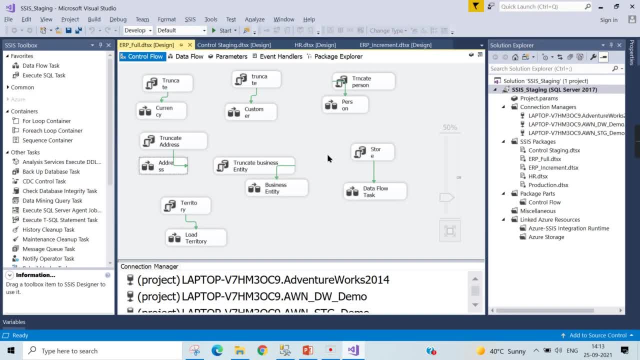 from here in the staging how we will do it. let's take the currency. okay, so here what is the package i use. so these two tasks will do the currency data. i mean load the data from the source oltp system into staging. so basically this will clear the data if already. 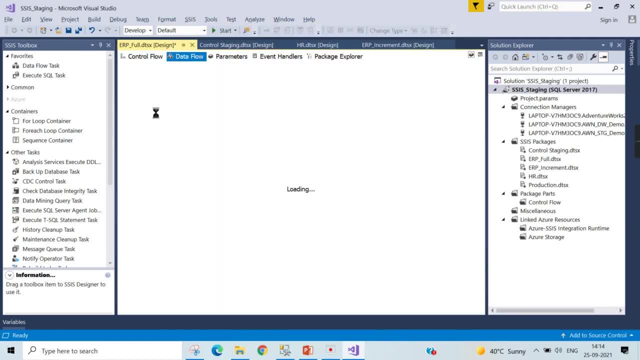 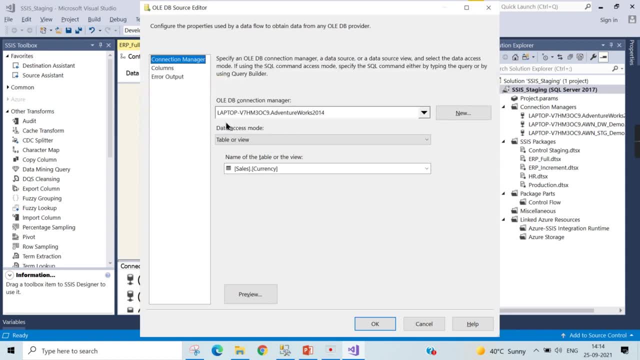 exist. okay, then this particular task- data flow task- does the actual source to target transformation. so you can see the source. this is adventure works, this is oltp system and the target is your erp dot currency. that is in the staging. so that is how you do then this. 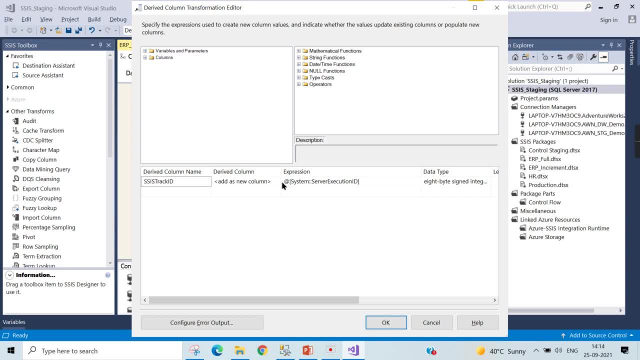 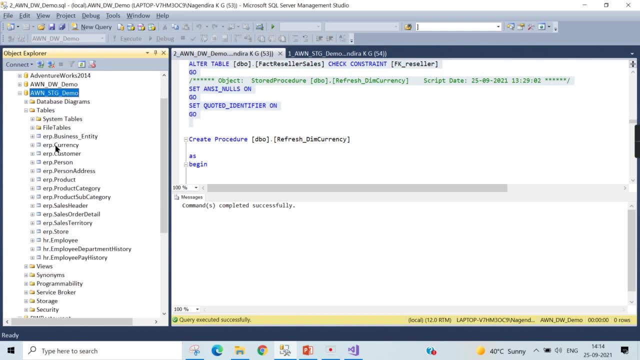 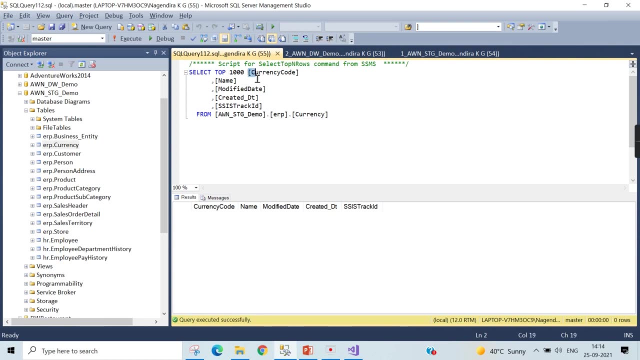 is another important concept. like you have ssis tracking id where you will keep the system dot servers execution id. what do you mean by that? let me show it to you. let me query this currency here. this is erp system currency, so i get currency code and currency name and when it is modified, 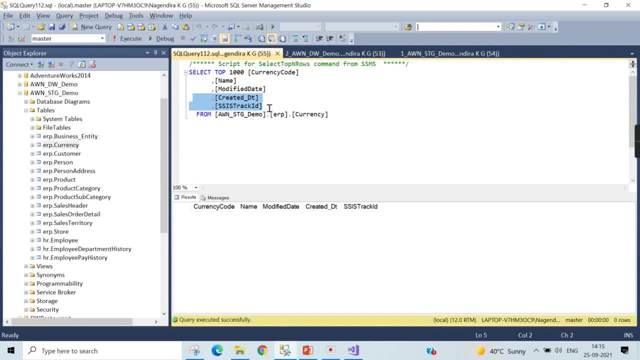 this is the erp system that is being used for tracking the data. so if you look at these two technical columns, that is created date and system tracking id that i created in this staging database. okay, let me show you the script of this. basically like this: created date will have the default value. 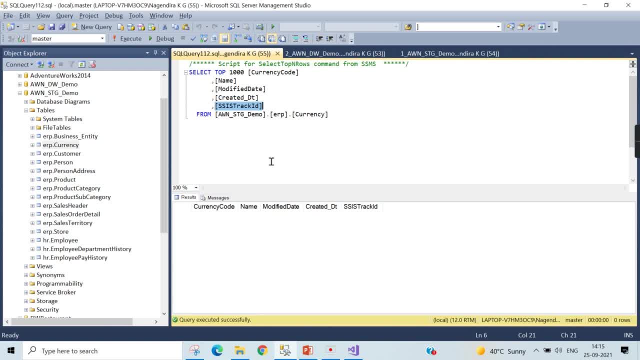 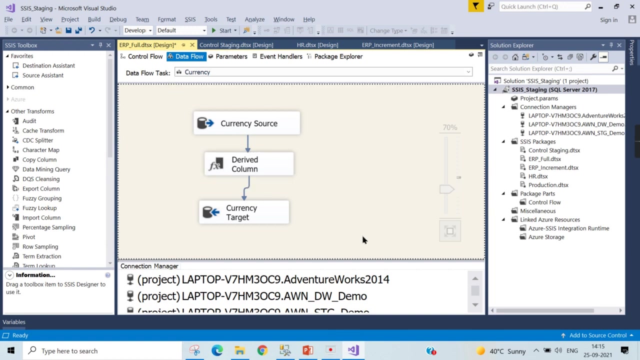 when it is stamped in this staging database. okay, that is how it should be. this ssis tracking id is Okay. Whenever you schedule this SSIS package in the agent job, it will create one ID, because it will be better. You will troubleshoot it because you need to know which one has brought this record in this table. Okay, This is for troubleshooting. That is, for your information. So that is how you will map it. Okay, Using a derived column. So this is why I insisted you to learn the SQL and SSIS while designing a data warehouse. 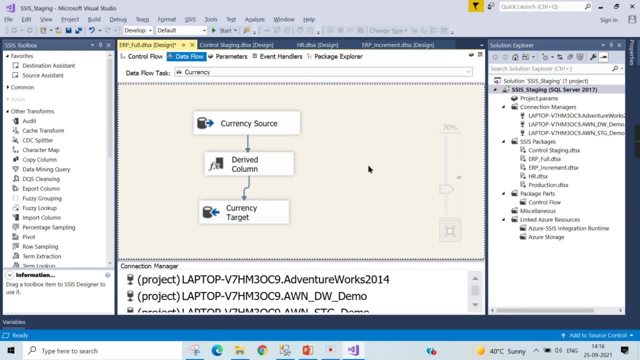 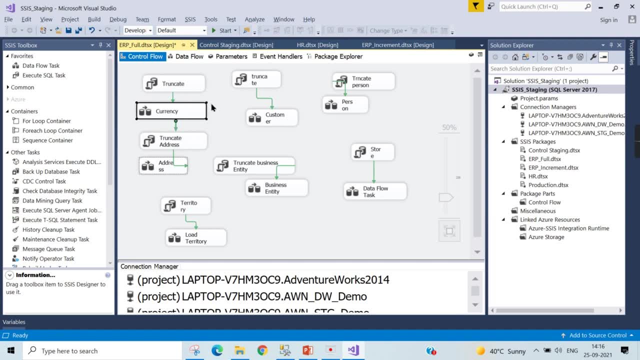 Understanding even Power BI, because all these concepts are interrelated. That is fine. Now I have made these two things mapping. Similarly, I have made all other tables required for my loading into staging. Okay, Now, in order to execute only this right, I need to use the. I cannot run the both the tasks together. I can either run single task. 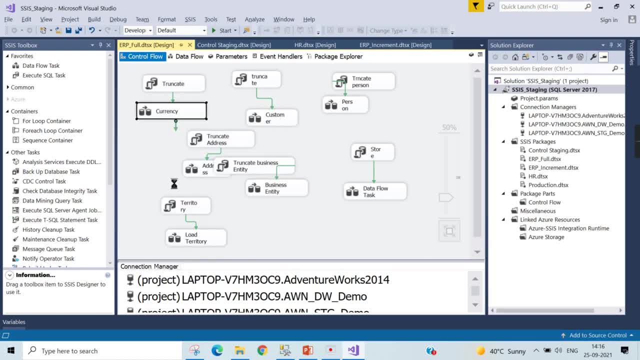 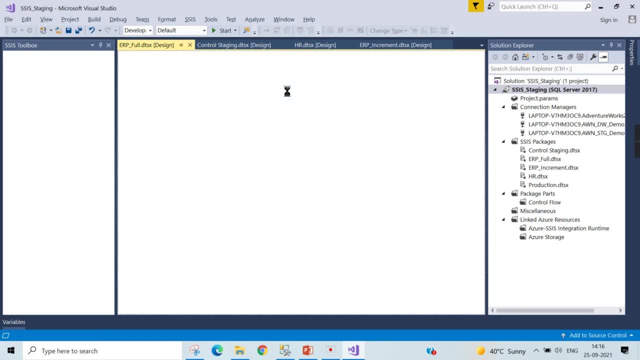 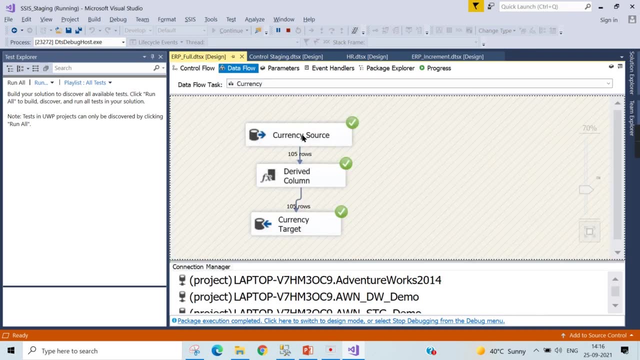 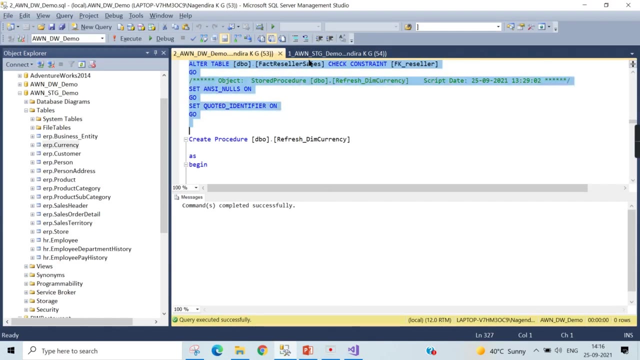 Let's say, Let's say like, if I execute this task alone, Okay, Now it will go and fetch me the data It is building the object. Okay, Now it will go and execute it. Now, you see, it will be very quick because it doesn't contain much tracker. You can see 105 rows read from here and 105 rows it has been loaded into target. So when I query it earlier- right, because when I query it there is no data- 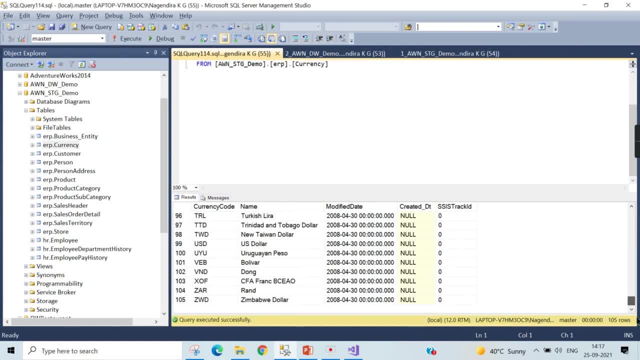 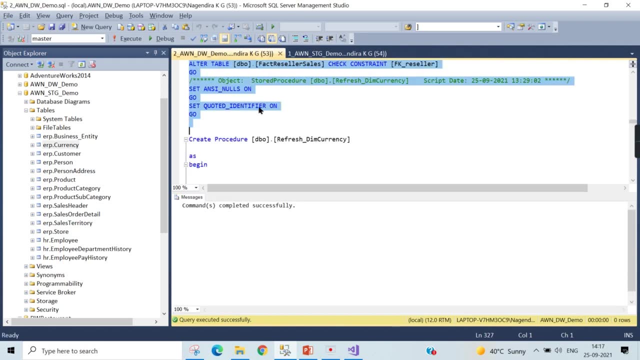 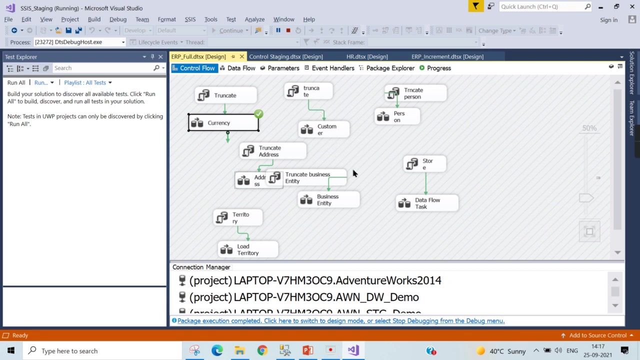 So now you can see in the staging we have got the data over here. So ideally it will be like a get date. The get date should be the defaulted, So we can add it. I missed out. That is fine, You can add it for your reference. So now we have loaded it here. Now, similarly, you can map or do the multiple table mapping one by one. It is manual work. 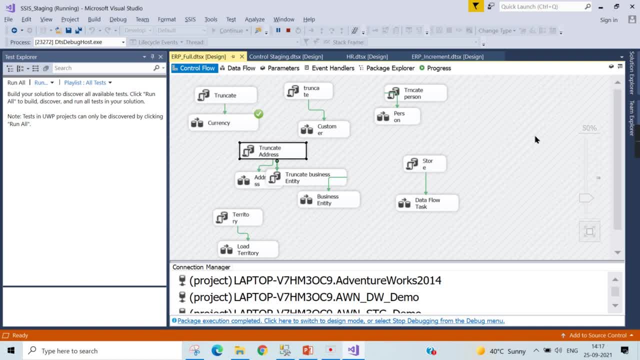 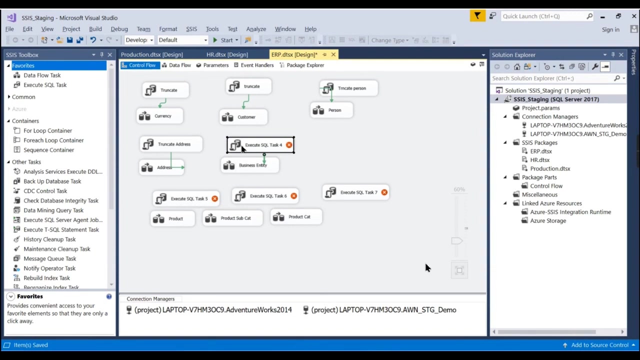 have a choose, some tables, and everything will be generated. every, each and every table has to be manually created. okay, that has to be manually done. I will show you quickly how I developed while developing it. it took a long time. I will fast-forward it for you now. so now you can see how I manually did some of the 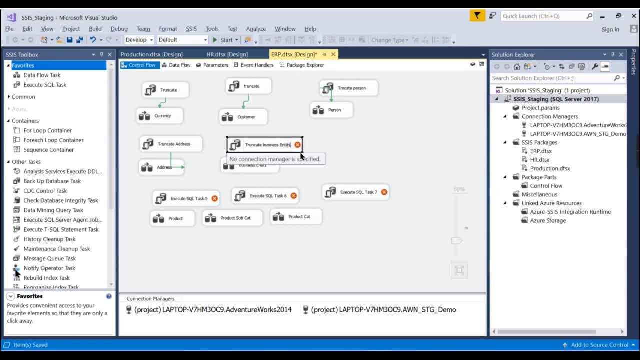 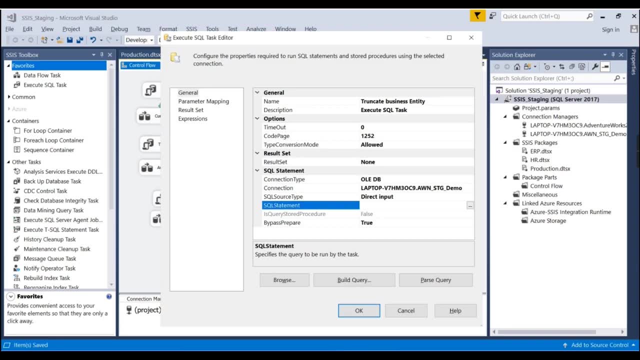 tables. I will quickly walk you through for one or two minutes. like this is: I'm doing it for entity where I need to choose the source and then I need to rename it properly. see the business entity I'm doing it for. so I'm I need to. 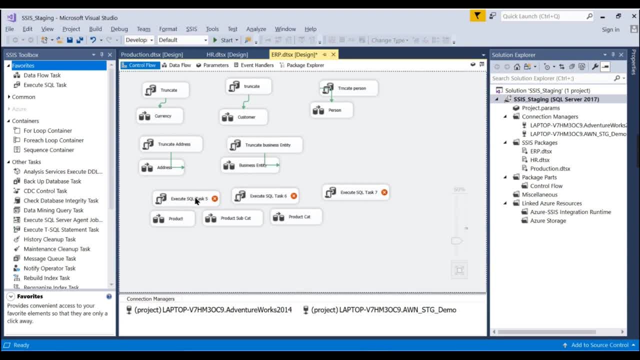 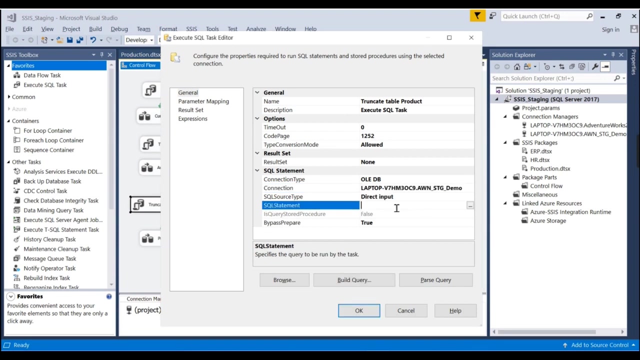 paste that right. I need to copy that script then, and I am doing it for product table, so let me do some fast-forward for it. please speed faster so that it will be very quick. so I'm doing this for a product table where I'm choosing the staging because I need to truncate that table while loading it. so 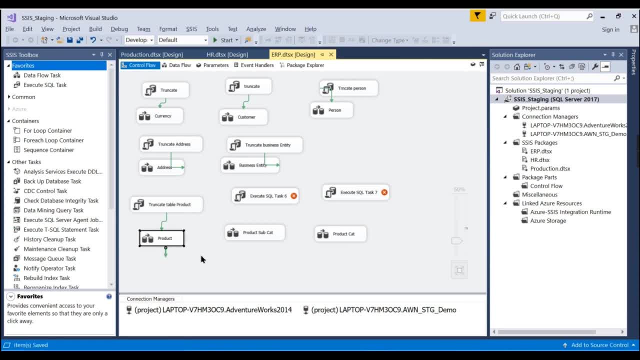 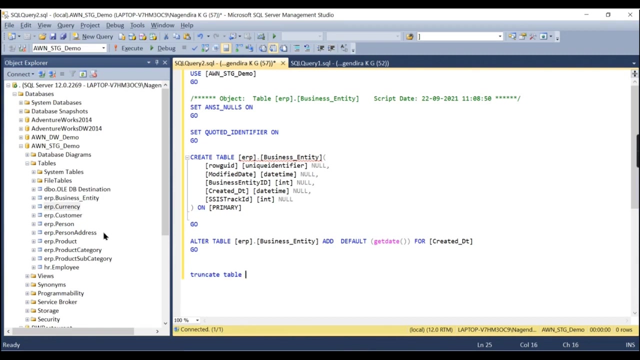 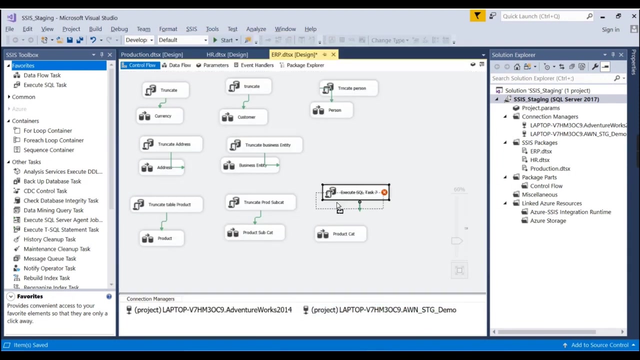 I'm just doing that now in the product table. okay, so now here I have a mapping or not. I need to check. you'll check it out. I think I did all the mappings before the all the tables. I am just using that truncate concept only. that is why you don't see how I do the mapping from the 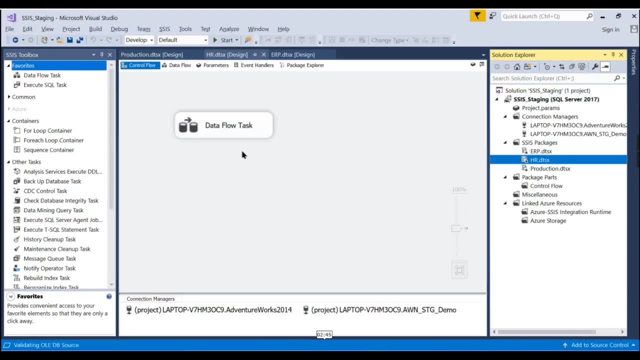 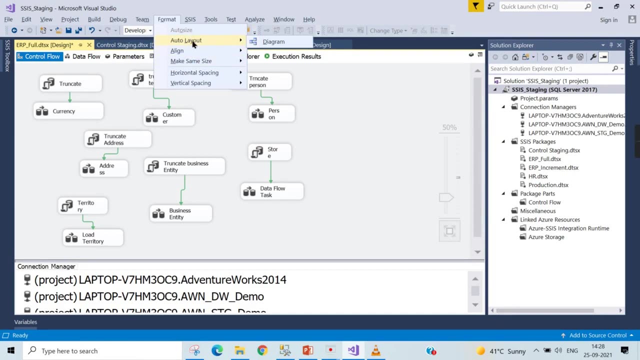 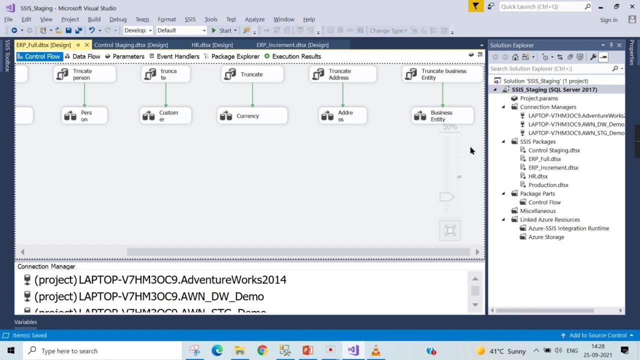 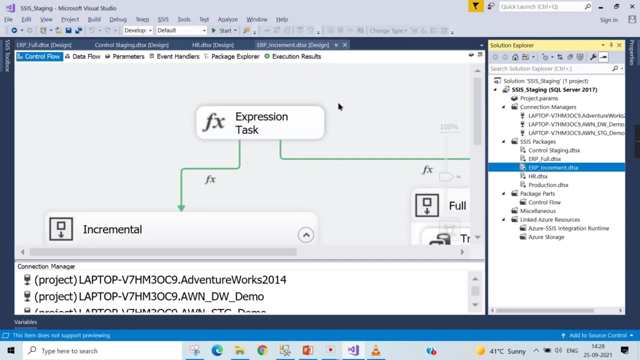 source to target. so that is absolutely fine. let me fast-forward this also now. I this is employee and there is no table here. I hope you understand now. now let us align it properly. so now again, before saying I mean running this package like I have designed it, like ERP full and ELP incremental package. I will come to this. 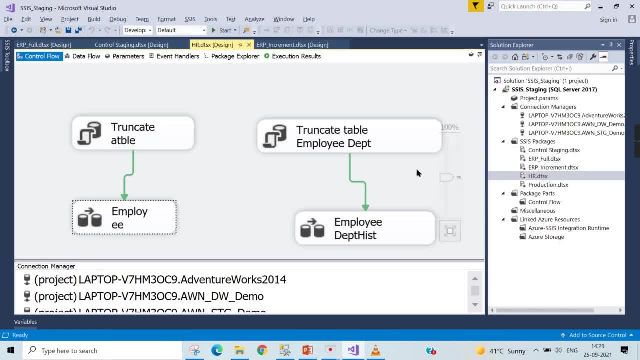 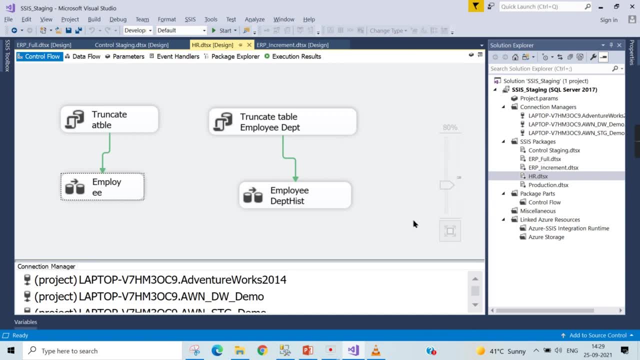 little later. so again here, based on the source system, you can define the packages right. so ERP is one source system. you can define all the tables over here and the HR will be another department or another source where you get the data. you can keep it here, then, one important point I want to highlight. 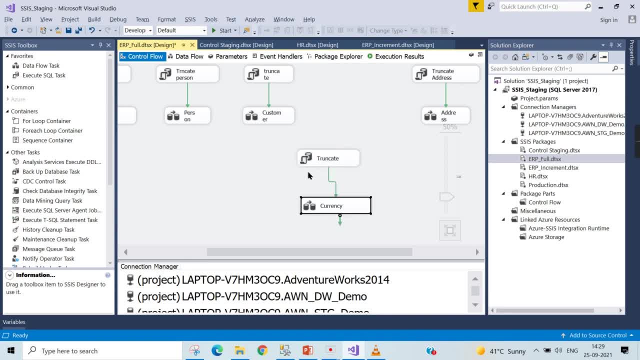 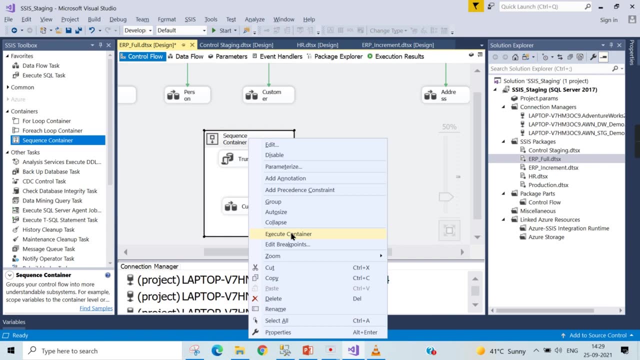 is like while troubleshooting, if you want to run only this particular package, you can run it before you can execute, right click and execute. but you cannot do together. for that only we use sequence container. what, in this case, what you do? you put it together, then right click and execute it, so you can run multiple tasks. 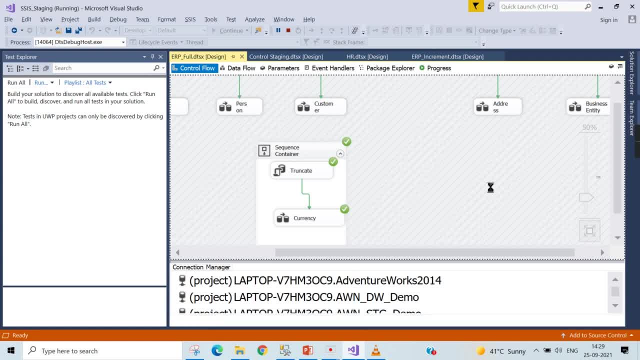 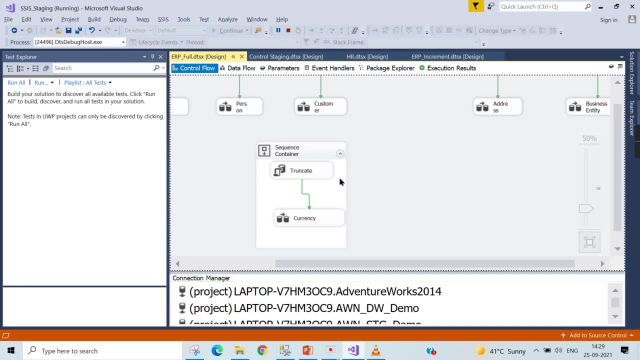 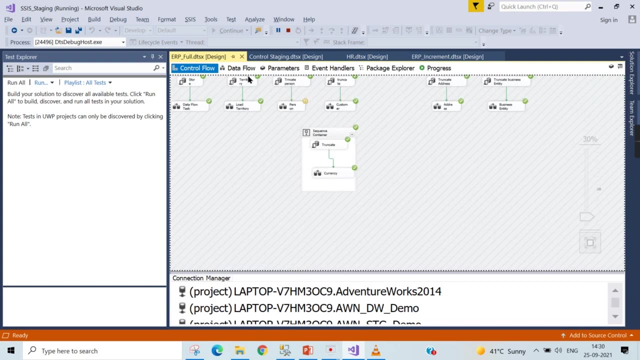 okay at a time. so now you have loaded it here. so let me run this ERP full package. now we are trying to load the data for some of the tables, that is, especially the dimension tables. now you can see all the tables are green like store territory. person. person is running maybe. 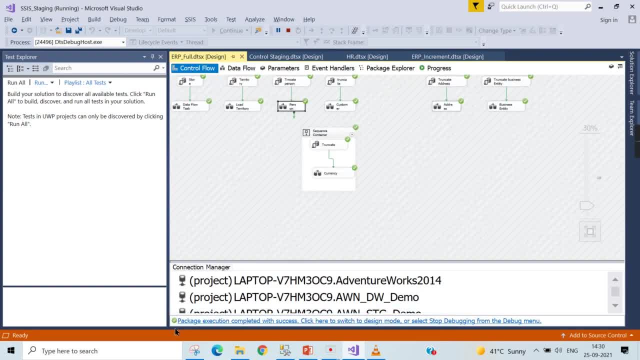 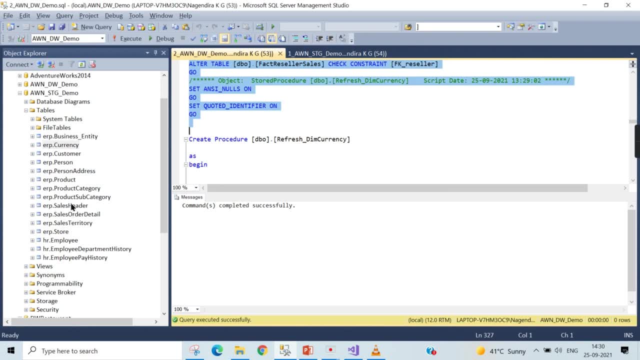 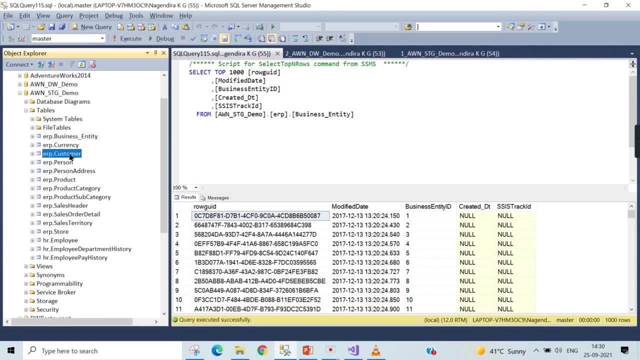 it contains some data. now it is also completed. now it turns into green here at the bottom you can see. so now all the tables are completed, except the sales. okay, that is the fact table. I have designed a different package. now you go and query those tables. everything is in place or not? yes, it is. 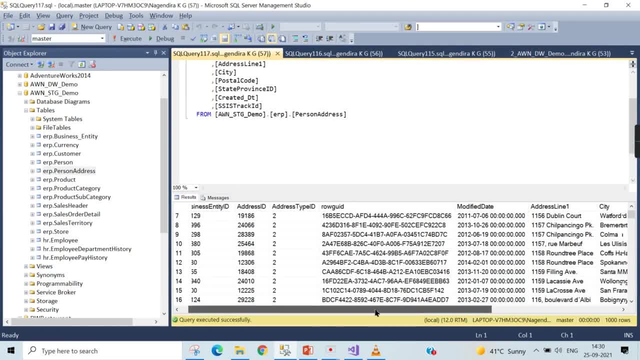 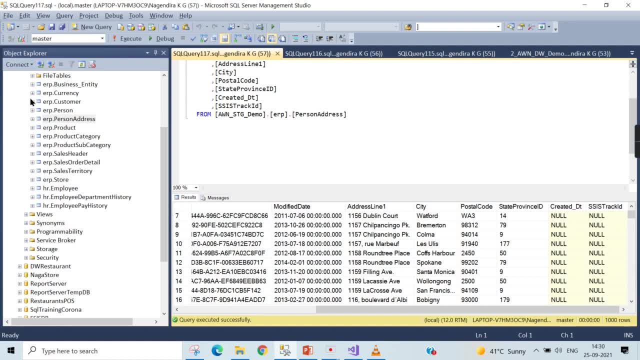 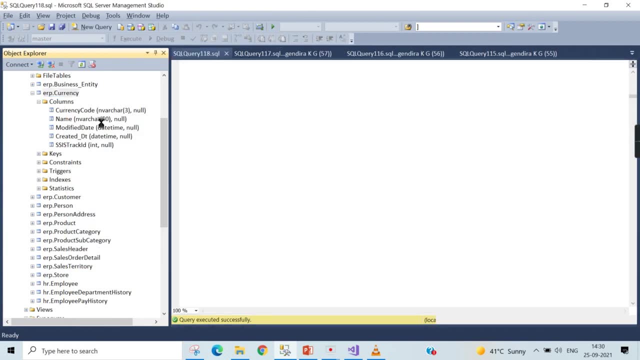 so now you can see all the tables over here. it is populated. that is absolutely fine here. I didn't do any mapping. just for your understanding. for one of the table I have put that SSIS tracking ID so that you will properly implement the solution, even the created date you can put. 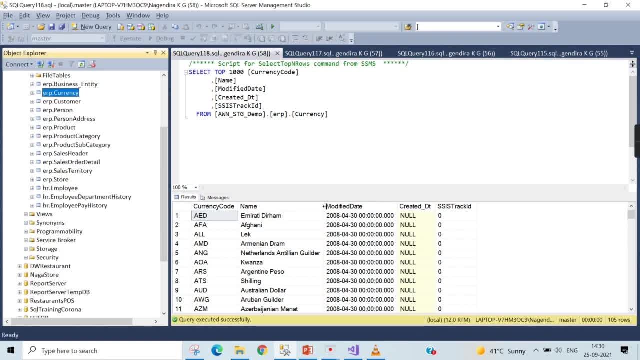 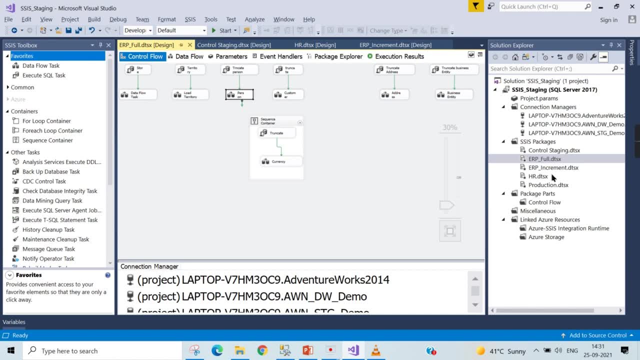 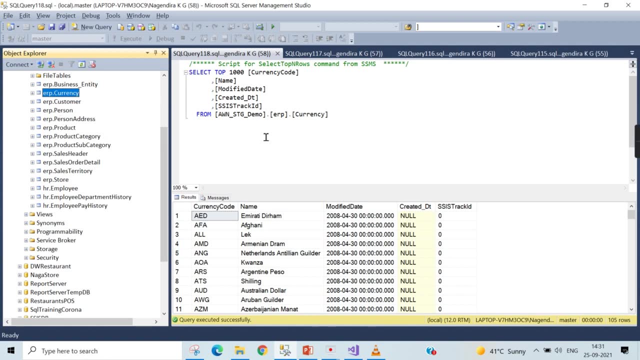 the default it to get date. so this is fine. now let us talk about the incremental load for the tables. okay, so for small tables like this, you can truncate and load it. obviously it is fine. but what about some tables? it is very huge, right? you cannot keep pulling the. 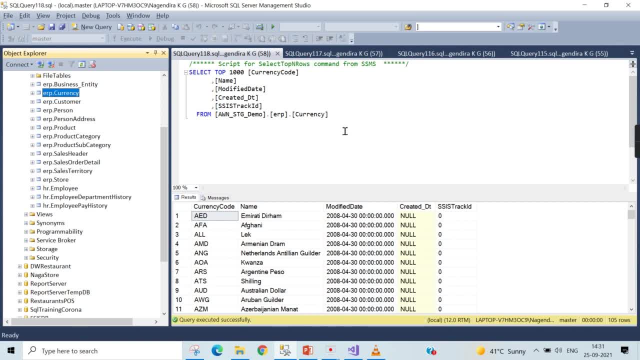 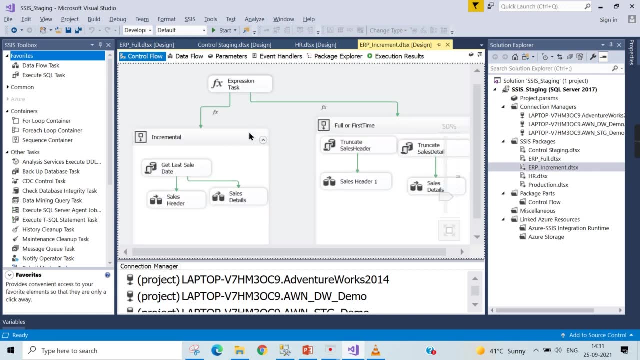 entire data from the source to the target or staging. so in that cases, like order detail, order header, you need to do the incremental load well designed, right shape dimensions of the tables. this page is ready for the pack. I have defined the whole model and now here we present you howлет, that is. 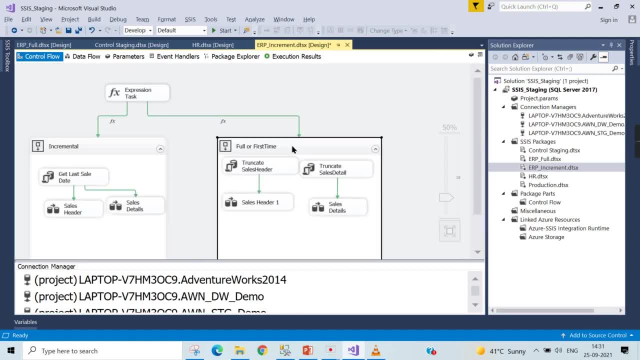 how will you design it? that is the question now for this. this is the package I have designed here. it is very simple. concept like how you can implement it here is like: this is the full, our first time load, meaning like the first time, whatever the data in. 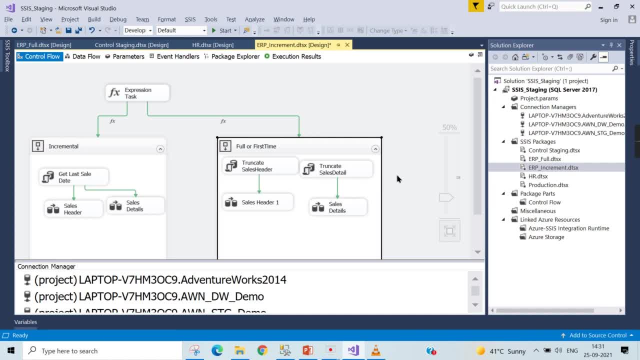 the source, it should read data. I mean that way. we implemented data arrows so we need to truncate and reload entire thing. that that is in the beginning stage. I'm saying so we need to load the entire data one time, once we load. after that, once we populate the 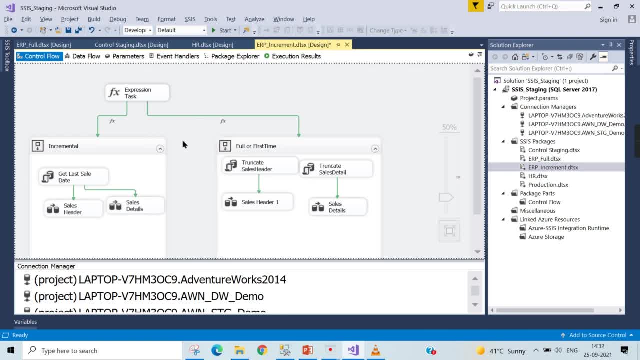 fact table right, then we will do the incremental for that, you will do the this particular incremental. this is very simple method. there are very proper way of doing it for you to understand what is incremental load. I have designed like this so to explain this one: the sales header and sales details. okay, these 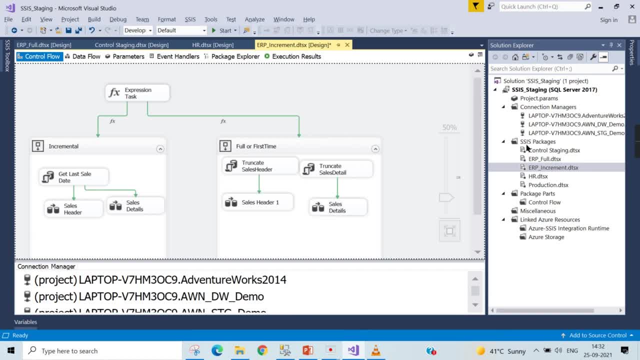 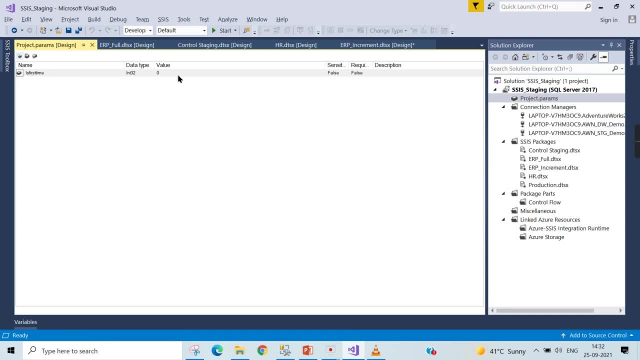 tables we have to bring from the source to target. so how we are designed is like I have created a project. parameter is first time load. okay, that is set to zero means it is incremental. if it is set to one means it is full load. so now you. 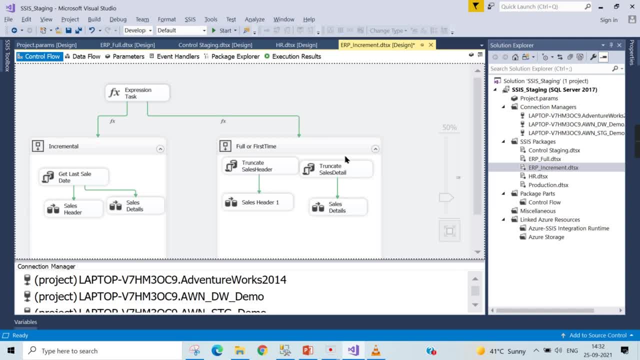 can go and check this ERP incremental package. what I have written here, it is just a dummy expression. now here I have written the logic here. here the project is first time load equal to equal to one, then use this flow. if the project first time load is equal to equal to zero, then use this flow. so either one of the flow. 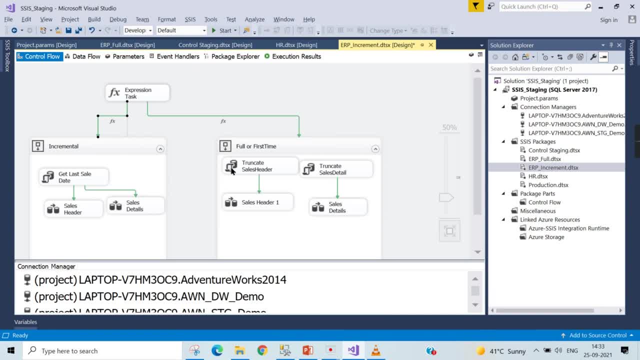 it will navigate. that is the main purpose. I need one taskbar. you can go and check this ERP incremental package. what I have written here: it is just a dummy expression. so I have written here: it is just a dummy expression. so I have these two tasks. that is why I use the sum dummy expression task. now I have set. 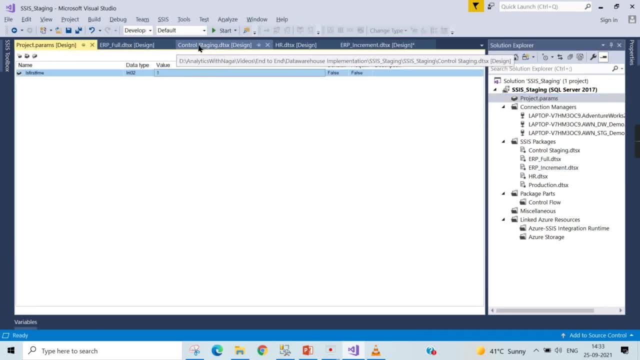 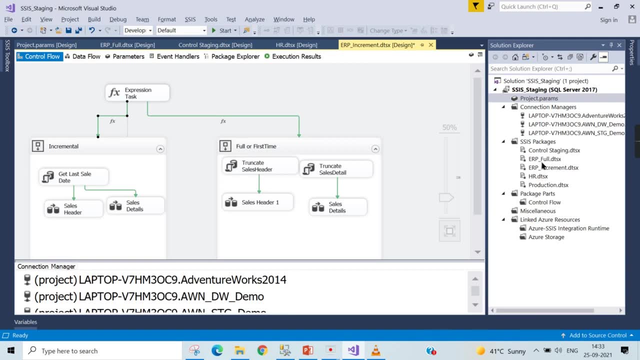 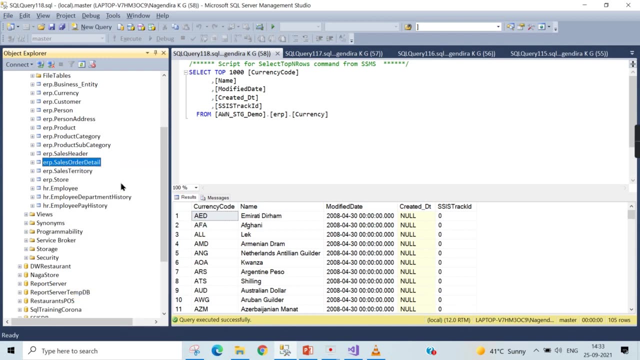 these two tasks. that is why I use the sum dummy expression task. now I have set this project expression, I mean, is first time load equal to one, so this will load entire data from the beginning. okay, now let me run this incremental. now you go and check here. before this, you do not have any data in the sales order detail. 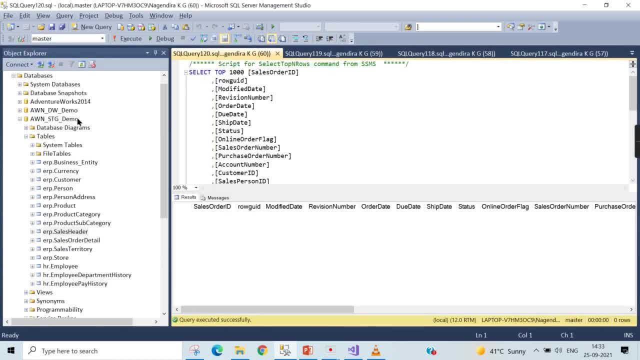 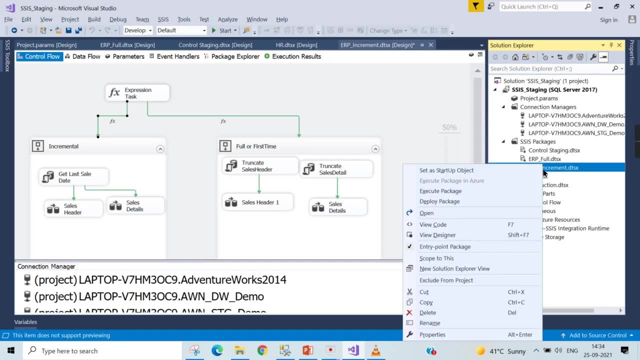 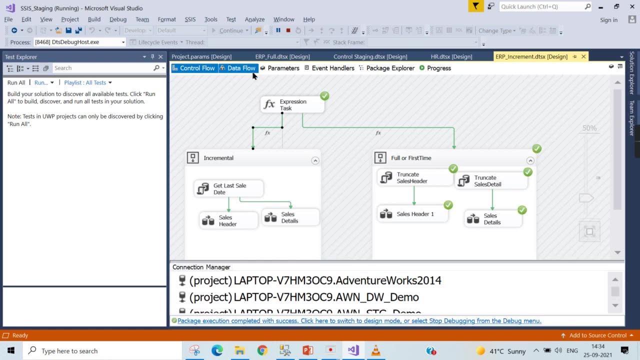 as well as sales header. okay, this is what the sales header is and this is the uh, the staging um in the date staging database. now let us run this entire package, execute incremental. now you see the data has flown to this path. okay, to this path. now you go and check. 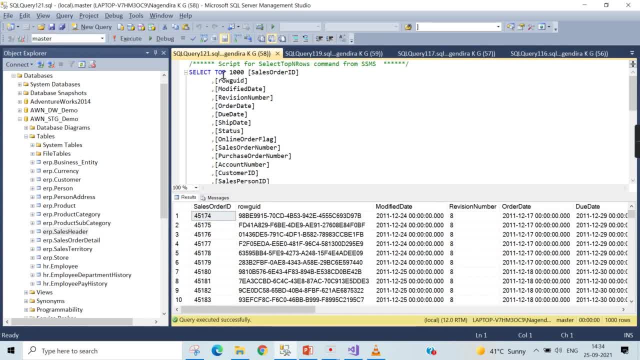 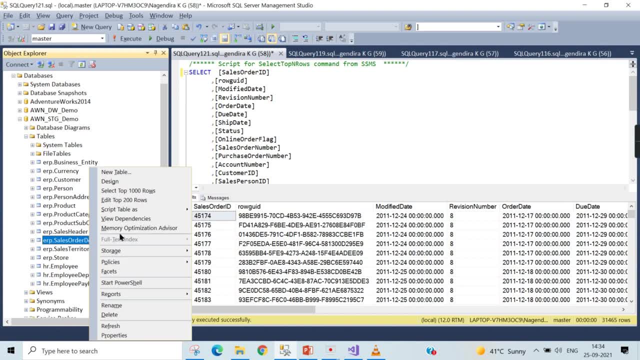 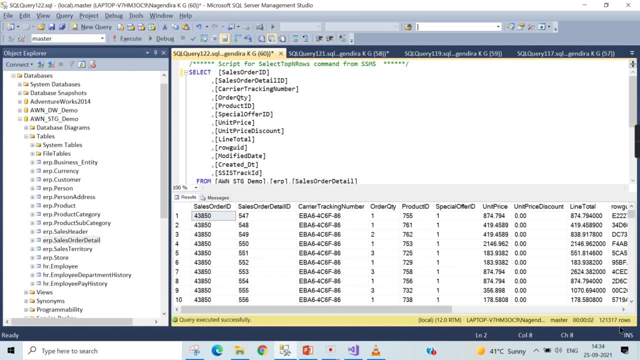 uh, the data over here. the data has been arrived. there are around i think 60 000 or um. there are 31 000 in header and it is more over here. i think it's around um hundred and twenty one thousand here. okay, in the detail. so both the tables we have loaded. so 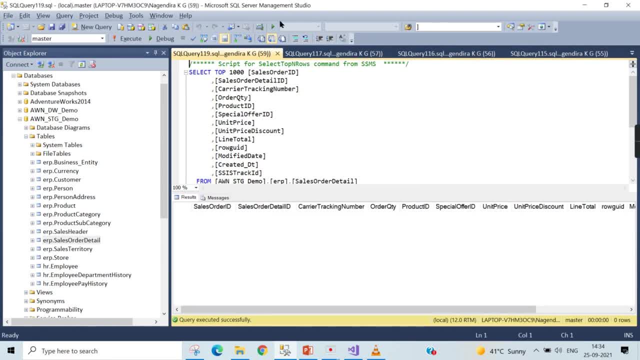 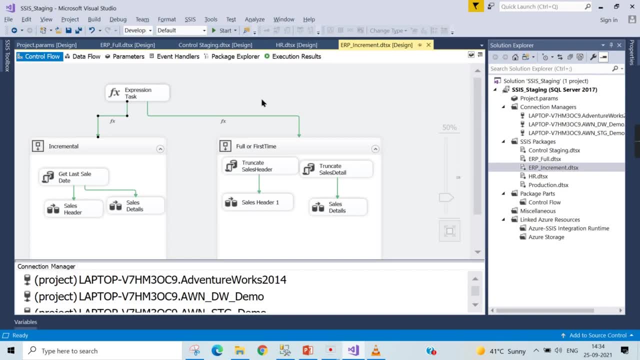 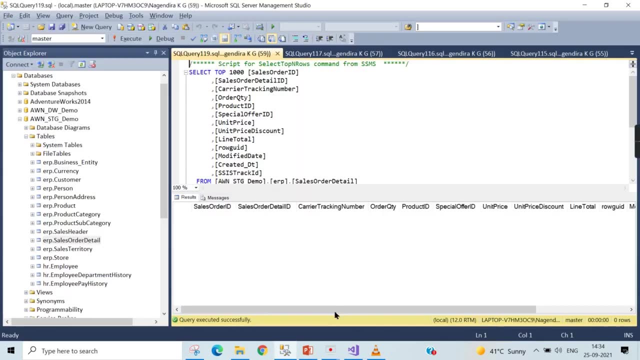 this is what. uh, you will load your from your source data into target data here. i didn't run the incremental load yet. this is the first time load. ok, I will once I populate the fact table. then I will come to this incremental load concept next. now let's go back to our presentation and put this: 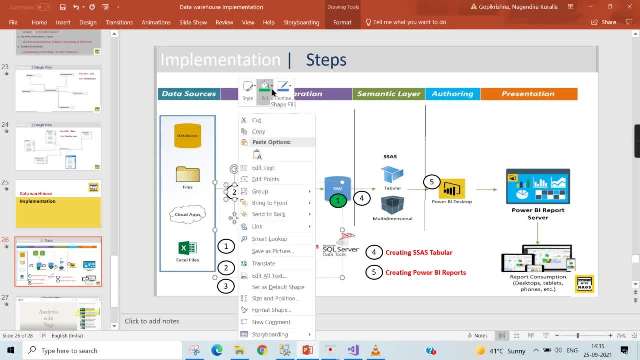 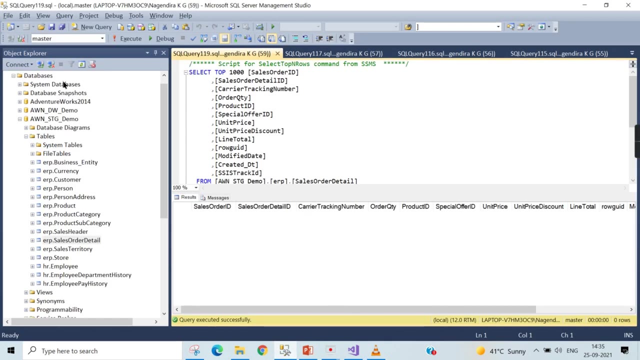 as green. ok, now we have brought whatever columns ok in the source and then we have brought into staging here. now we will move on to the third part, from the staging to data arrows. ok, now you can see here we have already designed the some dimensions and fact in the data arrows using the create table scripts. 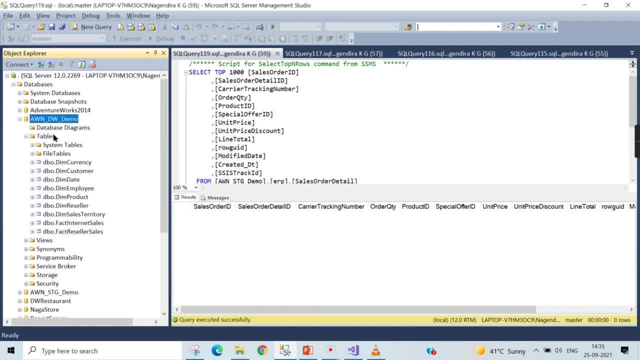 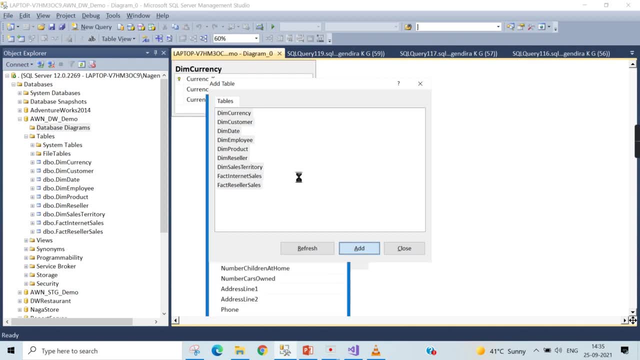 correct. so once we draw it in a diagram then you will look. it will look like a typical star schema. this is for you to understand how we have designed right now. ok, this is one of the sales data mart for HR data mart. we will take it later now. 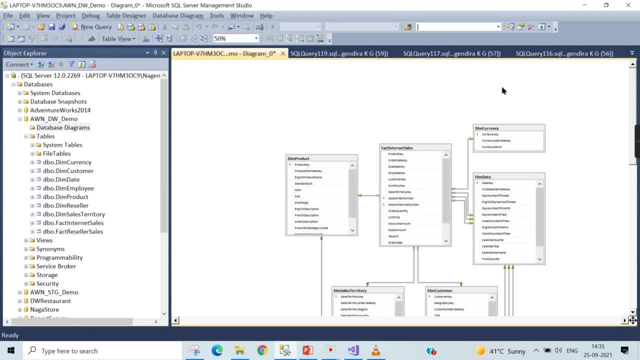 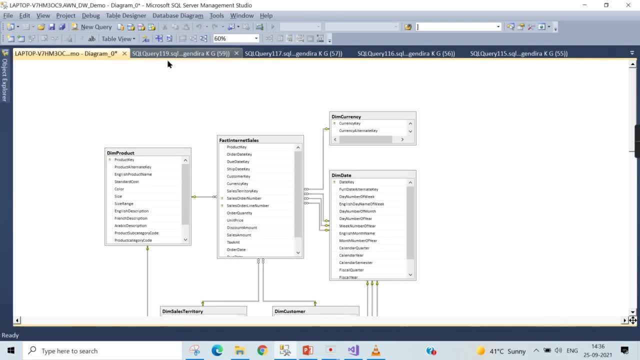 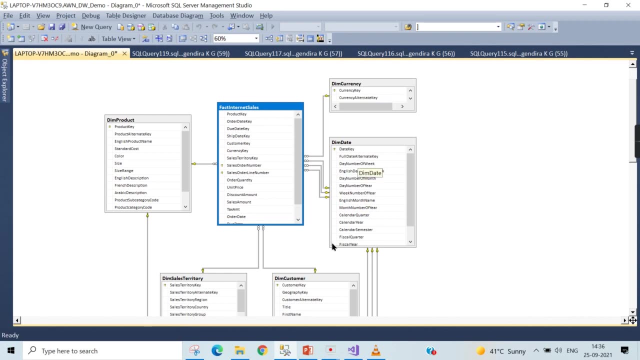 you can see here from this diagram. ok, let me select all. I think. I can choose name only. I think it's not puzzle, that's ok. fine, now you can see. this is the fact: table surrounded by five dimension table, currency, dim date. again you have a reseller. that is also. 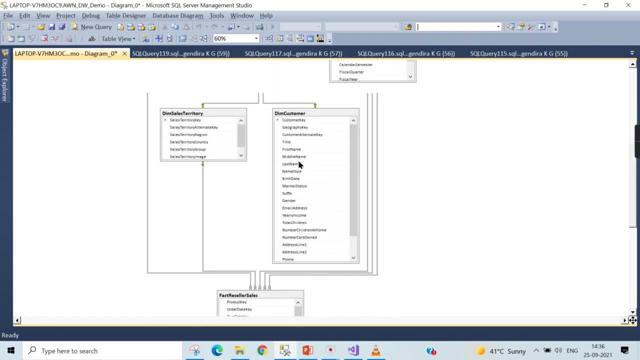 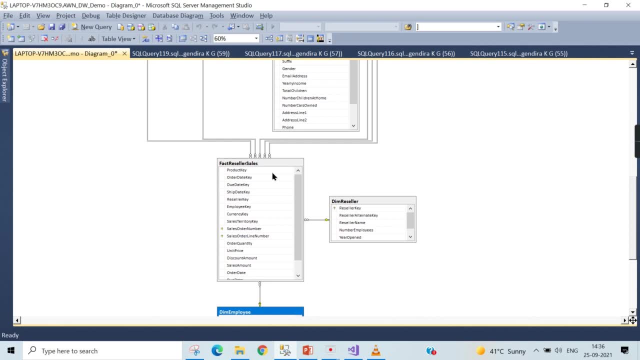 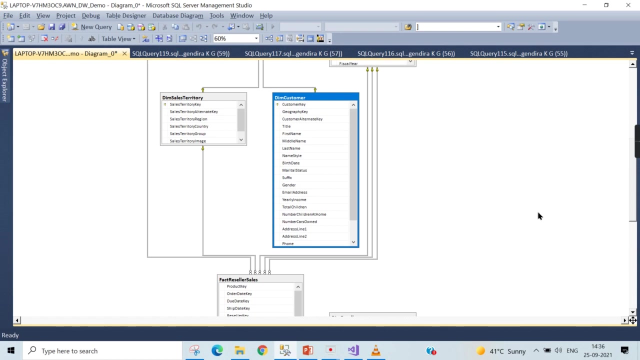 essent mainly to the territory. ok, these are the fact tables surrounded by dimension table, employee, reseller, then it is date, then the territory. ok, these are the two fact tables, then, surrounded by different dimension. and customers belong only to internet sales and reseller is related only to the fact. so 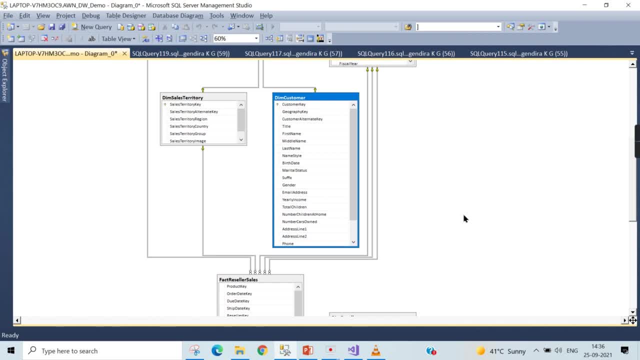 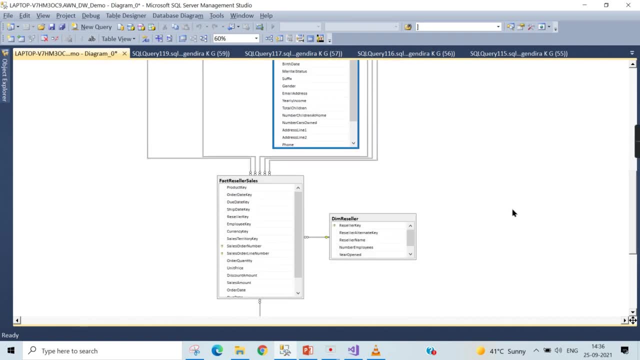 this is what you need to understand. lot of people ask me how many fact tables, my, your different fact tables and dimension tables surrounded it. okay, so this is how it will look like. this is the sales data mark contains two fact table: one is internet sales and the reseller sales. to make you to understand, I have explained. 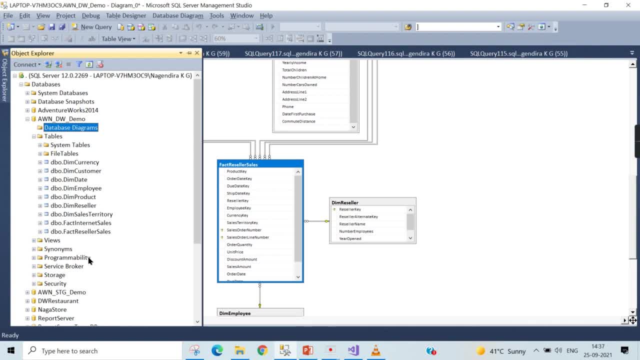 this. now we need to populate these tables. that is the ultimate aim of our data warehouse implementation. we will go one by one, so which one to start first? typically, we need to populate the dimensions first. correct, because the fact table contains the foreign key reference. right, so your primary key. 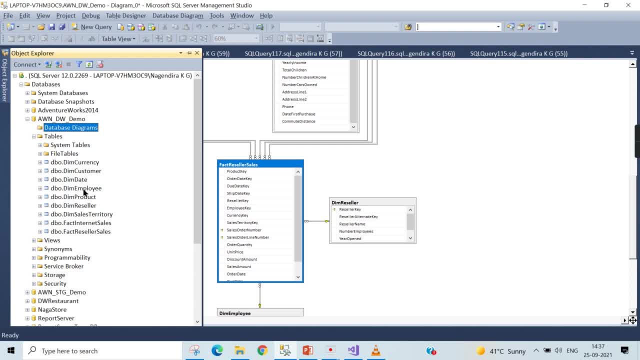 should be created first. so it is a thumb rule. like you need to populate the dimension first, then followed by your fact tables. so we will go one by one population. so let us. I will explain you one or two tables, then I will execute the script and it will be easy to understand now how a dimension can be populated from. 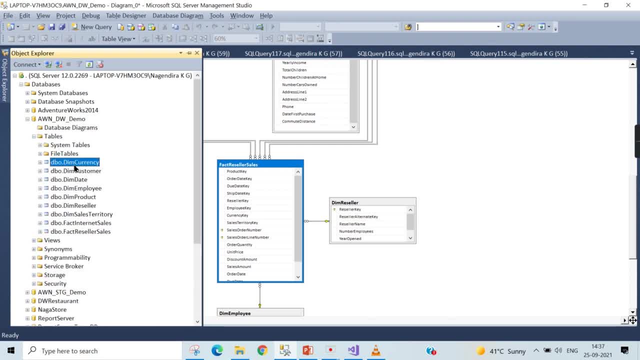 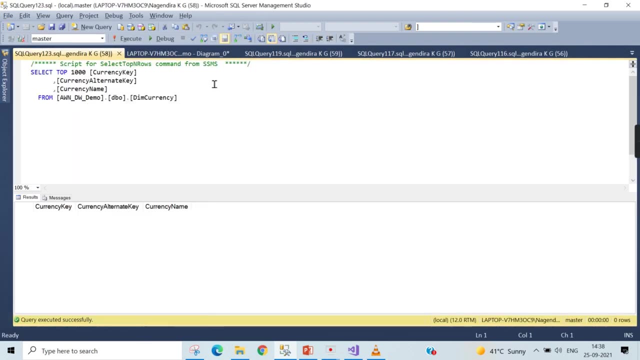 the source table. so one I will explain about dim currency, another about dim product. let us see the structure of this dim currency. so dim currency contains alternative key currency name. let us try to create. it does not have any data since it is having only the structure we created in the data warehouse. so currency. 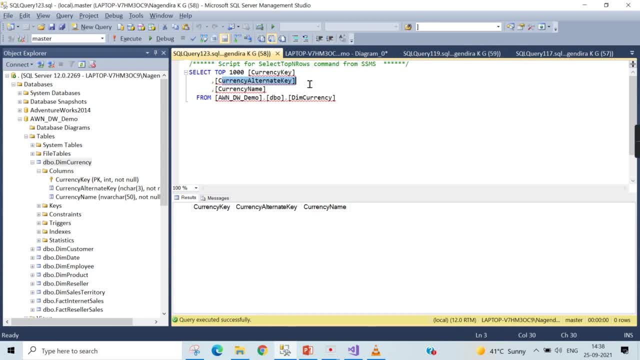 alternative key is basically the business key: that transaction is happened and other things are. descriptions is very simple and this is what we created as a surrogate key, that is identity, one of one. so how you can populate it: ok, from the source. so in the source we have ERP dot currency, so this is pretty straightforward, simple. 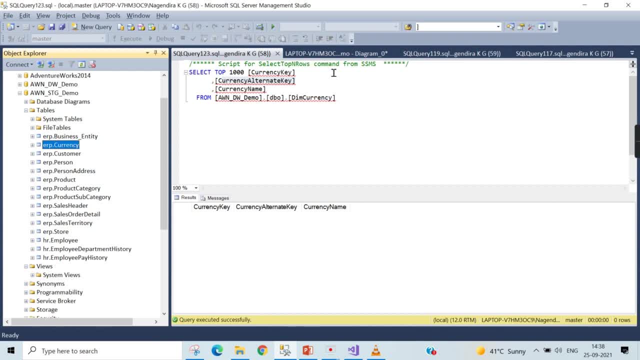 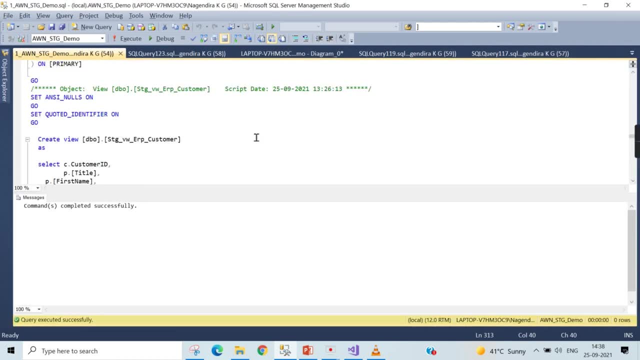 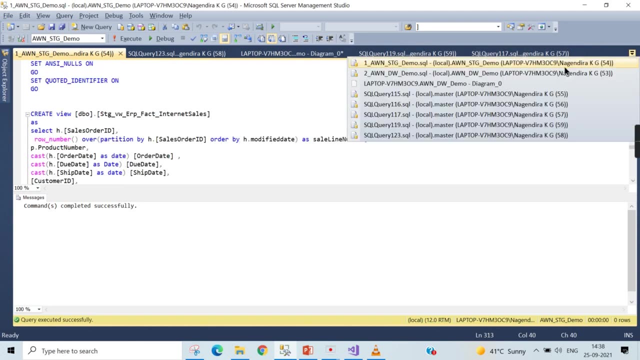 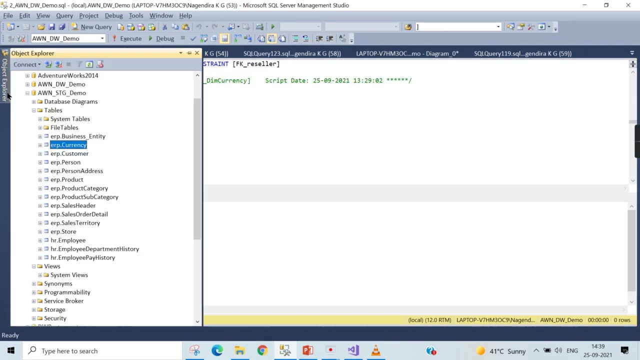 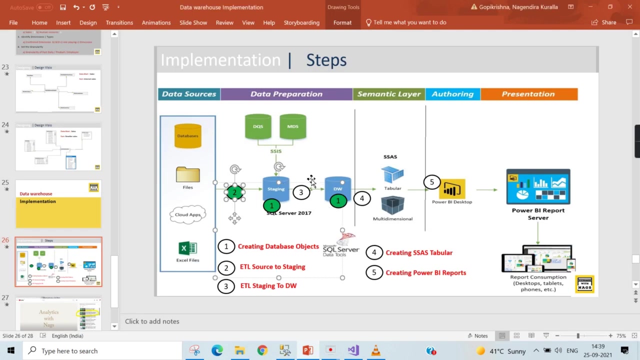 dimension and we have some script for it. ok, let us go to our awn stage in demo and we have no views for it. then I can go to this DW demo. so for each dimension population, you either from the staging to data, or all right from the staging to data, or either you can use a size package. 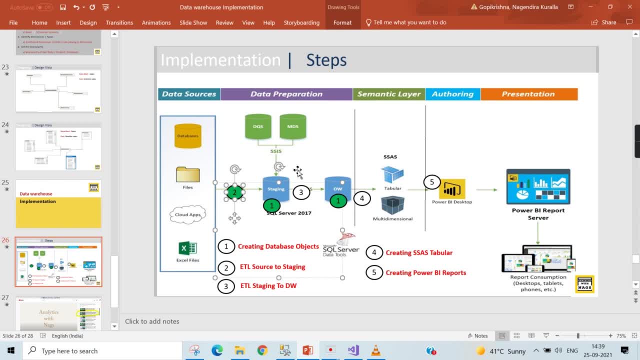 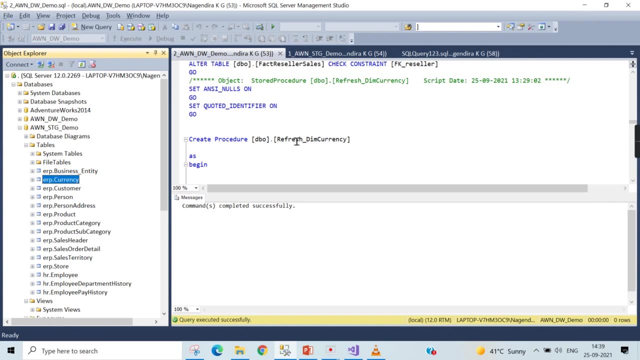 are right. 1 procedure: okay, that is very simple because most of them familiar with SQL. write a procedure that will populate data from staging to data varus. then call that procedure in the SSIS package. okay, that is what we are going to do here. so this procedure is written in the awn data varus demo. 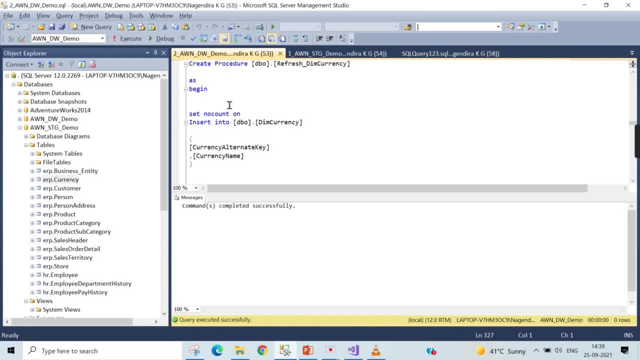 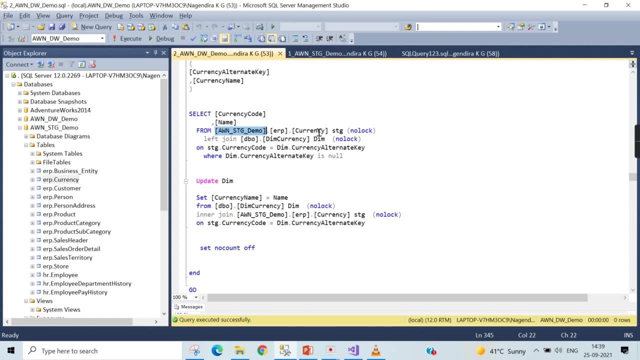 okay, I am back to the script. so what is the script? let us walk through together now. insert into dim currency currency alternative key currency name. then select from awn staging demo: okay, from the staging database. okay, the currency table should be fetched and leave join of dim. 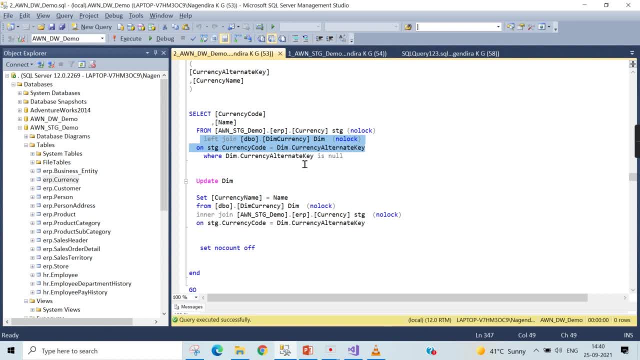 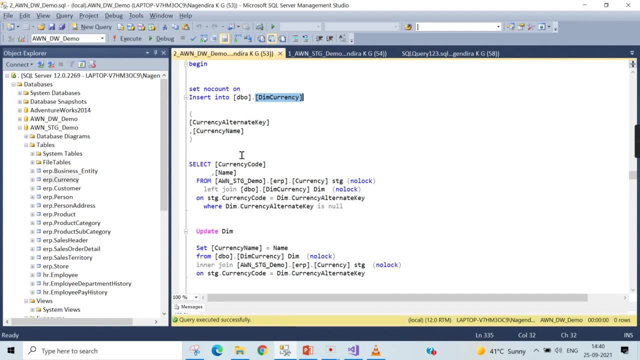 currency with the business codes. if the dim currency code is null, what it means nothing this contains. if it is like inserting a data, okay, assume you have five currencies initially in your business. you loaded it. then next time, this in this source, right in the staging table, from this source it comes to staging contains seven currencies. okay, initially five. then you 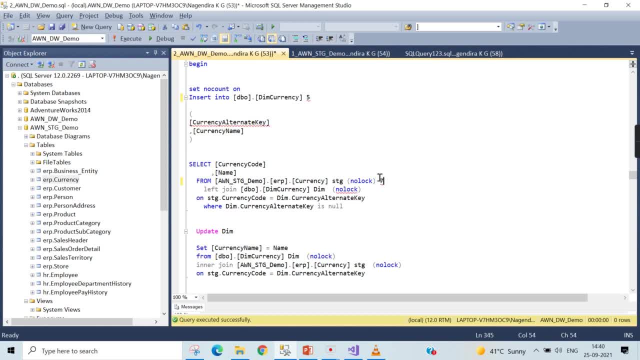 got seven currencies here. now you need to load only remaining two currencies here. that is what this will do. so lift, join will have seven. okay, left table will contain the seven and this dim currency will contain the seven current. so if you do the first two, the first term, which is: 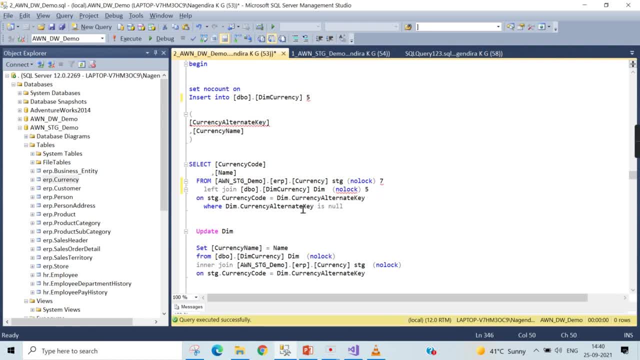 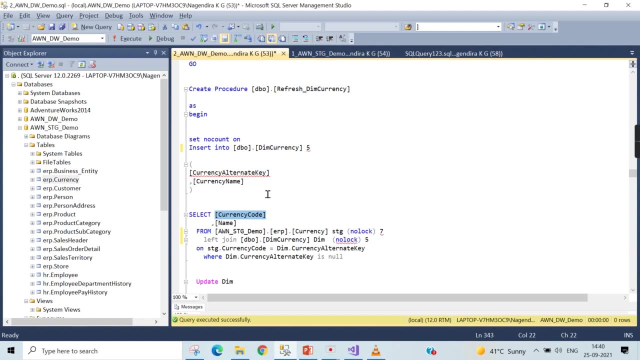 five, then you are joining with both the currency code. then remaining remaining two will have null values in the dimension. so this is the typical way of loading the dimension table. okay, so once you load the business key and its description. okay, that is enough. then you will do the update. 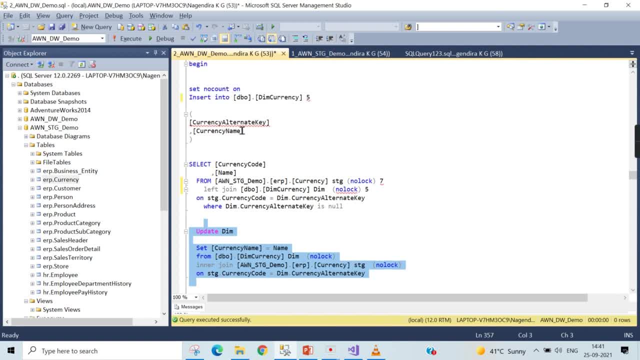 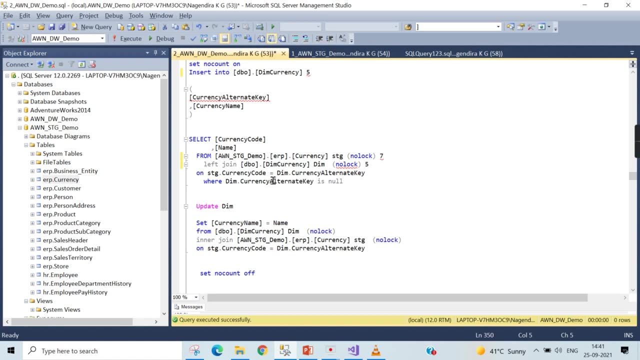 okay, update means if there is any property changes for the currency, then you will do the update. so this is first few lines of code is for inserting the dimension. next code is to update your dimension. update the dimension description. your business key won't change. you will join with. 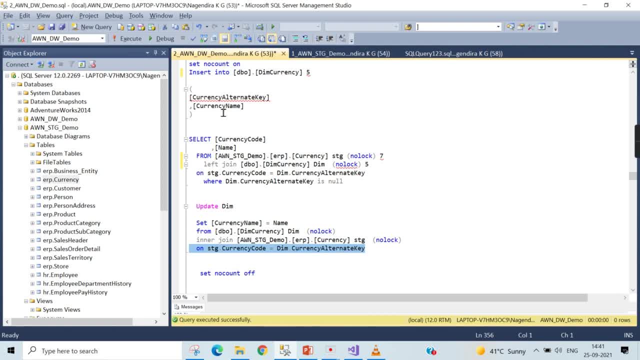 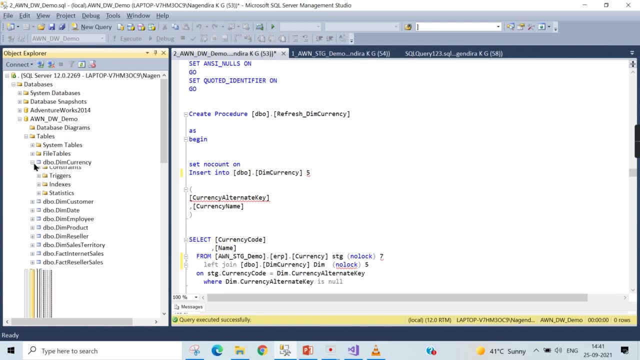 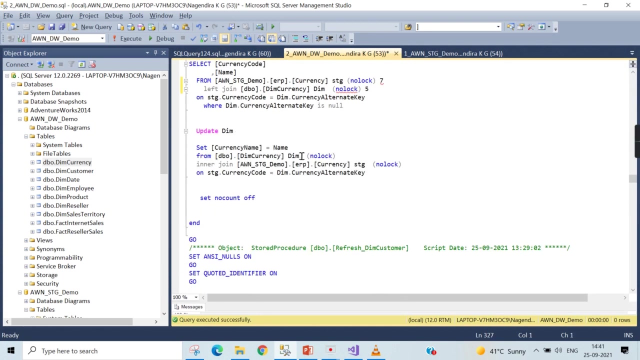 the business key, currency code, alternative key. any other related descriptions will change. okay, this is what. so you will generate the surrogate key here. i mean in the data warehouse. okay, now you see there is no data in the currency table. okay, in the data warehouse. now, what i'm going to do? i will create. 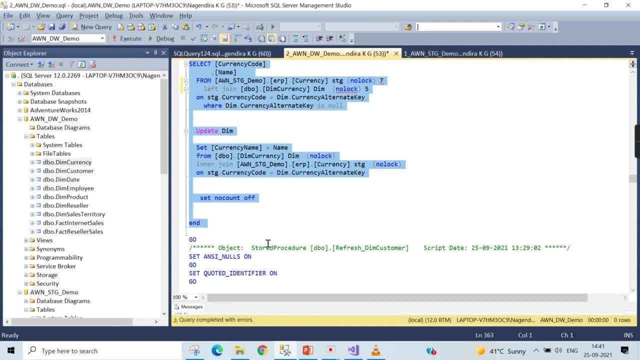 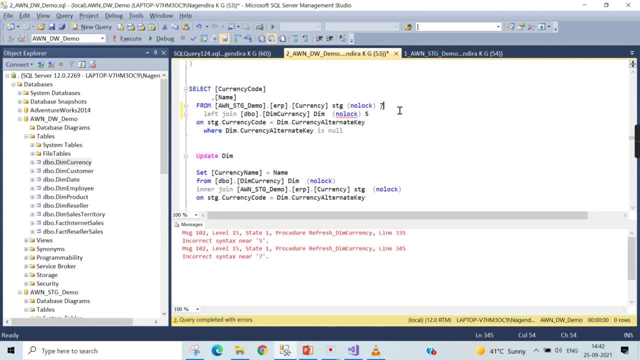 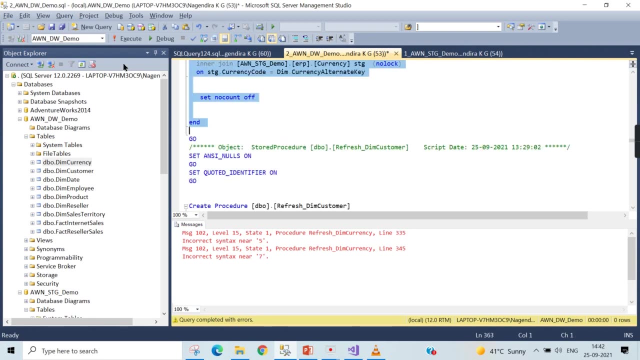 this procedure. okay, it's done. it says some error. let's see what was it. okay, i have written five, six, seven over there. that is why. so do not mess with your scripts. that's fine. now it is completed. now, procedure is completed. that it will again create this structure in the database, like in here. 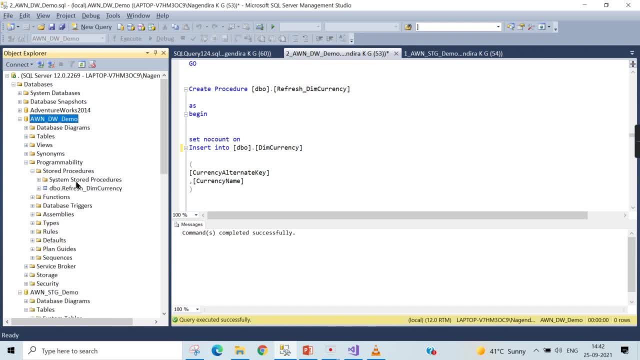 those who are not so familiar with database you, i'm just showing them. now. you see, one procedure is created, that is logic, is written and it is stored here. now how the data will come. now the data will come here. no, still it will not come because you need to execute it. so i just selected. 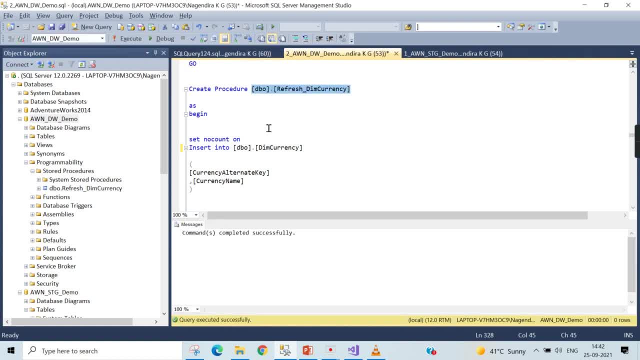 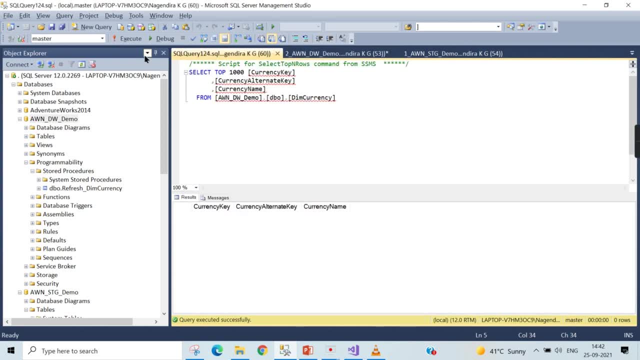 it and executed. this is manual. i am doing it manually in real world. you can do it manually. will call it in a procedure. i will show it to you next. now i executed it. okay, now you go here and check your data. now the data has came in your data arrows from your source to staging. we have used. 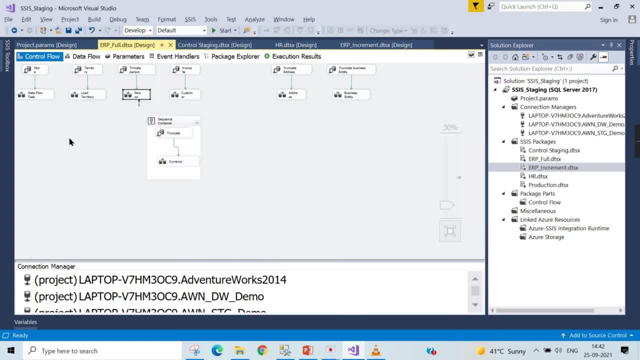 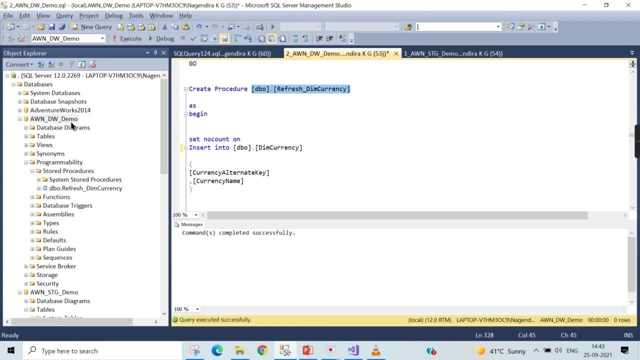 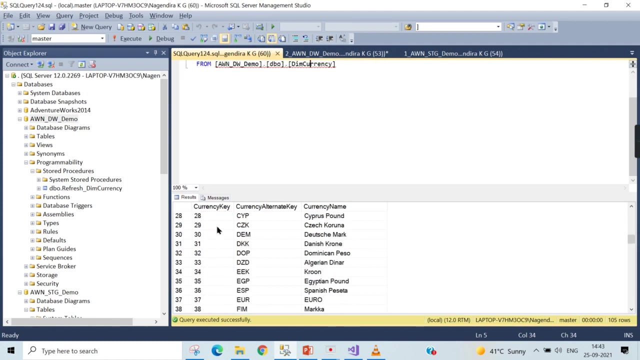 ssis, right in ssis, we have brought this currency data. then from staging to data warehouse, we have written one procedure. okay, that procedure will populate the dimension table. okay, now we are done with dimension, because it is identity column. you have generated the currency key here. this is step number one. let us walk through through another. 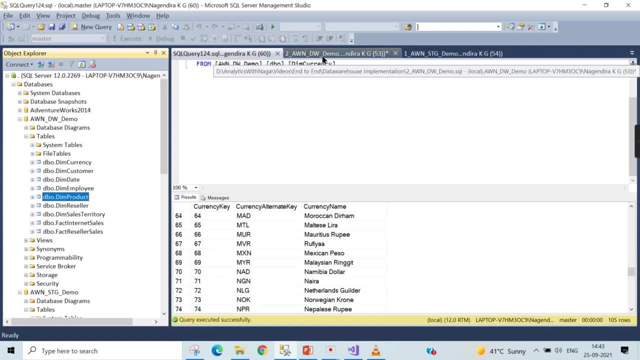 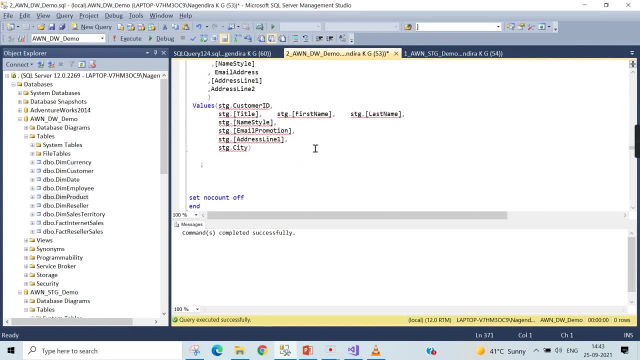 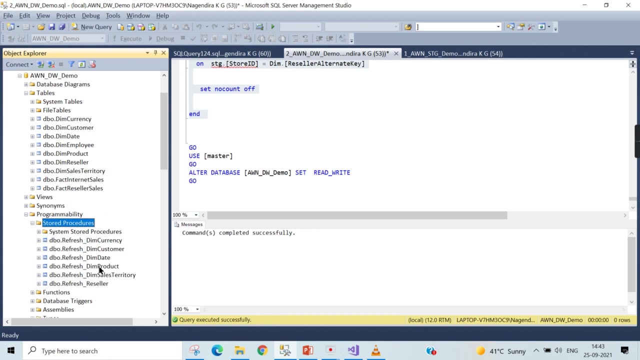 table, dim, product, similarly how we will populate. so for this, let me create other dimension tables quickly. okay, then we will walk through some other. i mean to say like product dimension. so similarly for each dimension. okay, i have created one procedure. i'm not going through all, i'm just sharing the script. you can go through it. 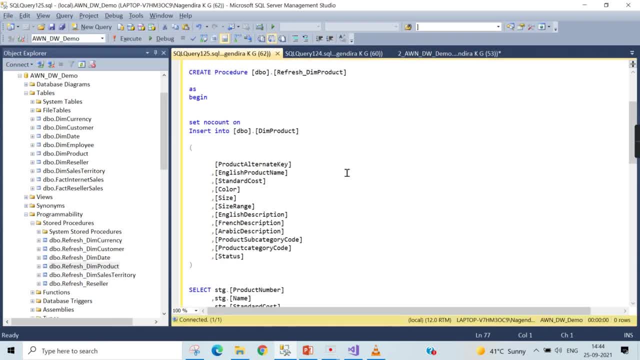 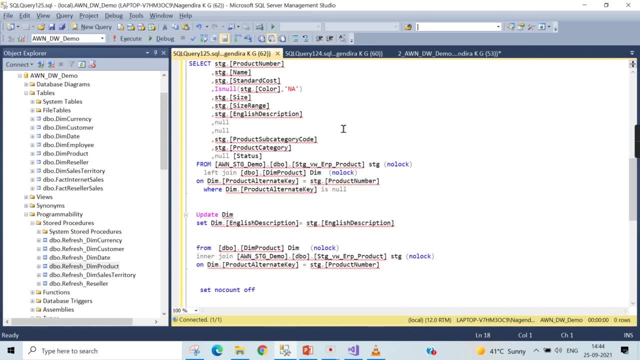 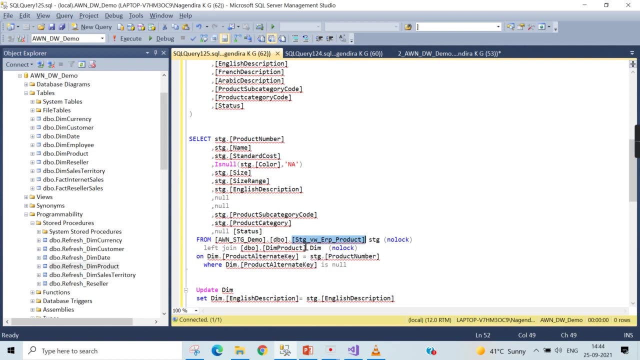 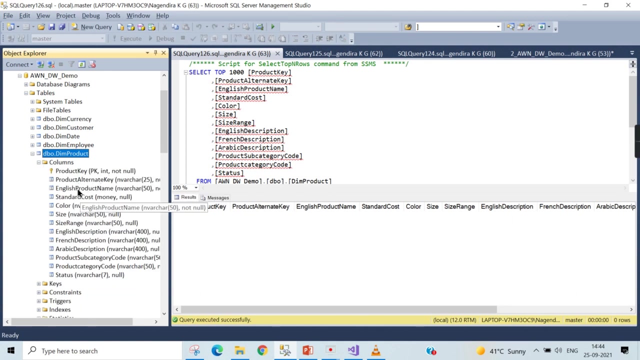 so now let me focus on the dim product, so that refresh dim product, this particular dimension, why? most of the things i will try to cover instead of directly picking it from the product table, from the source right, i have written a view for the product. why? because you see here in this product what are the columns present, all the attributes here. 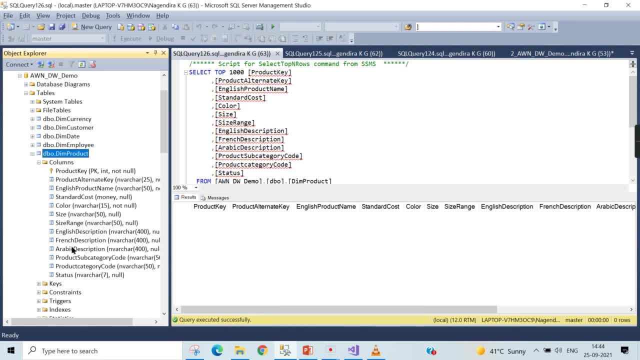 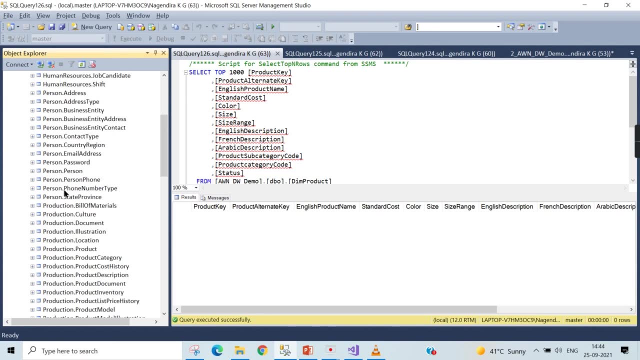 product name, cost, color, size, size, range. everything is fine with the description. i mean related to the product. then you have a product subcategory and category this information in the source system. okay, i will go to the source system. it is not available in the same table you can see here: 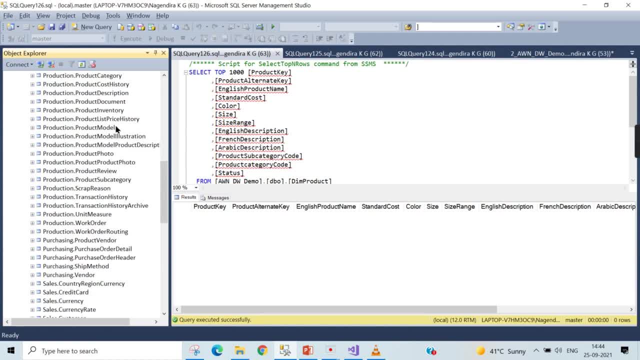 sales. where is that product? i think in production. let me check it out. so here you can see: production dot product category, then production dot product subcategory and production dot product. these are available in three different tables, so you need to join these tables- three tables- and bring it in a. 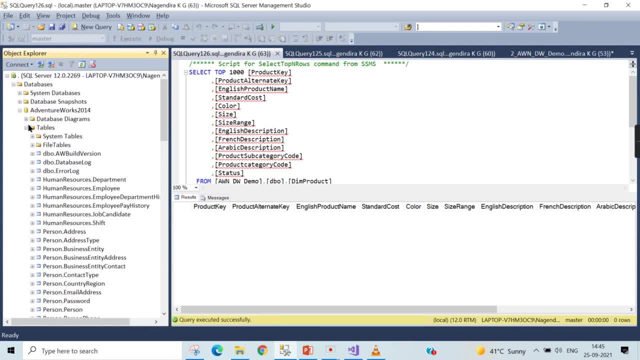 single table. so this exercise, either, you can do it in the source system. most of the time what happens source system will not allow you to create any objects on the system for this reporting purpose. okay, if they allow, then it is better you bring it there. so that is why we need to bring those. 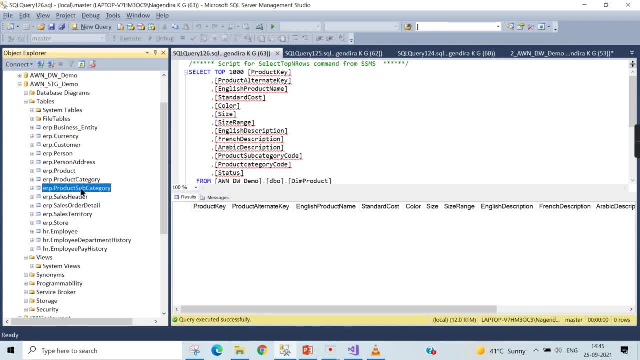 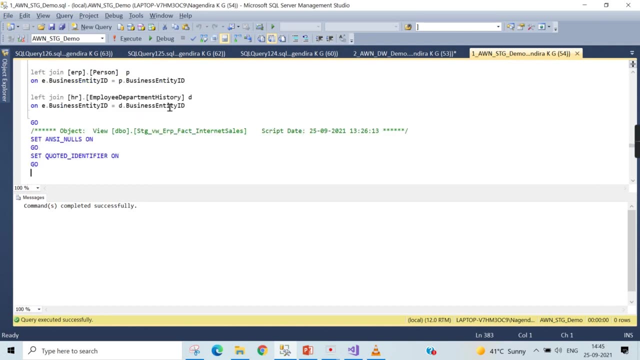 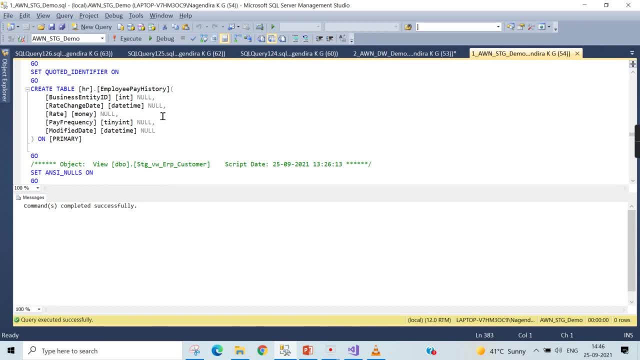 you no need to worry while you are practicing. just you can execute the script in a single shot, so all the objects and views will be created. i am going to understand, so here let's see any views has been created earlier? no, I think no, so let us run this staging views. so I hope it's fine, perfect, so now. 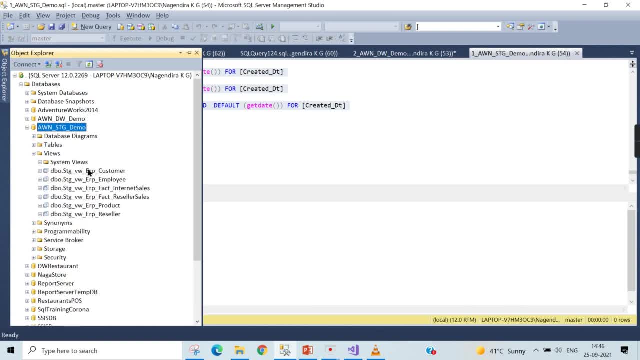 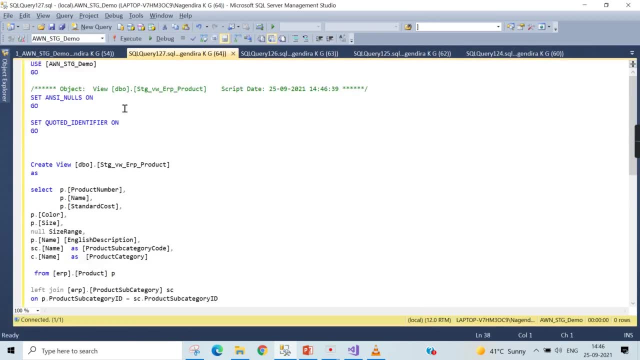 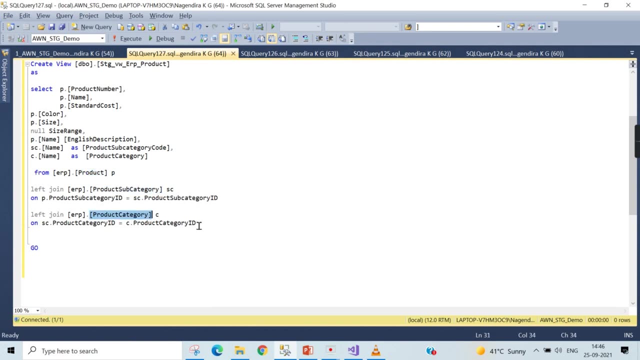 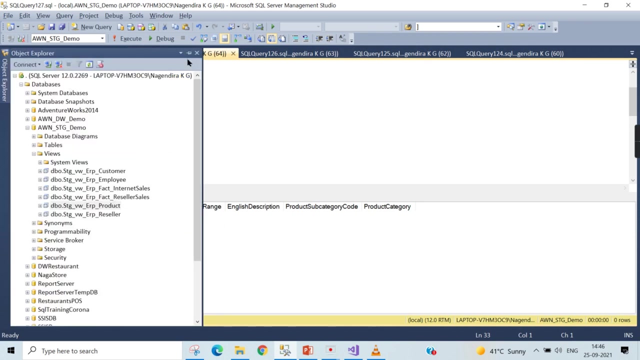 let me refresh this database. you go and see here now you can see I have written that view for product. you can see here from the product: product category, product subcategory. I mean product subcategory and category. I have joined and brought the respective columns. when you query this one, I'm not sure the data. 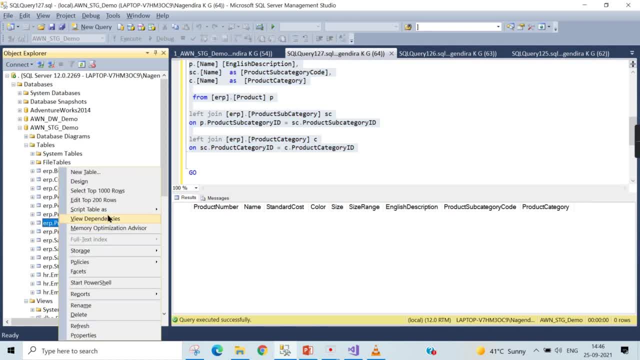 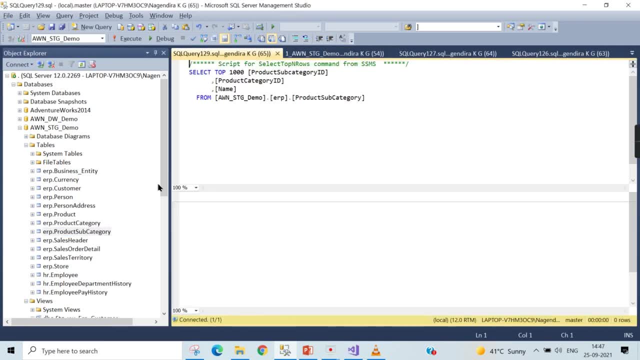 is not coming, let me check what happened. I hope data is not available here, so let me go ahead and run it and see if I can see any views has been created here. so let me go ahead and run it and see if I can see any views has been created. 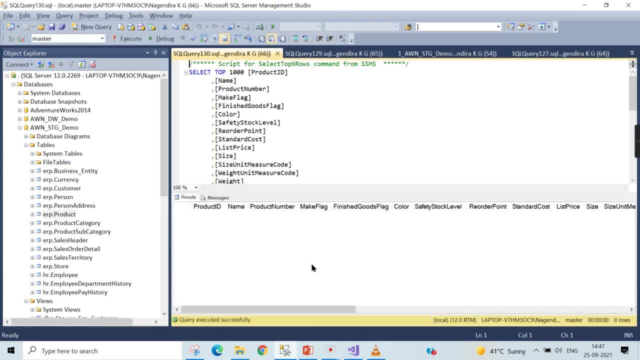 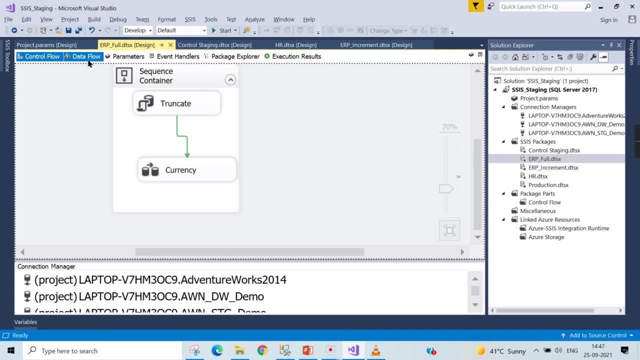 in this tables? not sure, so let us run. I hope I have run this package right. so whether the product? okay, see, this is ERP, for my understanding, for people's understanding. what I did is like I have made this product related tables in the production source, baby you. as I said before, ERP is one source, HR is one source, production is. 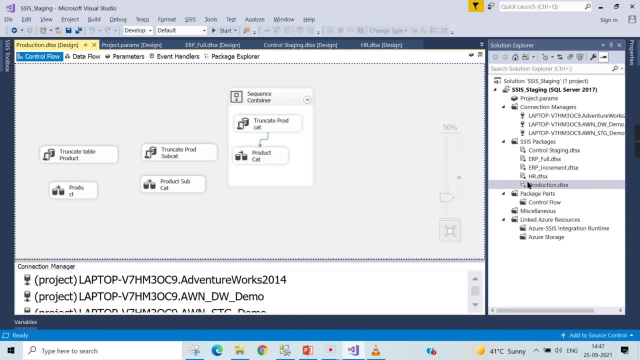 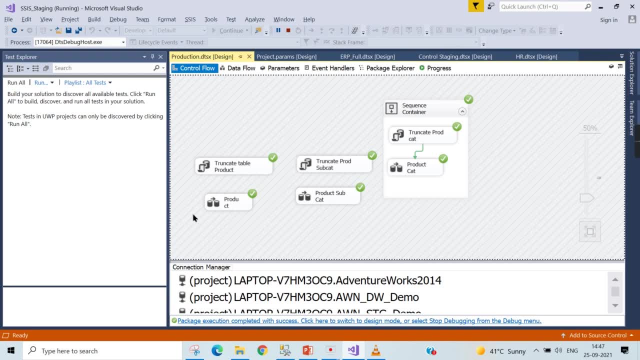 another source to make you to understand. I made it here, so that is why there is no data. so it is always some confusion. you need to understand what is happening, then it is easy to understand. so now I have run it. now I will go back to this. 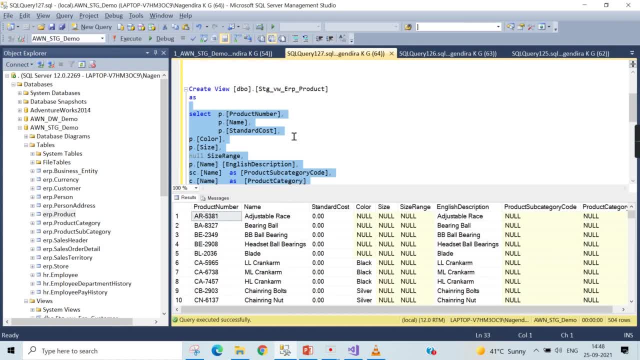 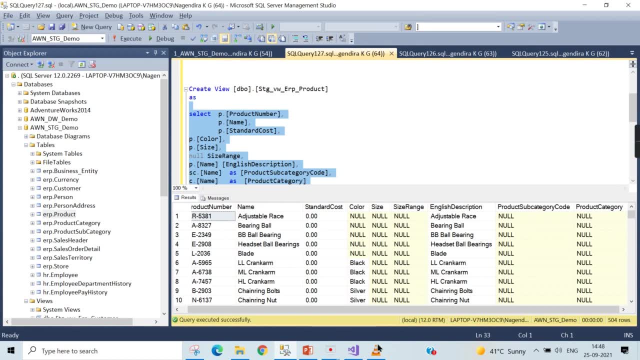 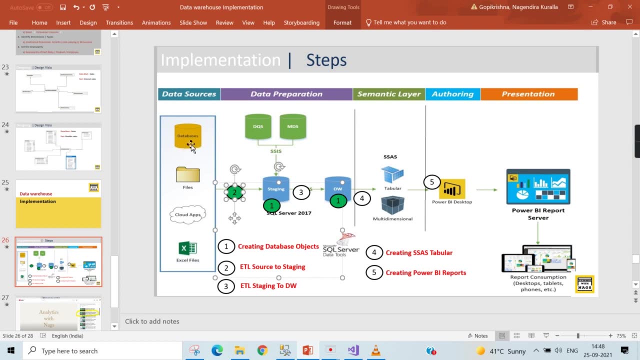 script, that view I have written to make it fit into the dimension table. okay, so what is the purpose of this view was? the first step is let me revamp someone who has confused here. so all the table? there are two to three tables you need to match. 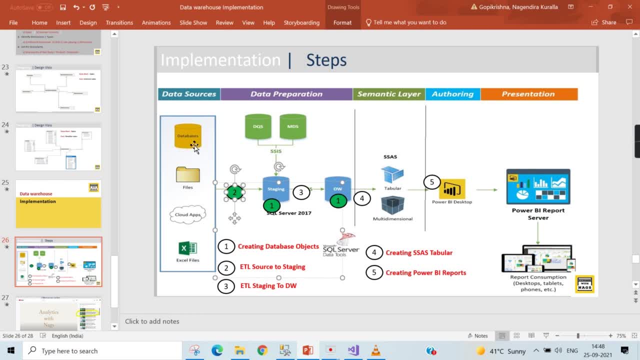 or join to populate into dimension. so if there is any provision to filter out of, we create a view in source, you can read, write it. otherwise you bring those tables here and create a view to join those tables, then write. I mean, then you populate it here, that's it. 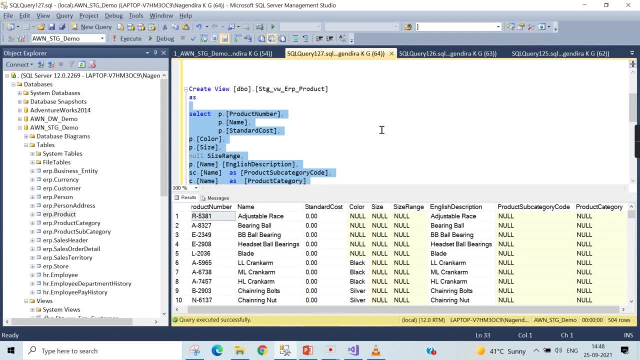 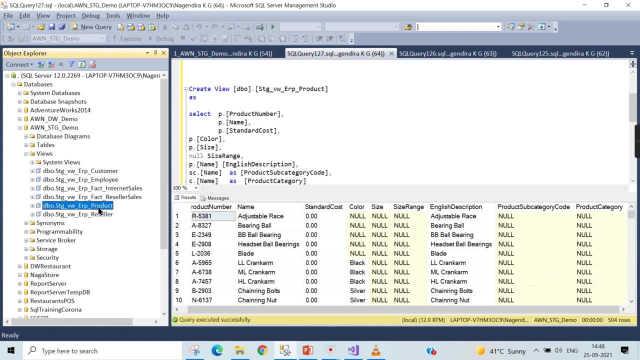 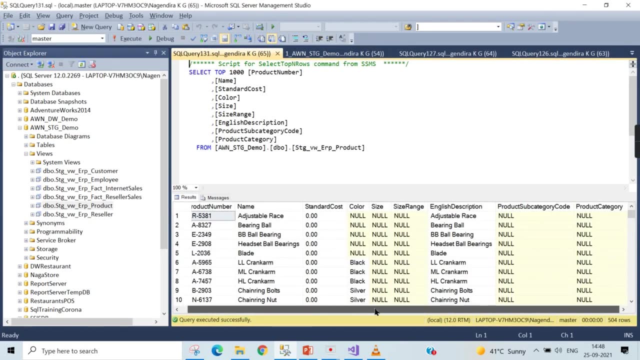 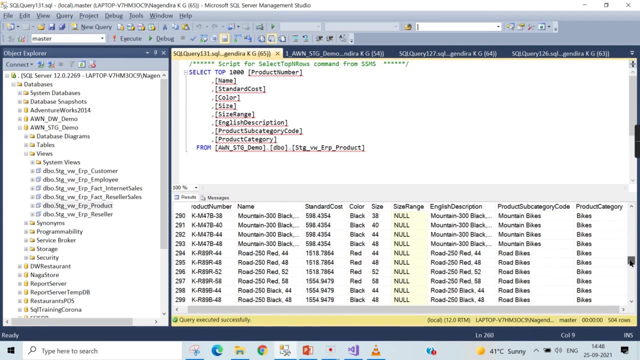 that is what I'm saying. so now we have created this view already. okay, now you can see here: the view has been already created. now, once you create- now, once you create, you will get the respective data, you will get the categories of category. there are some products that doesn't have sub category and category also. okay, 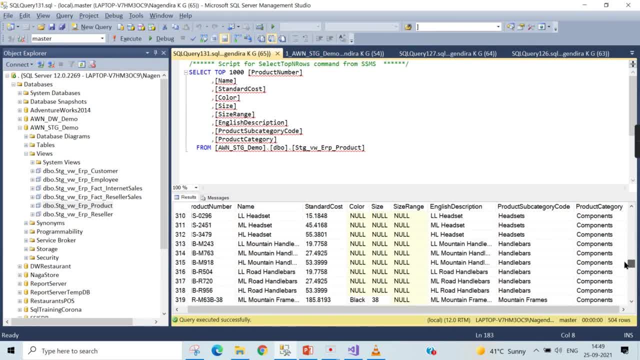 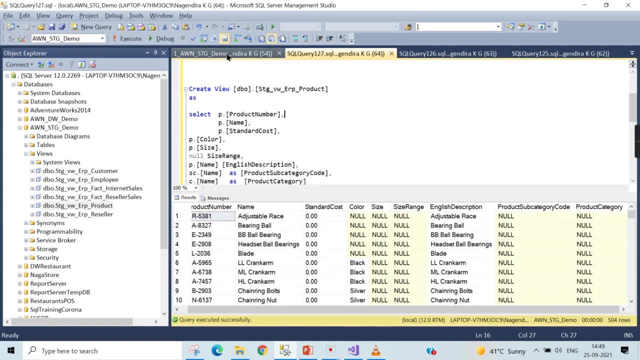 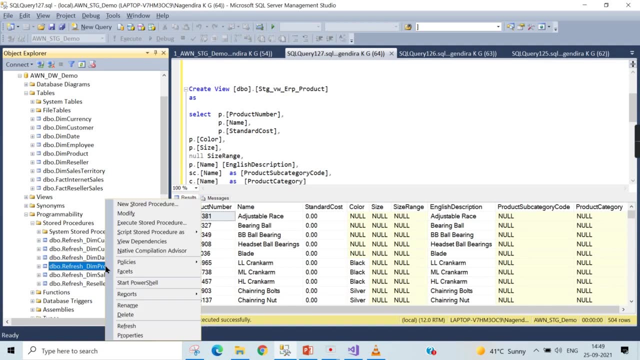 that we will take it later. that is not part of the discussion today, but you can see how we have brought the product and product sub category category to align with the dimension. let us move back to the dimension query and we'll go to the ding product stored procedure once again. now here is the catch. again, it is the. 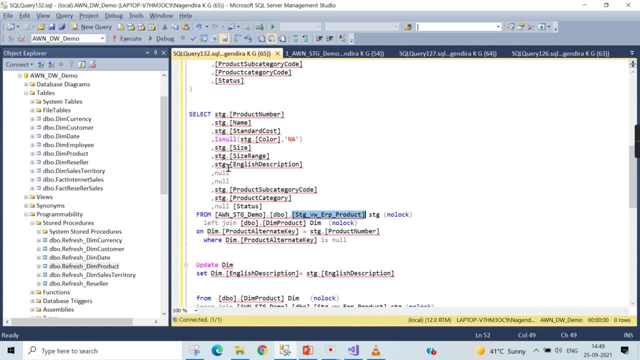 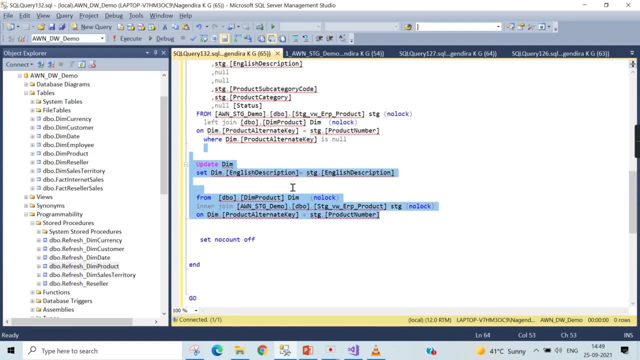 same kind of logic where you can see I have used a denoted field, so data field, denoted field is my product and I have the stage okay left, join using the alternative key, then product alternative key is null, that is from the dimension is null, so you will insert it, then you will update it. so this update, it is not only. 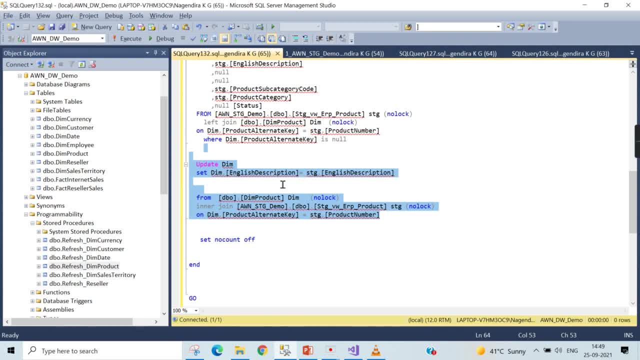 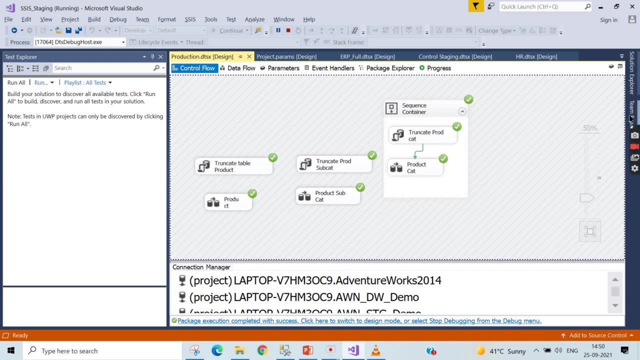 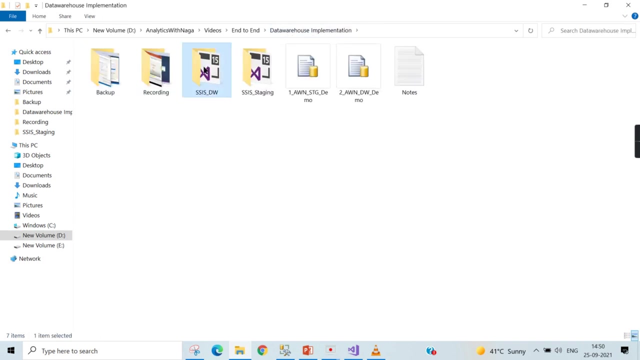 one column, whatever columns you feel it will change. this is typically scd1 change that you need to put it over here. so this is how i will populate the dimensions now to make you to understand. uh, i have created the ssis package for all this procedures calling, so now you have. 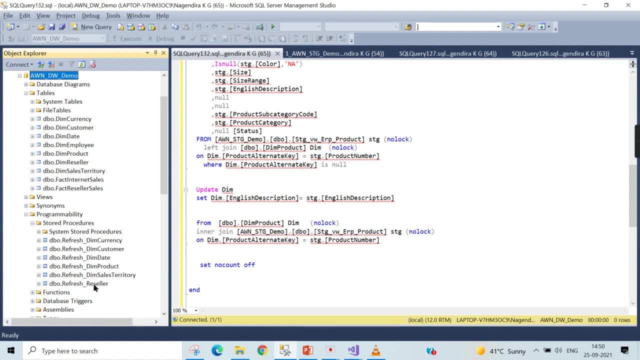 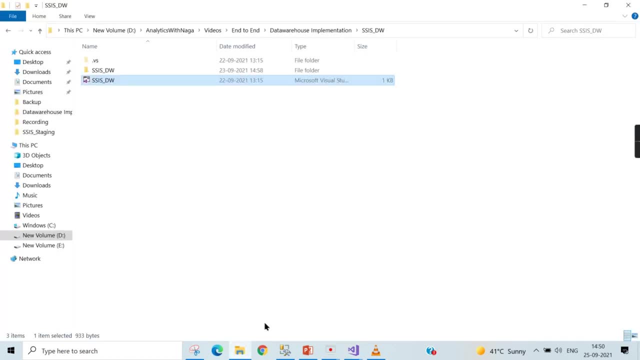 this data barrows, tables and procedures that will refresh from the staging to your data warehouse tables. right procedure is there? how you will call it? you will call it in a ssis, so i have a separate solution. like over here, there are two solutions, you see, data browsing. 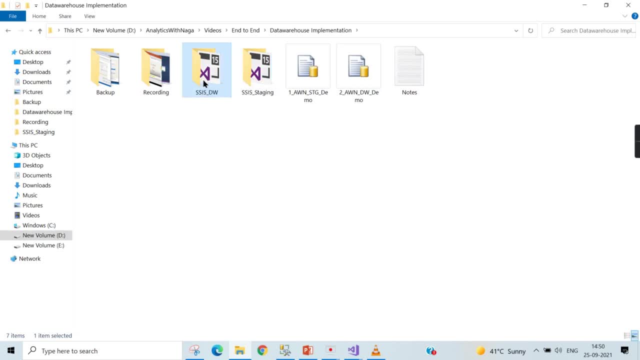 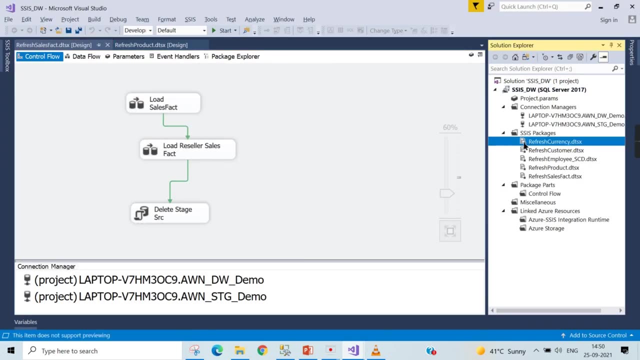 implementation: ssis one project and ssis data was another project. this is ssis, so i have opened ssis data arrows here. so for each dimension population, i have called the procedure. you can see customer, you can see cd product, the product sales fact, everything right. so now we will run one by one. 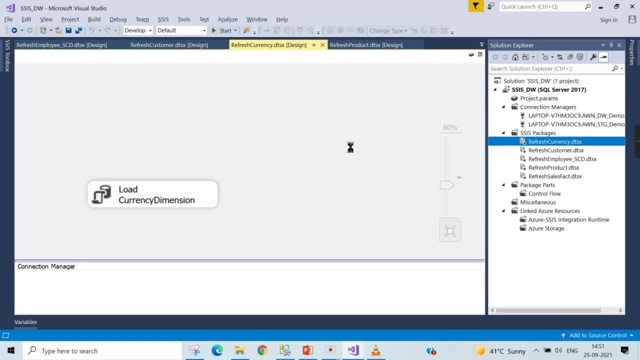 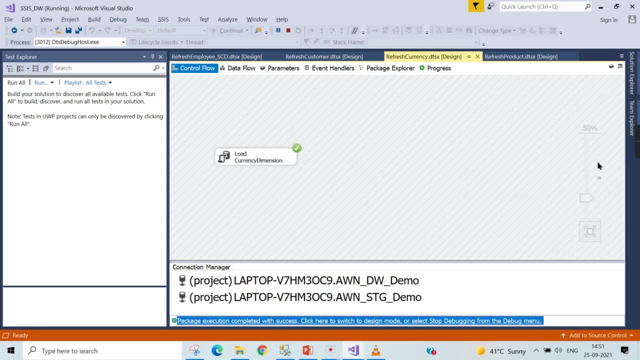 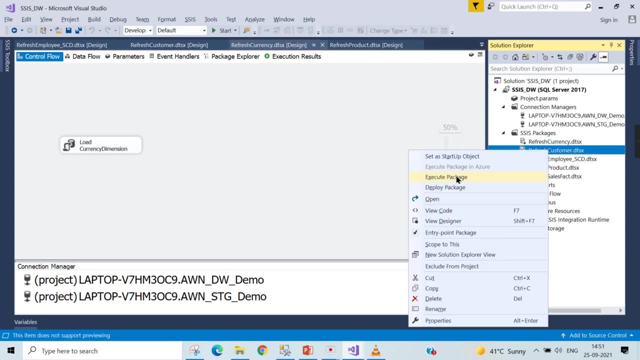 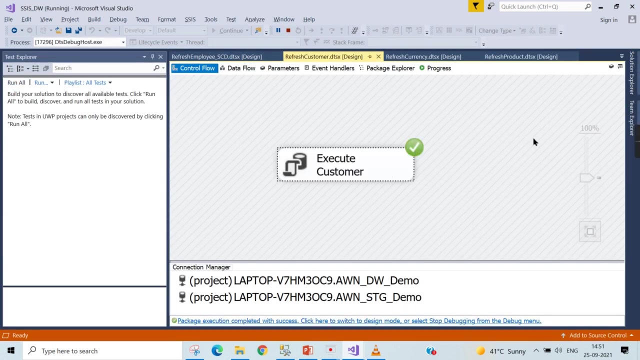 then we will check it out how the data has populated here or not. so currency: we already run it. so that is fine. and you have customer, let's run again. okay, and you have, i will going to cover employee scd2. that is why i have not run that one and 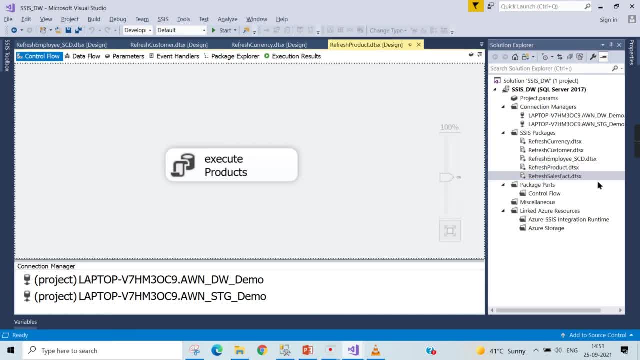 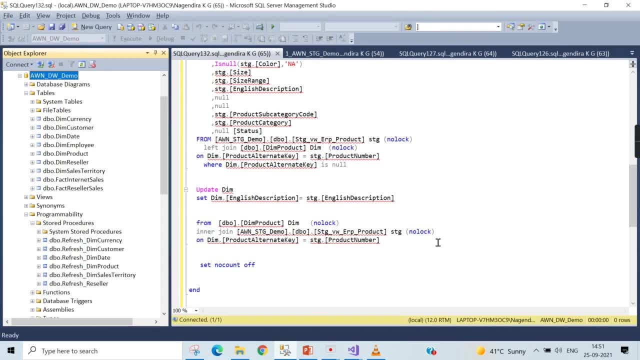 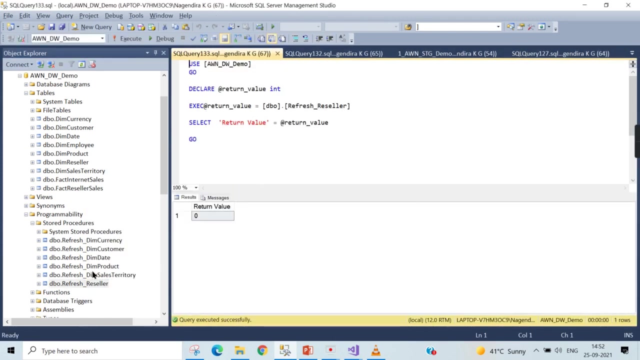 refresh sales fact. i will cover it later now. we have loaded currency, currently customer product and then employee will come to that. before that, i will load this reseller as well as dim product. i didn't had a package to execute this reseller, so let me run it over here for you. 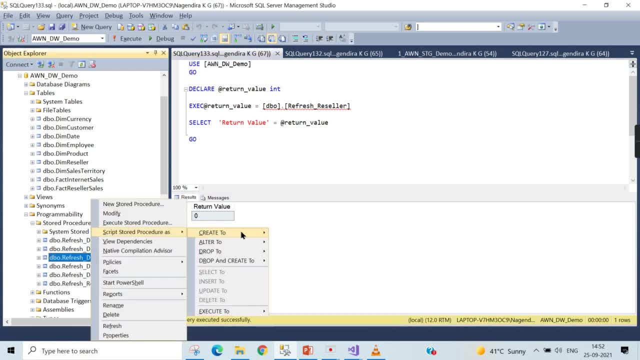 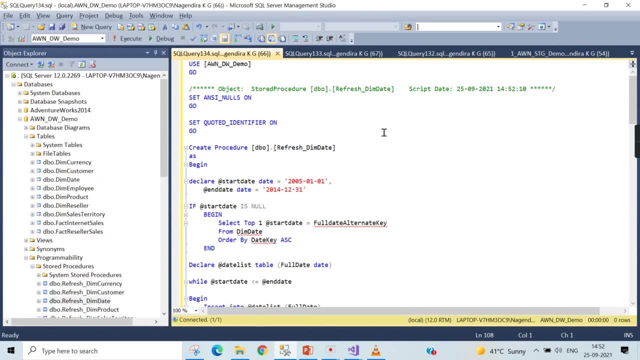 to understand. i have done that. then, for dim date creation, this script also i will provide. so there is no source data available for dim date. so what i will do? i need to generate that dim date. so this is the procedure to do that. so refresh dim date. i will quickly show you to you. there is no time for. 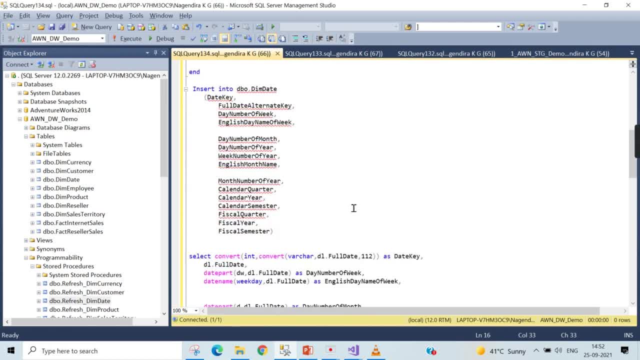 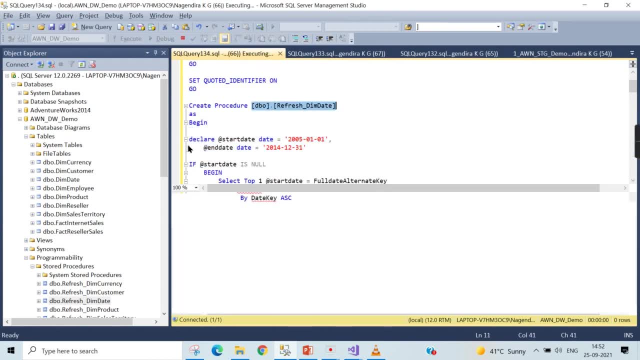 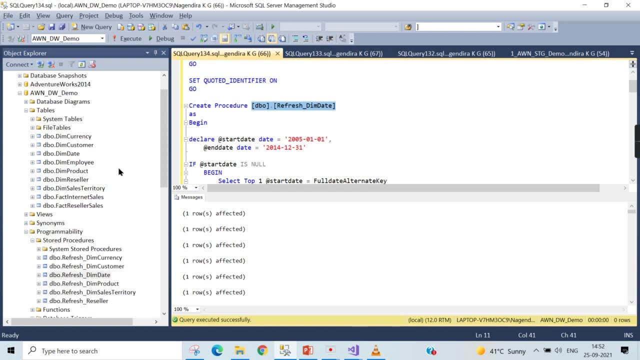 us to explain it detail. so start date and end date, then this script will populate the dim date table. okay, so just, i am going to execute this. so, basically, once you create the tables, you have this stored table procedures, then you will execute one by one. now, once you executed it, now you go and check all the 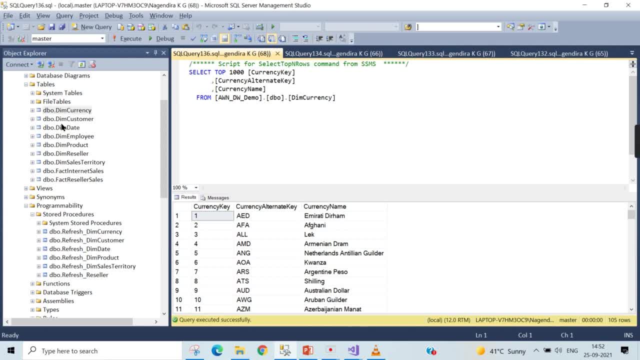 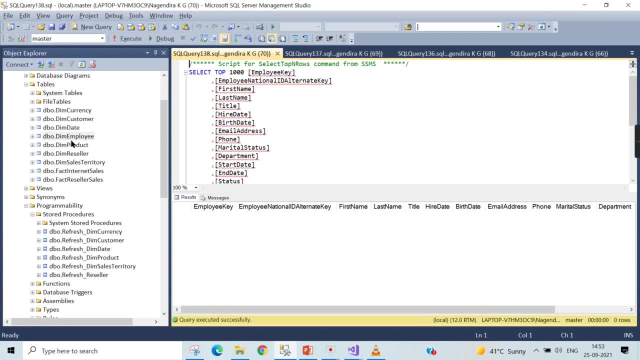 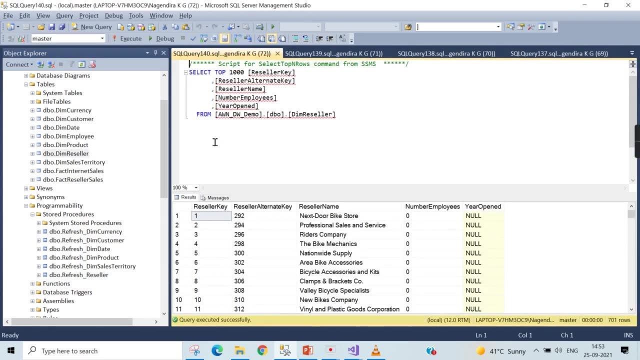 tables, the dim tables. you will get to know all the tables, having the data one. if you do not have either, you need to run the packages here or the respective procedures you need to call the employee belongs to scd2. i will explain it in a minute. 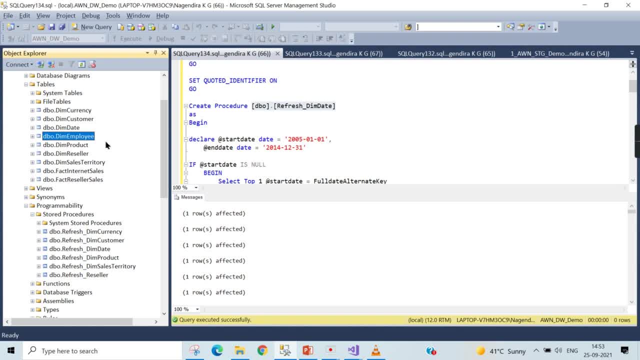 now, except dim employee, we have populated all the dimensions. as we said, we need to populate the dimension first, then we need to go for a fact now: to populate dim employee. this is basically employee is designed as scd2. i will take a moment to explain what is scd2, how to handle it then. 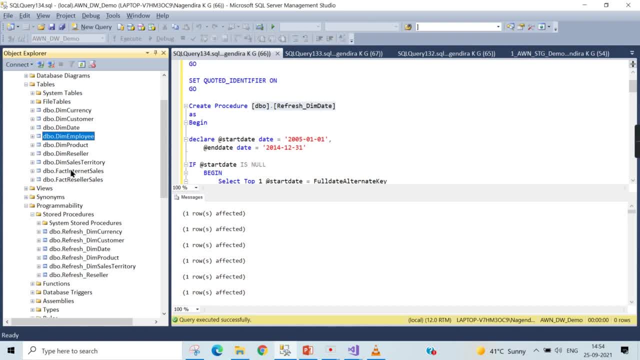 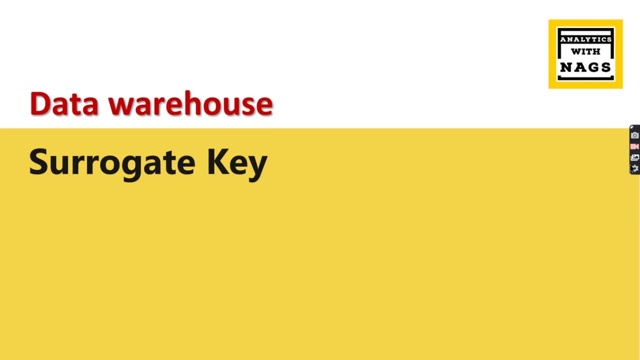 we will populate this employee. once we are done, we will move on to populating the fact tables. so now we have seen how to populate the dimensions first, and while populating, we have came across the surrogate key identity column in the dimension. we need to know this importance. that is where 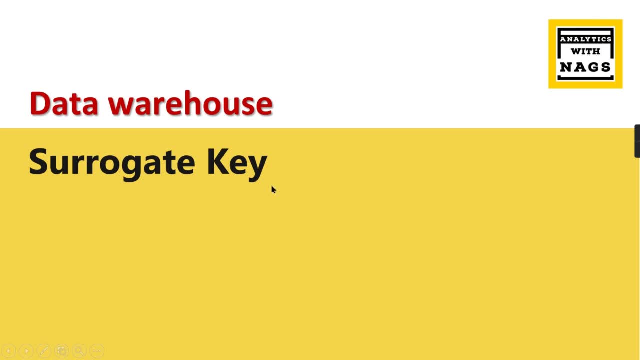 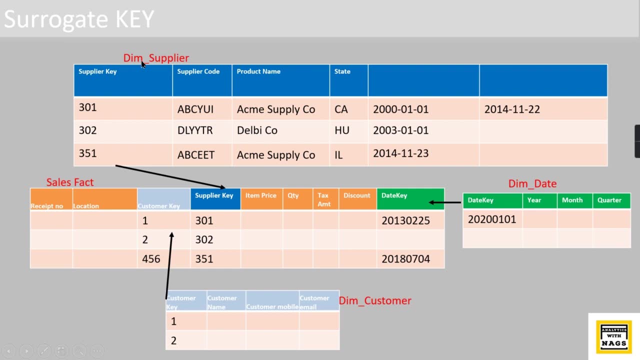 the core logic of data arrow. success lies on. let's try to understand it. so now you see, with the end, the example, one of the example i have. this is a dim supplier and this is the sales fact table and dim date and dim customer, usually from the business. we will get the supplier code right. 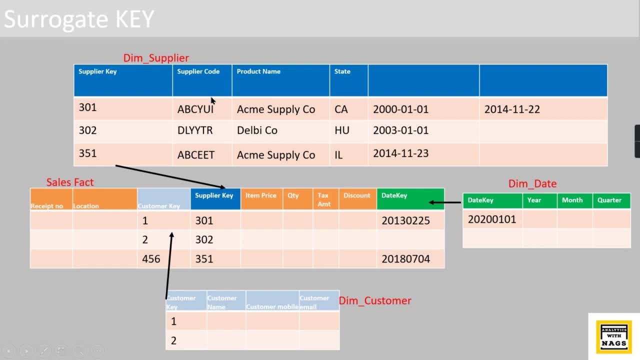 you. they maintain it can be id or code or whatever from the oltp system. so if you maintain this column in the fact table, there are 1 million, 2 million records, right. the core factor is, like the supplier code, it can be 1 million, 2 million records, like there is a. the core factor is avoiding the happening, which is right. only it can be that that the 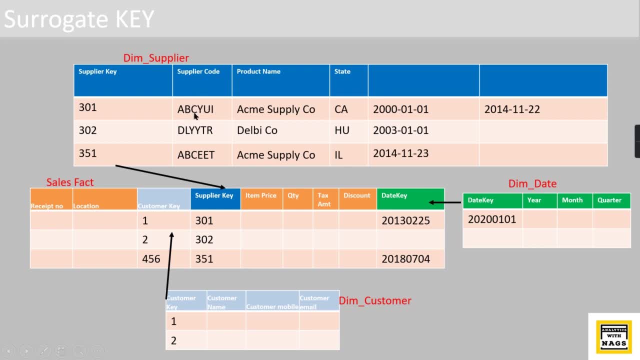 the supplier code. it can be n worker. you see a, b, c, y, u, y, which is: each character takes 8 bytes. i think so it will take 8 into 648 bytes to store, whereas the integer column for each supplier you generate one surrogate key that takes 4 bytes or 8 bytes. i'm pretty much not sure. 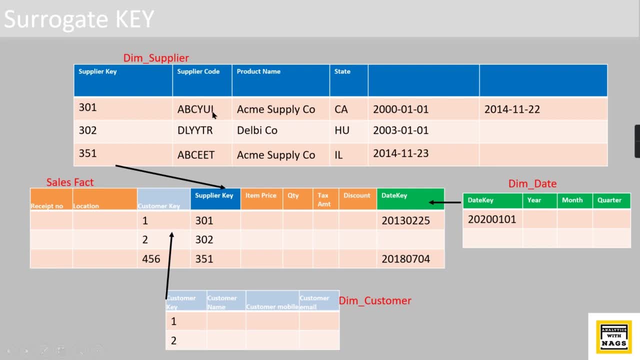 so this is the core difference from the 48 bytes. assume it is 8 bytes. the integer takes 8 bytes. so from 48 bytes for each record, it takes only 8 bytes and not only in the dimension. in the fact table it will reduce the amount of storage space, like 48 bytes, into 1 million, right? 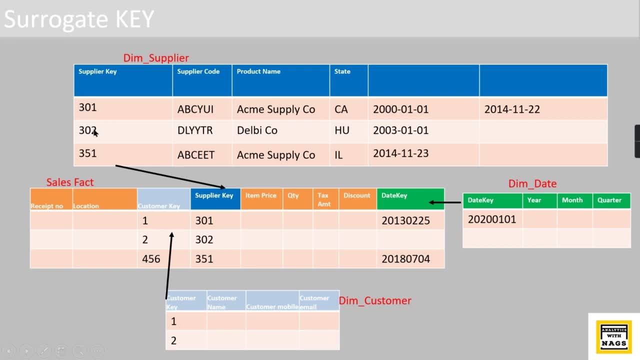 you are reducing one sixth of it because 8 bytes. so this is the core concept behind the data warehouse success. the storage in the fact table will reduce because the fact table will contain the foreign key references of your dimension table and which is nothing but a surrogate keys, which is an integer column, along with your measures, which will be a numerical. 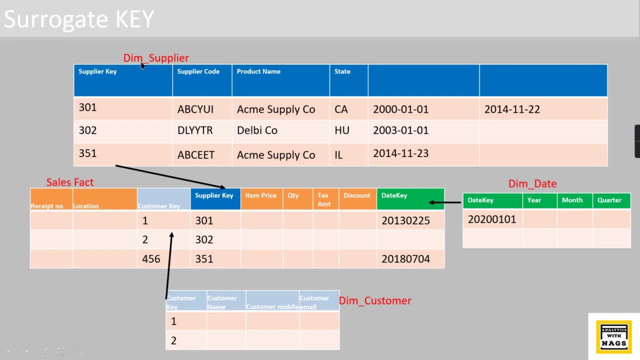 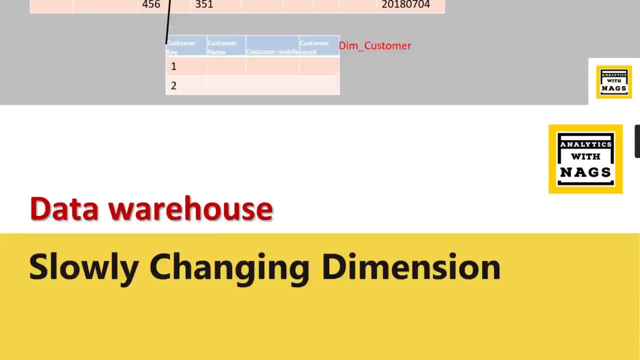 column. so this is what a surrogate key purpose. for each dimension you will create a surrogate key and that surrogate key will be referred in the fact table. i hope now it is clear why we are generating the surrogate key in the data warehousing design. the next important concept is: 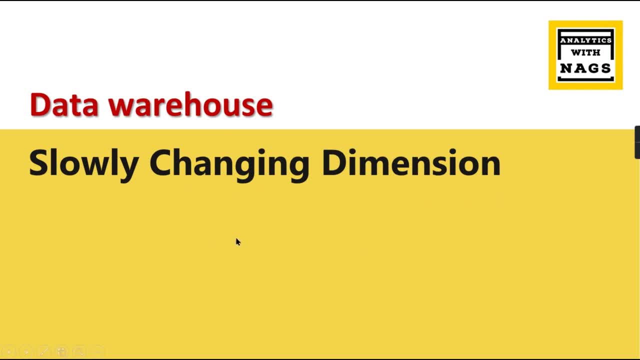 like slowly changing dimension. so we have started with populating the dimension tables first, since it generates the primary key and whatever we seen, like currency and product, which are scd1, meaning like they don't maintain history. what is history say? for example, a product is categorized from: 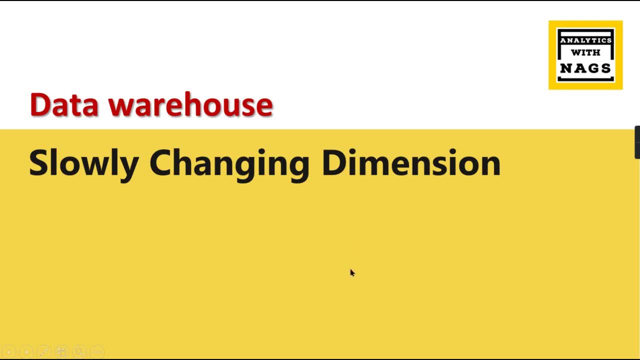 a category a to category b, when we are not maintaining the history. the latest state that is for a single product, it has changed it to category b. then we will maintain only the category b. then it is called scd1, there is no history maintained and whereas if you maintain history, that is called 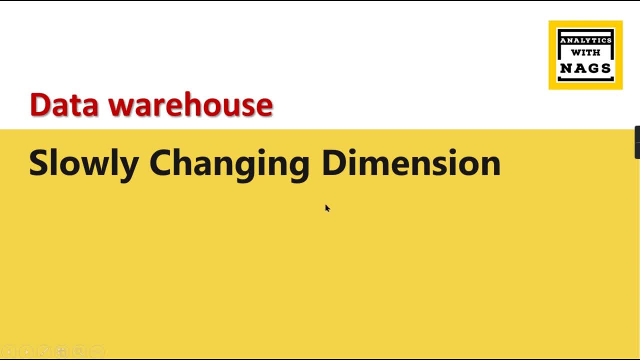 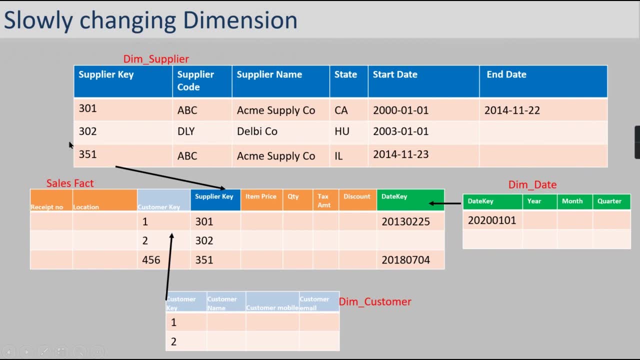 slowly changing dimension 2. that is what we are going to see now. so now we have a typical example here, and what is the main purpose of maintaining the history? right that i will also explain it now. for the same supplier, you see abc. here you understand the concept of surrogate key 301 placed. 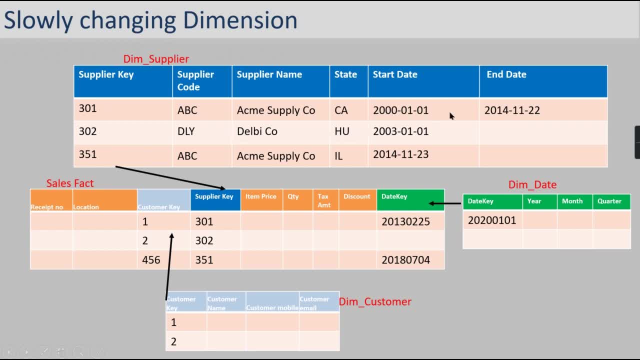 here now you see the dates right. he belonged to. this supplier belongs to ca state till 2000 till 2014.. so, whatever transaction happening during this period, when we do the report right, when you choose 2013 in the report, it should be categorized under ca. 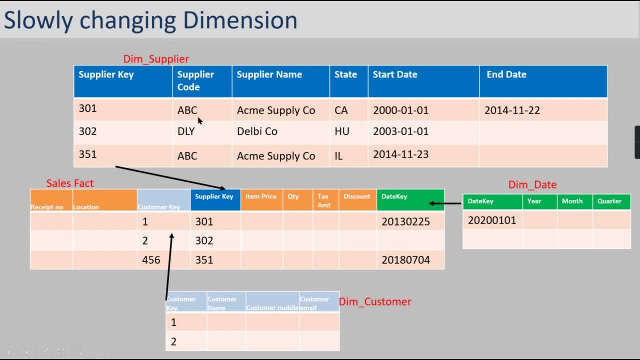 and after that, 2014, when this particular supplier moved to some other state il. that is, from 2014 11 23, right? so this should be tagged after 2014 11 23 under the state il. so how you can do it so you. 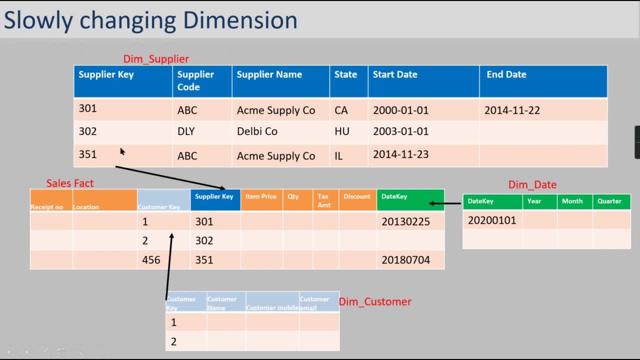 need to do is you need to populate the or maintain the history in this dim supplier table, like supplier code, as i mean from this bit and this period. right, this is what the scd2 means. you maintain whatever changes you know which attributes to be tracked, in this case state has. 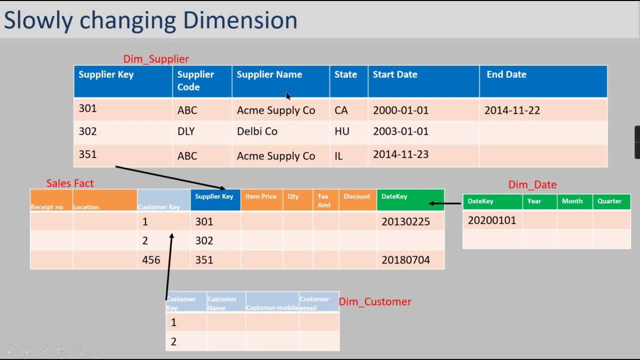 to be tracked. if there is a name change, whether you need to track or not, that you need to decide. so you should always change the name to the columns in order to be able to keep the history for a particular column, then it is called scd2. if we say acme, supplier company is not change. i mean if there. 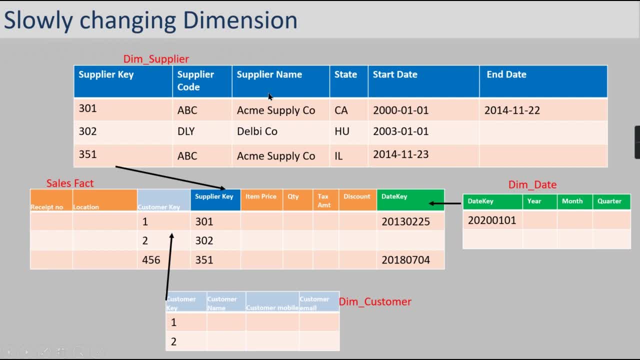 is change. you don't need to maintain history. they update this particular supplier name for entire previous records. then it is called scd1. so this is the code difference and how it will be useful in the reporting. whatever you choose, before 2014 11, the reports will show again ca because 301 tag for you. you see the date, the 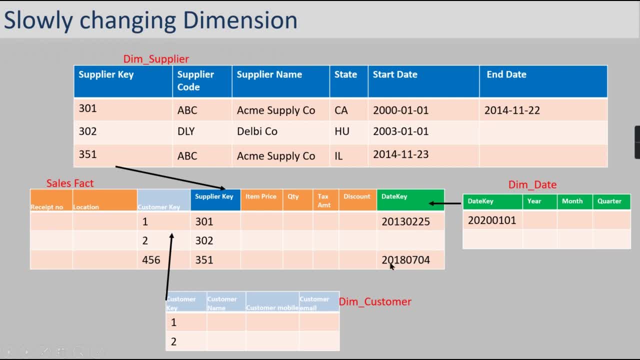 date is 2013: 0 to 25. now, in 2018, this particular abc has dead some transaction at that time. this supplier key is tagged because the transaction date look up here from start date to end date. okay, then, along with the supplier code, you will get the supplier code in the fact table. 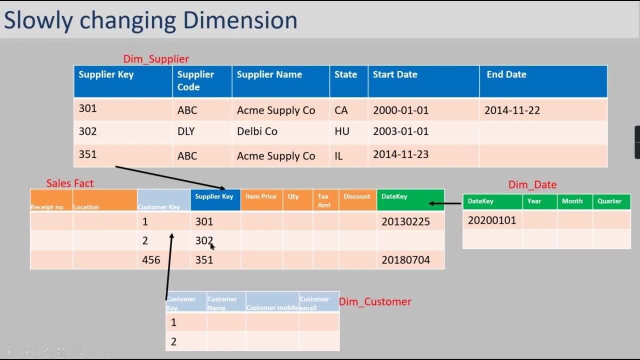 source in the staging. i will show it to you how you will populate this surrogate key here. okay, while doing the fact population. you will understand it clearly now i am focusing on this. so, basically, you need to look up from the source system the supplier code, along with 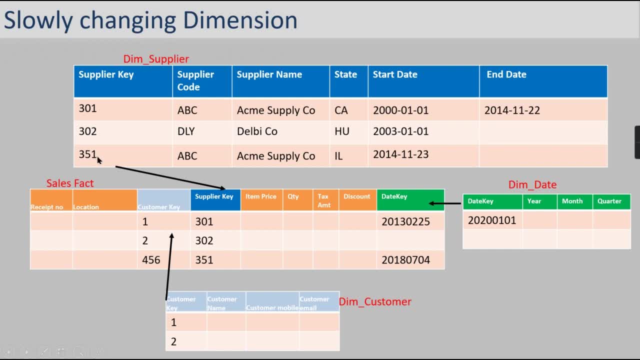 start date, end date of the transaction date to get the respective surrogate key for the 2 dimension, then you populate it. you need to look up from the source system the supplier code along with the start date. So this is how you will design it and why it is important. during this period it will report under CA and after that period it will report under IL. When this is your requirement, right then you should decide that particular dimension as SUD2.. In our case, we are going to show you the employee dimension as SUD2, how we have designed it. Let's check it out in the demo. 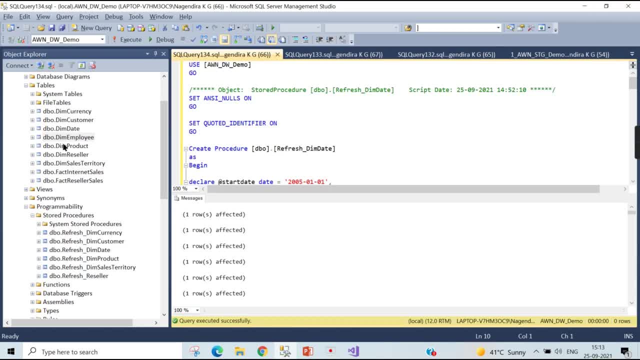 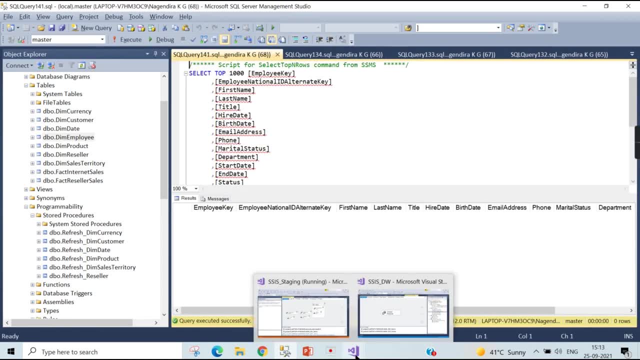 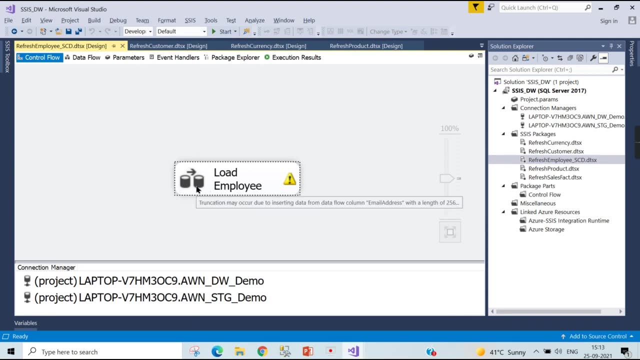 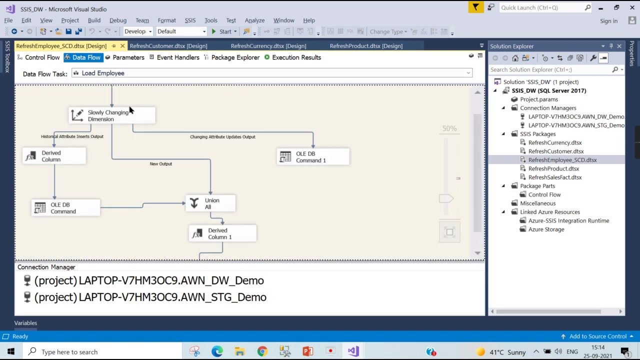 Now, as we have already seen, this employee table is not been populated yet. because it is, I want to demonstrate SUD2 logic to you. So this is where I designed this SUD, where we have a separate task called slowly changing dimension task. Either you can go by this task, but people only have to go by this task. 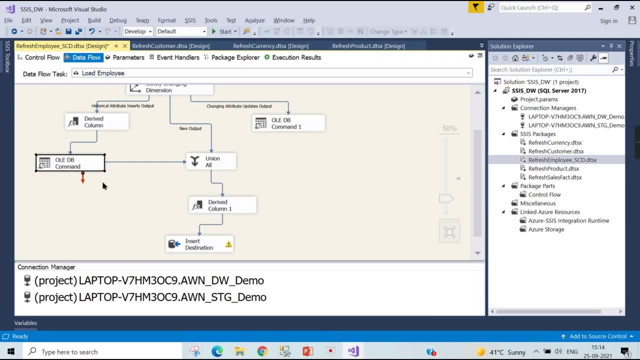 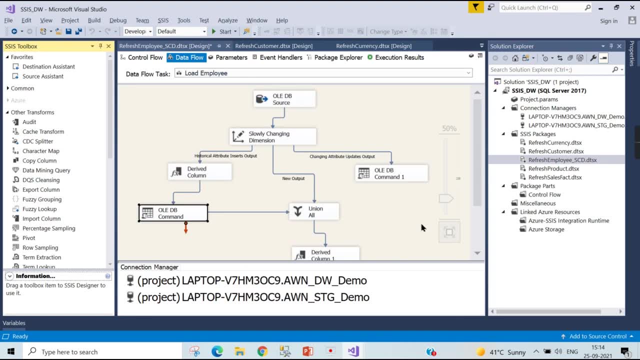 Either you can go by this task, but people only have to go by this task, Either you can go by this task, but people only have to go by this task. If you don't follow this because of this OLDB command, which is slower, you can write programmatically but due to time constraint, I followed this slowly changing dimension task itself. 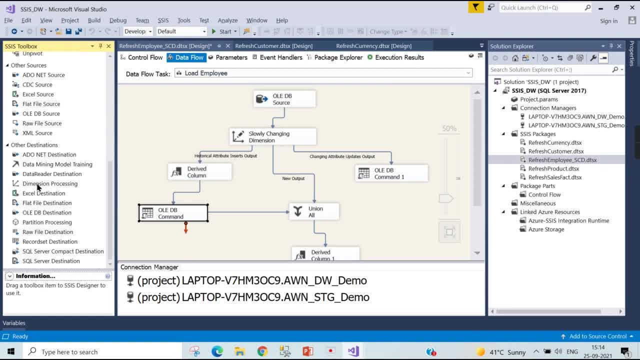 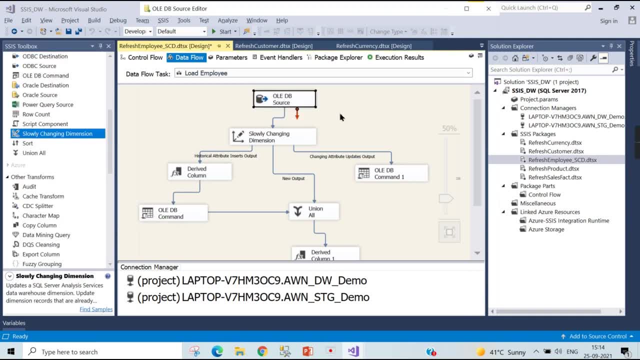 So you have a task here like slowly- where is that it's under common? slowly changing dimension. once you design the source from the source view, ERP employee, right, then you will configure this okay. So you have a task here like slowly- where is that it's under common? slowly changing dimension, then all the data will be populated here. 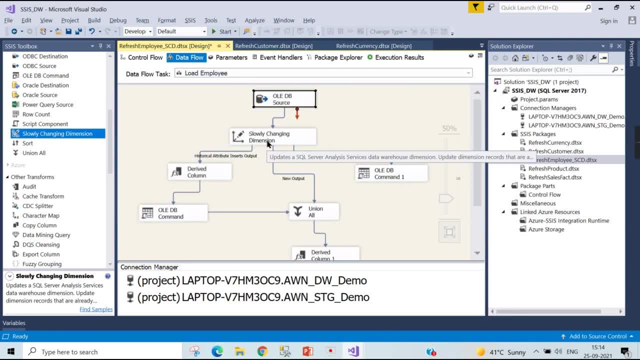 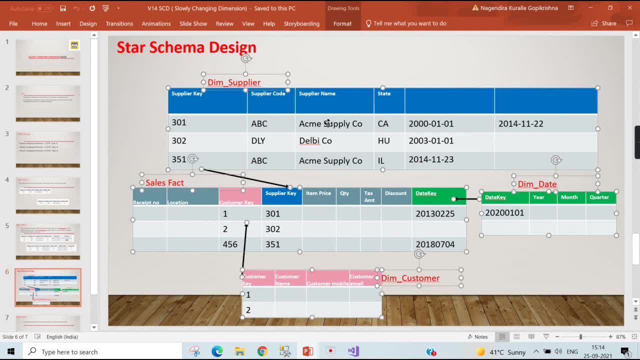 If it is this particular task, will handle both. like as I said before. if something changes, okay. If it is this particular task, will handle both. like as I said before, if something changes, okay, You do not want to maintain history, update it. that is SUD1 for supplier name or employee name. 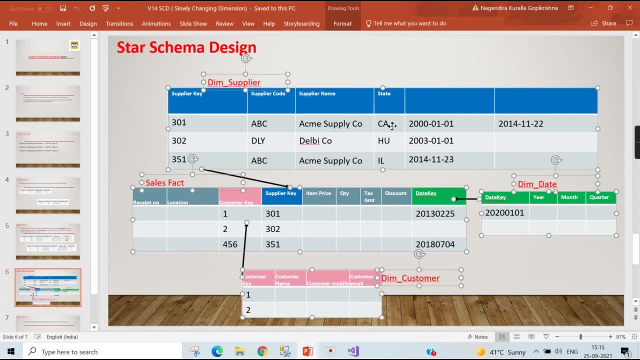 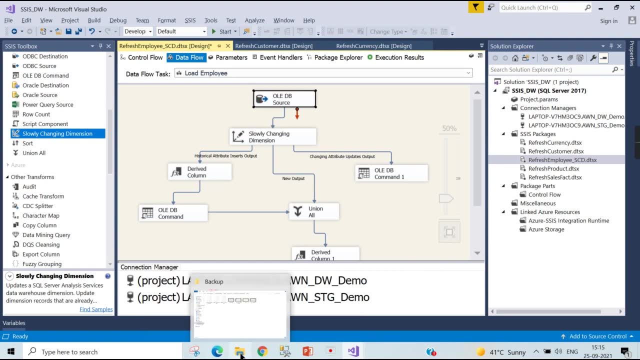 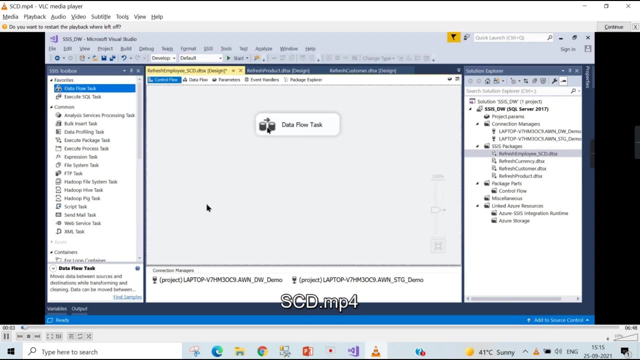 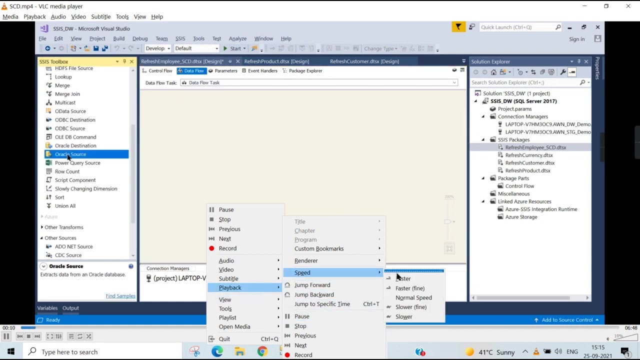 Now something is changing. you need to track history. that is what the flow follows here. Let me play one of the video that, while I'm creating, I recorded it so that you will understand it better. Now you can see what I'm doing. I will just do the fast forward speed is faster, so that you will understand it. 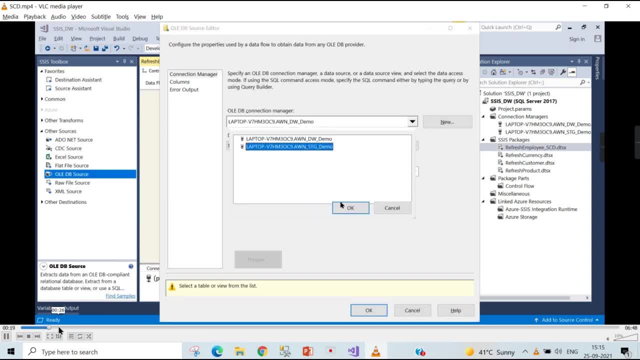 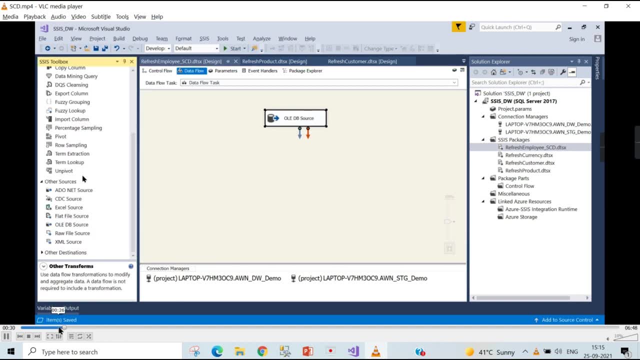 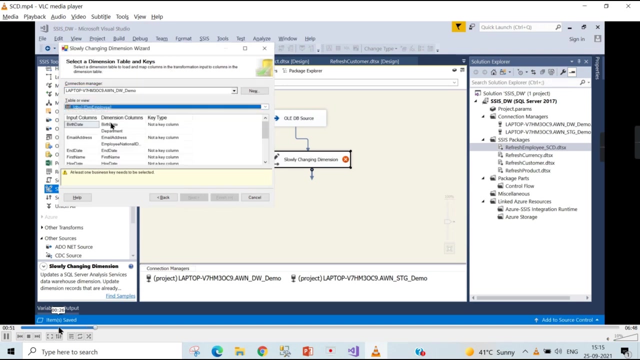 So I use the source from here. I picked up. I have written the view. Obviously I need to get it from multiple tables, So I picked up. Anyway, I'm sharing that view. You can explore it Now. I drag and drop this slowly changing dimension. Now, once you click on it, you choose select the dimension. You need to choose a target table here, So this is dim employee And here you need to choose the. 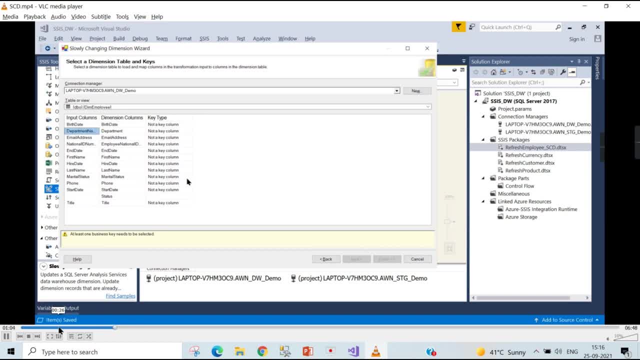 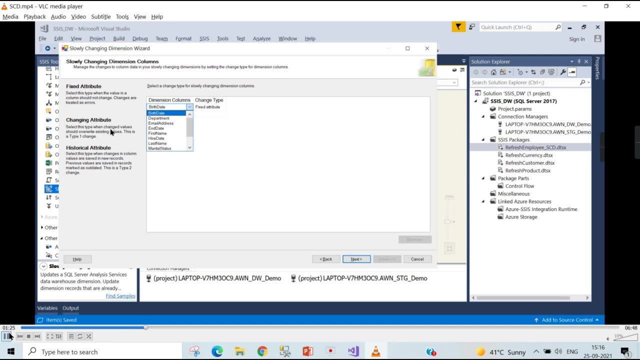 business key. Business key is like as well, You look up to look up right, whether they exist or not already. That is what. So this is the business key, That is, an employee national ID. Then here you need to choose- Let me pass it here: So the fixed attribute. if there is a fixed attribute that should not change, then it will fail. So skip this part. We need to focus on changing attribute and historical attribute. 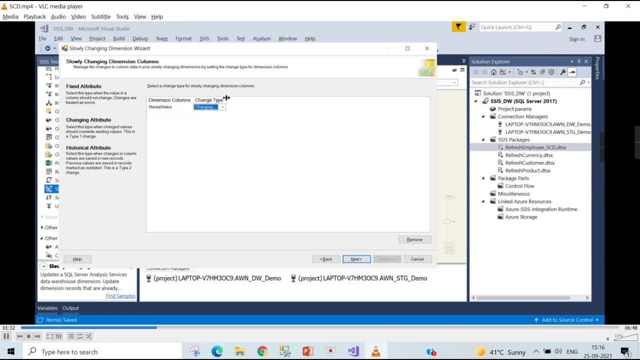 Basically like birth date won't be changing, right, That you don't need to mention, that is for fine. So marital status will change. changing attribute: Correct. So changing attribute. you will do the update If marital status changes. no need to maintain the history for it For that. you just say it is the. you have changed the marital status. 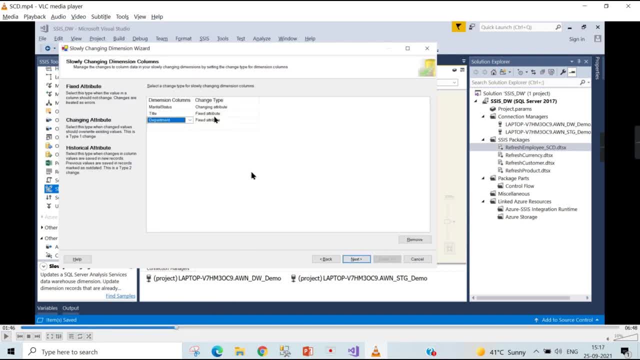 So here, what I'm trying to say here is, like the marital status changes, You don't need to maintain the history for it When he got married. that is not very good comparison. You can keep him as married or unmarried at the current state. So that is the changing attribute that is called SED1.. No need to maintain history. But when there is any department changed, okay, that becomes. 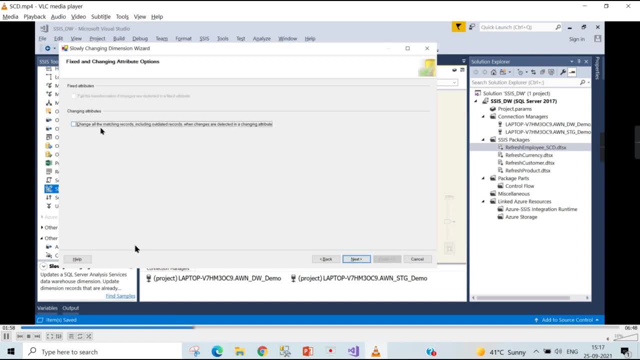 a historical attribute, so you need to choose that one. that is what scd2 is now here. these things will. it will ask whether it should be applied for changing attributes for previous record. you say yes. here is the catch. you need to choose the start date and end date. that is the key factor in the 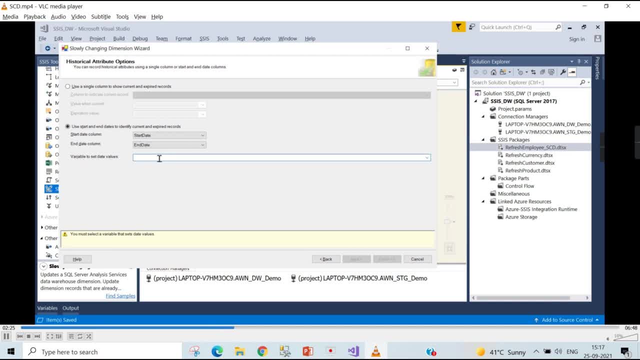 scd2. so you learn more about scd2, you will get to understand it. so here in the start date column what i need to mention for the new records: right, so systemcreated it, i am keeping it. next you can click on next: inferred is different concept. you can skip it for now and uncheck it. 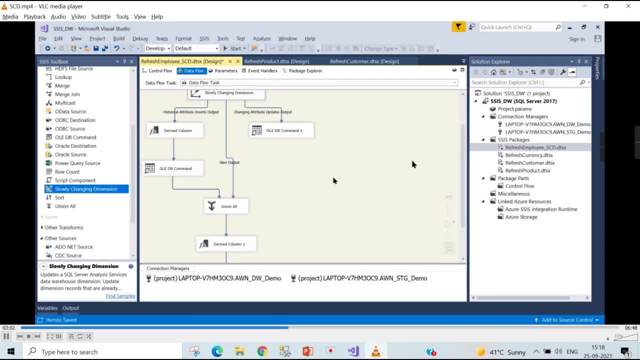 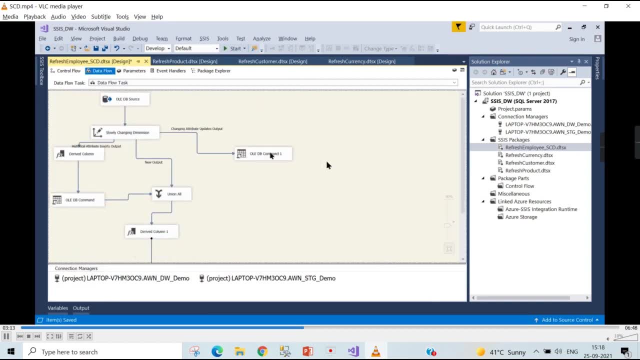 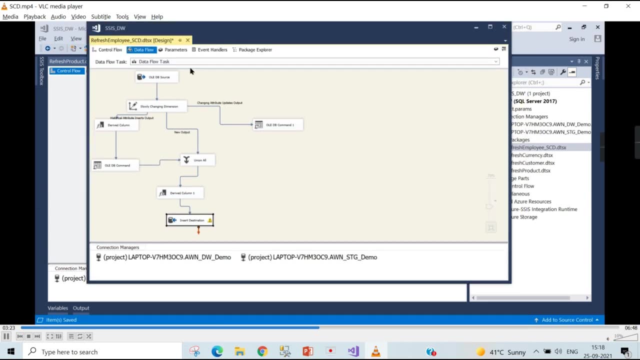 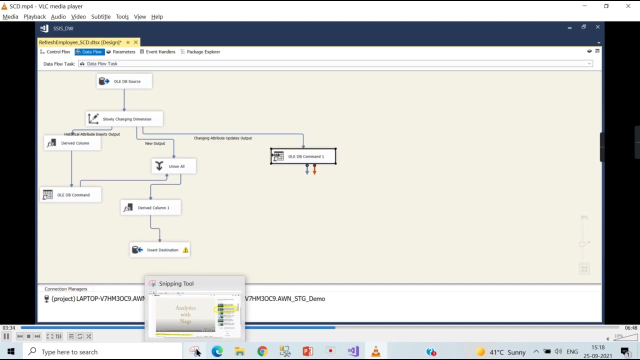 once you are done, you click ok. the this slowly changing dimension task will create a separate flows for me. so basically, like towards your right hand side, like oldb, command over here the changing attribute. let me zoom in so that it will be fine, so you can see that changing attribute, that is scd1. what it will do, it will create one for each. 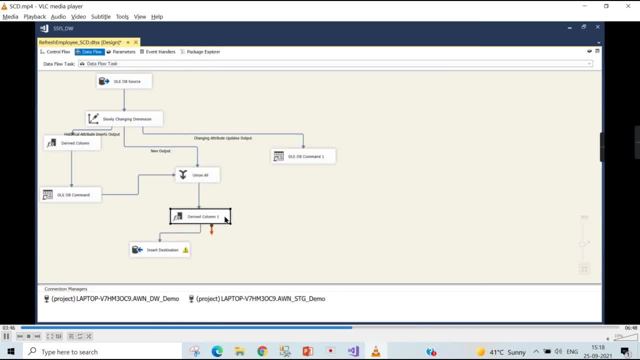 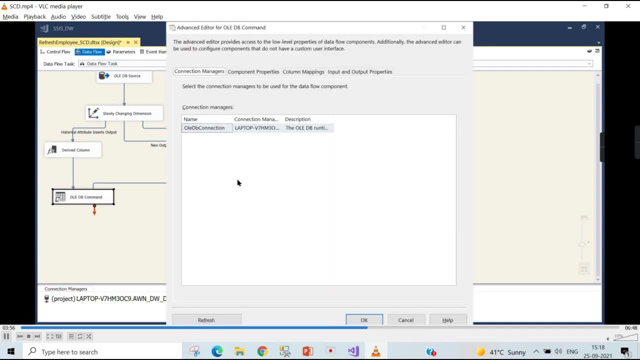 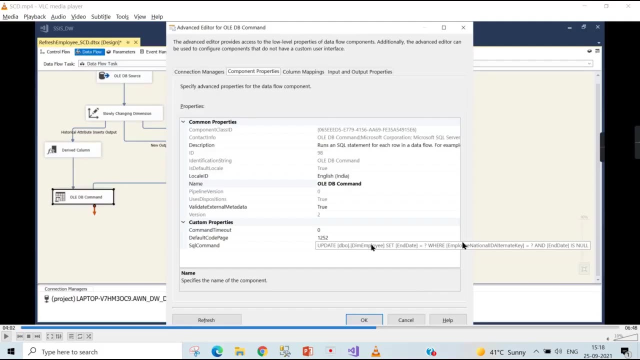 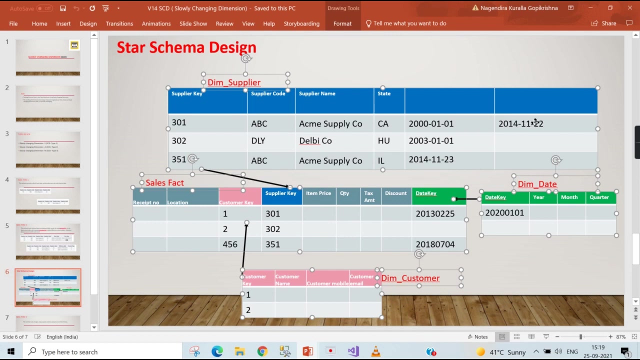 record. it will send you an update query and for historical attributes, that is at the towards your left. okay, that is, it will derive the column and then update the old record. so here i will pass. what i am saying is you can see here: this record is valid till 2014 11 22. okay, on 23rd, only this state has changed. 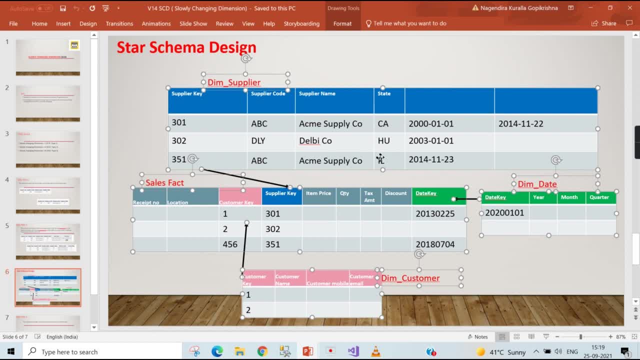 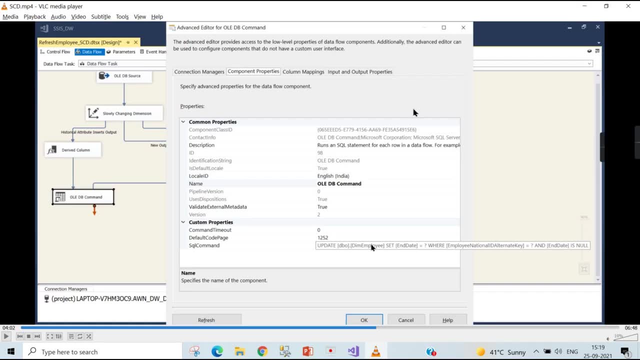 that change has been detected, this particular column, some data has been changed, then you need to expire this old record, then create a new record, right? so that is what it is happening here. that update has to be happened. so now we are setting the end date to the. 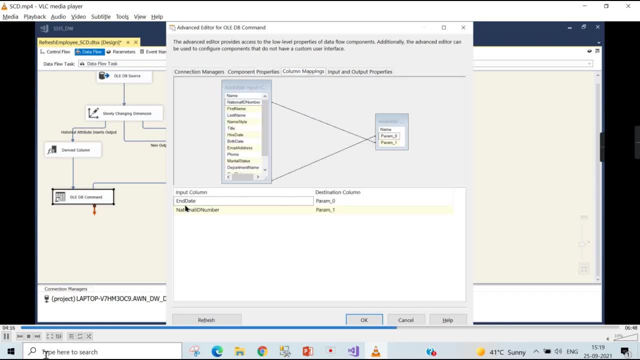 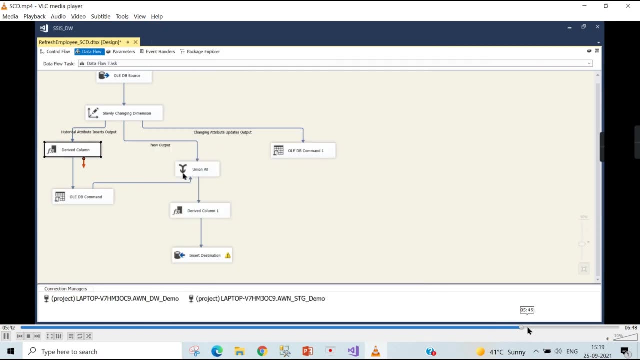 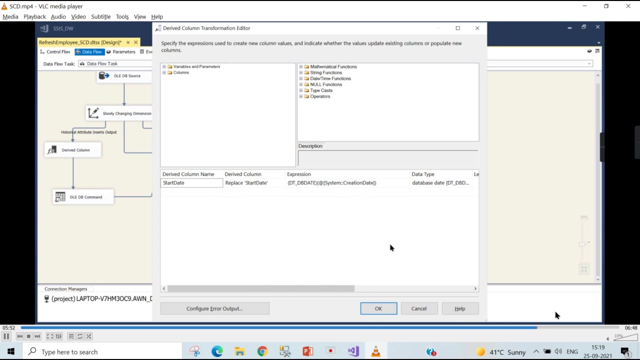 삼성. so after that we need to do some Johnson test. at least we should start this and don't forget, while standing center flow of your outcome over here. let me just go ahead of- i keep checking the map at the moment- this center flow of the output. you are giving this a sample. 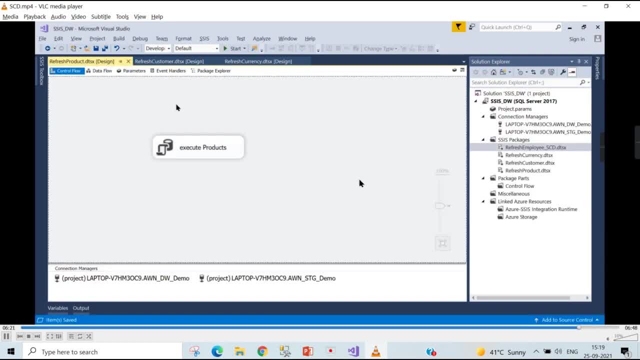 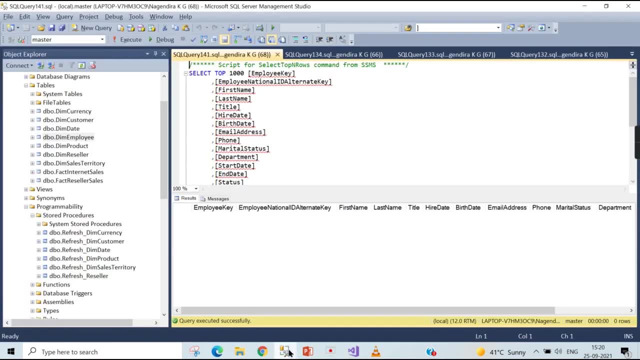 trace. so this is the record that we are getting. so which is our new output is asking the new Bed comparator. this is the data you need to remember. I hope this is clear. there are different ways you populate the scd2 tables: where you maintain the scd2 tables and once 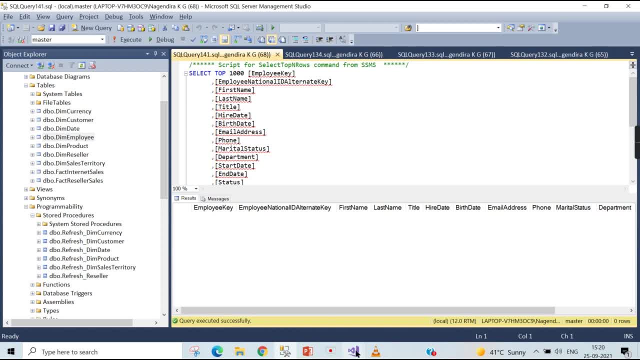 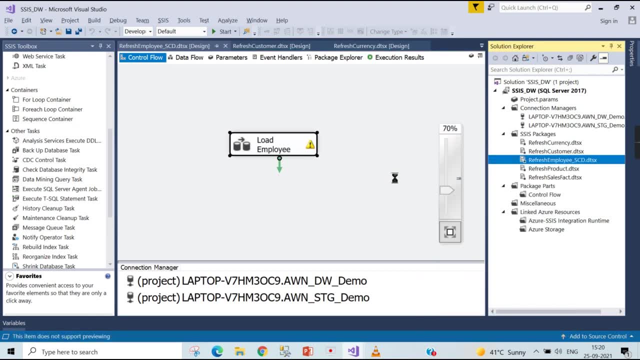 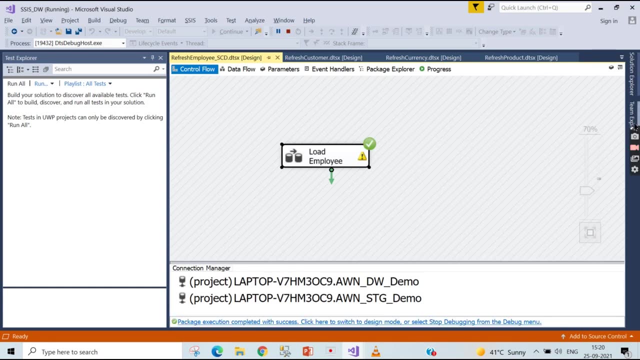 the data changes, you can populate it. this is the one of the way I followed. now, how you will populate it. just this is already designed. just go and execute this package. so either you write a procedure and call it in SS package or execute manually. this is for the one time. I mean initial going forward. 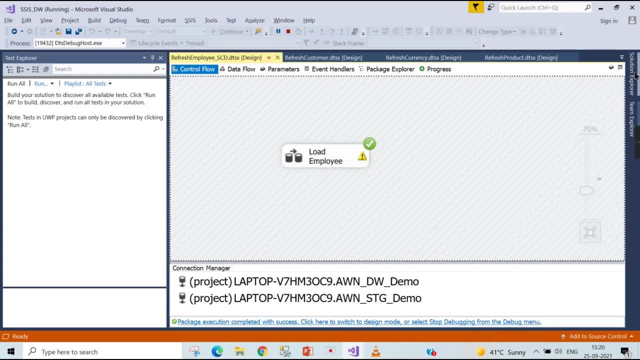 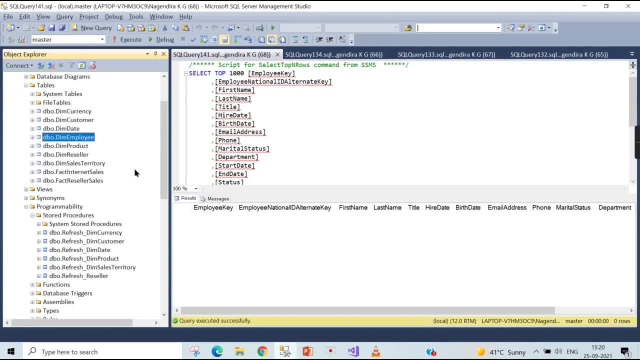 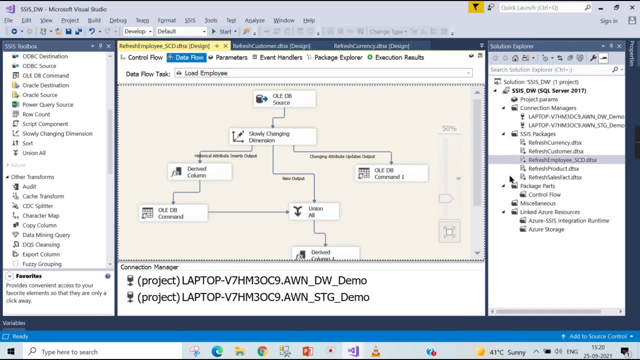 regular schedule. you will schedule this package, okay. so every time the new data comes, this package will be executed. that is fine. now you go and check this employee table: here there is no data. let us see why. you can see that the data has been executed. and you can see that the data has been executed. now you go and check this employee table: here there is no data. let us see why. 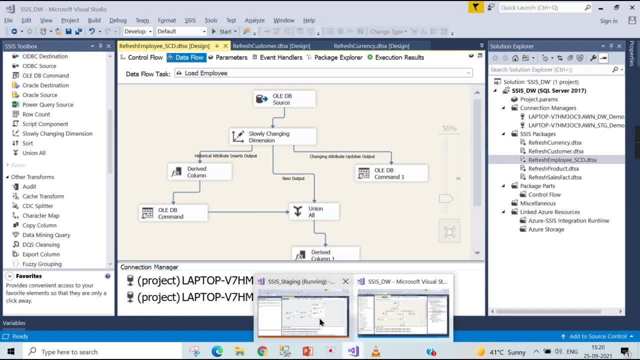 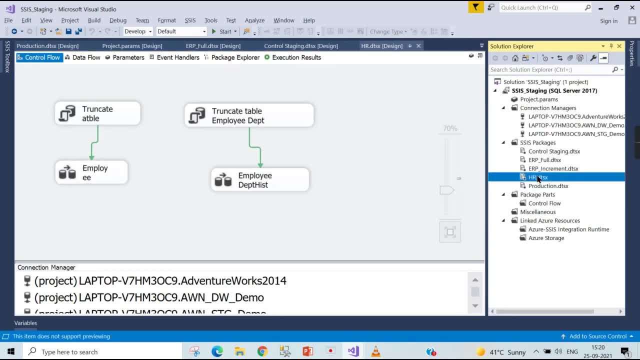 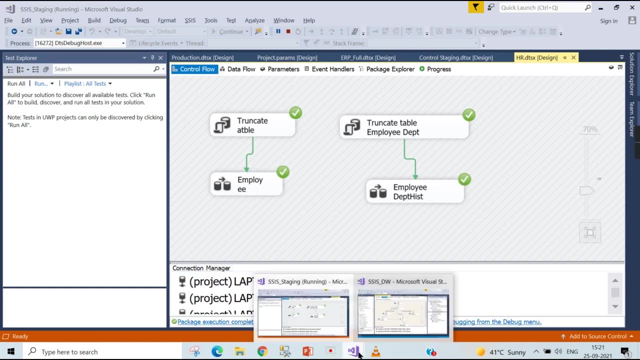 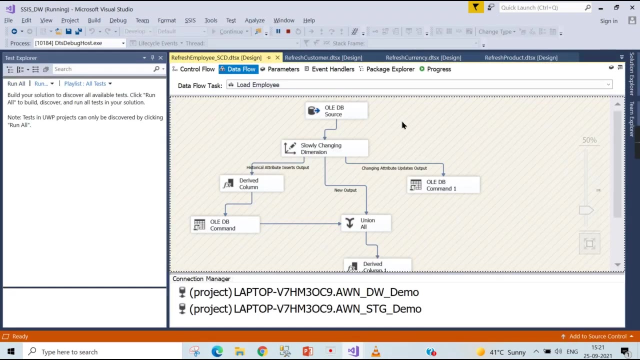 whether okay. even I didn't run the HR package here in this source, so employee tables- I have kept it here. we didn't run it, so execute this one as well in the SSIS source. now you go to data barrows: refresh scd2. execute package there you. 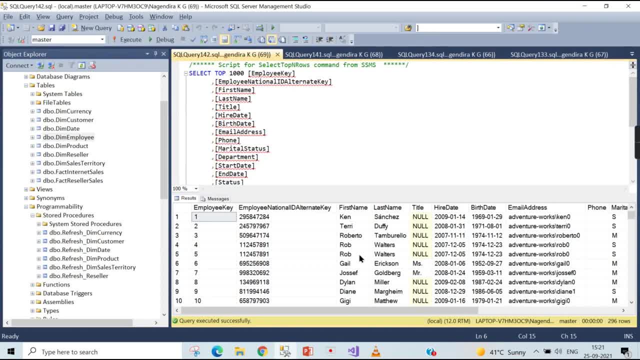 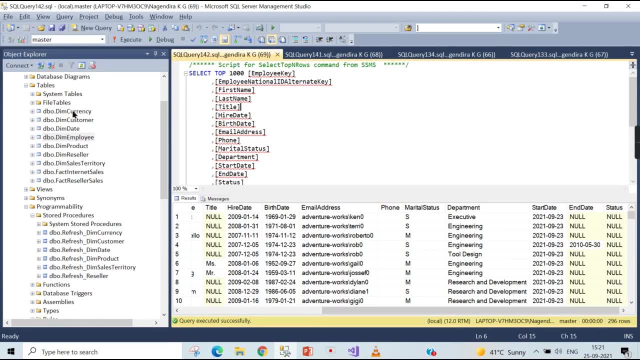 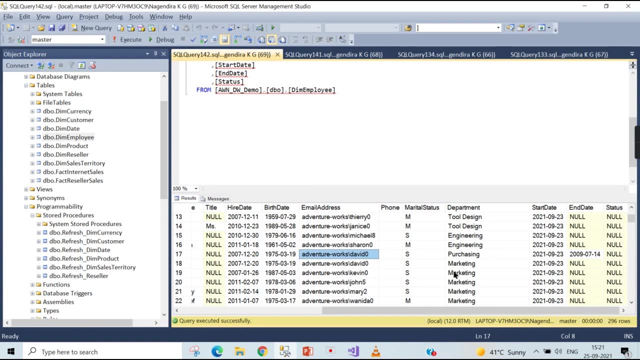 go. now it has done, it has loaded the destination. now execute it. now you got the data over here. now this is how you populate all the dimensions. whether it now there is no change in data in the employee, but still you can see some difference. I hope there is some issue here. it should not be 29. 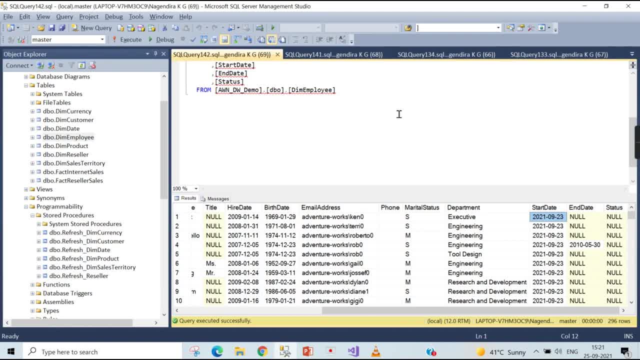 to 23. that is, forget about it. we need to rev up, remap it. but to understand the concept I have populated here, okay, so let us try to update this script. so do remember to update this script. okay, it should be mapped directly from the source system, but now there is some issue. to fix this one, let me update the. 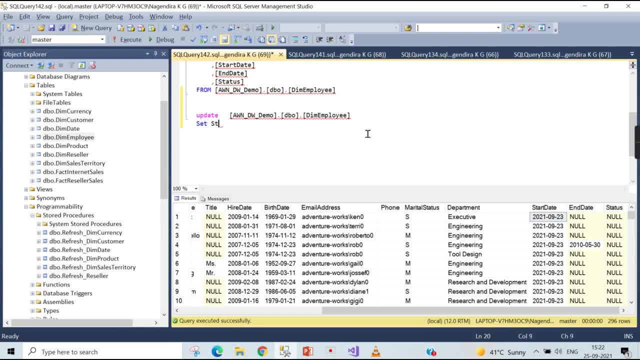 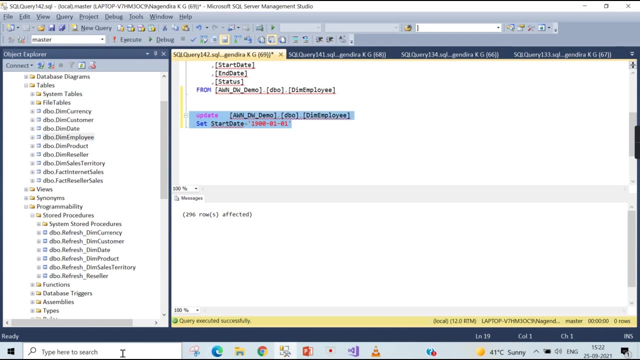 start date. set start date equals 20 post 1900 from 1900 01. okay, fine, so this is fine. I will make a note of it. I'll take a notepad, I'll give it in script to fix, otherwise some something else will fire. okay, this is fine. so we have populated the first step towards here. 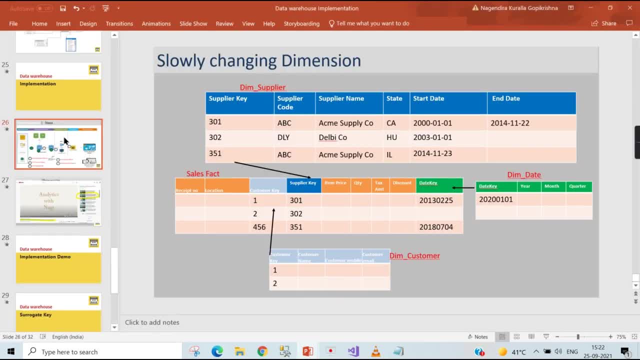 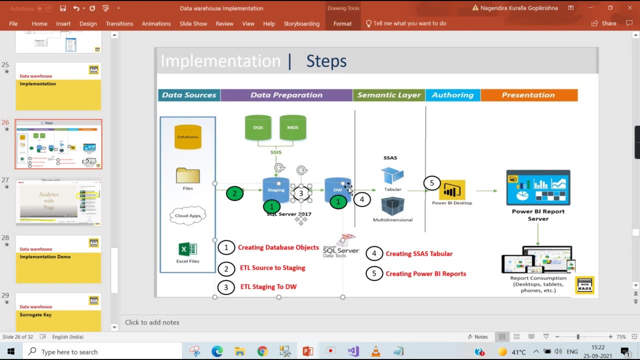 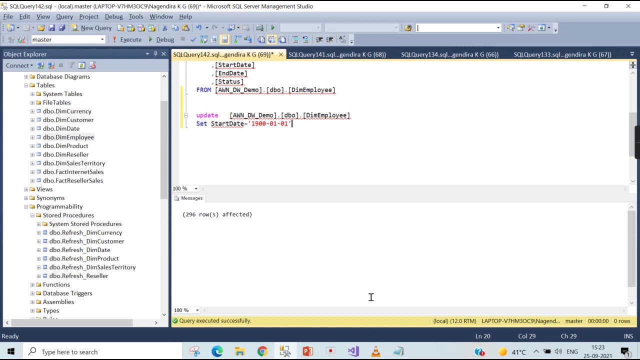 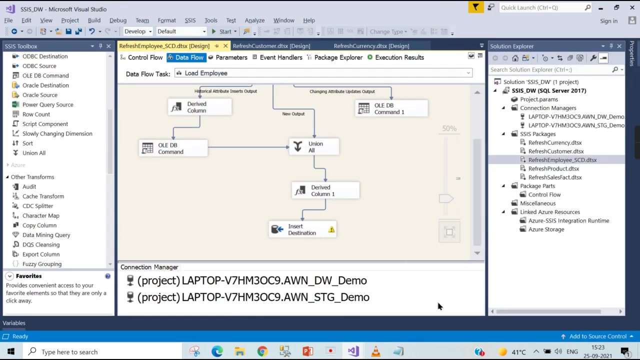 like we are still in this step, like from staging to data warehouse, but we can say like halfway through we populated the dimensions. next we will populate the fact. fact, where is that? whether we have run the ETL or not in the SSIS, let's see. I think this is the 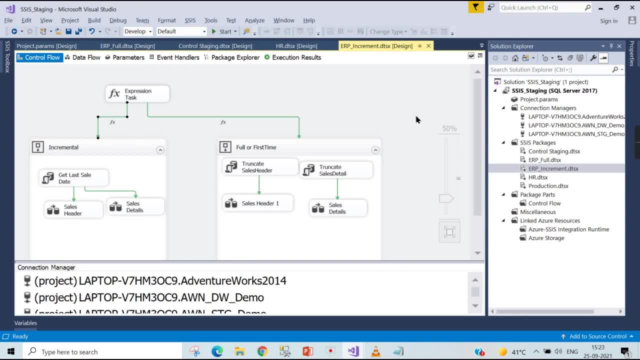 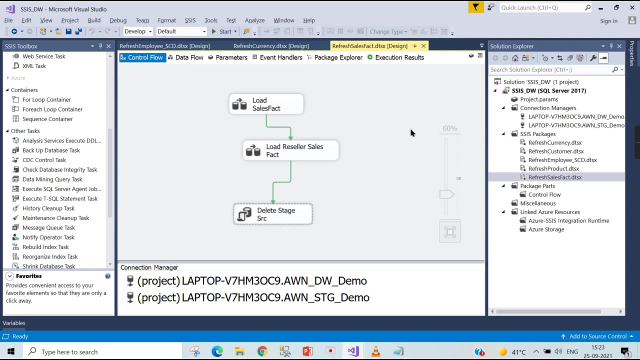 one right: the sales table, the incremental and sales. we have already executed incremental. now I am in the full load, the full run. it is already executed. now we can go to our data warehouse package and then check the fact population logic. now the fact population logics over here where we need to load two fact tables. we 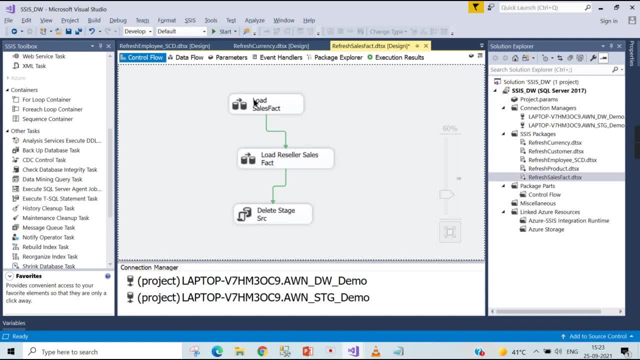 have decided one for internet in terms of data yesterday widget image: if you leave it, satu file ekta aku tarih kart. Elijah enk Tonight the fact population logic, where we need to load two fact tables. we have decided another for reseller sales, how it will look like now going back here, it's a. 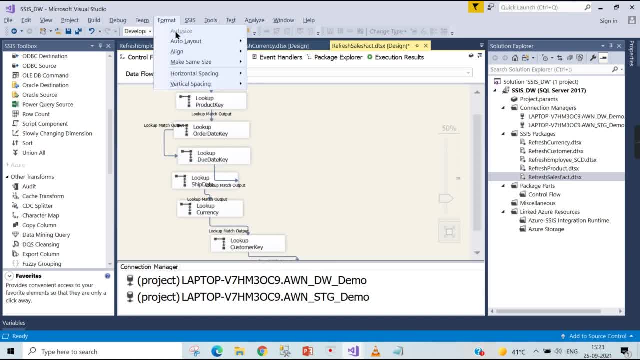 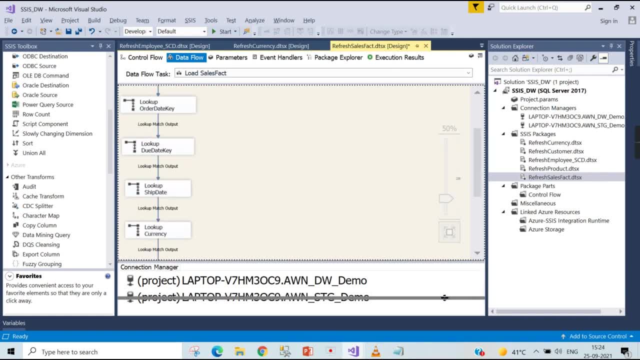 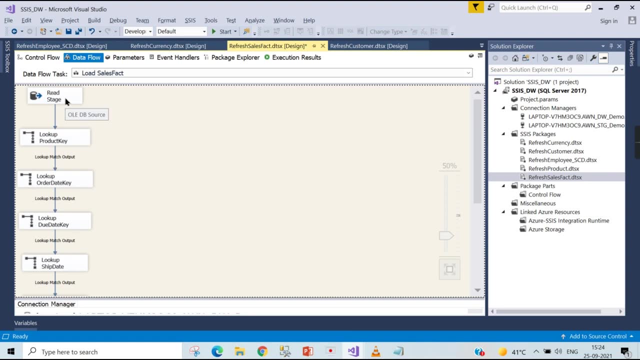 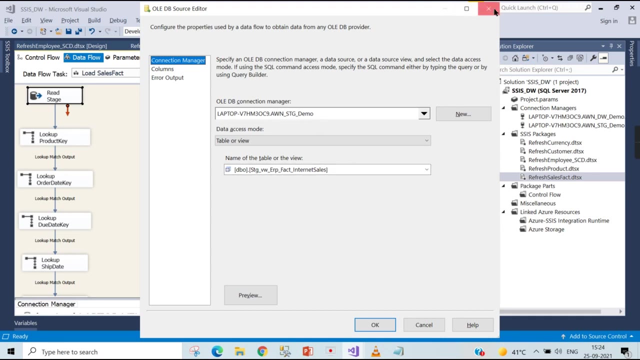 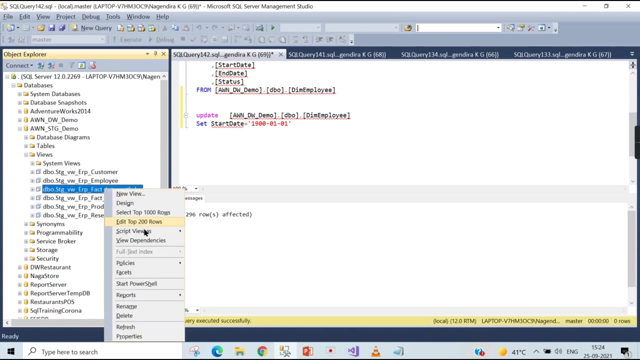 huge flow where- let me arrange it in a diagram proper way and you can see it here- we close everything. okay, now you can see it is reading the from the staging. let's see this view. stage view: ERP fact: internet sales from the a, W and stage demo. so we will go to stage view. this is internet sales, how it has. 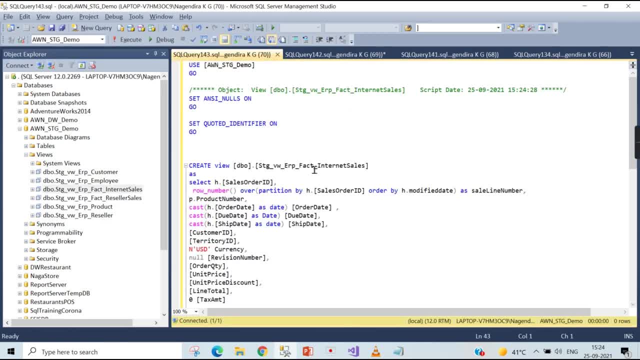 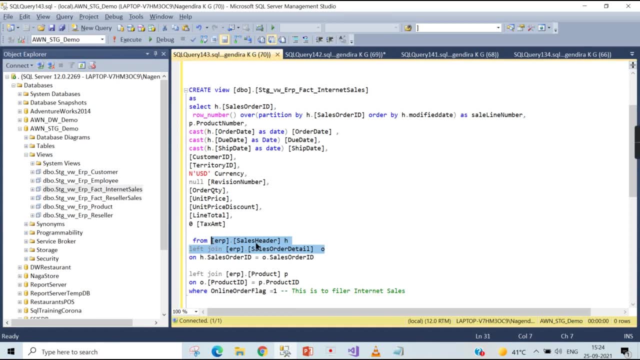 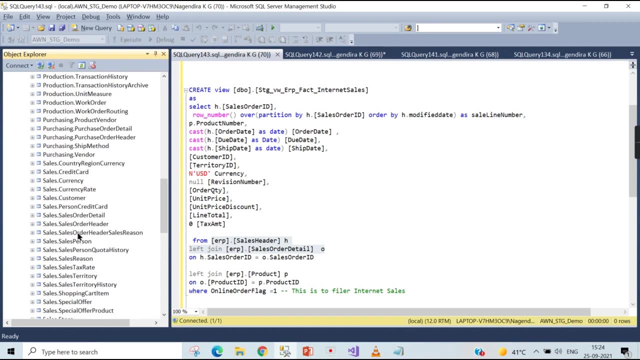 been written. now you can see here how it has been written. from the sale header, sale detail. we combine these two tables in the ERP system. we already seen anything here. the sales header and sales detail, both together right. i mean header will have only the header information, detail will have each line item, one product. what is the product different? 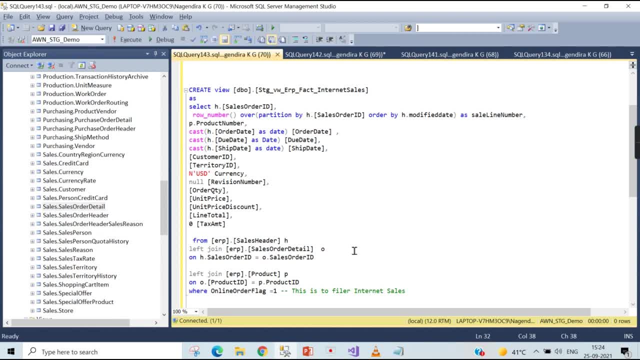 products. that is how it has architected. but now we cannot, no need to maintain the granularity here. we cannot maintain two fact for header and detail. this is: how are the designing? the experience comes. you need to design the fact at the least level so you maintain it at the 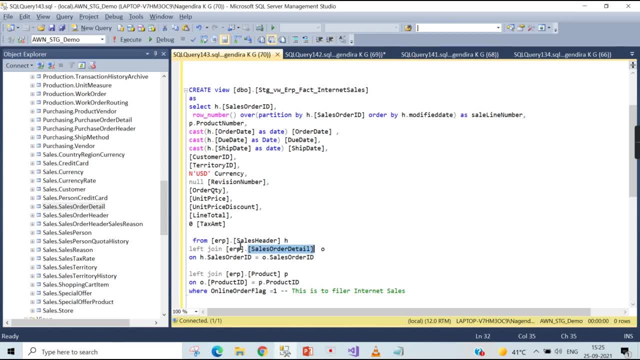 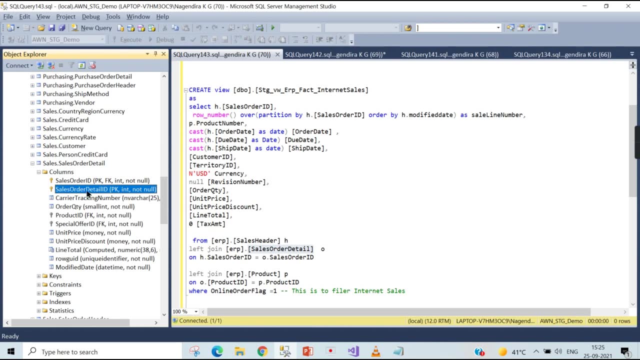 order detail level. so no need to maintain separate fact for header. so you combine this header and detail and you are maintaining at the detail level. this is the granularity you are maintaining. and again, this order detail ID is not for each other. there is no one to three in the source, in the 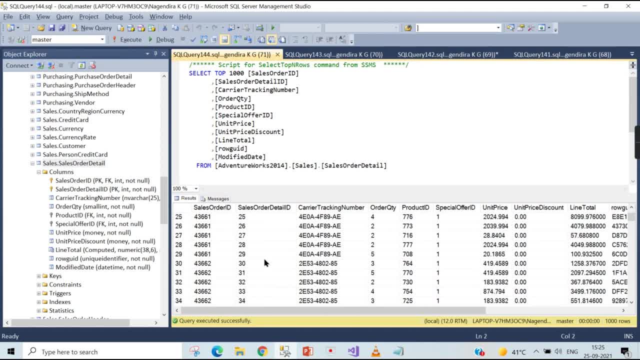 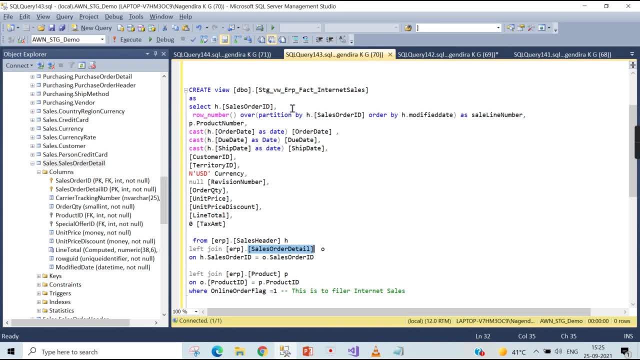 source you check here it is one, two, three and it is on incrementing one by one. this will be somewhat difficult, so here either, you can maintain that, but we designed in a way like it should be, say, line number, so for each order we need to generate one. 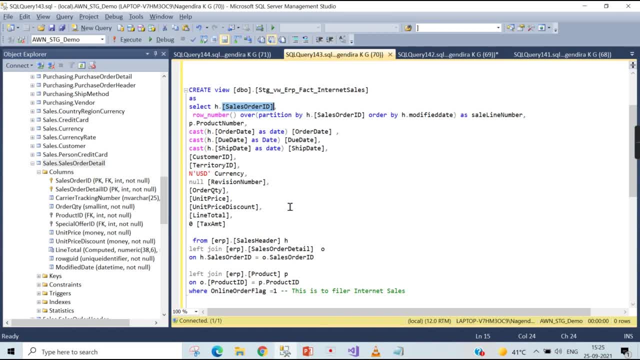 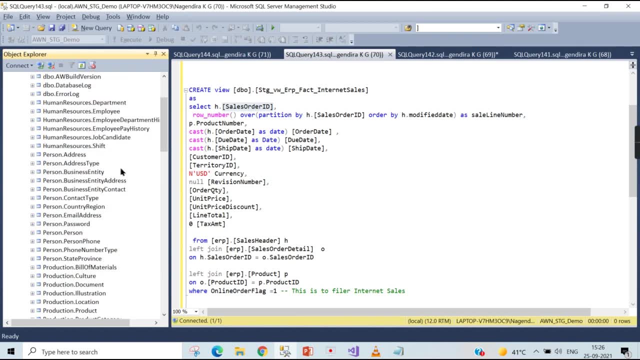 line number. so these kind of modifications, okay, these kind of modifications you need to perform. that is why we need the staging area. so why we need staging area people. some people think like directly from the source system i can generate the report in power bi those things is where 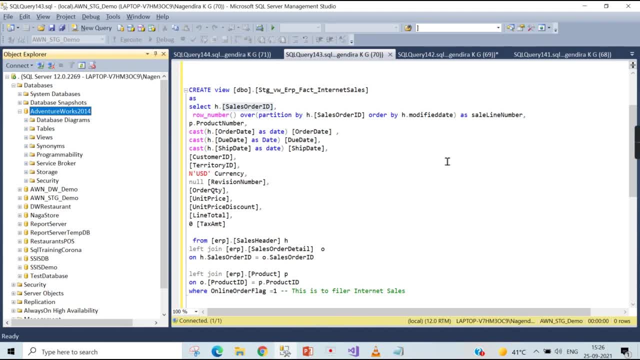 simple reports. it's fine, but when you want to have a proper modeling, proper database design, you need to have a staging area and data warehouse. that is where i am repeating so many times in many of my videos: you need to learn the entire cycle. that is a topic for. 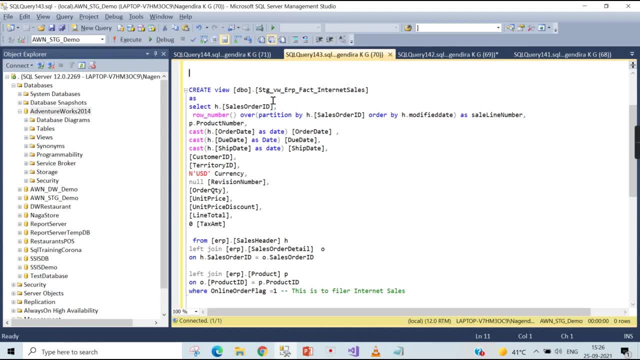 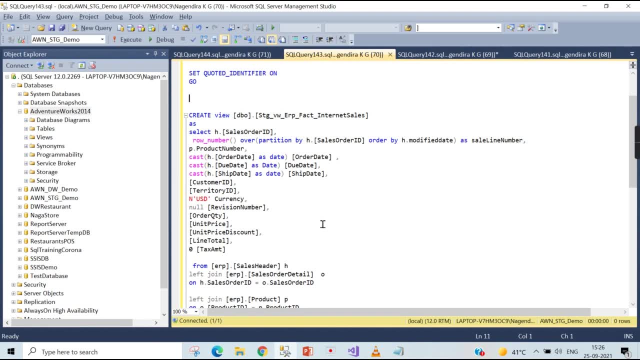 another day. but now to understand why we need staging here, you bring the tables and then you met some concepts here. i mean you need to filter now. you see, this fact is meant for online order, so you will filter it here. so these logics you are applying and creating it as a view. 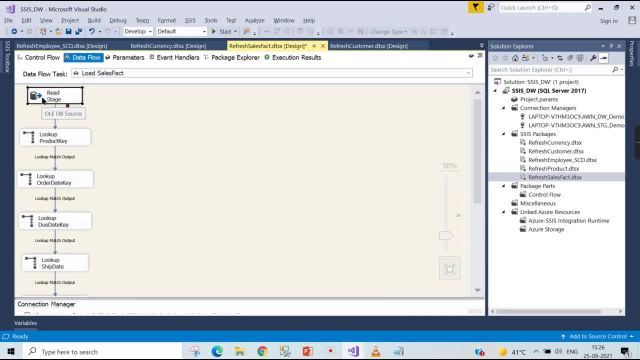 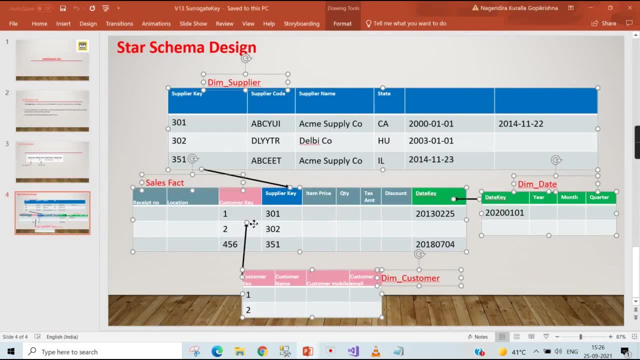 then going back to our data arrows. so this view, you are reading it. and then what is the main purpose of your fact tables? you need to generate the. get only the surrogate key, the reference from here, right, so the fact table contains key of your dimension table. how you will get so in the source you will get the supplier code. 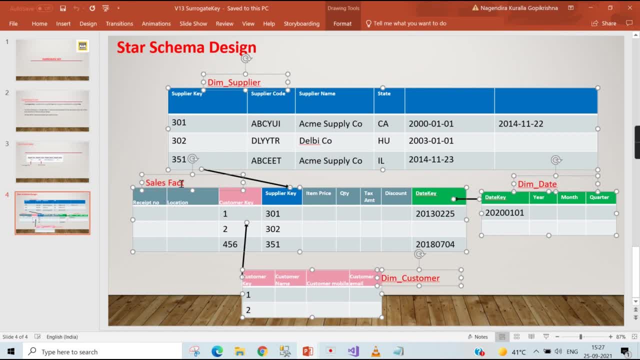 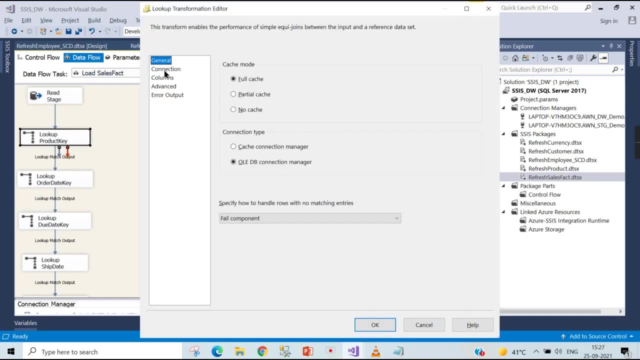 the supplier code. look up with the source tables- okay, this is fact table. then get the respective supplier key. so that is what we are doing. first we are going with product key. now you see, product key is looked up here. you need to select the product key from the data arrows, then columns. 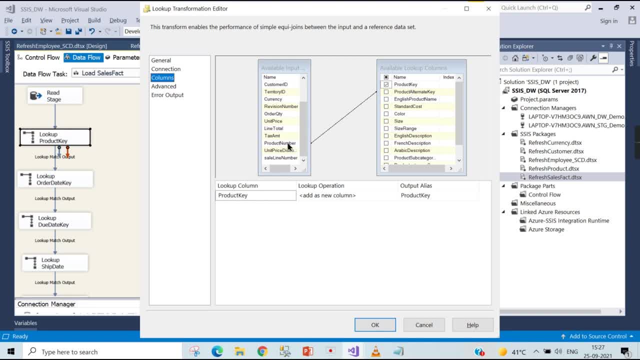 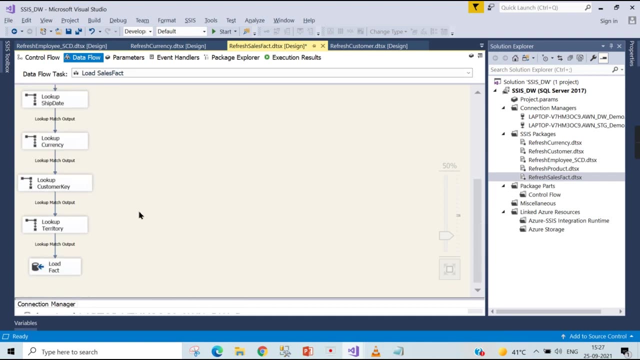 to map. here you see, product alternate key from the dimension here, from the source table, that is, source staging table. then get this product key here. that is how you will design it, similarly for order date key, due date key, shift date key, everything you will design and then finally you 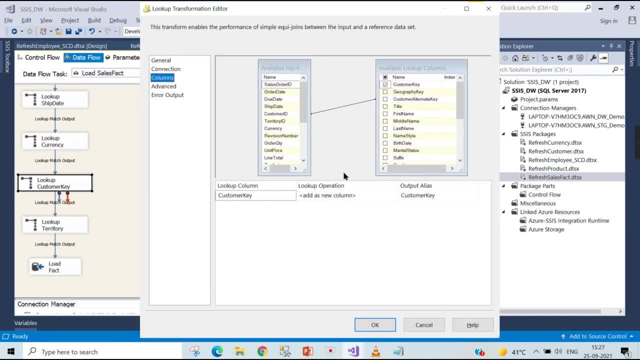 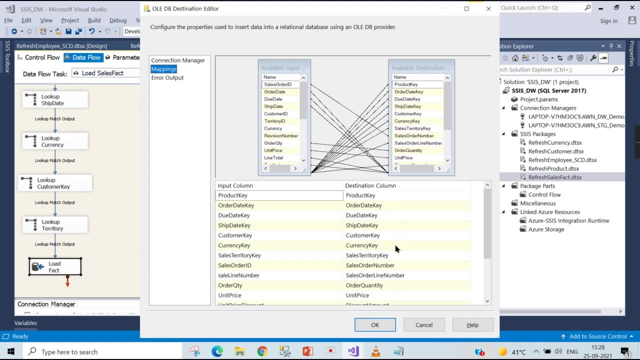 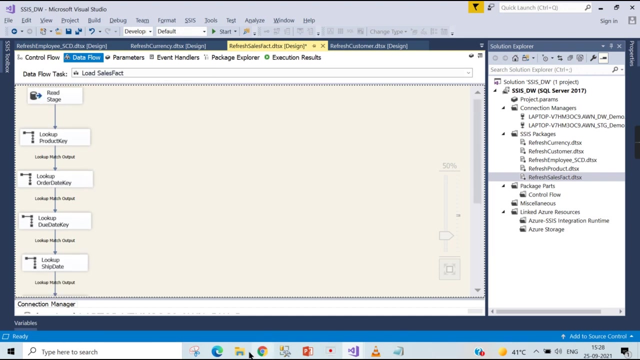 populate each table. you will look up some of the key column, that is, business key column, then then you will get the respective surrogate key. then finally, you load it into your fact table. the fact table: you will get product key, order key. so this is how you will populate your fact tables as well. 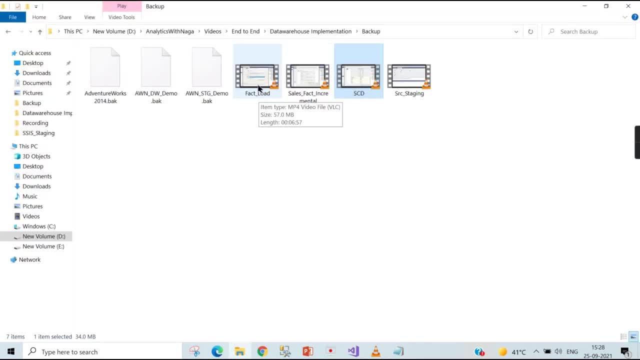 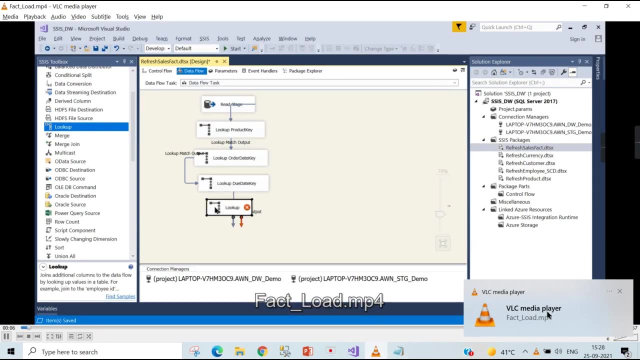 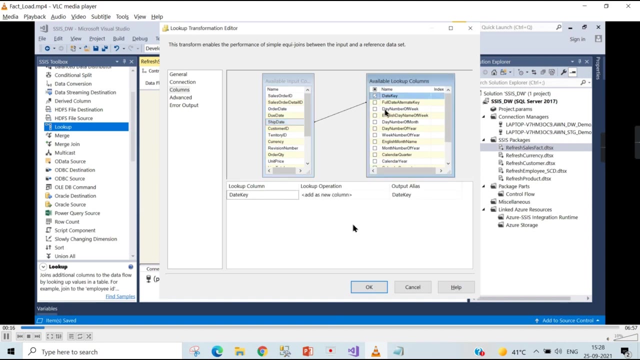 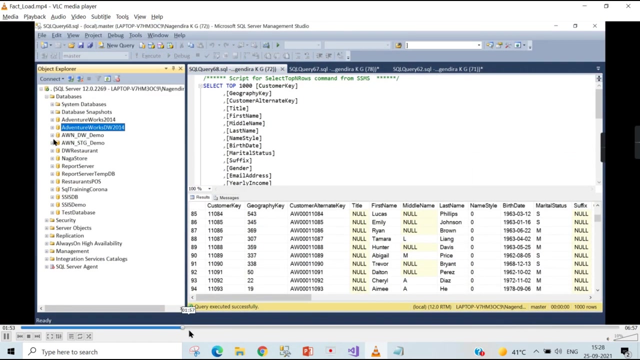 so how i have developed you can see here. i will quickly play this because i do not want to waste your time in doing this. so you see, i'll choose dim date order date here. so choose the and i will rename it to shift date key. let me skip some more time, so in between i might have faced some issues as well. now you can see. 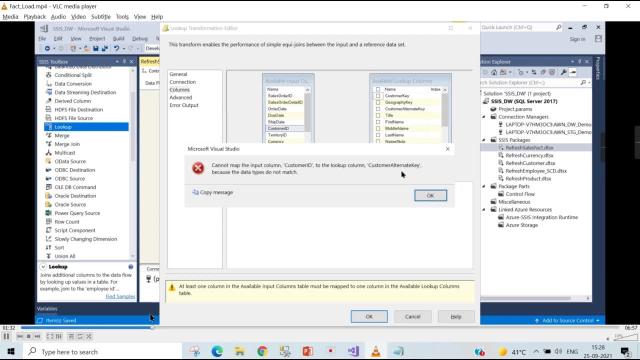 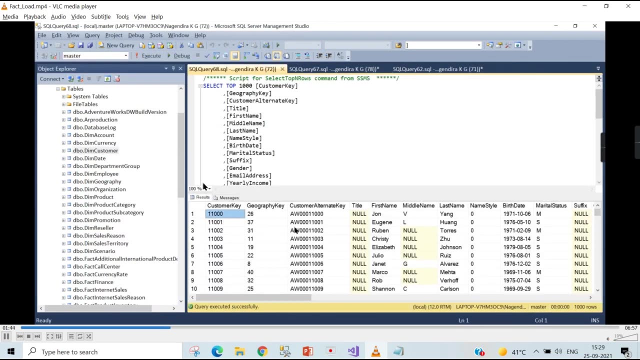 here some of the issues i faced in the customer table. now let me play it so dim customer, i'm trying to map when i place it. i am facing issues like you cannot map because there is a data type mismatch. so how i troubleshoot it? just go and query this and you see alternative case aw0011084. 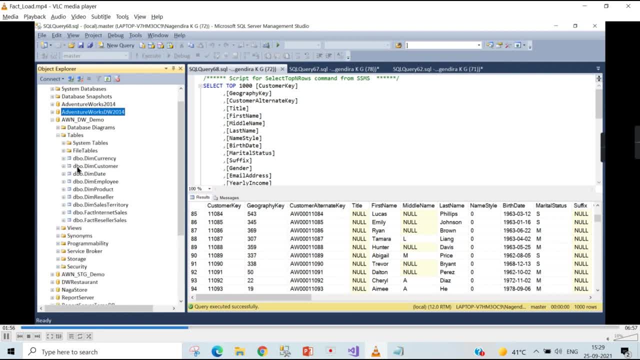 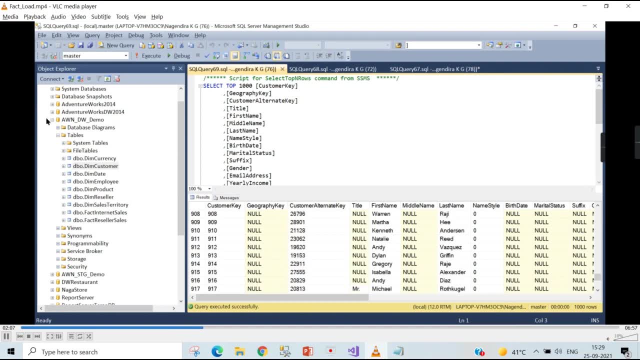 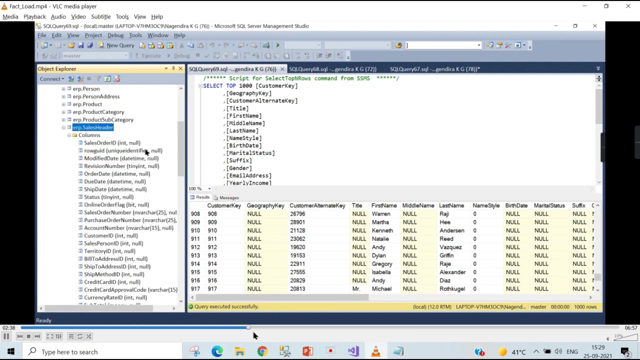 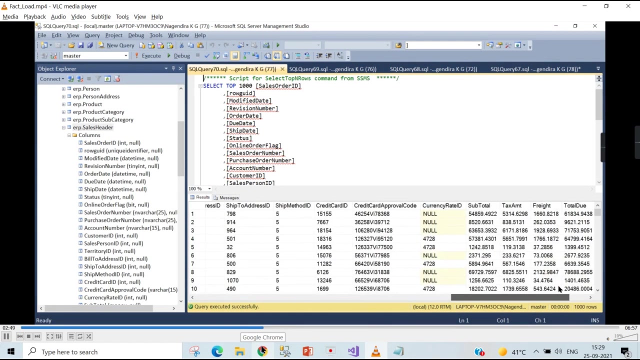 but in my customer alternative key in the dimension table is this one, 220 something. it's coming like integer value, whereas in the sales header- right in the sales header, customer id is there it is integer. i'm trying to find that column here, the customer id, okay. 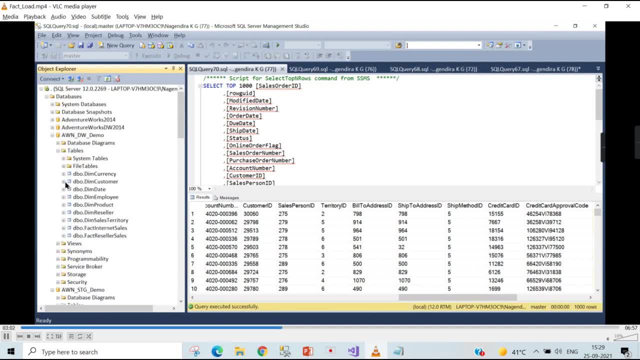 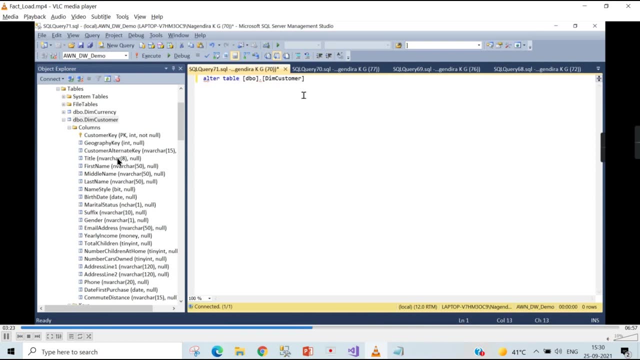 so the customer id is here, but alternative key, the customer alternative key here in the- uh, i mean dim customer is actually the. it is correct. basically, customer alternative key also contains the actual value of the as the number. but i define the data type wrongly. okay, that is how, if the error happens there, i am fixing it over here. 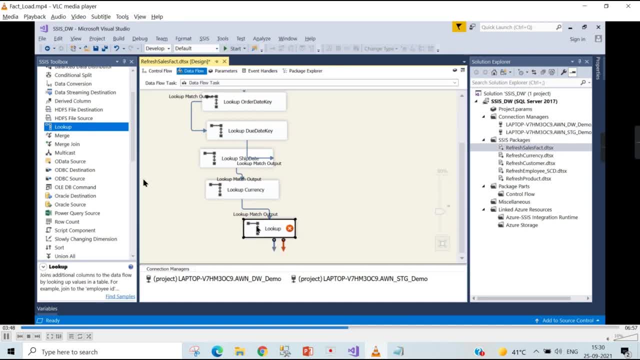 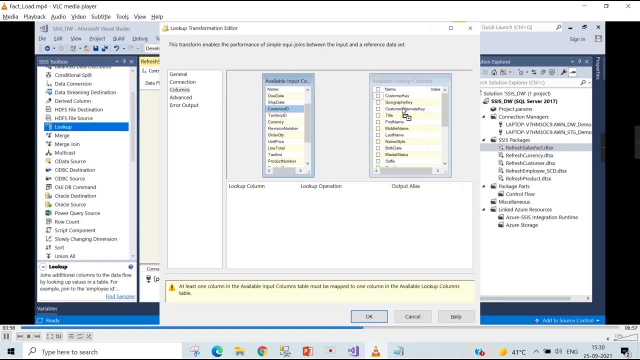 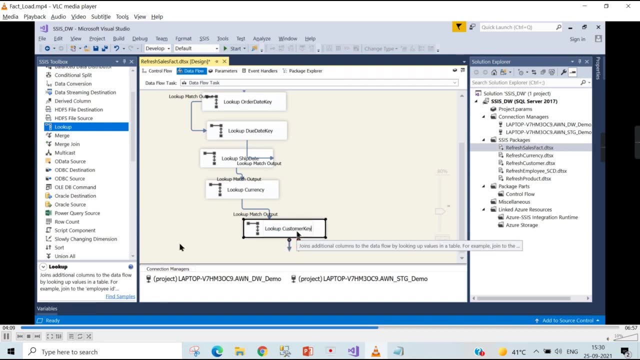 okay. so this kind of issues even i face, so it is not very simple. like i am showing it in this demo, i have created these things in very few hours. usually to build um these projects it will take a couple of months to design one data marks and everything is manual. you can see if it contains. 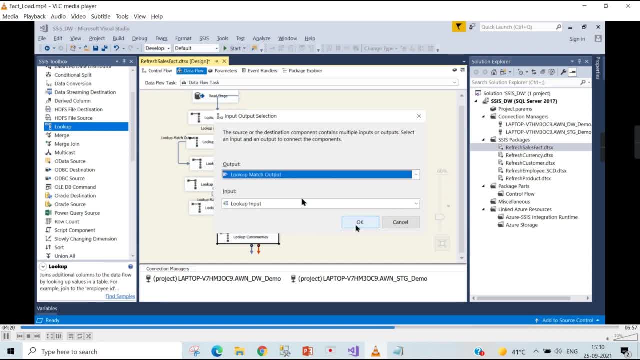 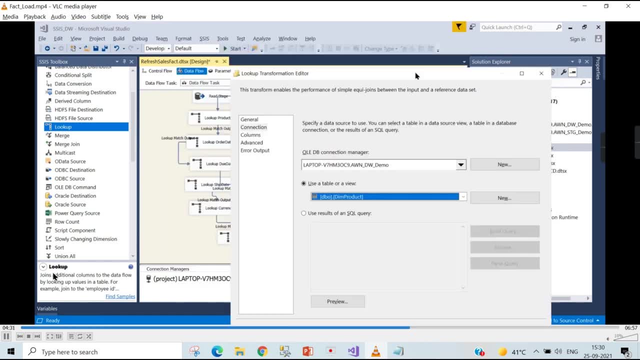 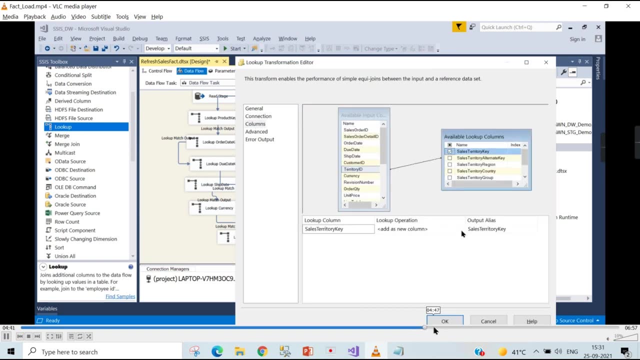 10 to 20 dimensions each thing. i need to map it manually as you can. you are seeing i'm once i fix that customer, i'm going for another dimension dim product here. so this is not as simple as that. i mapped it wrong column, i think. yeah, i choose the. 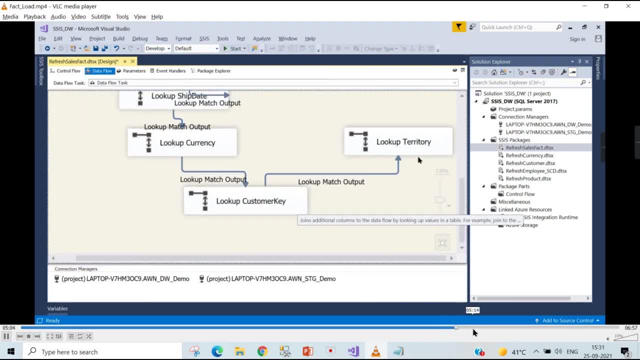 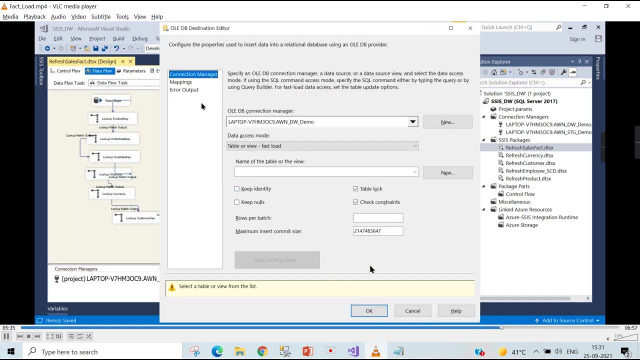 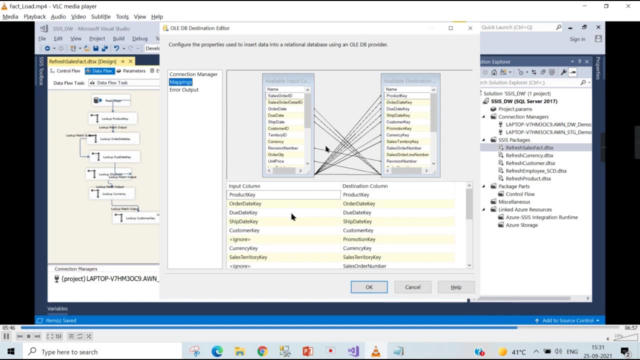 dim territory. finally, i'm loading into your fact table fact internet sales. now you can see all the columns having same name, so it has matched. so when there is no matching column, you need to map it manually. so this is more or less a manual work that you need. 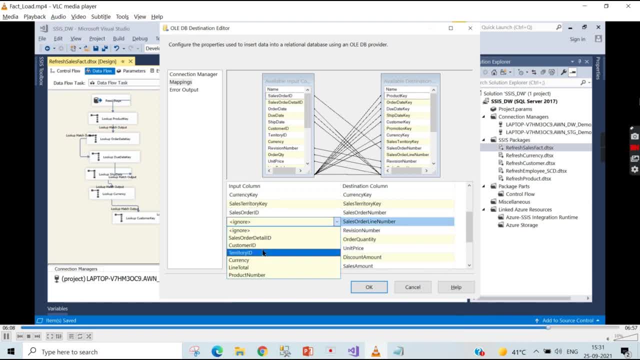 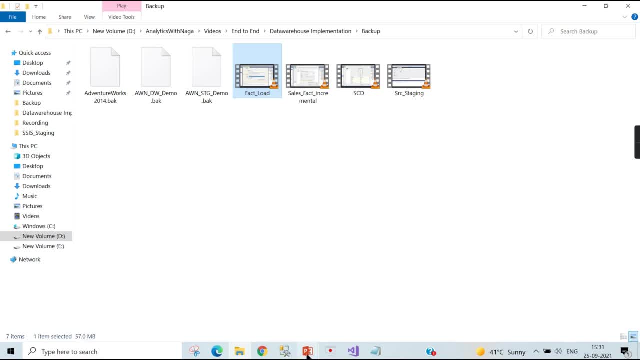 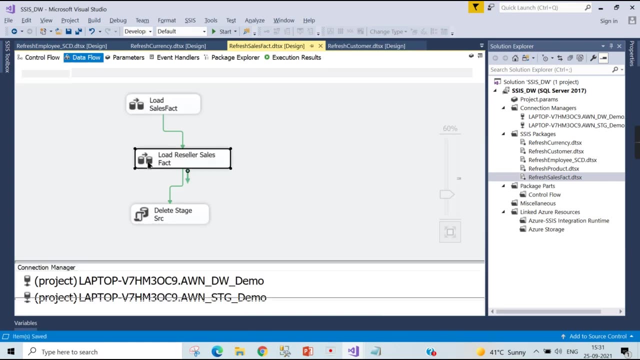 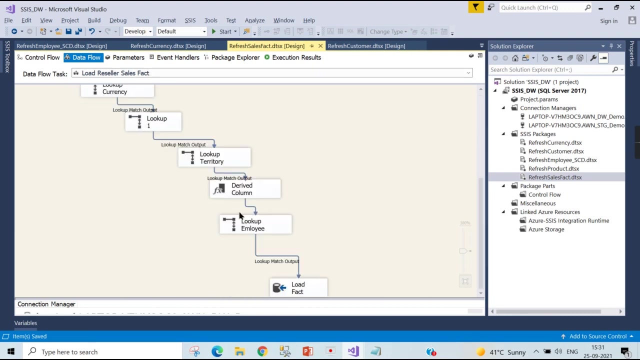 to realize it for each and every fact table. i hope now you understand how i am mapped it. let's try to run this package so that we can. this is how i developed similarly- uh, i have developed this- reseller sales as well, and everything is same for the. 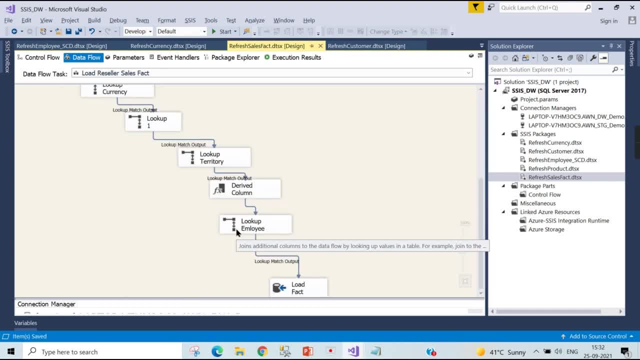 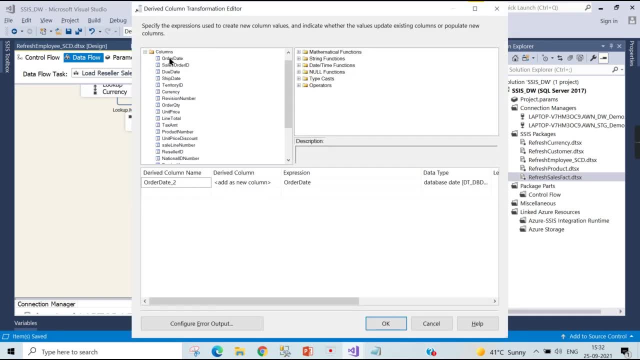 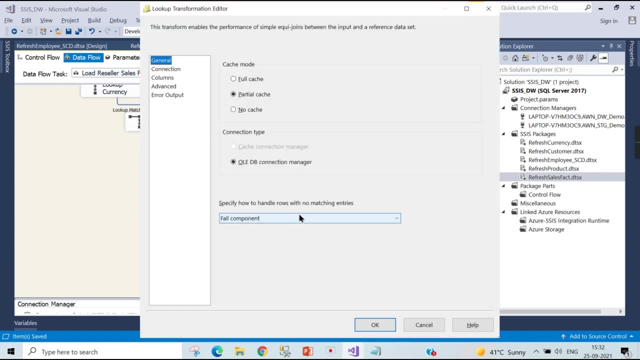 recently sales as well, but how i can do the lookup for the scd2 column? that should be based on the date. so usually you need to have the duplicate column for the lookup column. i mean the date. so i will have a duplicate column here because in the scd2 column what you need to do here is 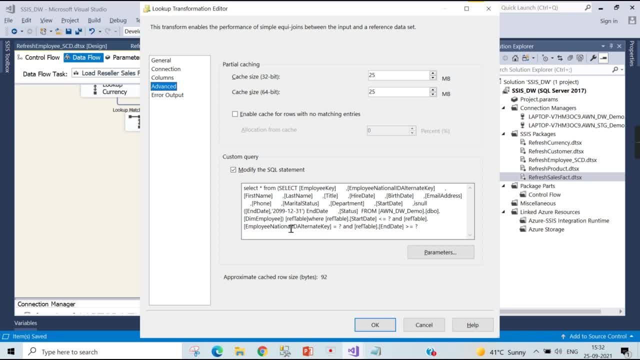 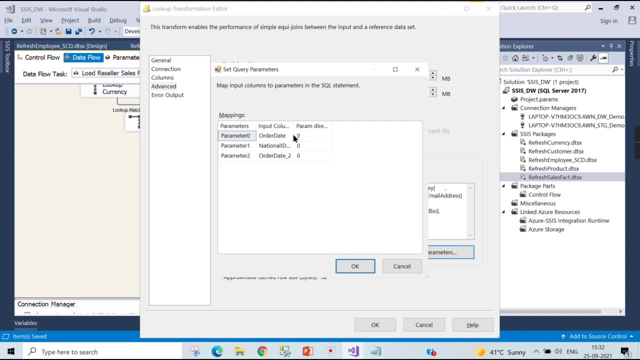 you need to do little advance. the employee alternative key should be filtered, right, it should be looked up, and then it should be based on different start date and end date. right, your transaction date, order date. so your order date is one parameter and order date two is another. 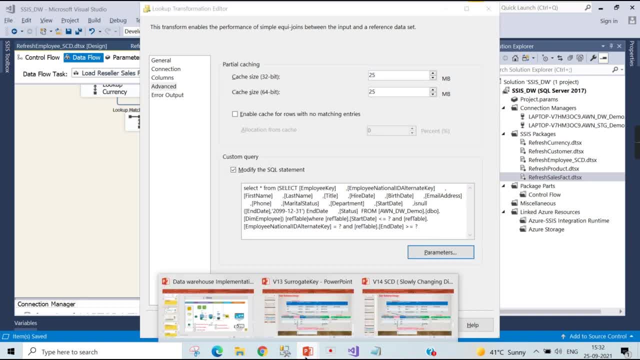 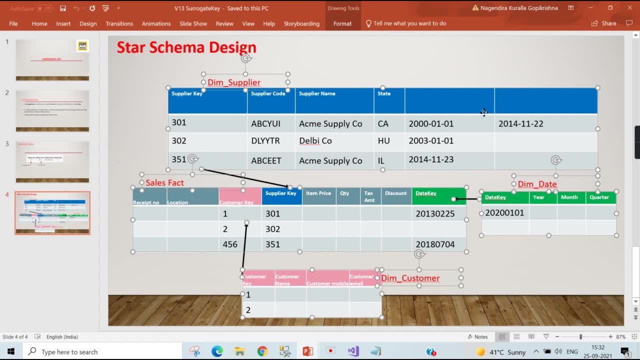 parameter. it should be checked between start date and end date to get the lookup value. you remember i explained so far. this is the transaction date. it should be looked up in the start date and end date, then get the corresponding key here. so that is the logic we need to implement slightly. 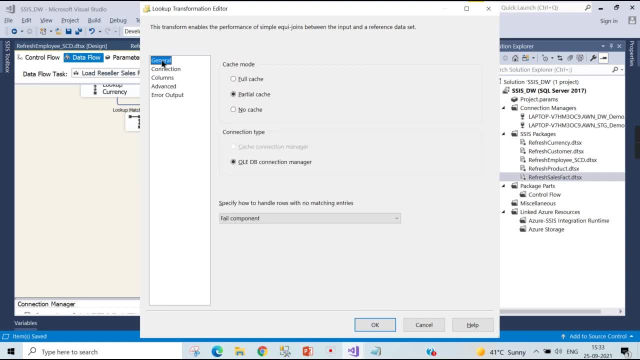 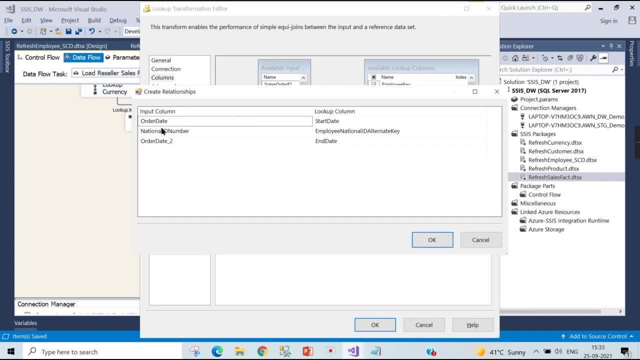 differently in this. you the lookup tables using some options. so you need to keep the partial catchy. you need to write some queries here. then here in the mapping you need to use the lookup column. then the order date should be repeated, the duplicated, using a derived column. then here in the advance you need to use this kind. 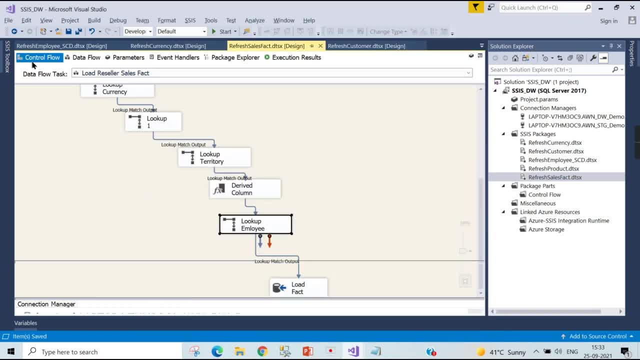 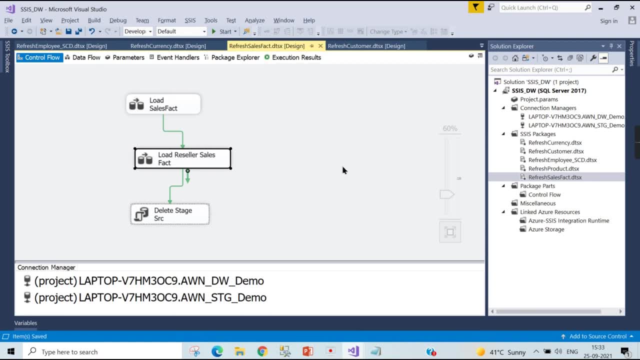 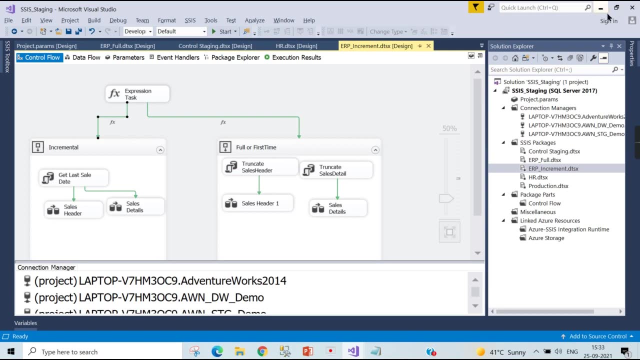 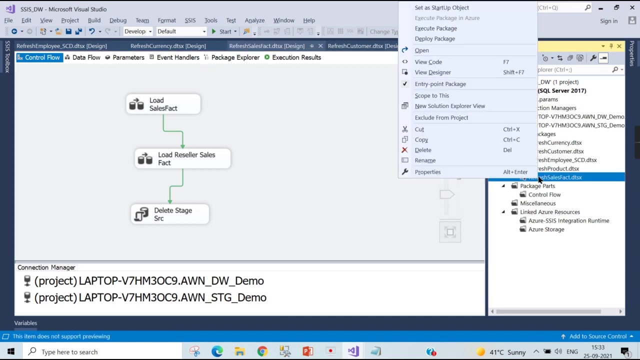 of calculations. this is the only difference in case of scd2 lookup. so these two things has been done. once it is done, now the fact table population here. what happens here is like: now i'm deleting it in the fact, okay, i will show the incremental load once i update it, once i completed the flow. now you go and refresh or 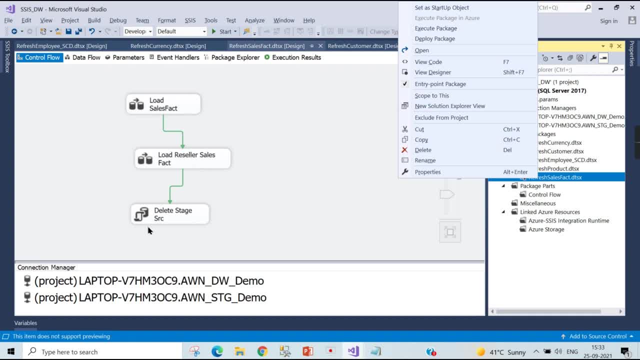 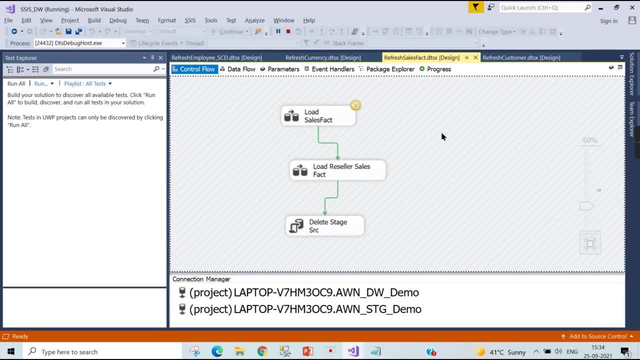 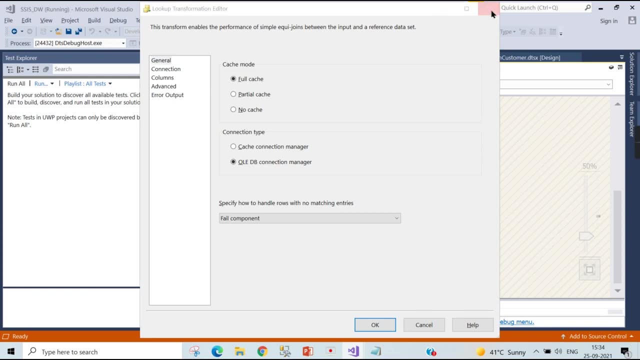 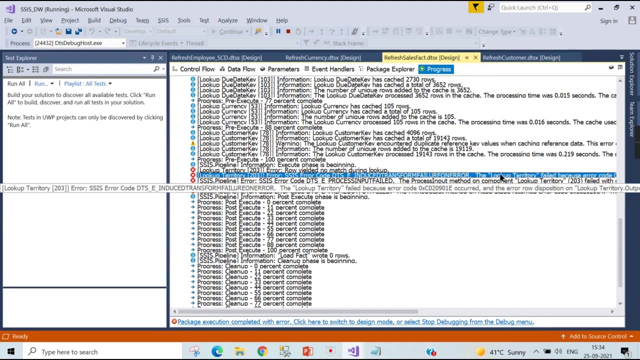 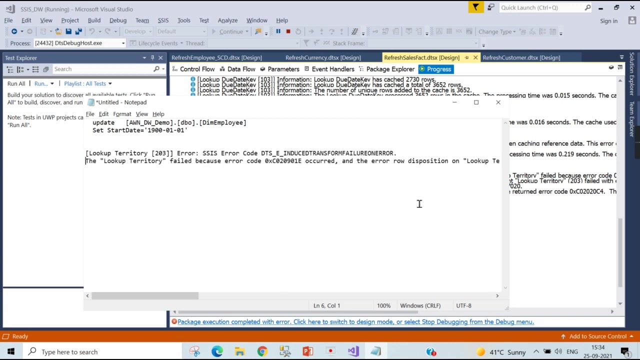 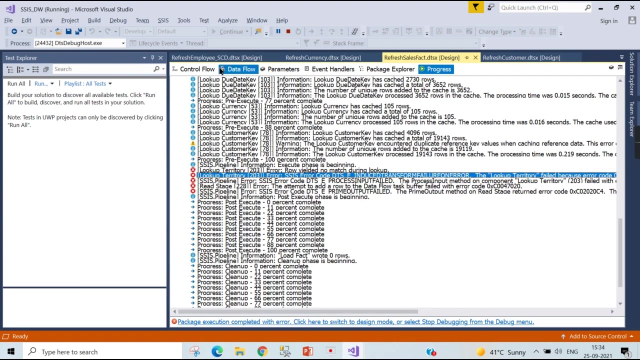 execute this package. then once the fact table is completed, then i am deleting the stage source. i'll tell you that why i'm doing it here. so there is error, i am not getting any shock because i know that might be some issues while executing it. let's fix it together. so these kind of issues always occurs. i think we didn't populated the. 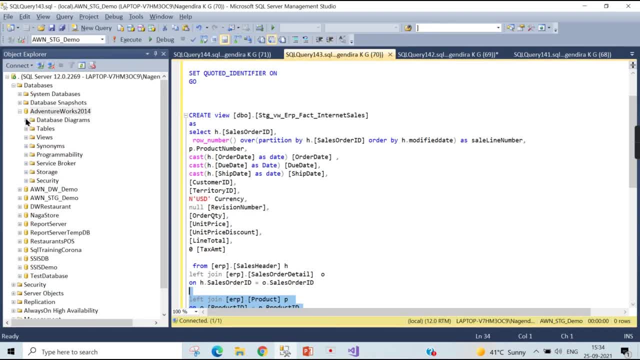 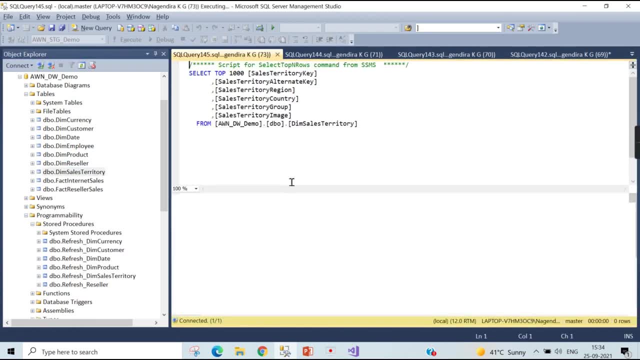 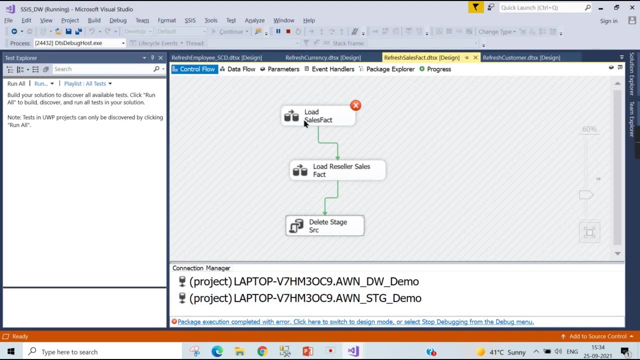 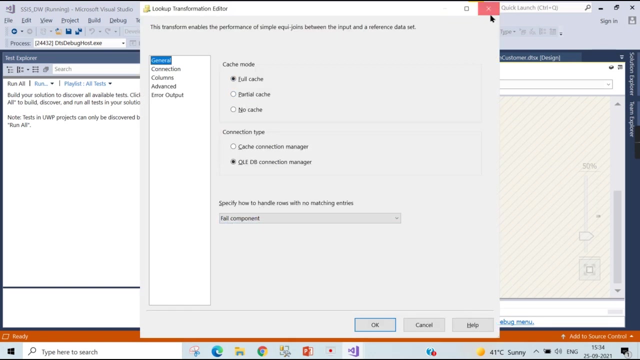 territory key. i mean, that is that might be the reason let's go and check it out in the data varus. okay, there you go. so because i know, because there is no data, so why it has failed is to explain it to you- that sales territory, when there is no match, okay, what i said: fail component. this is very 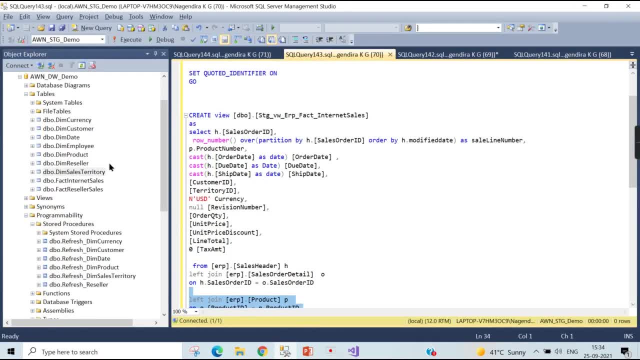 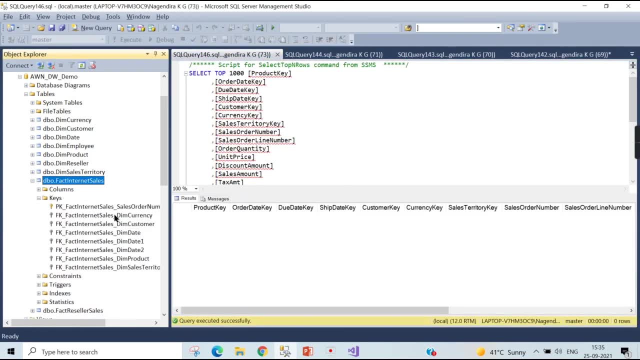 important because if you skip it, it will populate in the data varus. it will not be in the data varus. the fact table as null values. you have defined the keys here. everything is a foreign key reference, so you are ensuring the constraints right. the data warehouse data is consistent. that is the 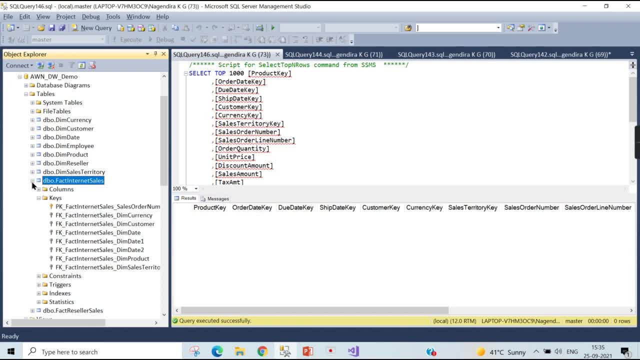 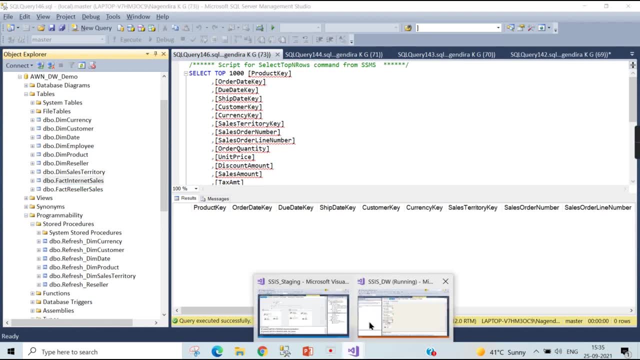 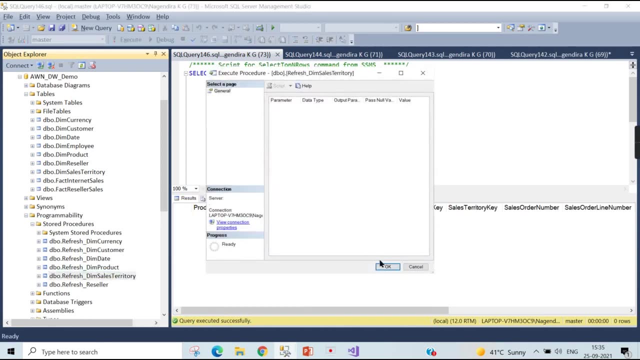 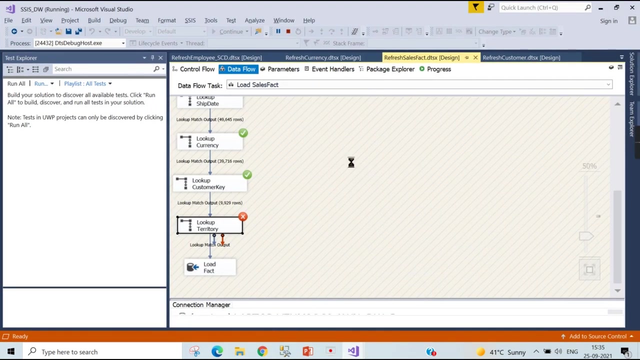 main objective. if you skip some territory key, then you are populating a faulty data. you cannot report under sales territory, so it is better you keep it failed so that it you can catch some issues. so dim sales territory. i will execute it now. there are different ways you can execute. that is fine. now you go and execute it. 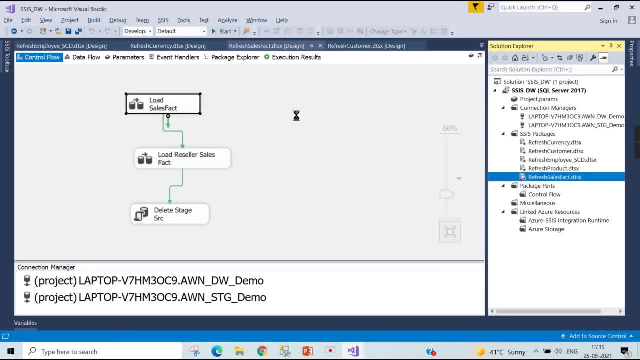 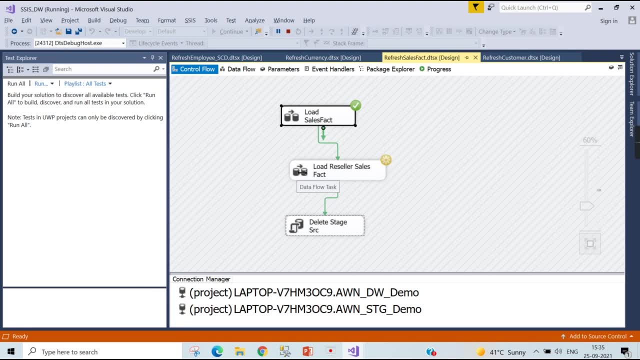 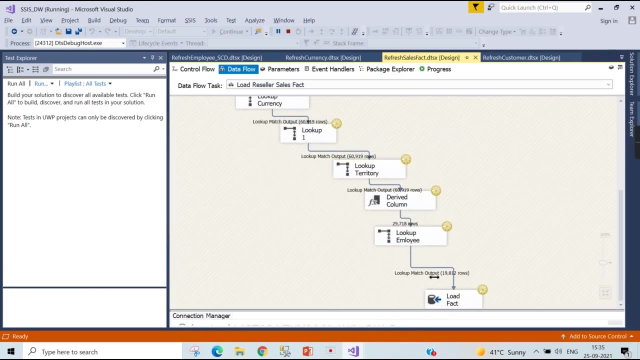 this package once again. so even we face issues. it is doesn't matter who develops or, but you should know why it is failing and you can able to troubleshoot it quickly. so reseller takes some time because of this. lookup is little slow and we can wait for it. it will complete in another few. 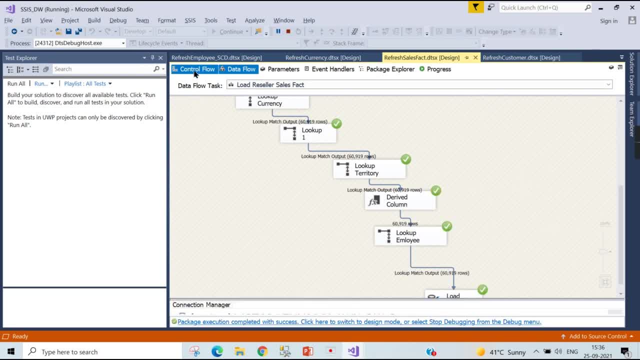 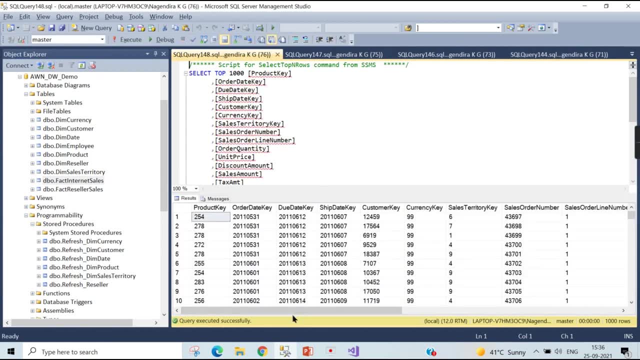 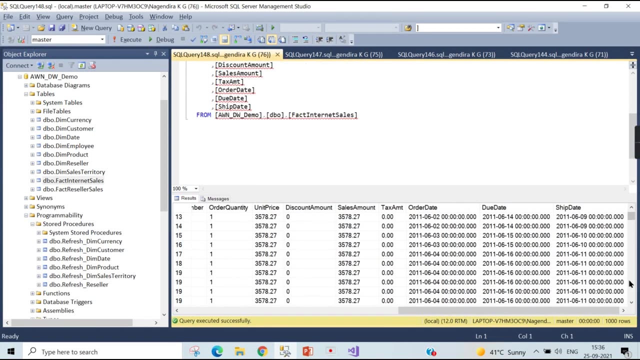 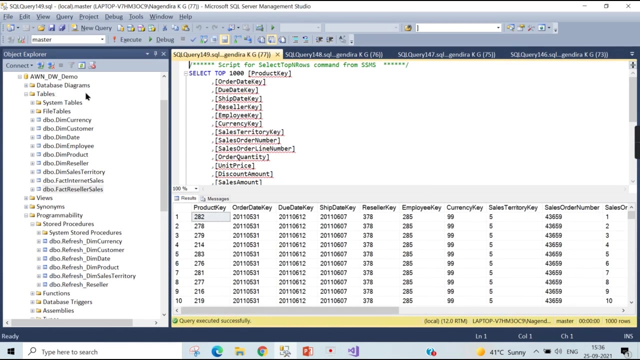 seconds. okay, it's done. it is green now and i've deleted this source. now you go and check this fact table, where you get all the surrogate keys populated, along with the measures. so this is how you have designed your data varrows and populate the data varrows using: 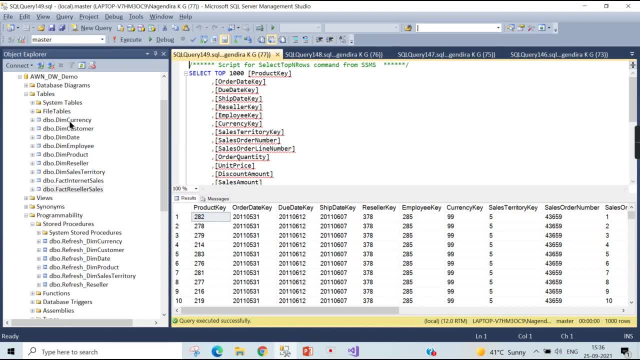 the dimension and facts. so you have your dimension populated first, followed by different fact tables. we are done with this population and have some of the things to cover regarding incremental load. once we are done, we will move to our next step: how you can create reports on top of database. 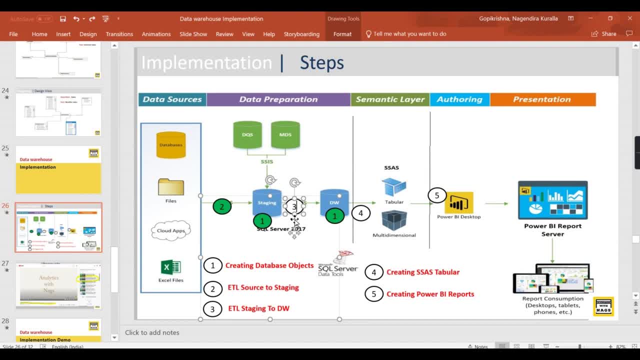 now we are done with this step as well, like we started loading the data from staging to data surgost's. first we loaded the dimensions, then we have done the fact table. so this is the cycle we need to follow. uh, like whatever we have seen so far, that is created. 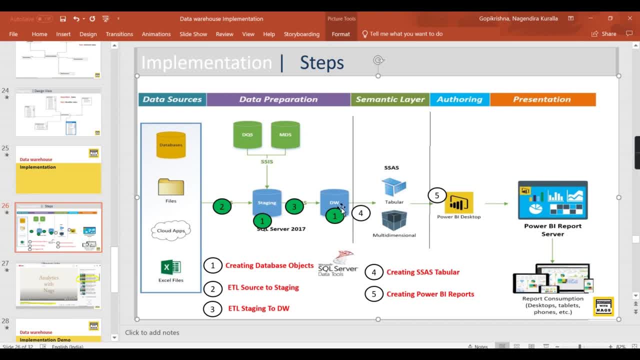 staging data and loading from source to staging, staging to data arrows. now, this is fine for the one single cycle, how this cycle will regularly happen, right? so for that to understand, we will take two scenario: one simple dimension refresh, another one for the fact, incremental refresh. right, so we will try to insert one record in. 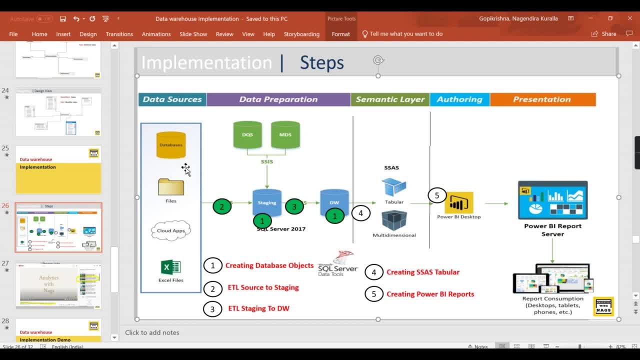 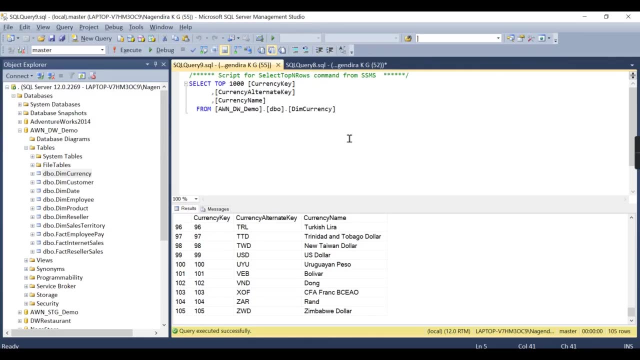 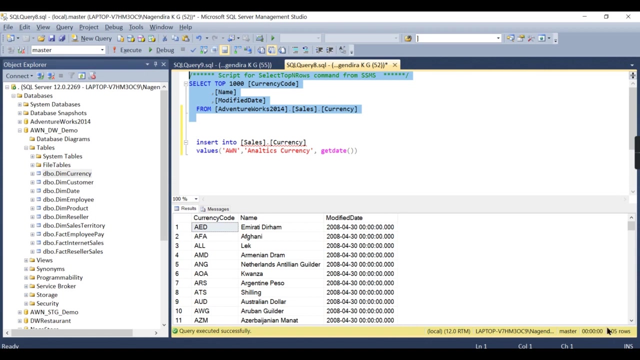 the currency in the source. okay, some new record added in the dimension. how will it will reflect in the data arrows. then we will add some more record in the fact table and how incrementally will extract it. that is what we will see right now. so, to begin with, in the source. now we have 105 records for the currency. you can see. 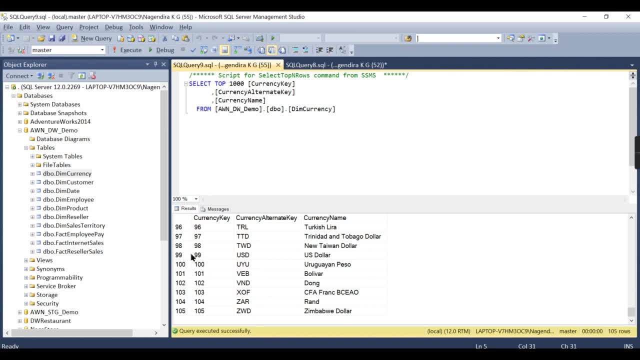 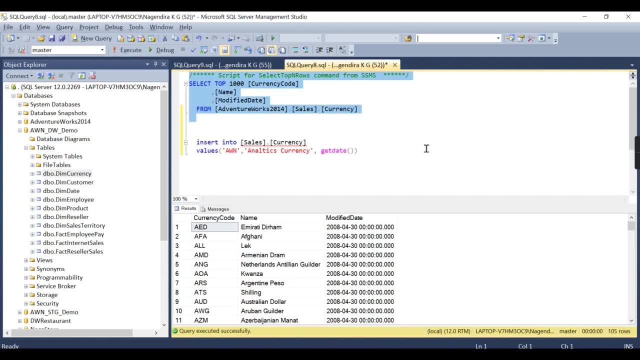 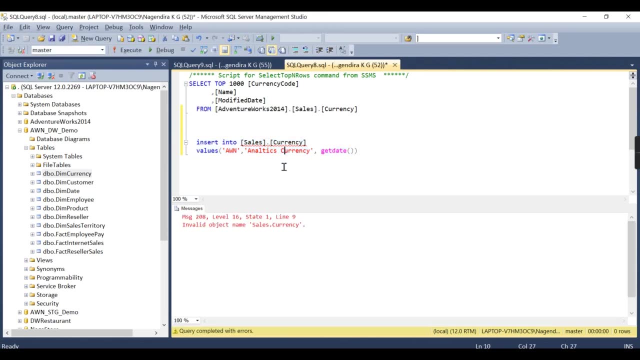 it here and in the dimension once, as we populated. this also contains 105 records. you can see it here. And now what I'm going to do. let me insert one record here in the source, that is, in the currency, So it should be with this database name. Let me add that database prefix. 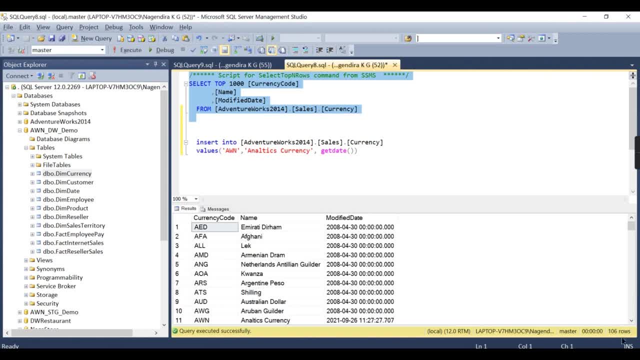 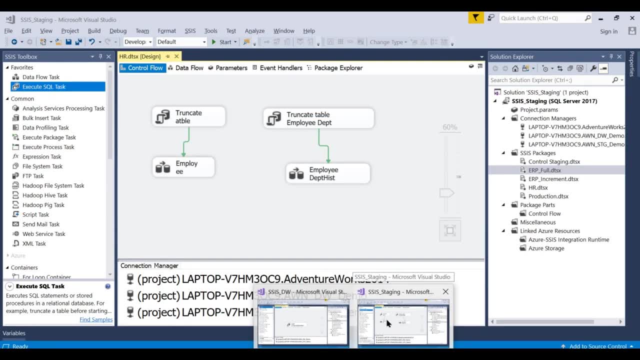 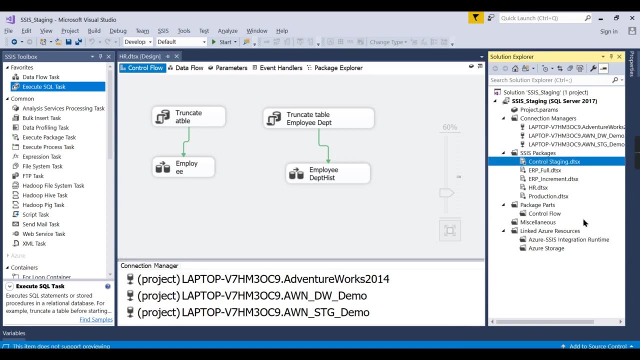 So now in the source you have 106, but in the data warehouse we have 105.. How this will reflect. We need to run this packages right one after the other. Basically, you will schedule this control packages, then that will call internally. Now we are manually running it to reflect the data. 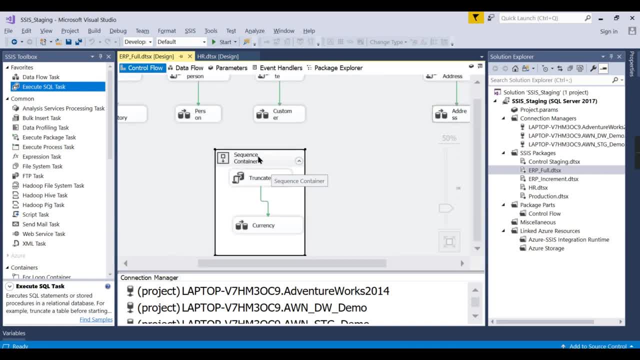 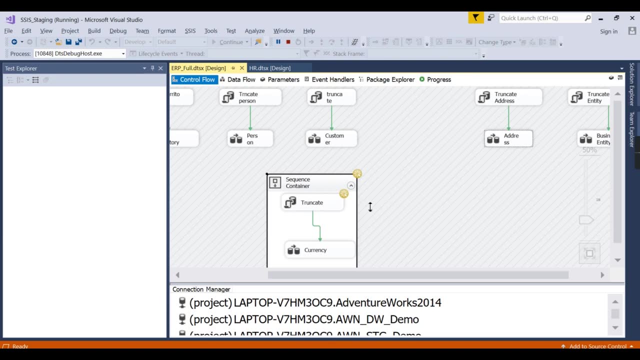 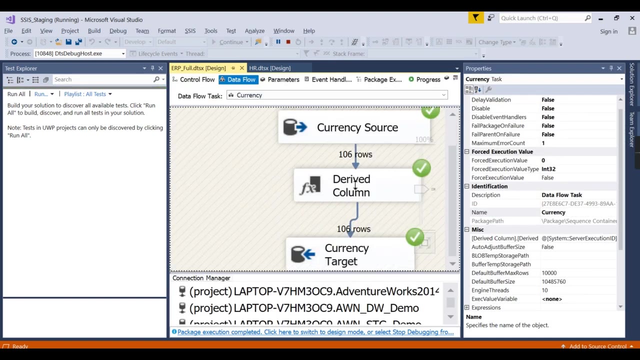 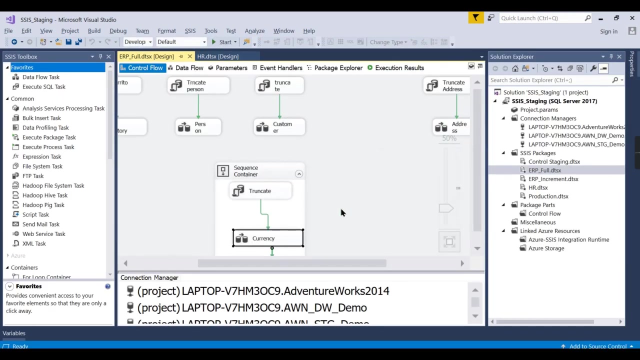 So the currency, let me run it here. that is in the from source to staging. I will call it, I will truncate and reload. So I'm doing it right now. So this will get me the latest snapshot of the dimension. that is 106 records in the staging layer. So it is running it. So let us go check. So it is 106 records, It is done. So you will not do it manually. Basically, as I said, you will schedule it. That will call this package. So this will have 106.. Now it has loaded in the staging How it will reflect. 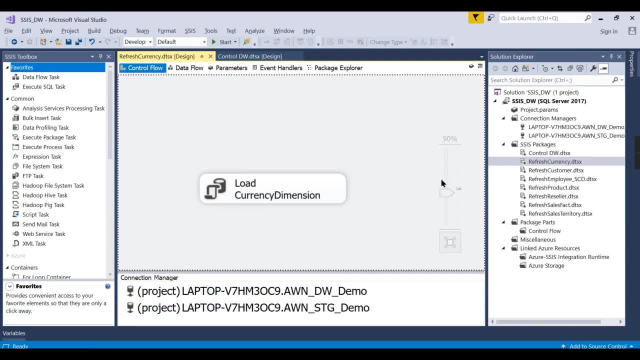 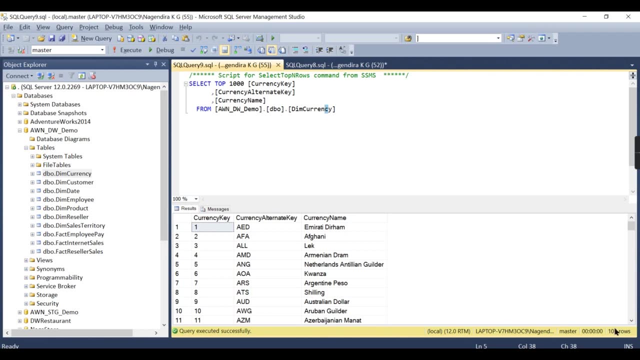 It will reflect in the data warehouse. You go and refresh this package here that is load currency. Once you refresh it it will call the procedure that we have already seen. So this is calling you the procedure. Now you go and check your data warehouse. here It was 105 before running, I mean before doing all these two packages running. Now when you query it, it will become 106. So that particular entry, whatever we insert at AWN- and I'll take it- 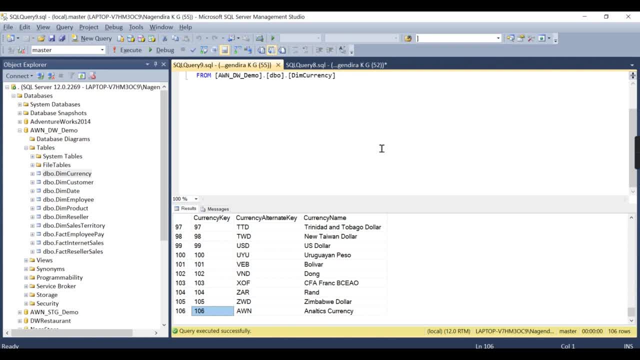 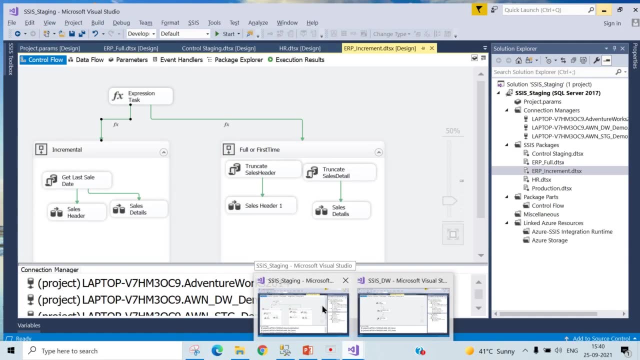 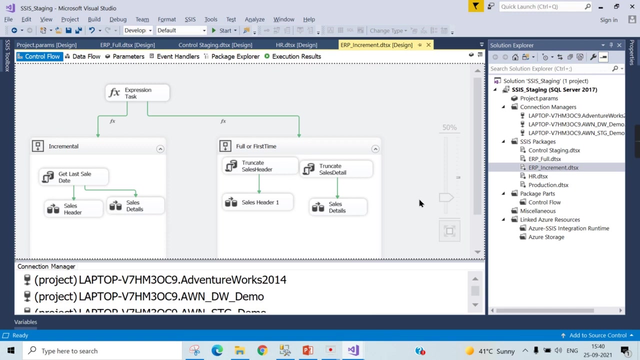 106 currency that has been introduced. This is how it will flow into your data warehouse on a daily basis. Let's check it out. The incremental logic for the fact: What is incremental load that we, most of them, ever like? now we have loaded the entire data set. So incremental load can be for any table. It can be for dimension and fact. I'm going to demonstrate for one of the fact table. 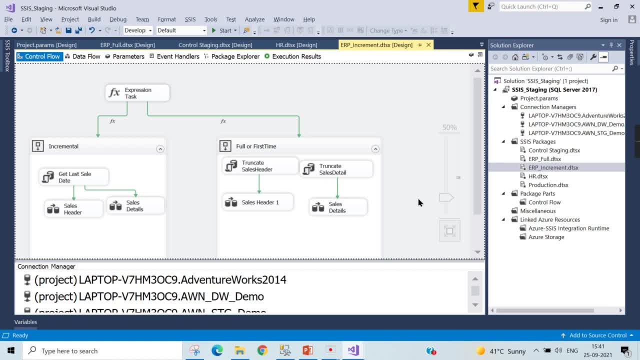 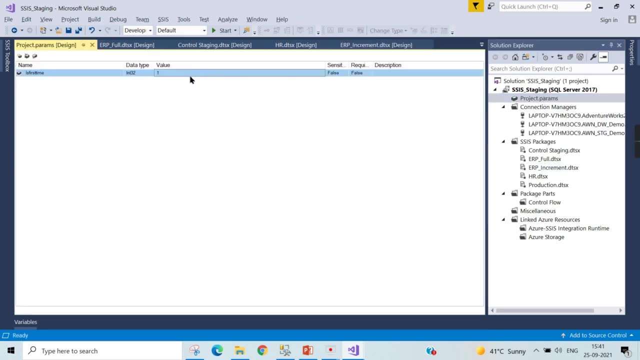 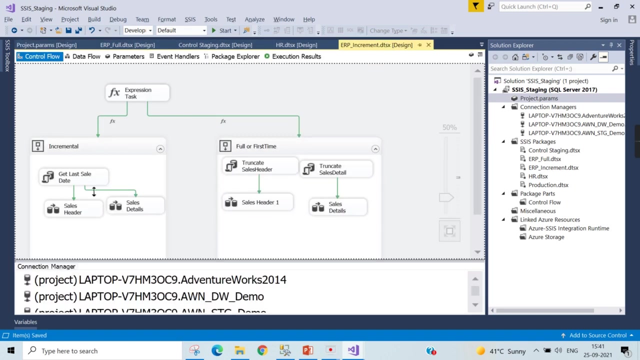 Then we will decide on how it can be implemented for I mean, then you can implement for any other tables. So, as I said before, this ERP incremental is meant for both first time load as well as the incremental load. Let us change this to his first time load, to zero now, So that package will run for incremental, this flow, And you can see here what is the logic I have written. It is very simple. 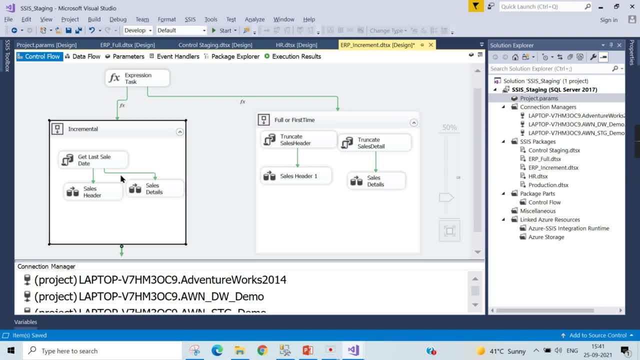 Very simple logic I have written here, but typically in practical implementation the implementation will look somewhat similar but little more proper way. OK, but this is the logic of incremental. So now, from the day we have started extraction until some date we have extracted the data, post to that There are some updates- are incremental records Only those records we need to be. 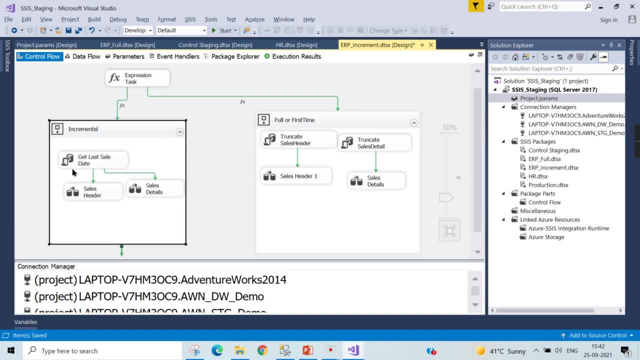 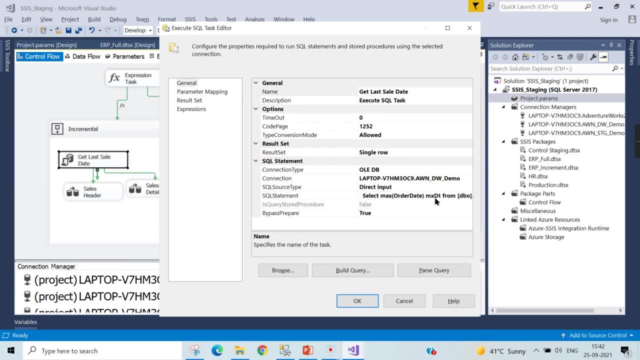 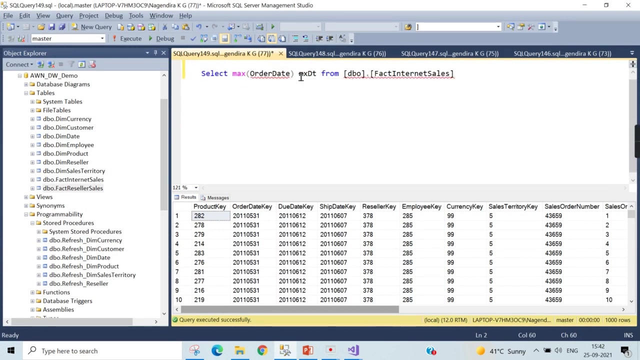 Bring it up. That is the incremental data, So how I know. So, whatever you extracted, now, right, you need to get that maximum date. So from where you will get it? you will get it from the fact table, The fact internal sales, maximum order date. OK, that is what it is. So if you are not able to see it, let me copy it and put it in the SQL window. So select max order date, max date from fact internal sales. Then, once you get that, 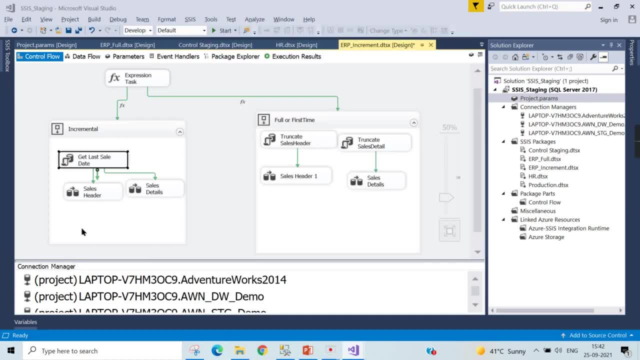 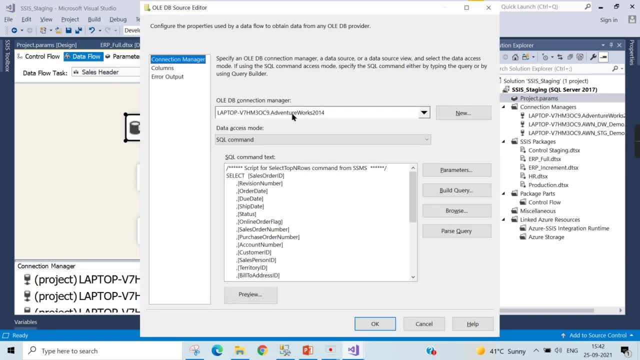 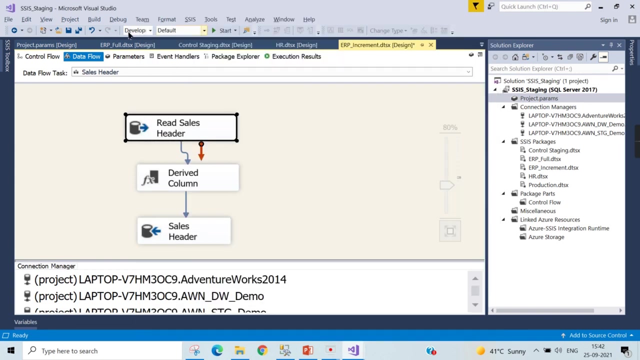 Using that column max, that the sales order table has been read from the source system. You see adventure works 2014, and then you put the question mark order date greater than from the where we have lost extracted date. So that parameter, you will map it here. OK, so this is what you need to learn about the SSIS, like how you can get the value. 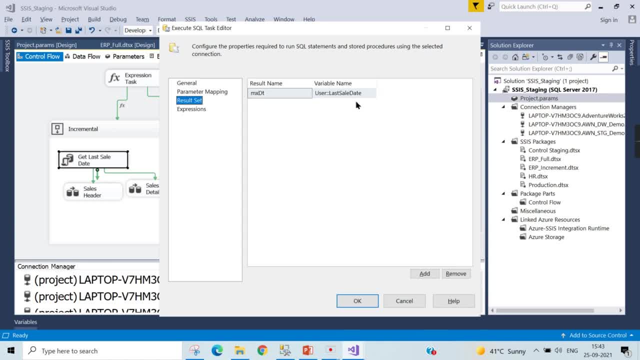 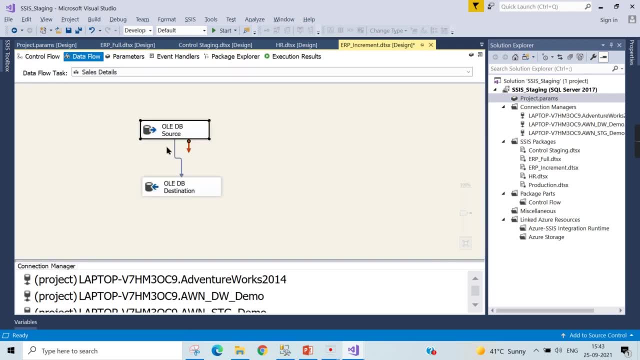 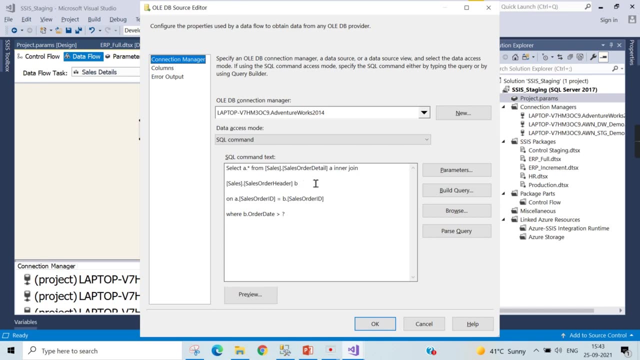 This value. you need to get it here. You need to set this result property, assign it to a variable. that variable you will use it in the query. Same way you will need for the detail table as well. So you do the inner join of header table, because only in the header you have that order date. So you will do the inner join and then, based on the header order date, you will get the detail table as well. So this is how you will implement. This is the core concept, but proper way. 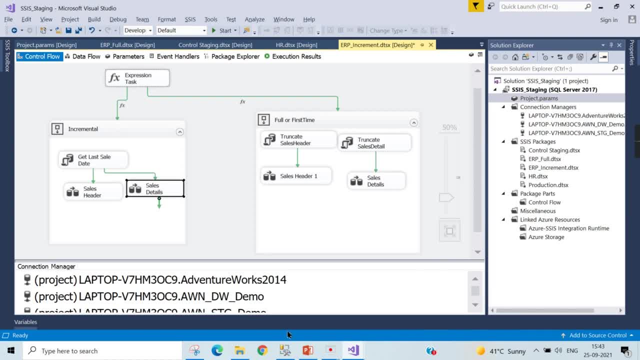 So the way is like for each table: you can maintain it in separate table, like watermarking table. So say, for example: this is sales fact, This is the last date it has been extracted. You can maintain it in a separate table. from that table, You can get it and after extraction you can update it that table. So that logic you can maintain. But for simplicity, this is the logic I've written. Now, when I run this particular incremental, whether it will have a data or not, it will have a data. 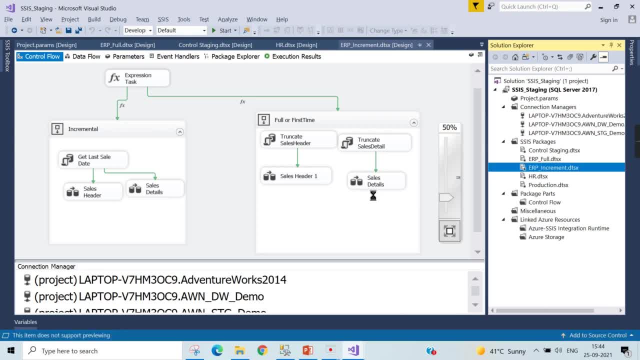 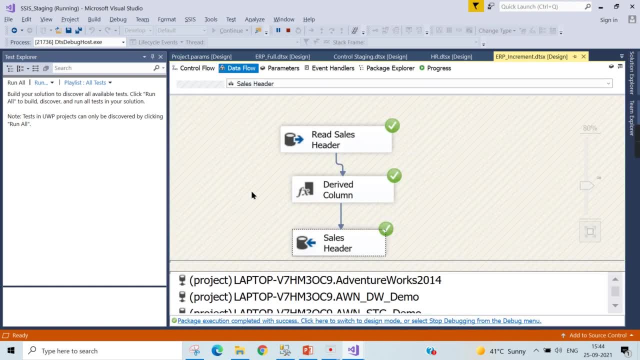 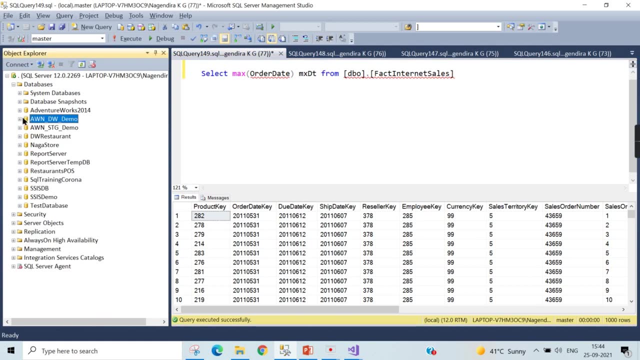 In short, it will not have any data. Why? Because all the data we extracted in source. we do not have any updates yet. So you see here it has run in this flow, but there won't be any data. You see no rows affected. So how we can? either you can insert some data in the source or what I'm going to do, I will do some updates right: Update in the data. Then we will check it out whether those rows are picked up or not. 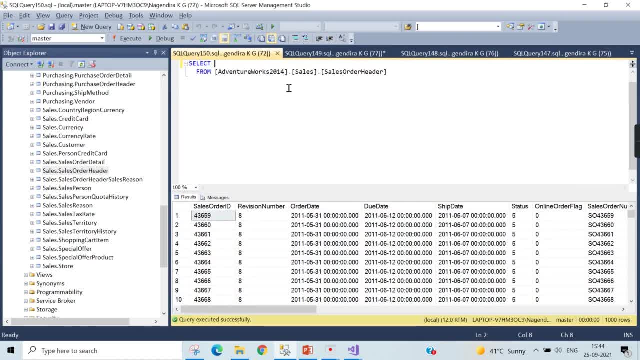 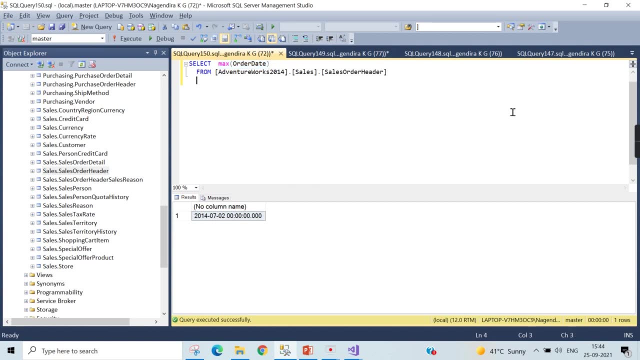 So let me do that- get a query like maximum order date. okay, now this is the maximum order date, then what I will do, I'll just slightly increase the one day here in the header, then we will see how it works. right, only those records will be pitched up picked. 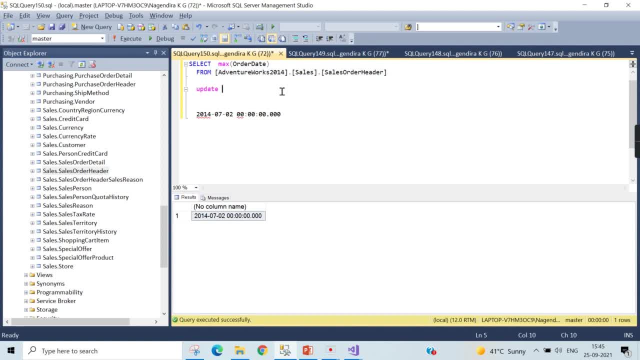 up from the source system, so update this one, then set order date. I do not have any incremental data, so I am just updating the existing records. are considering these records are newly added. okay, that is what my assumption is, so I will update it to three. don't forget to click on update. 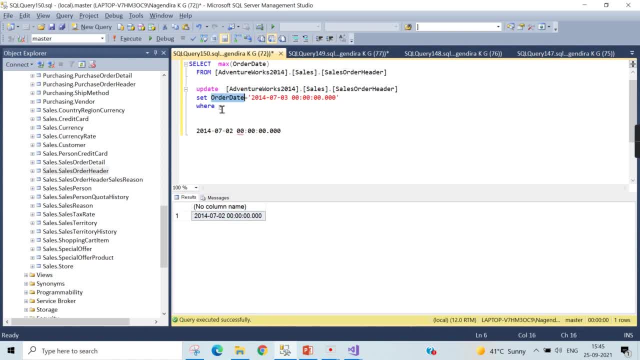 please do not forget to put the var condition, otherwise the entire thing will collapse. order date equals this. okay, this is the condition here. so order date. there you go. so there are 40 records got updated, considering these are the new records added in the mobile CAL jaa log. now again, I will open this update and hard drive set up what I feel that I need: 10 votes, knowing that after all the records have been pastry reorganized, I cotton tight. what classes currently uninstalled? so you get to replace edit access trim, and then I will fuckin Everest. and then is the next step. so you cannot do. 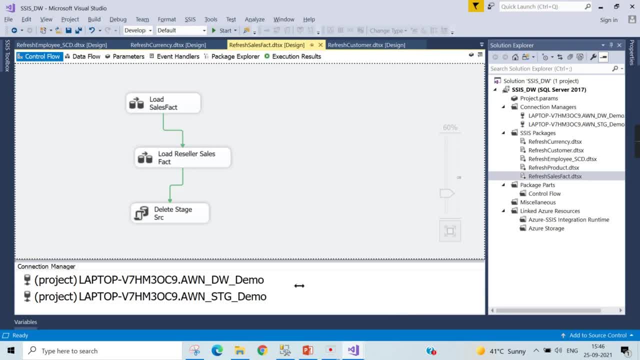 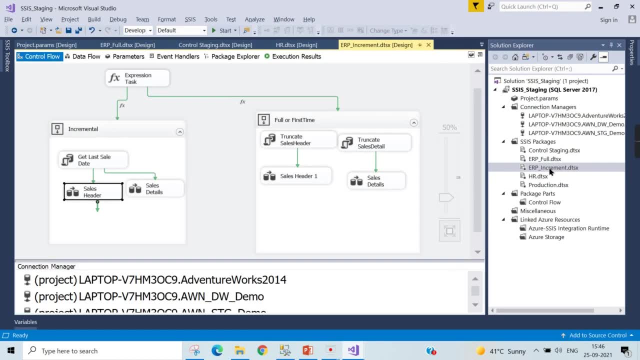 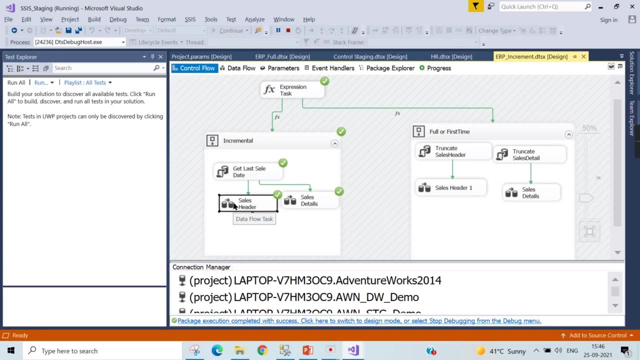 the OLTP system. so when I run it going forward in, either I can schedule it in the SSIS or whatever scheduling tool. right when I run it, only those records will be fetched. I am doing it everything manually, but in real time we will do it in the some other place. I mean to say SSIS agent. so now you can see those 40. 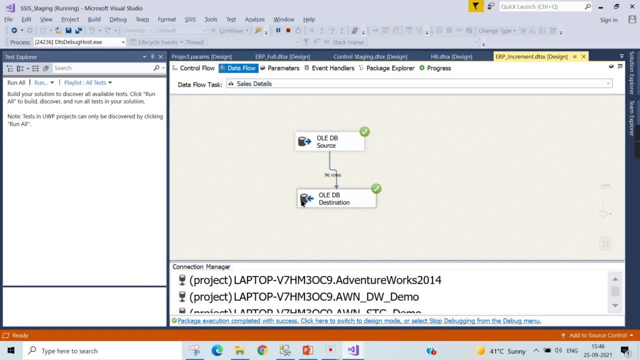 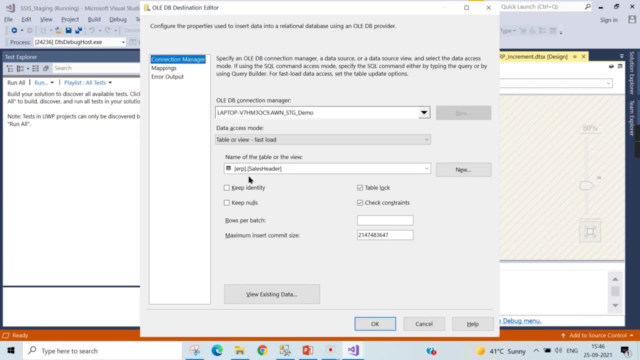 records only picked up here, even details. it will be more because details joined with the header in header only I have a date, so whatever respective records for those 40 will be picked up in the source and then it is in the staging. okay, now what is the target? you can see this is ERP cells and it is a staging database. 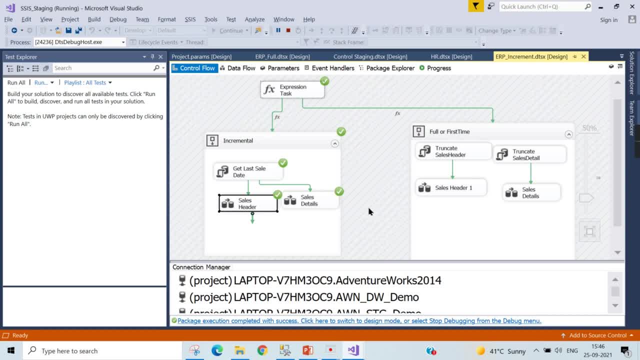 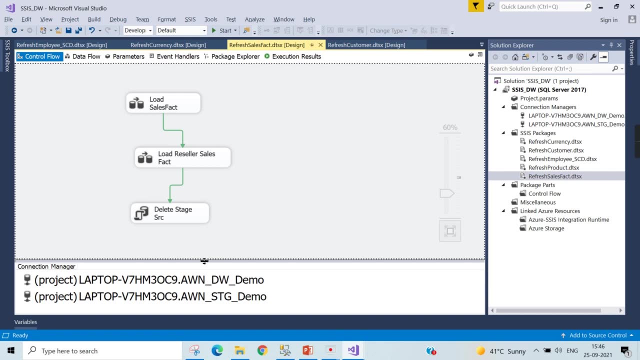 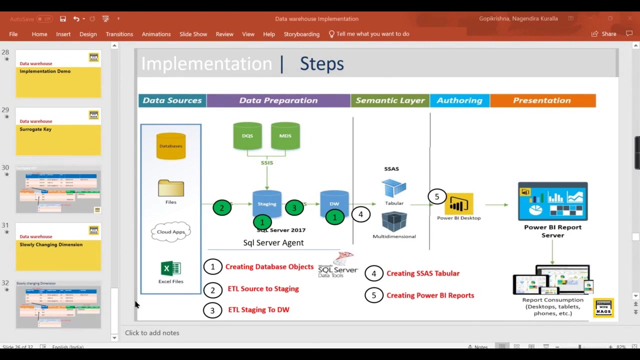 now it is not still at load in the your fact tables. okay, now, in order to run that fact table, you need to switch back to data arrows. so this is not run everyday manually. if you run it now, it will load the respective incremental data only. let's take a park. 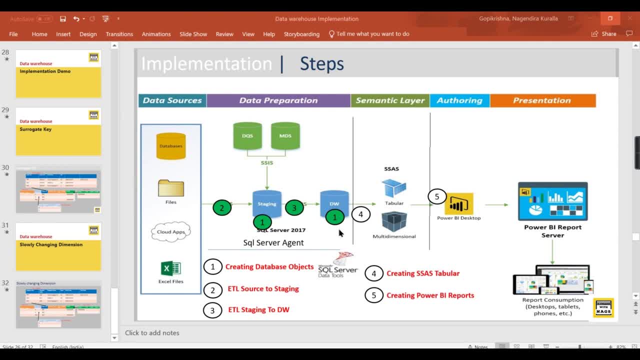 here and let's summarize whatever we have done so far and something that are still missing in the data virus layer. once we discuss this and complete whatever we do want to do in that errors, then we will move on to 4 & 5. so typically we have seared the data varus, so we will move on to 5 and 5 and so typically we have seen that data varus is not working. so we need 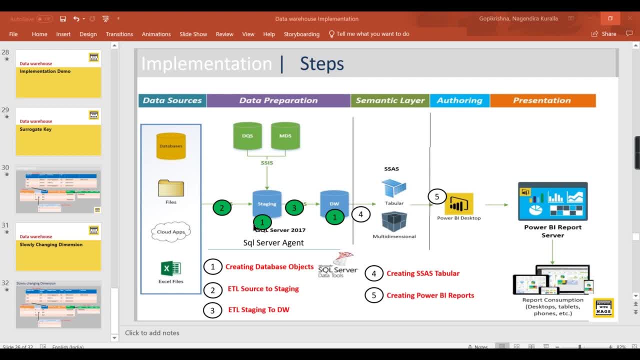 in the complete flow how you can build like staging, data warehouse and populating from source to staging, staging to data arrows. this orchestration is done in the ssis using ssis or some sql queries or procedures. you call the procedures in ssis to move the data between. 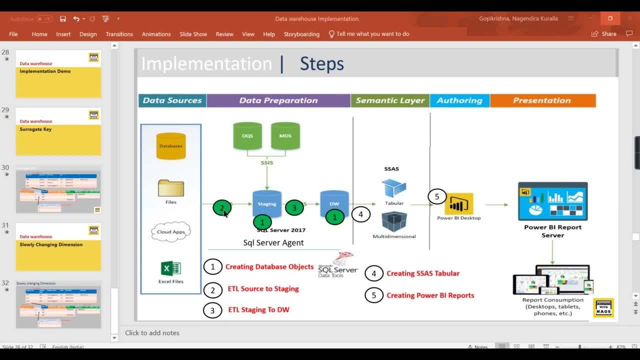 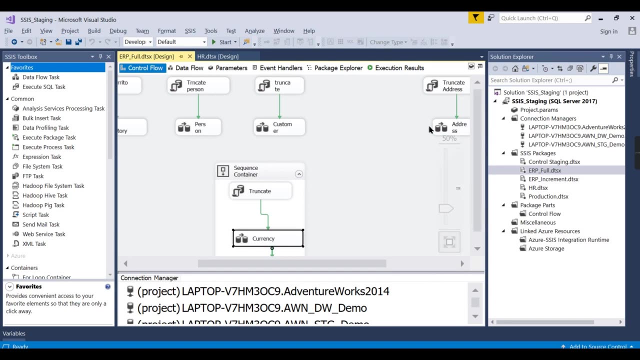 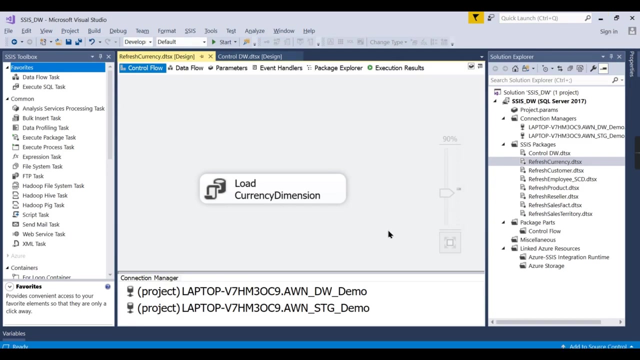 different layers and this ssis package to be run regular basis. how we can do that. that is the missing part we need to discuss now. so that is nothing but this ssis packages- whatever we have developed using these packages- right, these should be stored- are deployed in the ssis integration catalog. so what is that? in the sql server itself? 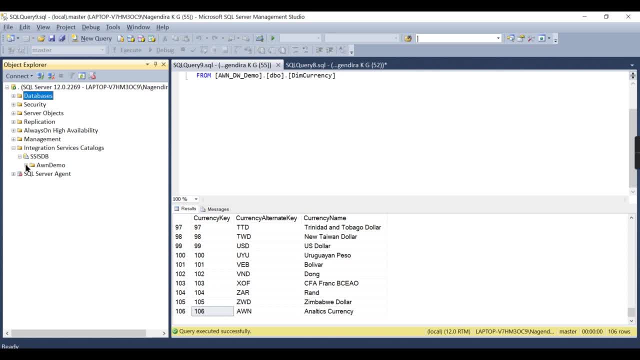 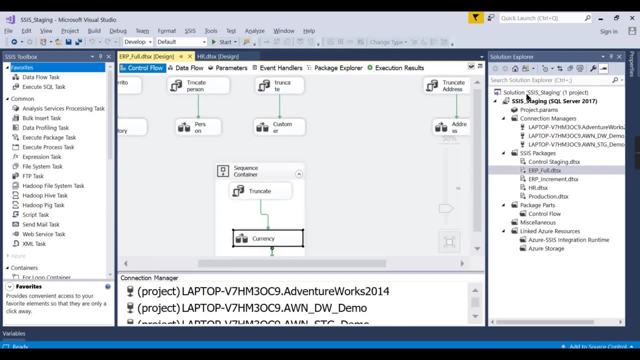 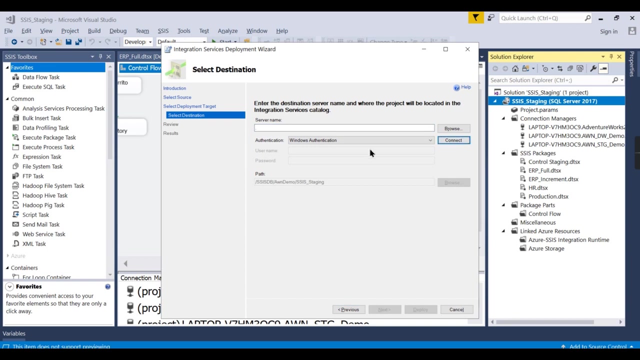 you have sql server integration catalog where you can deploy these packages or projects right over here. so how you can deploy it, so you can go here and deploy it. so just build this project and deploy it. and i will tell you another important aspect of it, what i want to inform about the controlling. 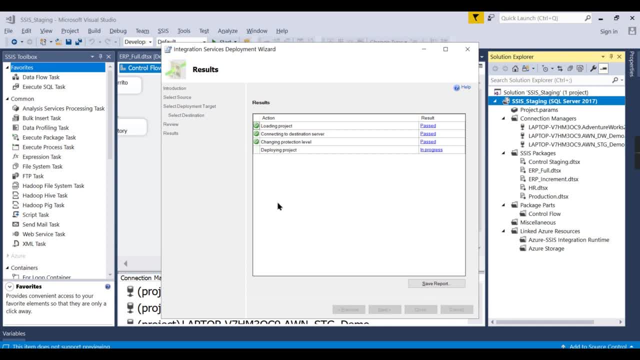 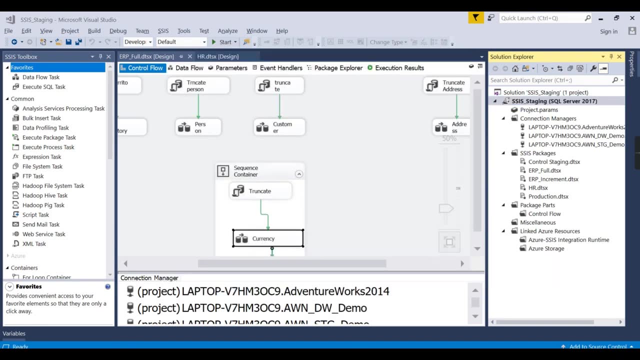 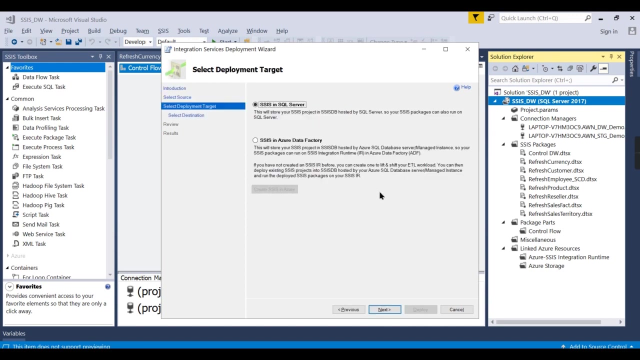 package. now we have this deployment done. so this is like ssis integration catalog is like storage for your ssis packages, where you can maintain those packages over there. so you deployed this staging. similarly, you go and build and deploy your data warehouse project as well. so, as i said before, there will be two projects: one for staging, another one for your. 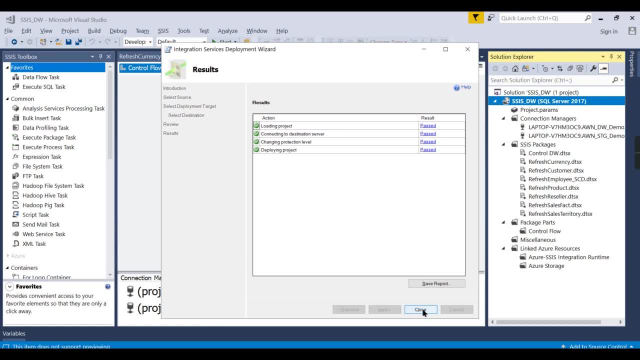 ssis, those packages here, and if you i have any questions, please let me know through the comments now. so what we can do, yo can we. you can deploy IIö in the ssis como uh and deploy you want to pay off your css, and you can deploy both the packages every year. so, as you can see, 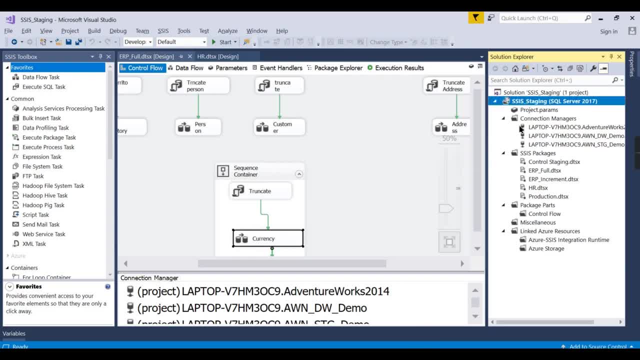 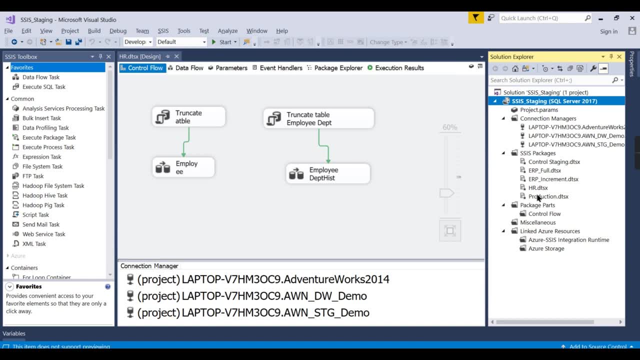 this one, this project, which is called an archiveCKS, you can apply either in north or south for all of an aspect. you see, here is like you, no need to manually run right here over, right. so you. that's why i already told it's like a controlling package. you call those packages over here. 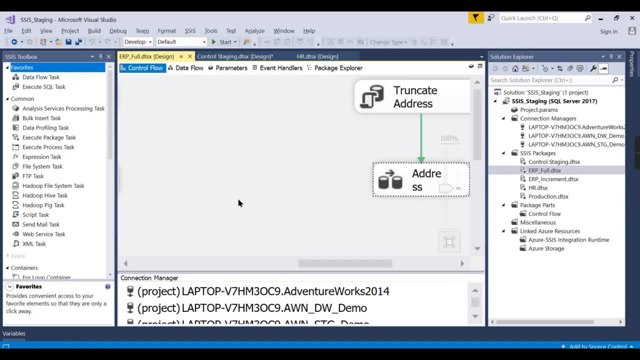 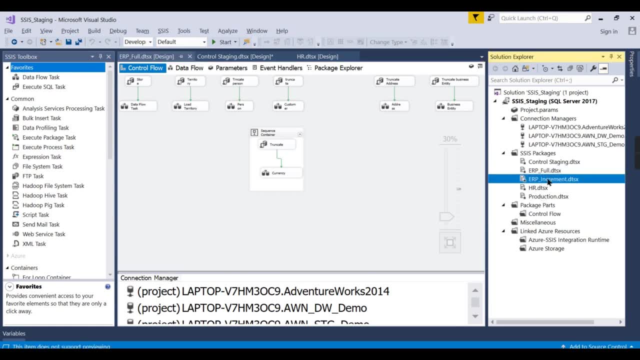 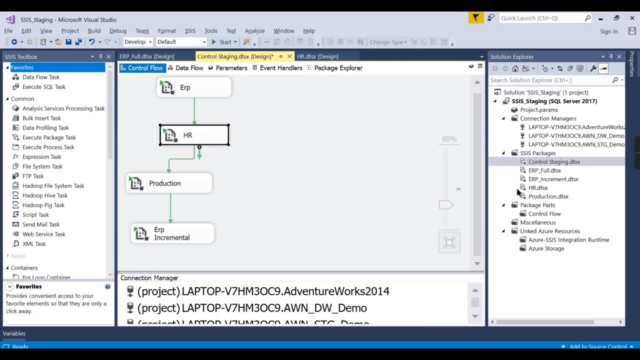 so this will call the all the erp related source tables- 10 tables. so how you will call, instead of calling this one, this one, this one, manually, you can create the controlling packages. then you can schedule this package. so that is why you create a control package. what is this control package? 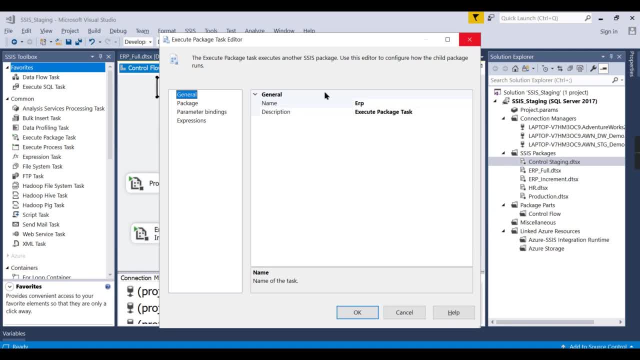 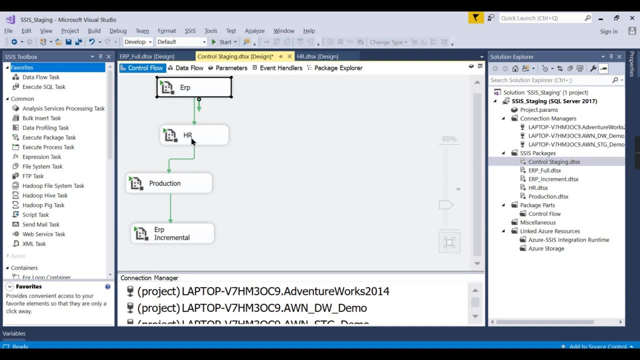 that intent will call the execute package task, that will call the another package. okay, once you call this package, this will call erp package, this will call hr package, this will call production, this will call erp incremental. so this is the flow i'm saying about. similarly, you create a 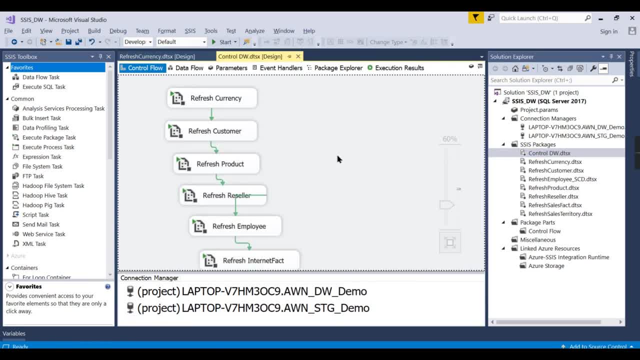 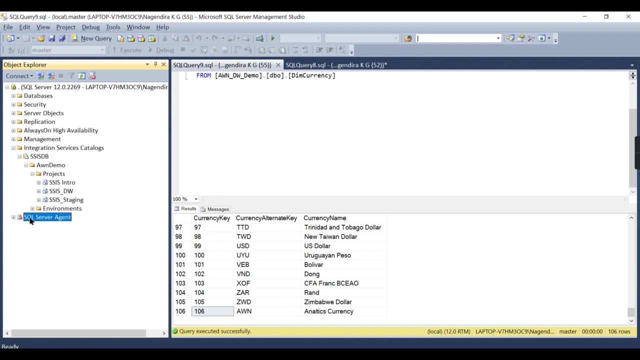 controlling package for the data arrows as well. so you see, i have created all the dimension refresh here. whatever is missing something- i think reseller or some dimension missing- i have created, i have created a control package. so this is what you will deploy it here. so deployment is done. who will run this task regularly? that is the task of the sql server. 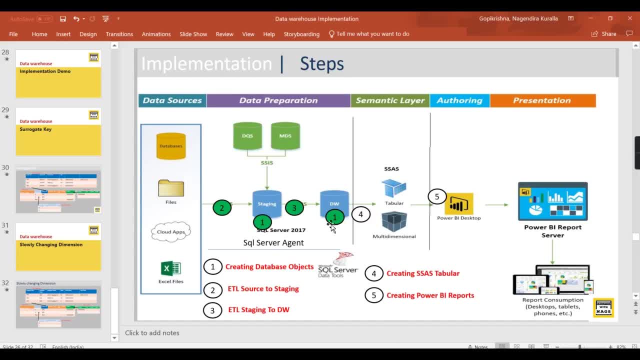 agent. so now going back to this presentation, now we have seen the entire flow and you have some control packages to run from sources to target- i mean staging- and you have a control package that will read from staging to data arrows. so when you should call how, what tool? 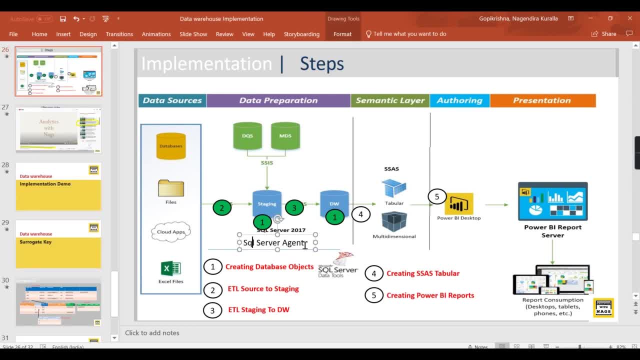 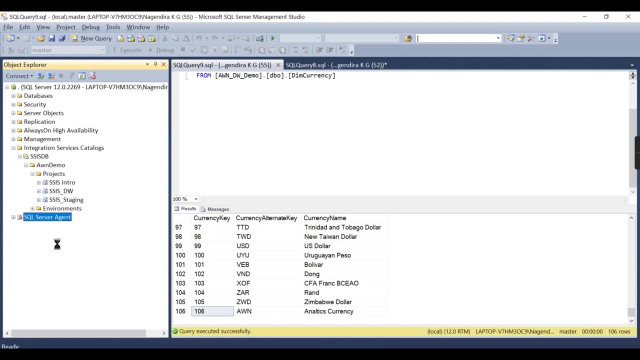 will call. so that is why we have a sql server agent. so this will call those two control packages. then the entire process will keep on flowing right. this is what it is now to demonstrate that you can add this sql server agent. let us click yes, let's say yes, and you can schedule a different. 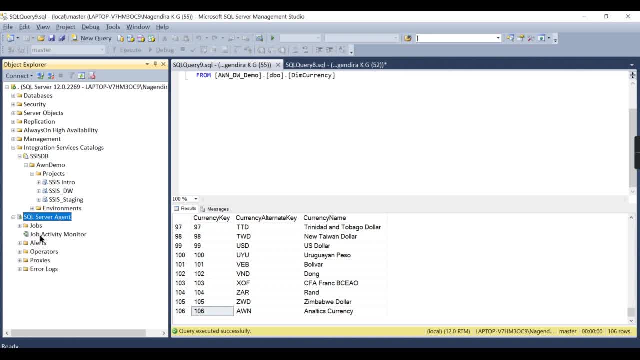 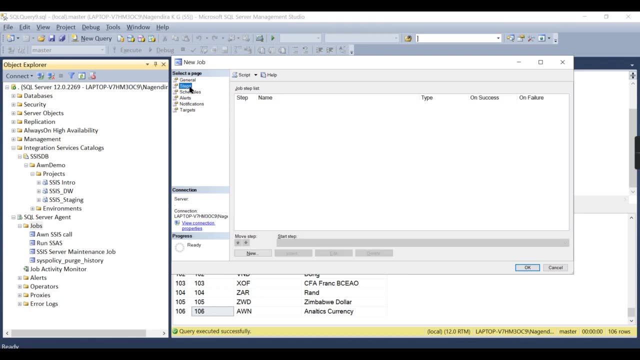 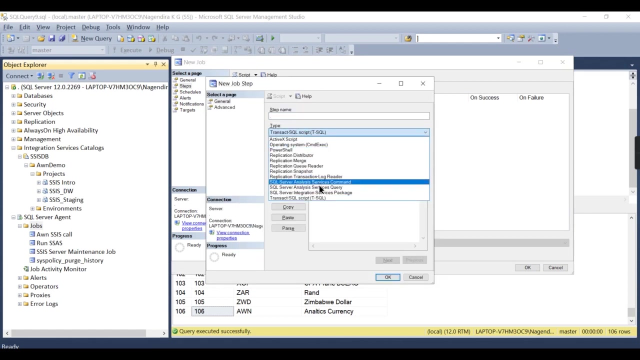 task. so it is not going to have only a single or one or two tasks. so, as i said before, you will create per each data match. so how you will create a job. so you click on new job, like stage job, okay, then go to steps new. so this is why it is not a very simple, straightforward, single thing. you learn sql. 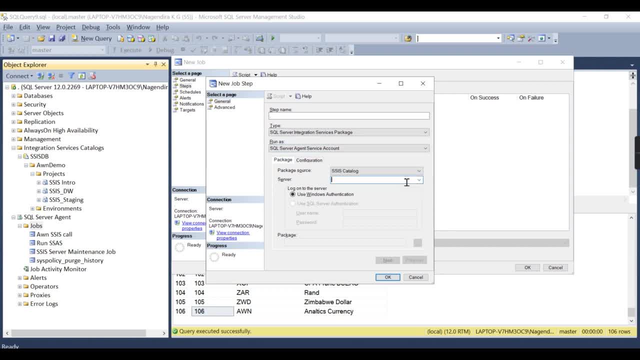 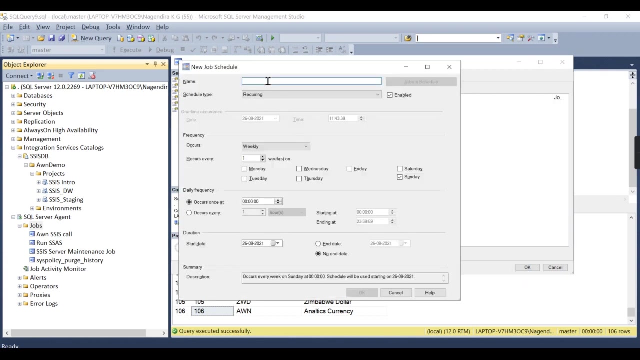 you will understand everything in data arrows. it is very complex, far complex than whatever we thought, right. so you choose the integration service package and then choose appropriate packages here. right here i will choose the ssis control staging- okay, and then click on: okay, you can schedule this job to some timing. schedule a 2 am job- okay, something like that. okay, it can. 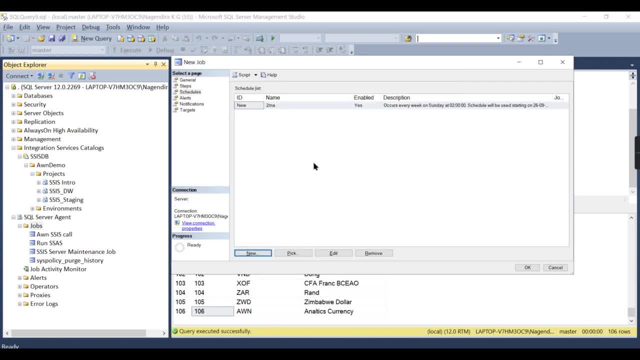 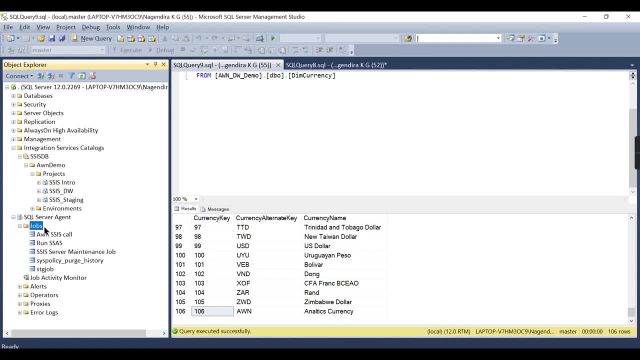 be anything. 2 am for day. it should schedule. you can schedule it so this job will run. so you no need to manually run all these things daily. so this is a string job. similarly, you can create the data arrows job as well for different schedule or, once the staging done, you need to call that one in. 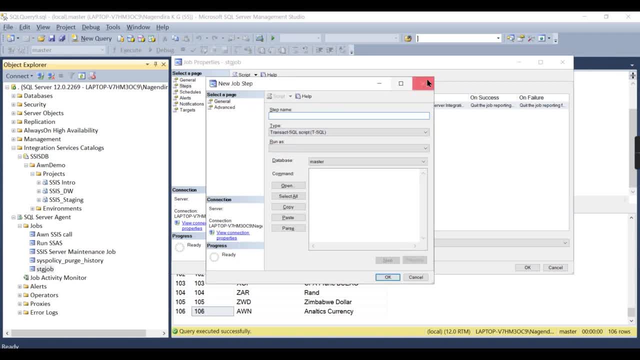 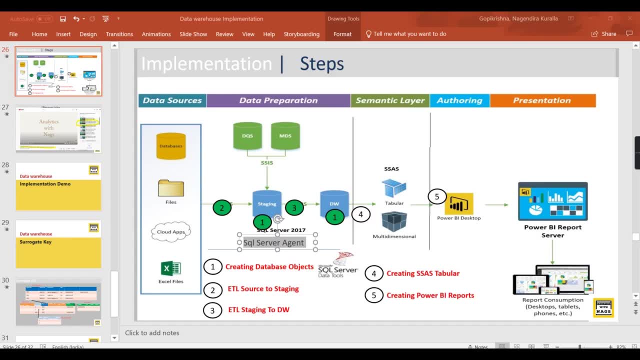 a next step讯: sql. Jamf that job over here itself. okay, this is up to you how you can run the schedule. this is fine. so this is what I want to highlight. we are done with our data warehousing layer. I have covered all the aspects which related to sales module. 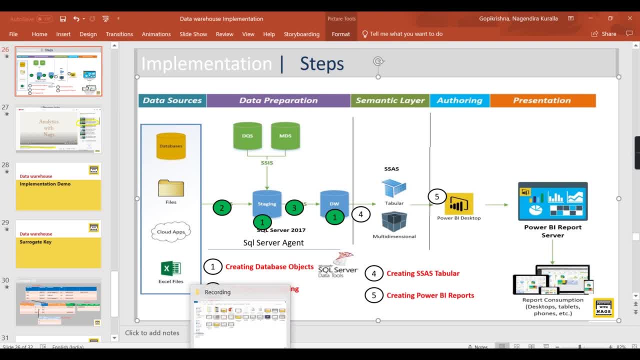 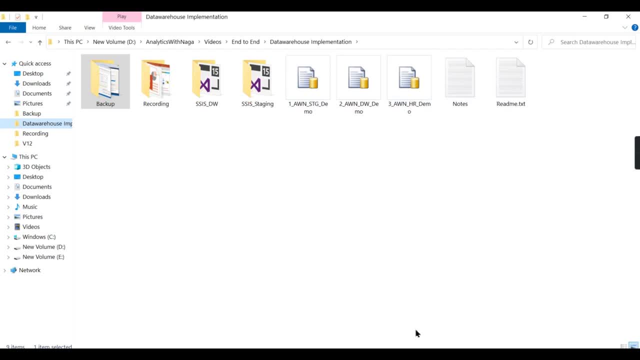 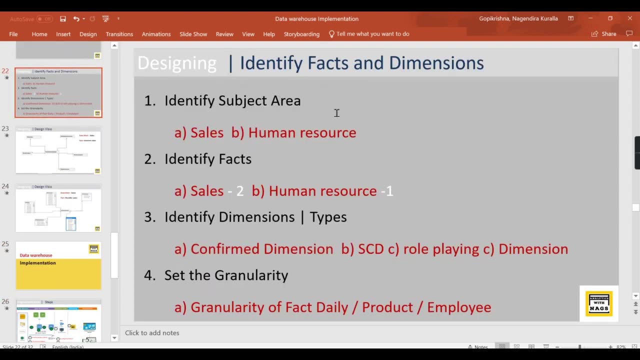 and, for your information, I have some quick method for creating the HR schema. like we have discussed here, we need to create two subject areas on a sales and then a human resource. I do not have a time to demonstrate or create the human resource data matter in a proper way, as we did for. 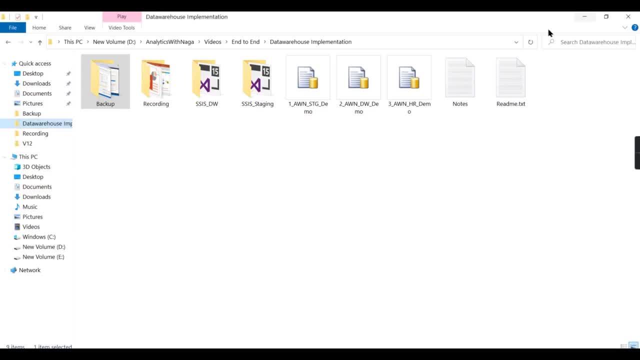 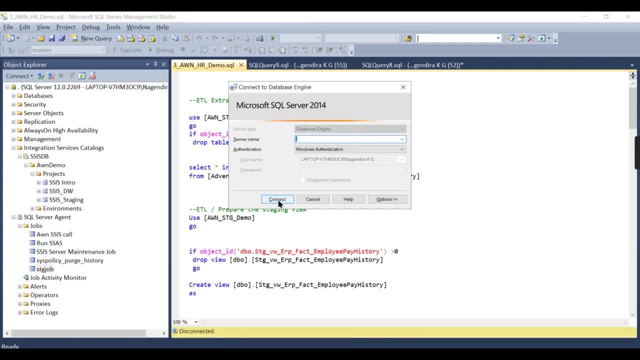 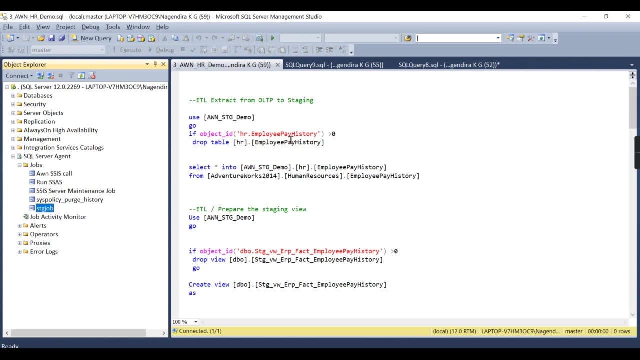 you sales. we created two fact and dimensions, so instead what I created is like: I created one script here, so this script will create you the entire thing, from the source to staging, staging to data warehouse and refresh logic, everything what I'm trying to say, you see, here we have fact employee pay, which is nothing. 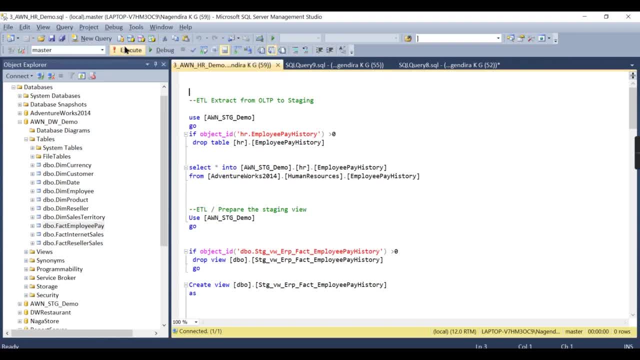 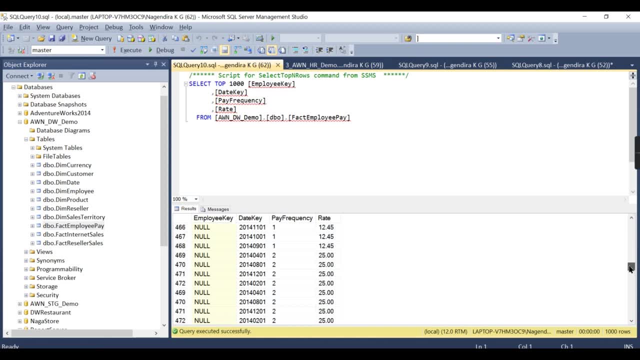 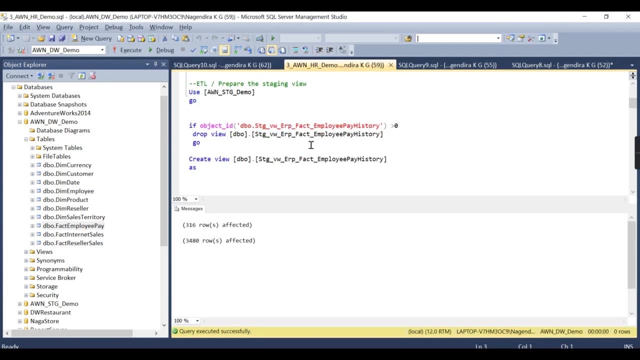 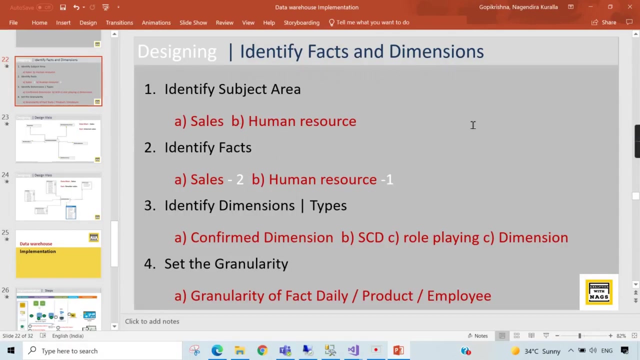 but you. when you run the script, this will create that particular fact table. what this fact table contains? basically this fact table. let me see why the employee records are not coming. so what I have done here is like to save our time. I have created a single script. 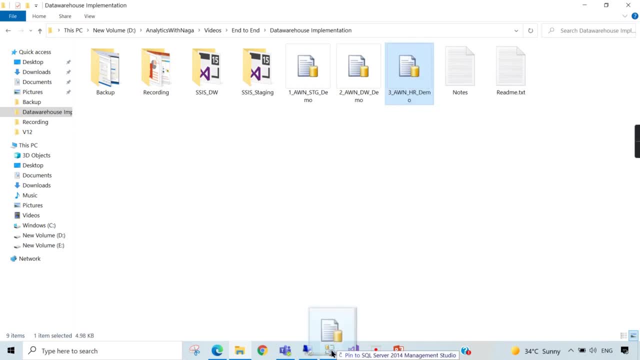 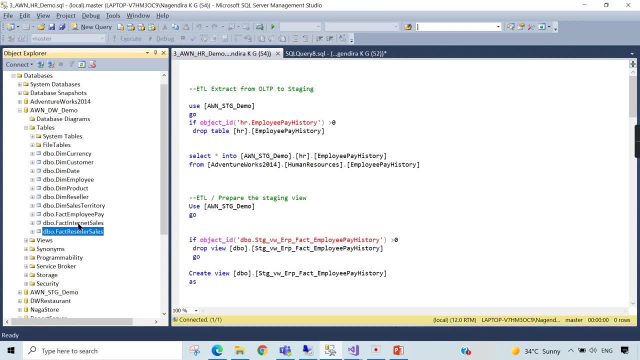 here awn hr demo, which will create a human resource data mart, a single fact table here. let me show that. one see, these two are belongs to sales data mart and here you have the employee pay when you run the script. okay, you see, some rows are affected here. that will insert this fact table. 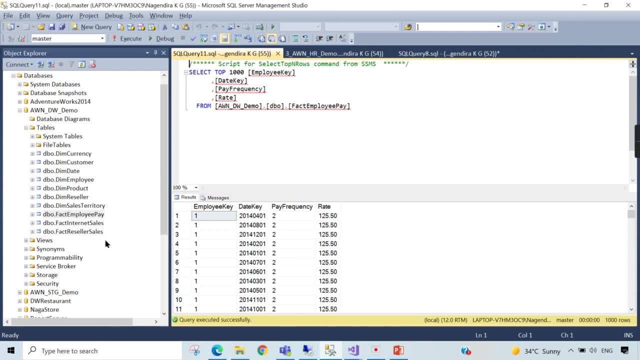 what it will do is it will create some records from. i mean, it will create some table in the staging area and then create some views, then populate the fact to create the your hr data model. i have created one single fact table. basically, what this model will do is like: 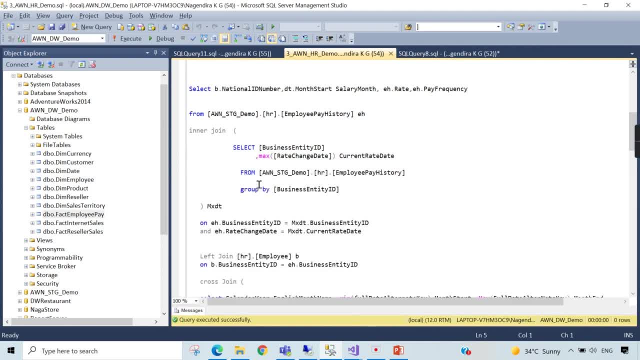 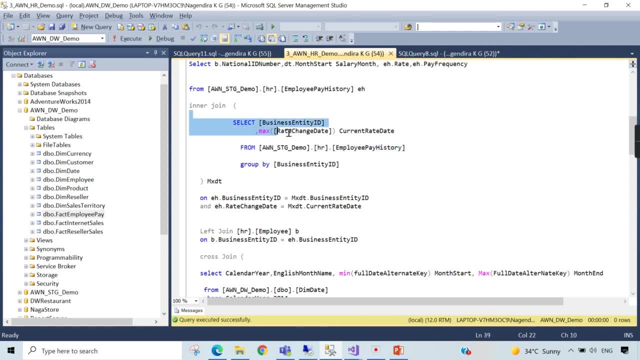 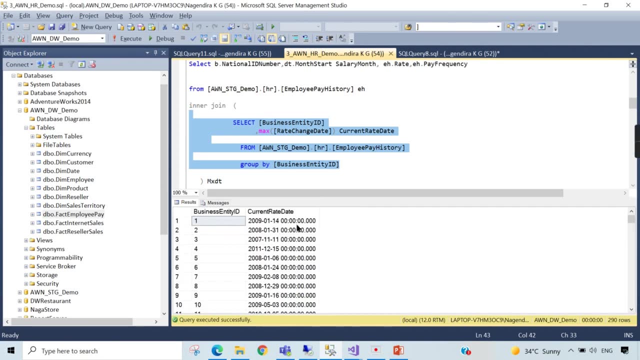 it will get you the data. okay, from the source. okay, this is the hremployee history, this is in the staging table and you will get the maximum rate this particular table contains when for each employee, what is his current salary. so business wants to see what is they are paying for. the 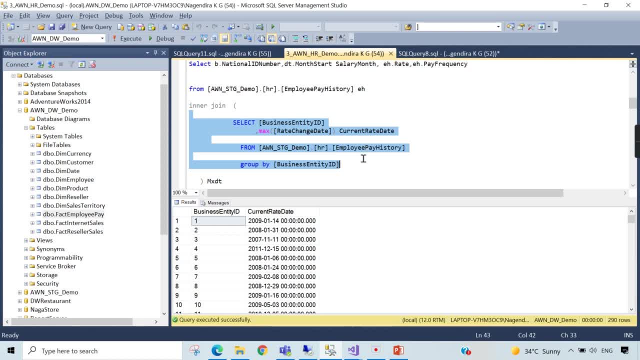 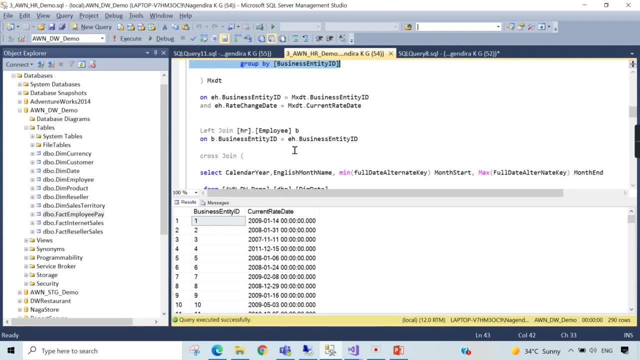 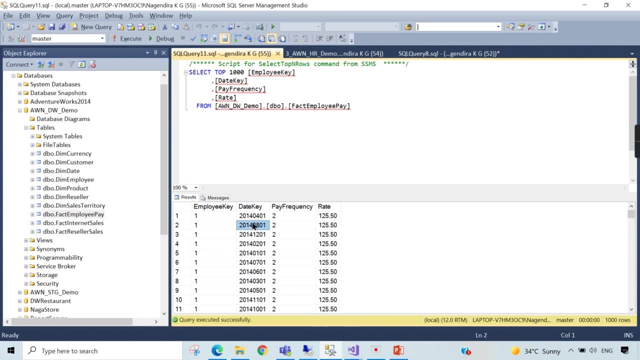 entire year. that latest year available in the adventure works is 2014, so i will get the latest pay range. then i will simulate for next one year that 2014 here. okay, then i populate it. so this fact contains only two keys: employee key and date key for each month. okay, how much they pay, they are. 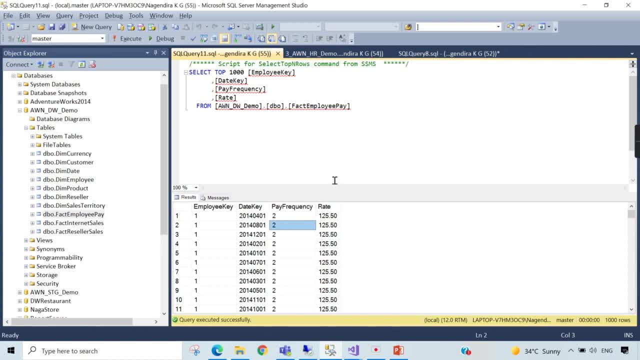 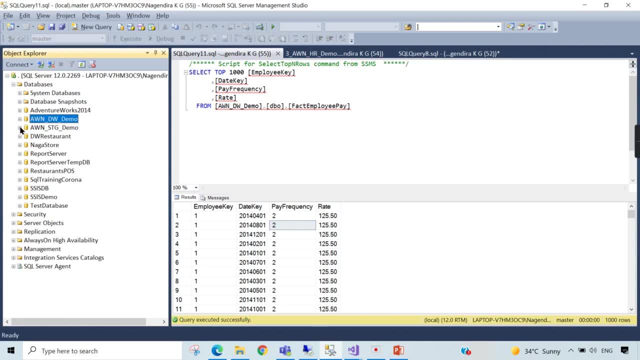 getting. that is what it is. it can be considered as a single fact table. so this is again a one data mart. so here, similar to the staging layer- erp, erp, hr- in data arrows, you can have a schema defined for these two. everything can be sales. okay, then this can be: 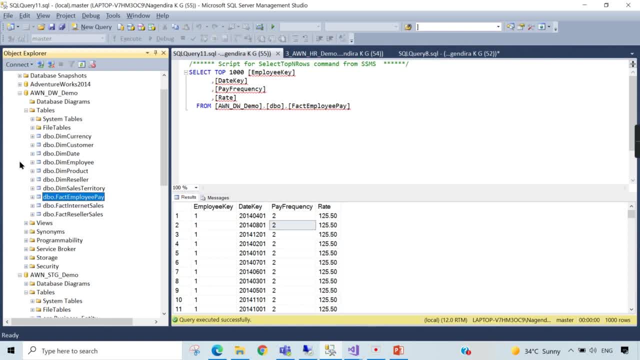 i mean this can be in the hr, so here also you can have a schema to distinguish between the data mass. for simplicity- i have not done that- you can create it in a views. okay, once you have a dbo over here, you can create the data mass virtually in form of views as well. that is absolutely fine. 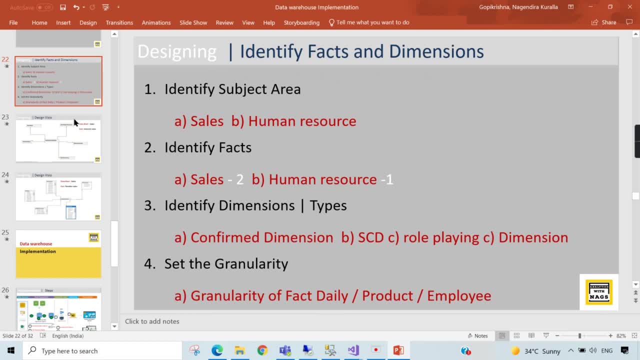 so what i'm trying to say, the sales we have completely gone through in order to create a human resource. i have prepared the script for you. you can run it now. you can create a human resource. i have prepared the script for you. you can run it now, you can. 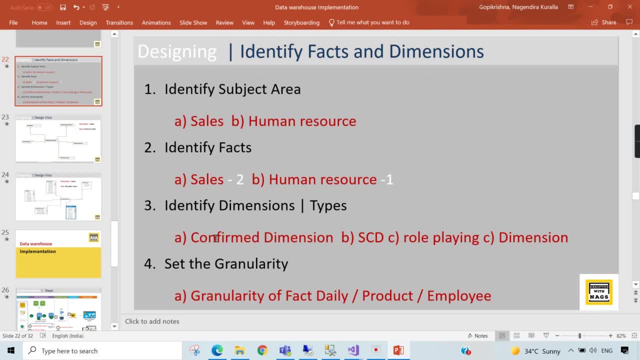 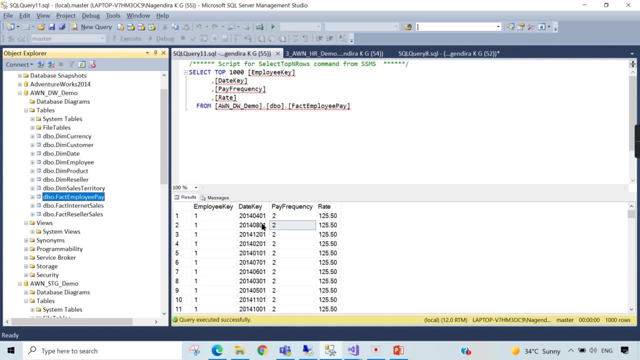 see how you can identify all these things in this entire demo the confirmed dimension is date, because this date is used in this particular fact table as well as internet sales, as well as reseller sales. so a particular dimension used in all fact or data marks, then it's called confirmed dimension. 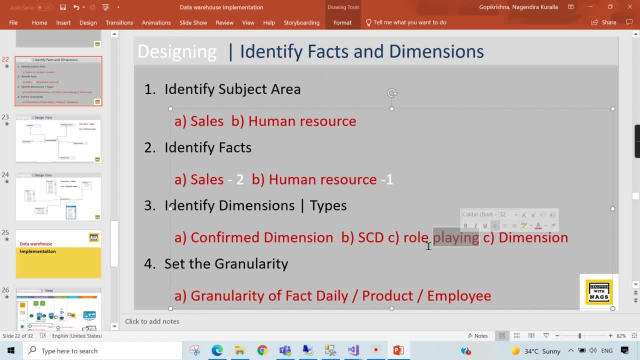 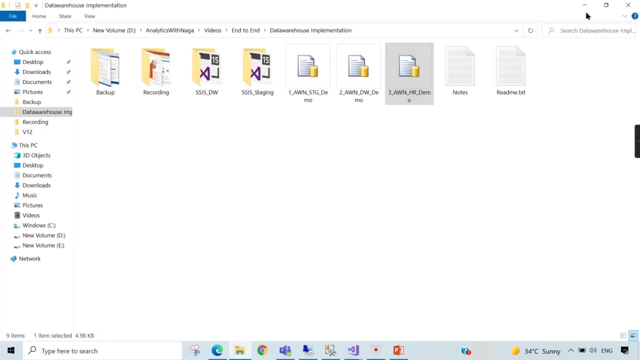 we have seen employees scd again, date place a role playing: dimension: order date and sale date, due date, everything then a specific, two particular fact tables called reseller. reseller belongs only to the this particular fact table. so these are the some of the things i want to highlight. 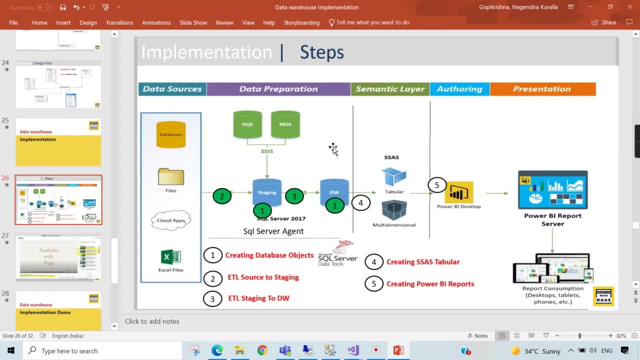 i hope we are pretty much covered. all the topics related to data borrows. i definitely sure you will get more questions. keep commenting on the below. let's move on to our next section. like covering this ssas and power bi. these are typically add-on to this data arrows or 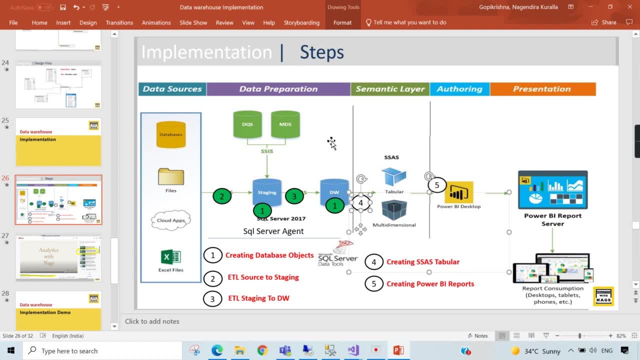 this is those who are only need to implement data arrows. this is fine. this video ends here. but why? these are things required because any data errors implementation requires either of them. you need to build a cube and then a power bi report. then only the data browsing end objective is met. right, only creating a data arrows doesn't make any sense. 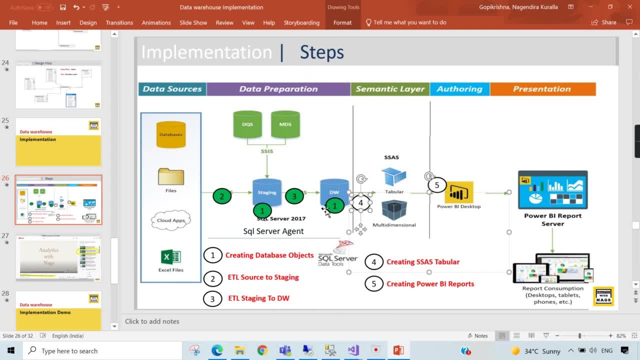 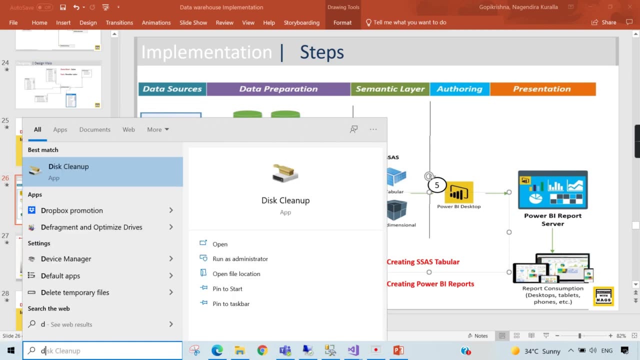 because everyone cannot know to write the queries in the data arrows. you need some application on top of data arrows. so these are the those things. let's start with building the ssas. ssas- uh, it's not ssas. you need to press ssdt to create the cubes. so i have a separate playlist for 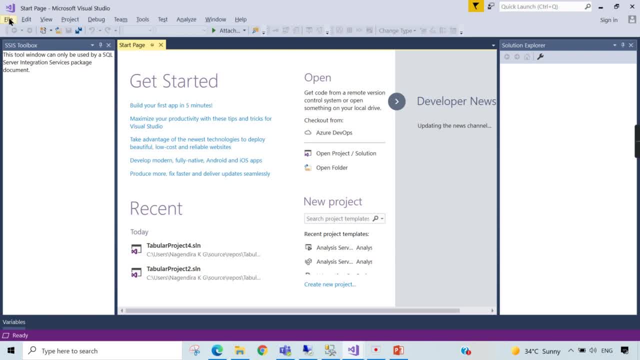 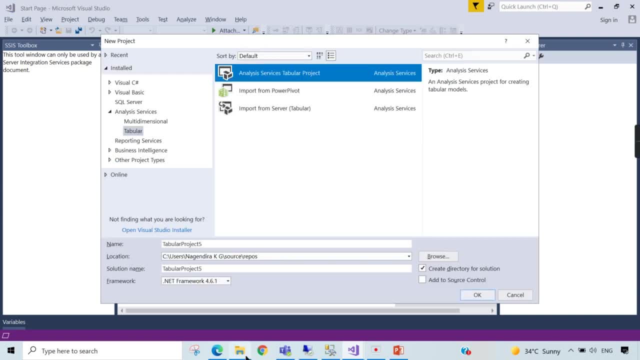 creating the ssas cubes. if you are not familiar, just go and watch my playlist: ssas tabular model. so now, clicking on tabular model, i'm clicking on it and let me navigate to here. then i create, i take this folder, let me store the project here. yes, awn, ssas demo. let me name it properly then. 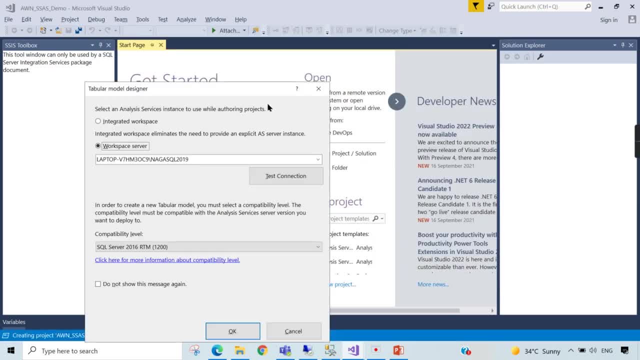 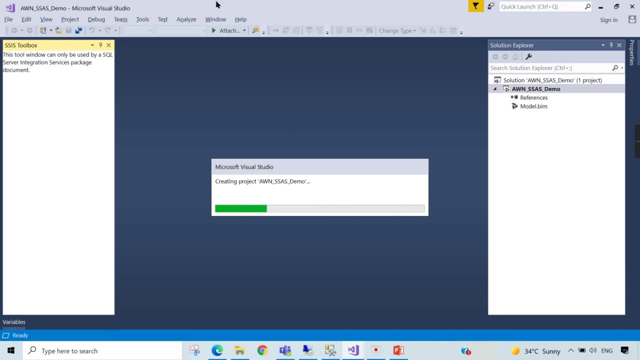 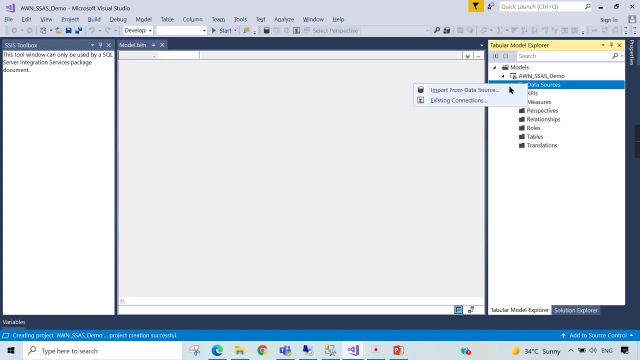 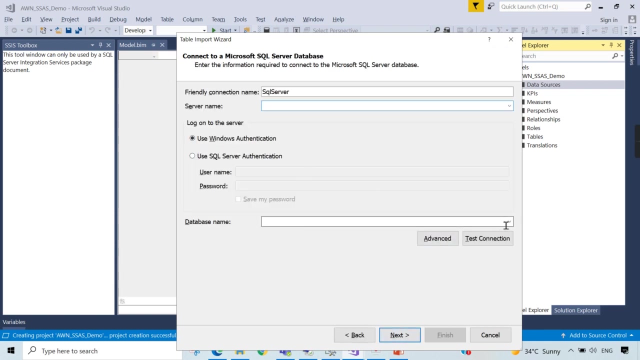 click on um, okay, then i choose my workspace server where i want to deploy it or work on it, so click on ok. so once you have this with you, then click on data sources- import from data source sql server and then you use database name. sorry, i think server name is. you provide a server name? i'm pressing dot for my local. 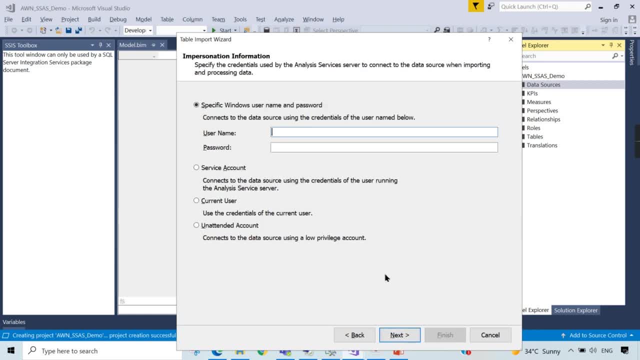 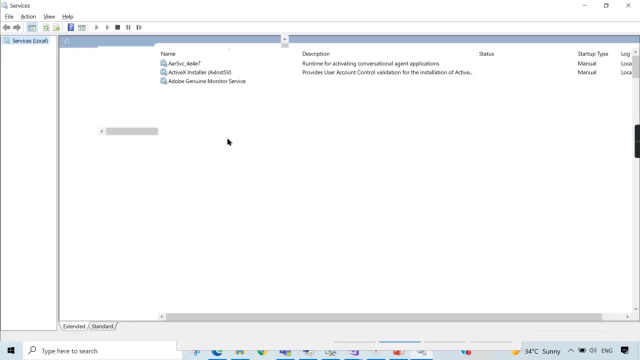 i'm pressing aw and dw demo and most of the people will face issue here. this service account: you need to have a permission. what is this means? this ssas services will run in one particular account, so ensure you add this account in your sql server. those who are practicing directly: they might face issues. ssas services will run in one particular account, so ensure you add this account in your sql server. those who are practicing directly. they might face issues. ssas services will run in one particular account, so ensure you add this account in your sql server. those who are practicing directly. they might face issues. 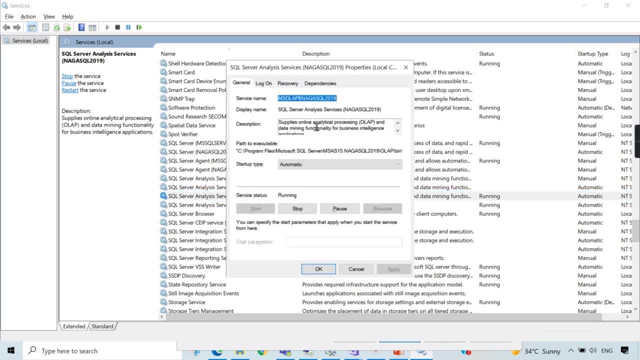 ssas services will run in one particular account, so ensure you add this account in your sql server. those who are practicing directly, they might face issues. i am telling. i am telling i had. so this is the service account okay, i had. so this is the service account okay. 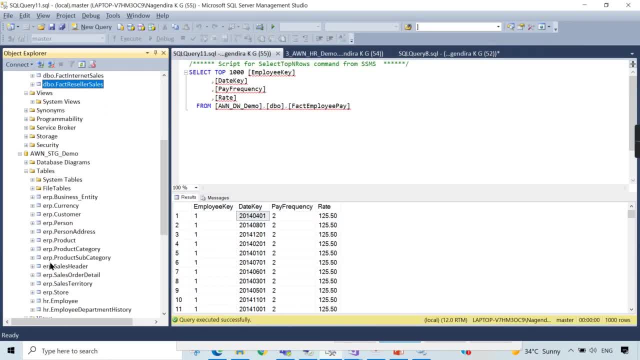 i had. so this is the service account. okay, take this service account, ensure you add. take this service account, ensure you add. take this service account, ensure you add the permission you added in the sql, the permission you added in the sql, the permission you added in the sql server. login here, you see. 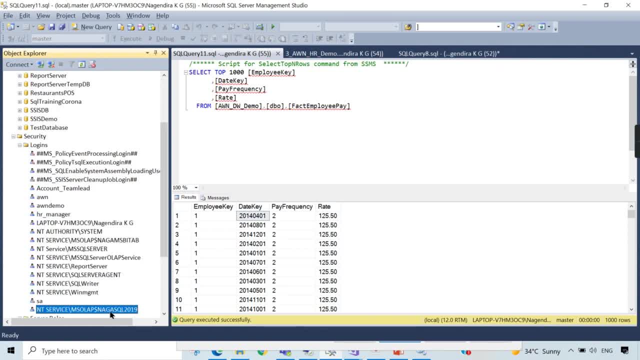 server login here. you see server login here. you see in this login you might you should have in this login. you might you should have in this login you might you should have added that account and give permission to added that account and give permission to added that account and give permission to read this database. you need to ensure. 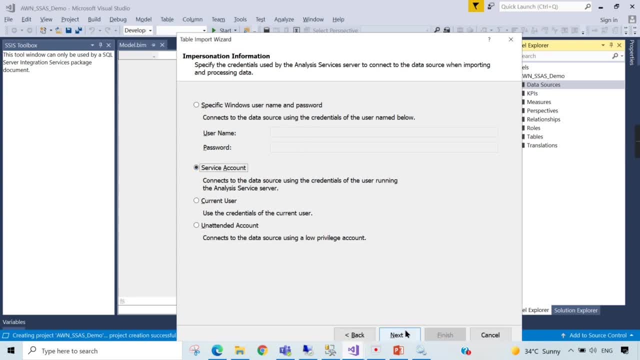 read this database. you need to ensure read this database. you need to ensure that that that. now back to ssh. then click on service. now back to ssh. then click on service. now back to ssh. then click on service account. select list of tables and views. account. select list of tables and views. 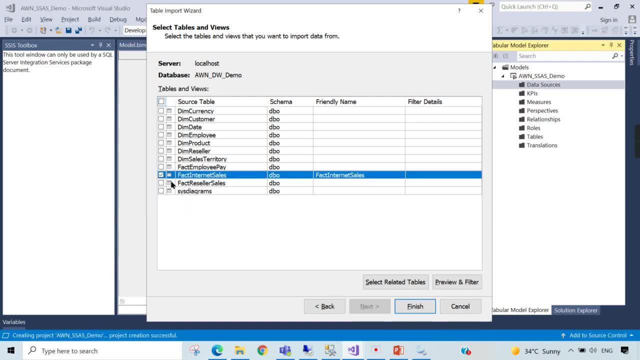 account. select list of tables and views. yes, so now i can build any model. yes, so now i can build any model. yes, so now i can build any model. now. let us build model for now. let us build model for now. let us build model for sales data mart, as we have only one and 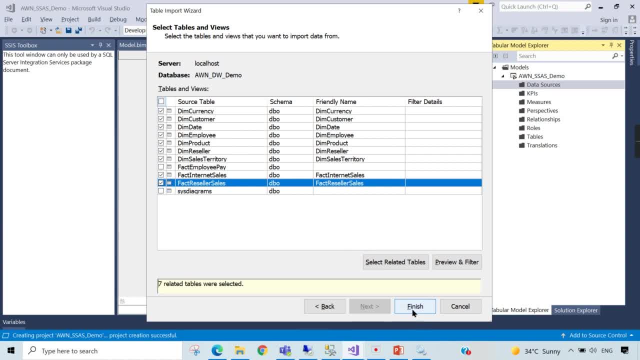 sales data mart, as we have only one, and sales data mart, as we have only one. and then i choose selected, then i choose selected, then i choose selected related tables. that will select all the related tables. that will select all the related tables. that will select all the related tables of those two fact tables. 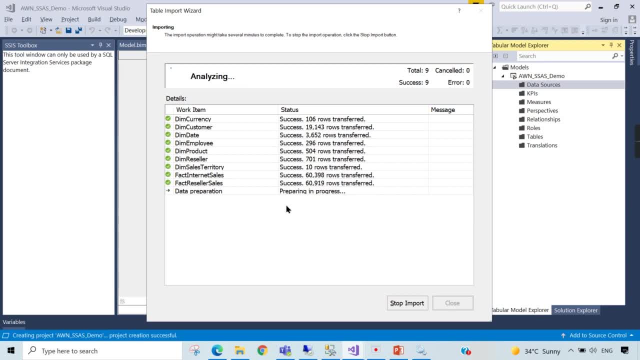 related tables of those two fact tables, related tables of those two fact tables. then it will read those data over here. then it will read those data over here. then it will read those data over. here we are, we are. we are done with um building the tabular model. 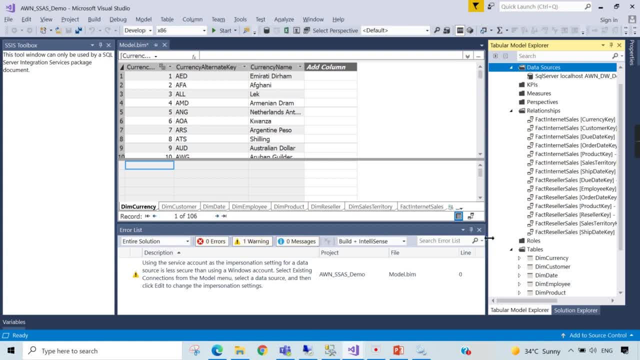 done with um building the tabular model? done with um building the tabular model? it's not, uh, i mean we are not done, just it's not. uh, i mean we are not done, just it's not. uh, i mean we are not done. just creating the skeleton and you can start. 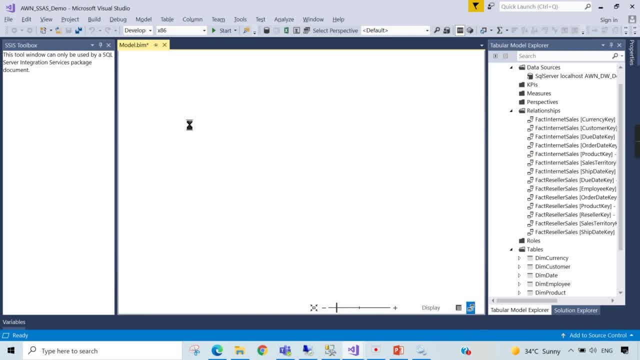 creating the skeleton and you can start creating the skeleton and you can start writing the calculations like mtd ytd. or writing the calculations like mtd ytd, or writing the calculations like mtd, ytd or whatever calculations you have. so now, whatever calculations you have, so now, 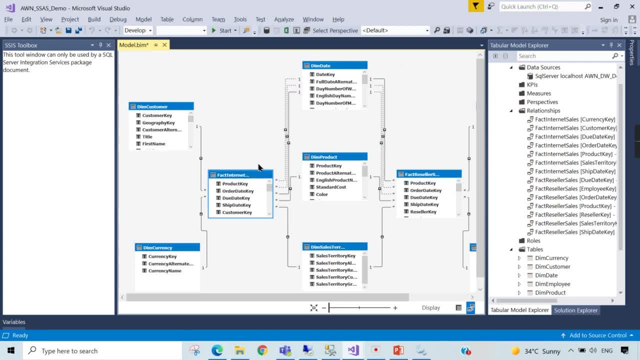 whatever calculations you have. so now you can see, you can see, you can see a beautiful star schema here, this fact, a beautiful star schema here, this fact, a beautiful star schema here, this fact: internet sales surrounded by internet sales, surrounded by internet sales surrounded by five uh dimension, and this reseller sales. 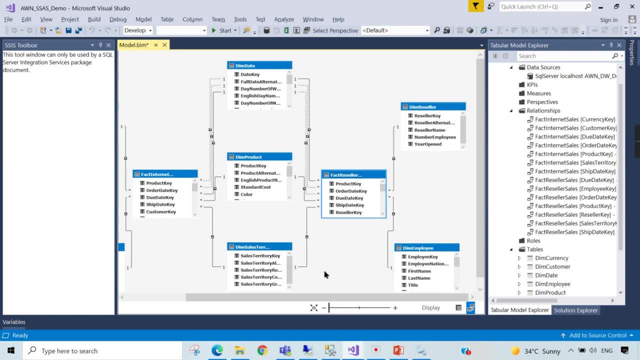 five uh dimension and this reseller sales five uh dimension and this reseller sales surrounded by, surrounded by, surrounded by four different uh four. four to five, four different uh four. four to five, four different uh four, four to five different dimensions. so this is how you different dimensions. so this is how you. 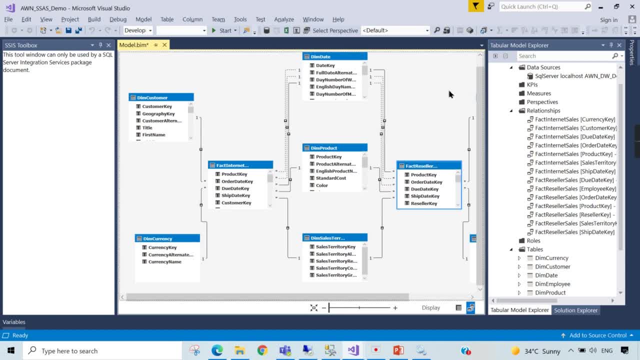 different dimensions. so this is how: you built a data mart that is sales data, built a data mart that is sales data, built a data mart that is sales data mart and you have imported it mart and you have imported it mart and you have imported it and you, in sales data mart, you can have. 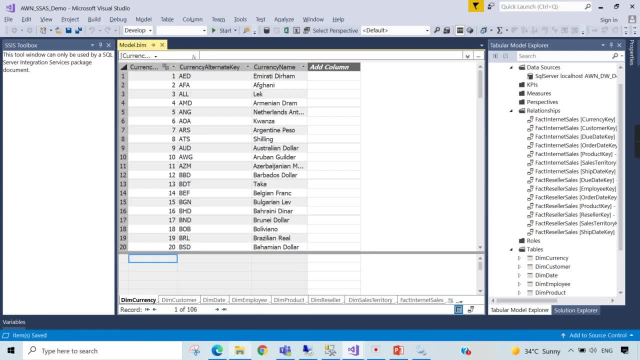 and you in sales data mart, you can have, and you in sales data mart you can have other fact tables as well, other fact tables as well, other fact tables as well. okay, it depends, so now to give you quick. okay, it depends, so now to give you quick. 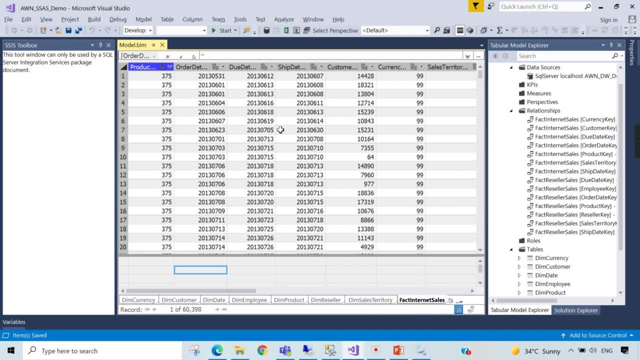 okay, it depends. so now, to give you quick calculation, let me write calculation. let me write calculation. let me write: start writing some uh dax queries. i'm start writing some uh dax queries. i'm start writing some uh dax queries. i'm not going to. 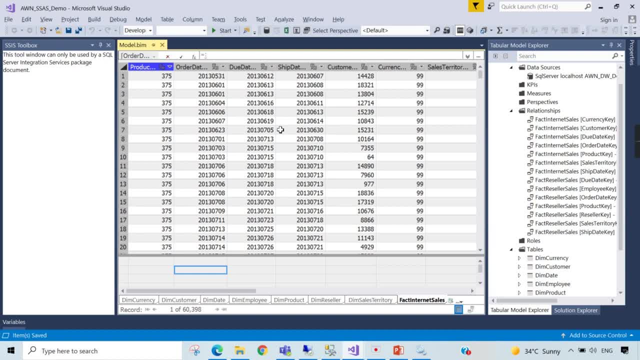 not going to not going to spend much time on it, i'll just start spend much time on it. i'll just start spend much time on it. i'll just start writing, writing, writing some names over here like total sales, some names over here like total sales, some names over here like total sales, because this is not a focus for uh. 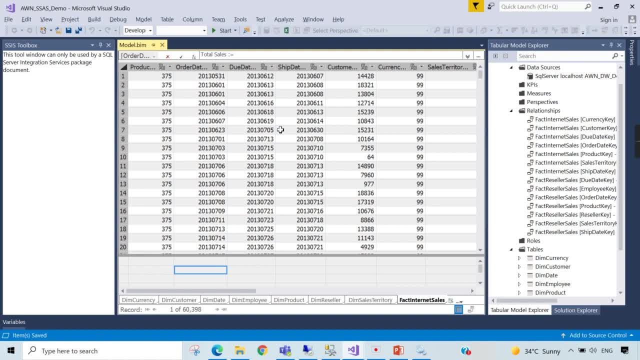 because this is not a focus for uh, because this is not a focus for uh, understanding, understanding, understanding the dax or ssas. so i'm just the dax or ssas. so i'm just the dax or ssas. so i'm just wrapping around quickly: quantity okay. 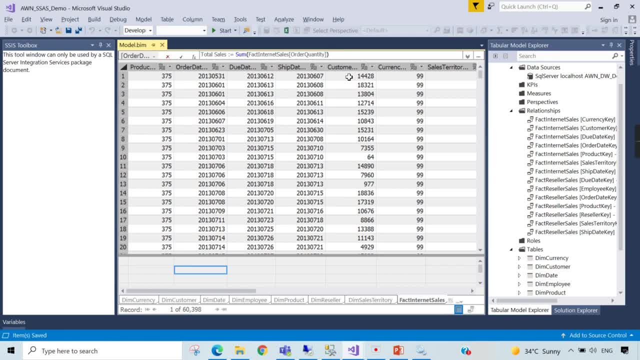 wrapping around quickly, quantity: okay. wrapping around quickly, quantity okay, so so so. order quantity from the sales, just uh. order quantity from the sales, just uh. order quantity from the sales, just uh. total sales quantity: total sales quantity, total sales quantity. this is the measure i've created, so i 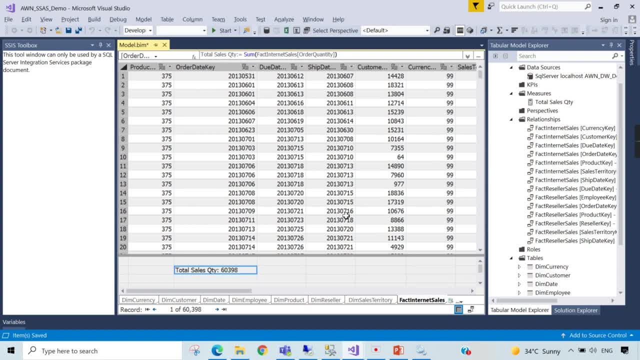 this is the measure i've created, so i this is the measure i've created, so i have have have gone through. i have detailed how you can gone through. i have detailed how you can gone through. i have detailed how you can create, create, create the calculations, everything. so those who 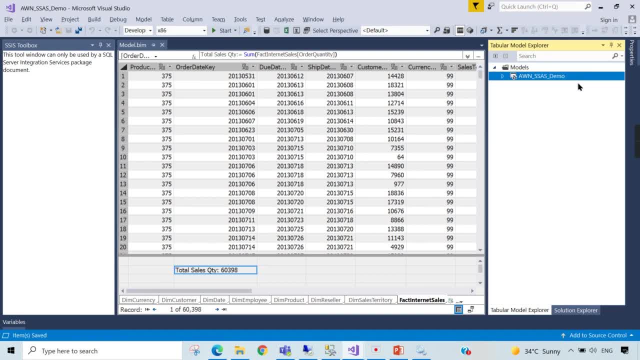 the calculations everything. so those who the calculations everything, so those who are not, are not, are not familiar why we need ssas. we can directly familiar why we need ssas. we can directly familiar why we need ssas. we can directly build uh, build, uh, build uh. we touch upon the power bi. now we are. 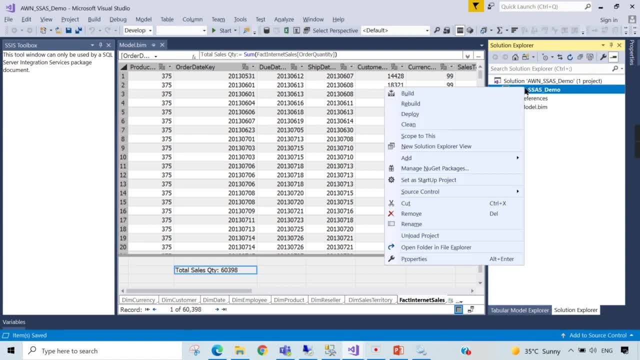 we touch upon the power bi. now we are. we touch upon the power bi. now we are. done with the simple model here. i didn't done with the simple model here. i didn't done with the simple model here. i didn't do much. create a only single measure. 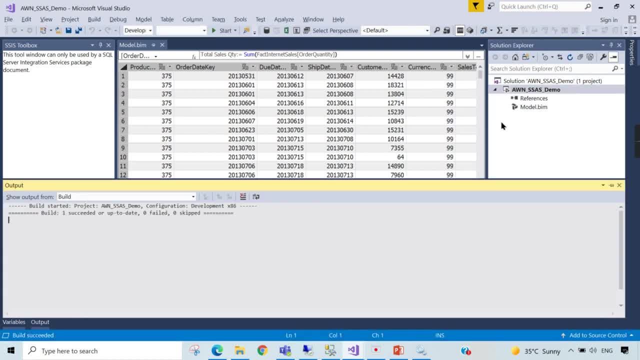 do much, create a only single measure. do much, create a only single measure. then you can build and deploy it in a. then you can build and deploy it in a. then you can build and deploy it in a server, server, server. so this ssas sits in the another server. 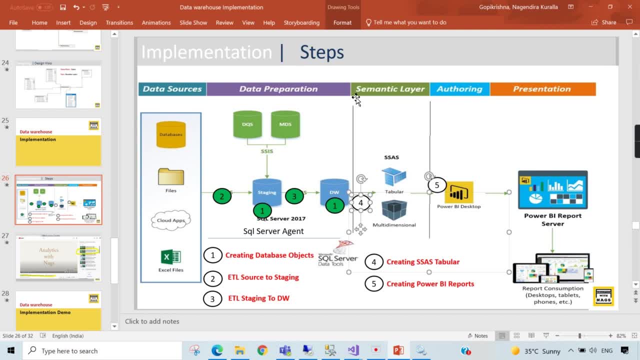 so this ssas sits in the another server. so this ssas sits in the another server. okay again here. when we go back to the okay again here, when we go back to the okay again here, when we go back to the diagram, you have a line here. so this is: 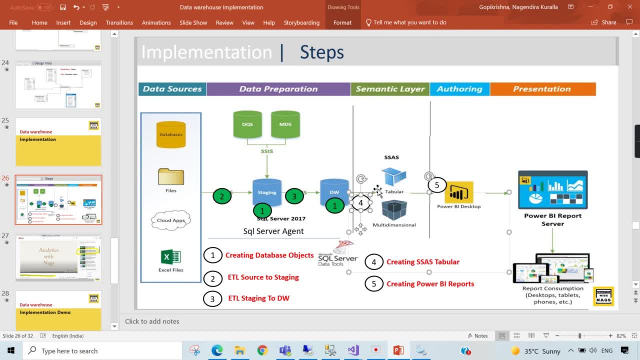 diagram. you have a line here. so this is diagram. you have a line here. so this is not a cube. this is only a data, whereas not a cube. this is only a data, whereas not a cube. this is only a data whereas we build. whatever we built now is the. 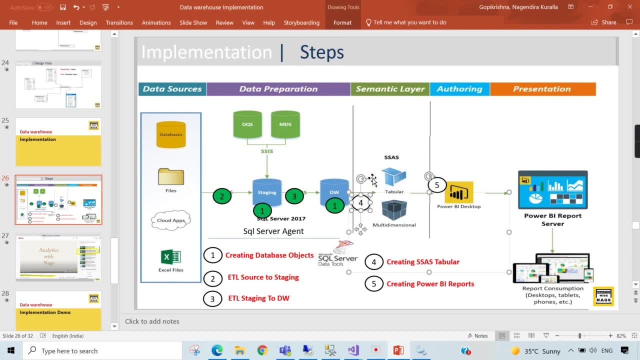 we build. whatever we built now is the we build. whatever we built now is the ssas tabular model. this will go and sit ssas tabular model. this will go and sit ssas tabular model. this will go and sit in another server. you need keep adding. 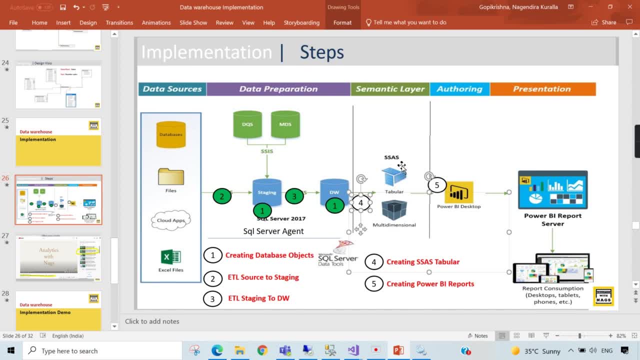 in another server. you need keep adding in another server. you need keep adding the servers. this installation, the servers, this installation, the servers. this installation is like sql server analysis service in is like sql server analysis service. in is like sql server analysis service in this server you need to deploy, so you 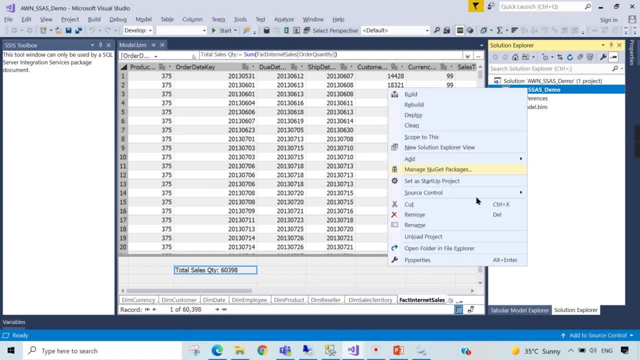 this server you need to deploy. so you this server you need to deploy. so you need to provide the server name here. so you can see: go and check the. so you can see: go and check the. so you can see: go and check the properties. you have the database name. 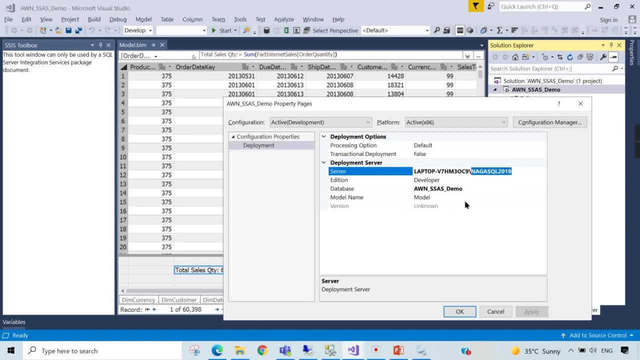 properties. you have the database name properties. you have the database name and you see this is the sql server 2019 and you see this is the sql server 2019 and you see this is the sql server 2019. is the server, is the server. 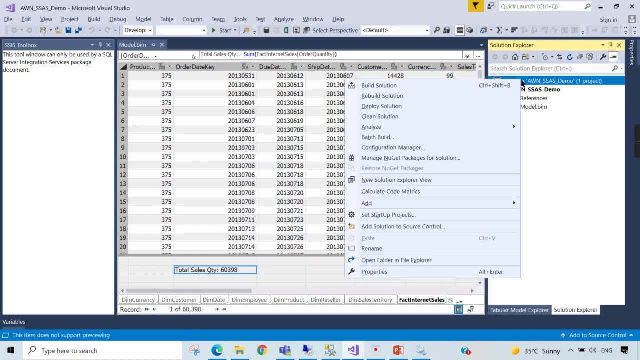 is the server version, which is nothing but the version, which is nothing but the version which is nothing but the analysis server, analysis server, analysis server. once you press and deploy solution, once you press and deploy solution, once you press and deploy solution, i hope there won't be any issues. 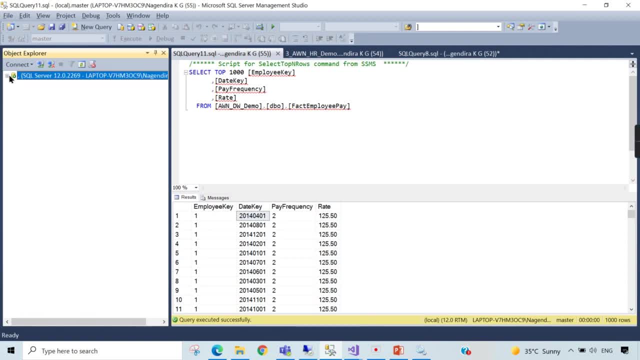 i hope there won't be any issues. i hope there won't be any issues. there you go, it is success. it is very there, you go, it is success. it is very there, you go, it is success. it is very quick, quick, quick. now you can go and check the analysis. 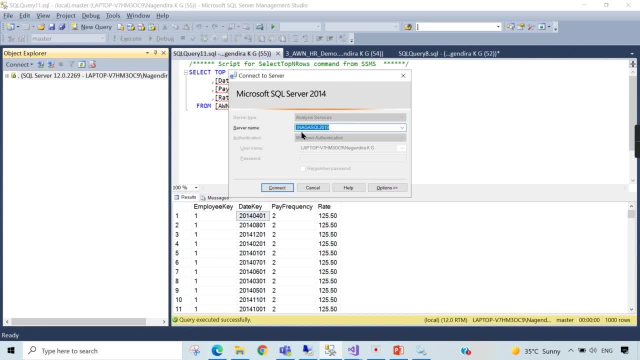 now you can go and check the analysis. now you can go and check the analysis service. how to connect service. how to connect service. how to connect: you go and click on this analysis service. you go and click on this analysis service. you go and click on this analysis service. you see connect to that server. 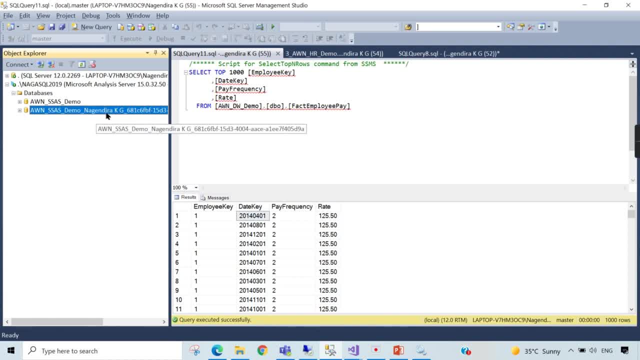 you see connect to that server. you see connect to that server. now you see this ssis demo, though. so now you see this ssis demo though. so now you see this ssis demo though. so it will create a temporary database. it will create a temporary database. 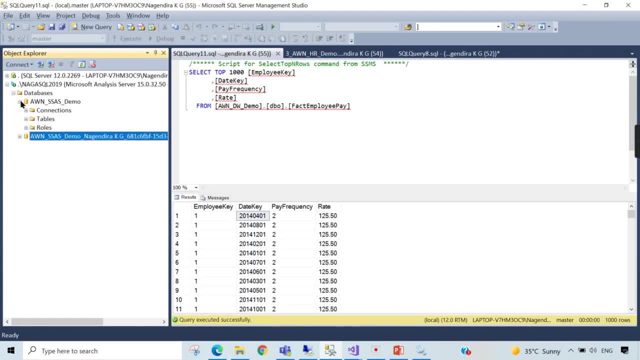 it will create a temporary database whenever i open here. so that is what it whenever i open here. so that is what it whenever i open here. so that is what it is. is is: forget about it. now you can write some. forget about it, now you can write some. 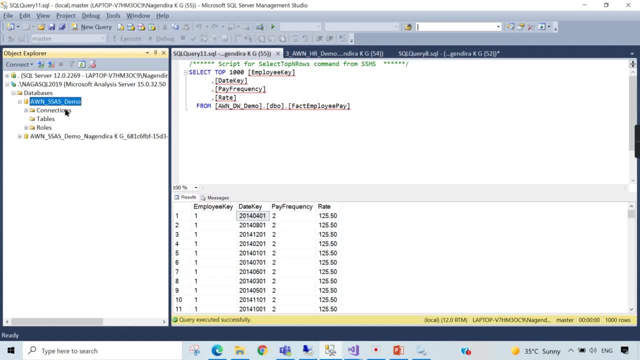 forget about it. now you can write some dax queries directly here, if you want dax queries directly here, if you want dax queries directly here, if you want, or you can, or you can, or you can connect to connect to connect to power bi and connect to power bi or you. 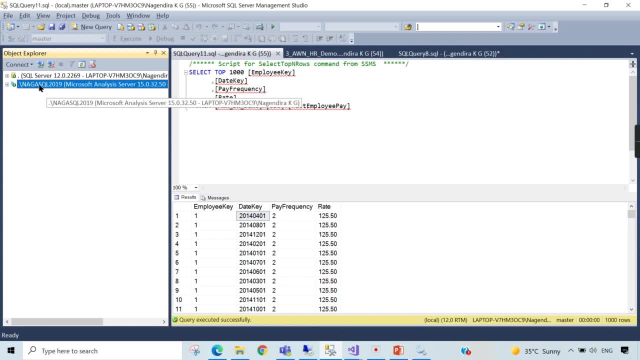 power bi and connect to power bi, or you power bi and connect to power bi, or you can from power bi can connect to data. can from power bi can connect to data. can from power bi can connect to data. arrows, arrows, arrows. so this is what a cube is. we are done. 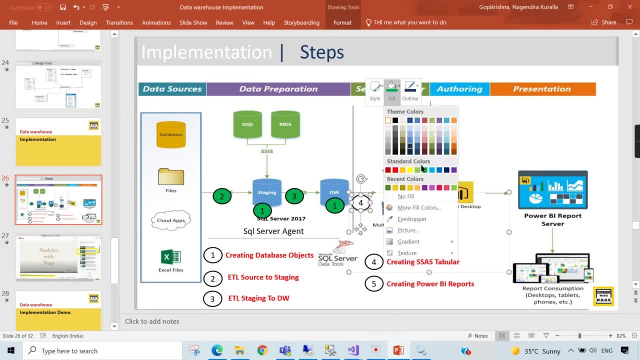 so this is what a cube is. we are done. so this is what a cube is. we are done with the cube, with the cube, with the cube. so let me have a green signal for it. so let me have a green signal for it. so let me have a green signal for it, so this cube you can connect from power. 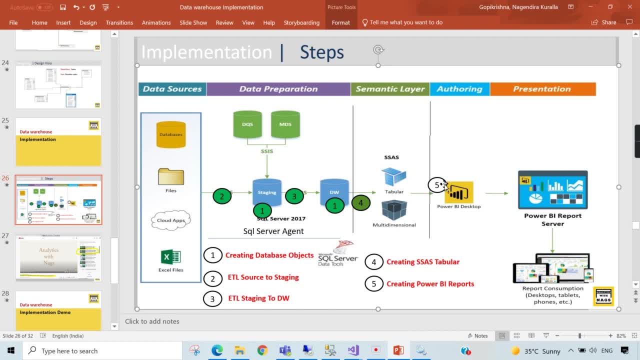 so this cube you can connect from power. so this cube you can connect from power bi. so next final step: what we are going bi, so next final step, what we are going bi, so next final step. what we are going to do now is like we are going to create. 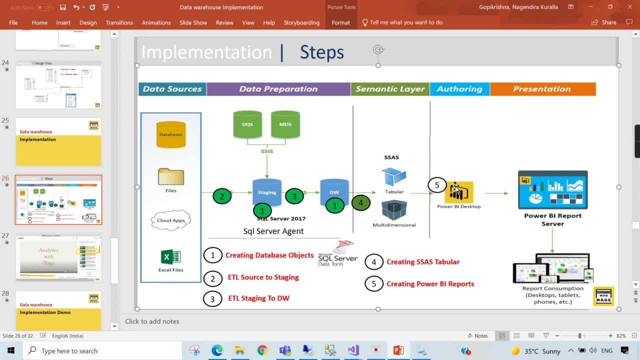 to do now is like we are going to create. to do now is like we are going to create. a power bi report from ssas- one report. a power bi report from ssas- one report. a power bi report from ssas. one report. another power bi report directly from: 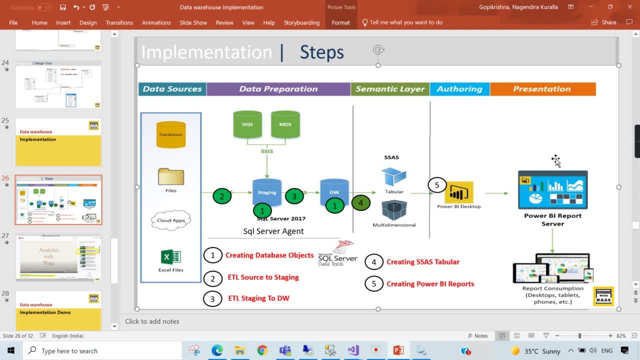 another power bi report directly from another power bi report directly from: data borrows- data borrows, data borrows. then we will discuss on why we need to go. then we will discuss on why we need to go, then we will discuss on why we need to go for both. 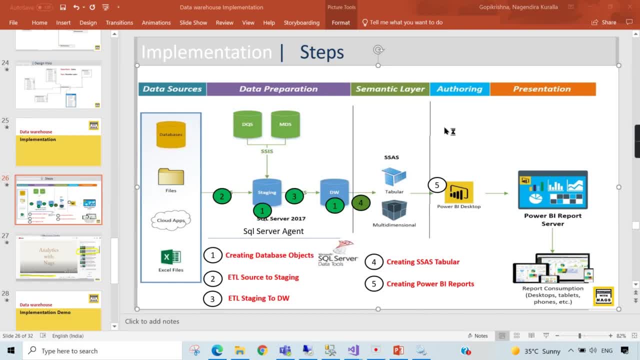 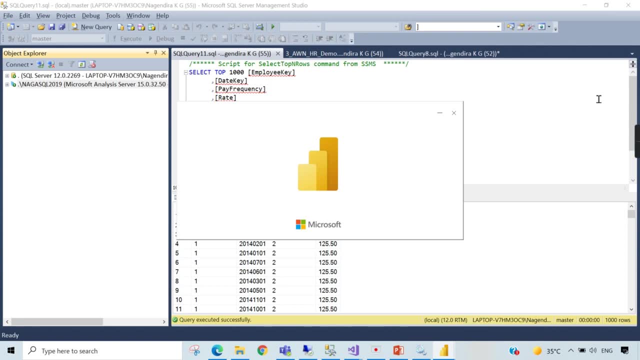 for both, for both. so let's talk about power bi desktop i so let's talk about power bi desktop i. so let's talk about power bi desktop. i mean start creating power bi desktop. mean start creating power bi desktop. mean start creating power bi desktop reports. i hope i understand. it's a too long. 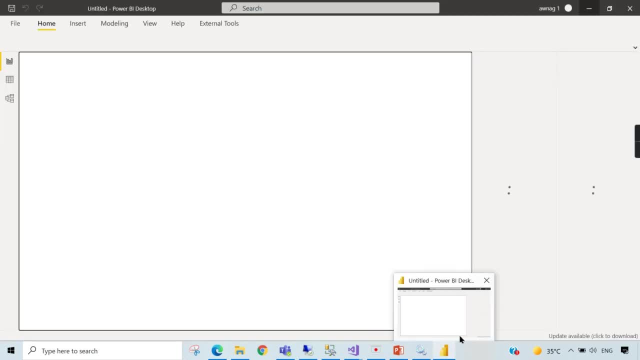 i hope i understand it's a too long. i hope i understand it's a too long. video, video, video. but i hope it was interesting to you to. but i hope it was interesting to you to, but i hope it was interesting to you to understand the entire concept. what is? 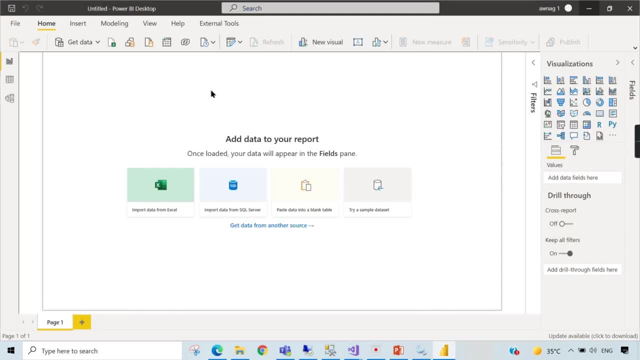 understand the entire concept. what is understand the entire concept. what is happening, happening, happening now in power. those who are familiar with now in power. those who are familiar with now in power. those who are familiar with power bi: they know how to get the data. power bi: they know how to get the data. 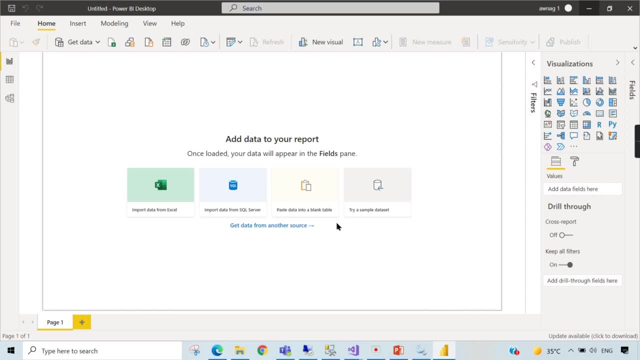 power bi. they know how to get the data, so go to get data. so go to get data. so go to get data. then you need to choose the, then you need to choose the, then you need to choose the. the different data types: first i will go. the different data types: first i will go. 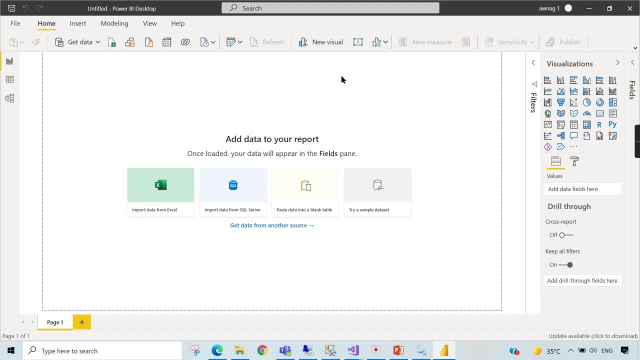 the different data types. first i will go to to: to sql server analysis service connect. then sql server analysis service connect. then sql server analysis service connect. then provide the provide: the provide the database name: dot slash nag. database name: dot slash nag. database name: dot slash nag sql. 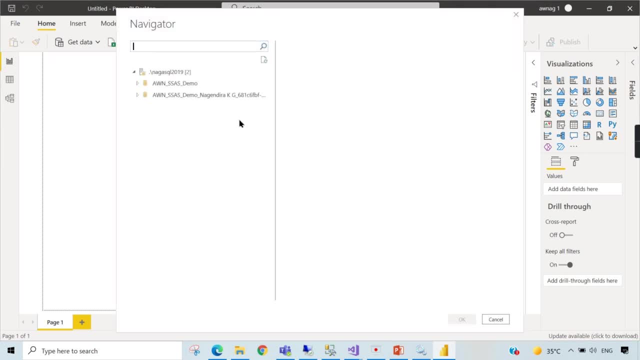 sql- sql 2019- that is the server name, and choose 2019, that is the server name, and choose 2019, that is the server name, and choose. click on ok, i can choose the database. click on ok, i can choose the database. click on ok, i can choose the database from here. 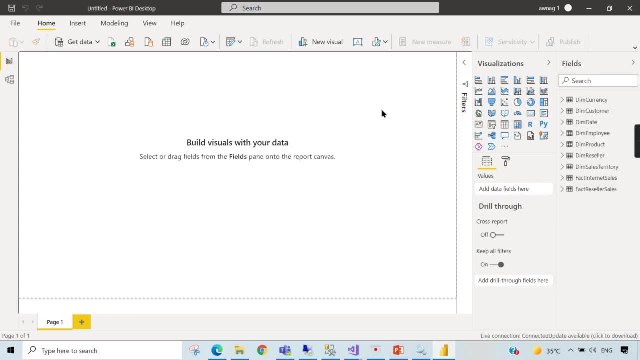 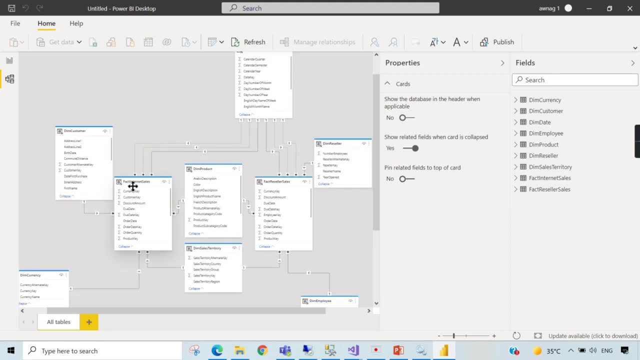 from here, from here. so now you choose the model over here. so we got the model again, you can see. so we got the model again, you can see. so we got the model again. you can see: the same model appears, the same model appears, the same model appears, as everything is connected, fact and fact. 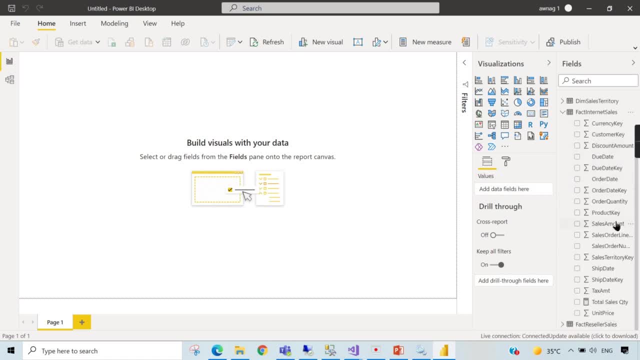 as everything is connected: fact and fact. as everything is connected, fact and fact. reseller sales- reseller sales. reseller sales. now you can also see the one of the. now you can also see the one of the. now you can also see the one of the measure we created here: the total. 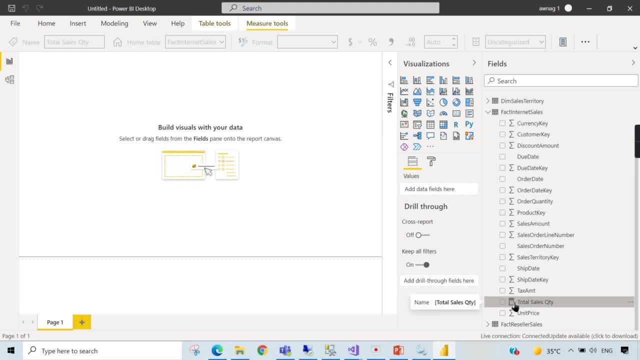 measure we created here the total measure, we created here the total quantity sales, quantity sales, quantity sales. the symbol it says like a measure right. the symbol it says like a measure right. the symbol it says like a measure right: the calculated, the calculated, the calculated measure right. and these are the default. 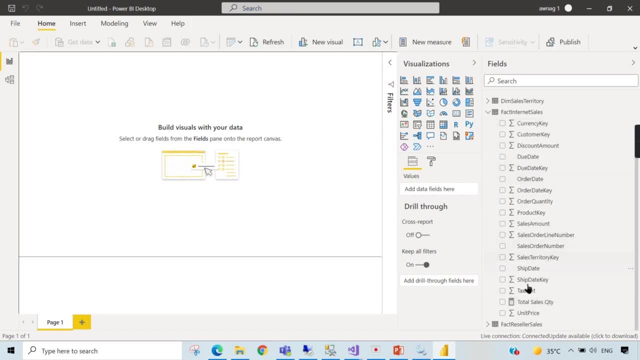 measure right, and these are the default measure right, and these are the default columns from the source table. now you columns from the source table. now you columns from the source table. now you can, can, can. to check it, just drag and drop this. to check it, just drag and drop this. 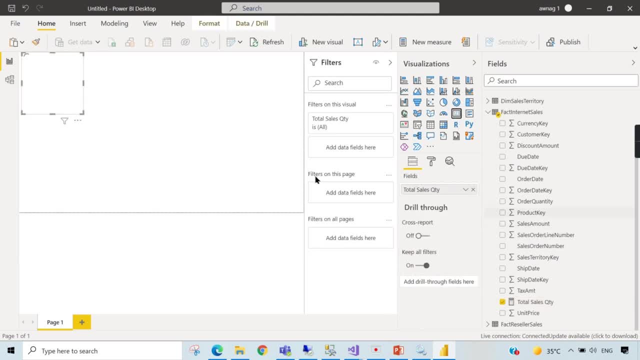 to check it. just drag and drop this columns over here and measures. just check columns over here and measures. just check columns over here and measures. just check those things are working fine or not. those things are working fine or not, those things are working fine or not. and then 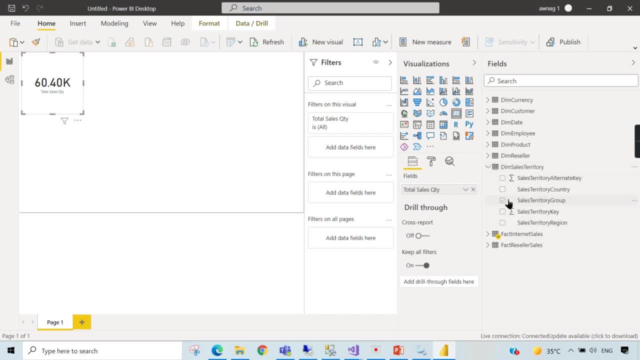 and then, and then. that is correct, the values are working. that is correct. the values are working. that is correct. the values are working fine and i can filter by fine, and i can filter by fine and i can filter by any groups as well. i can draw. any groups as well, i can draw. 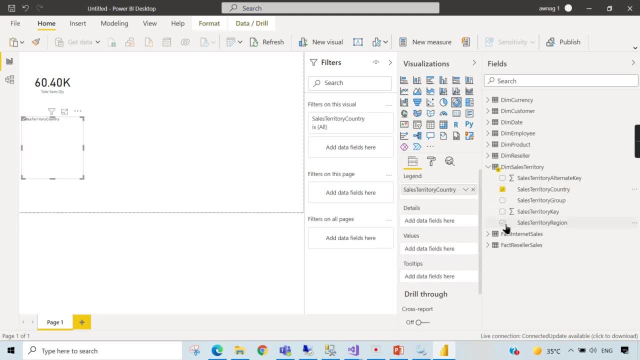 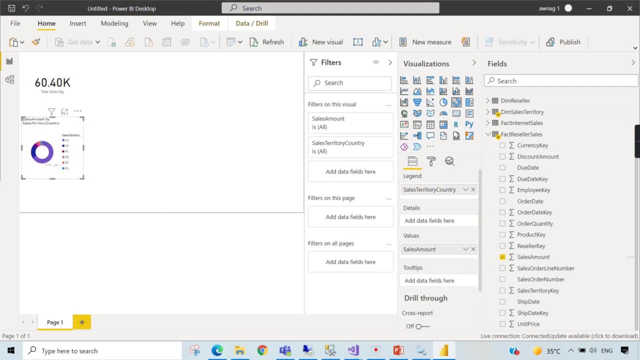 any groups as well. i can draw some of the graphs here using country, some of the graphs here using country, some of the graphs here using country. um, um, um. let me put the same total sales quantity. let me put the same total sales quantity. let me put the same total sales quantity or sales amount also, i can put here: 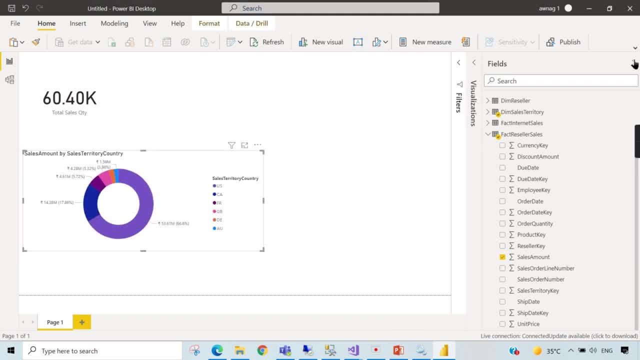 or sales amount also i can put here, or sales amount also i can put here: now, there you go. now there you go, now there you go. i i'm not focusing much on this, just it's. i. i'm not focusing much on this, just it's. i i'm not focusing much on this, just it's not. 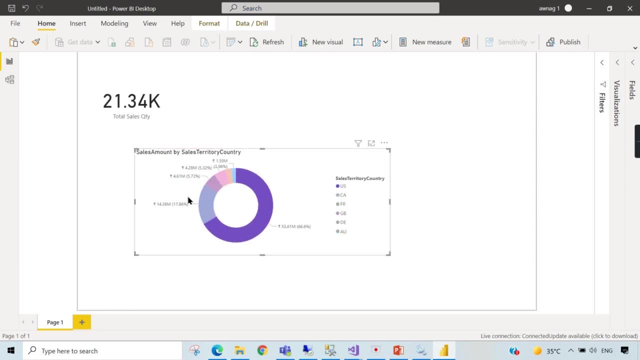 not, not our main focus now. now you can see when. our main focus now. now you can see when our main focus now. now you can see when you click on it it is also filtering, so you click on it. it is also filtering, so you click on it. it is also filtering, so it is. 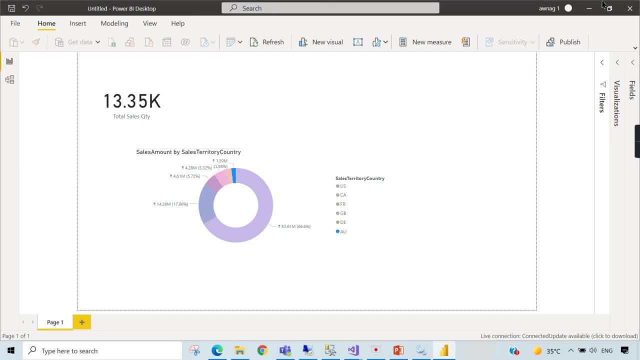 it is, it is more or less. i mean everything is more or less, i mean everything is more or less. i mean everything is interactive. so all our relationship interactive, so all our relationship interactive, so all our relationship, everything works fine, and everything works fine, and everything works fine. and one thing: we need to ensure all the data. 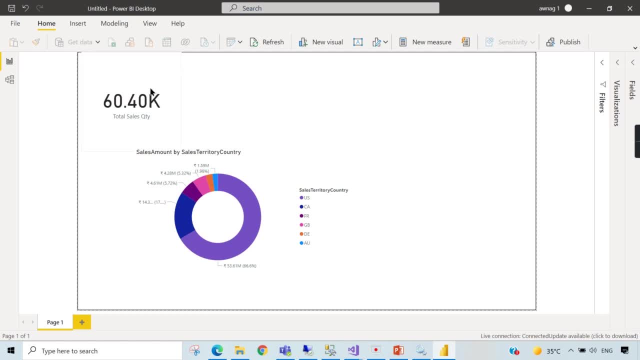 one thing: we need to ensure all the data. one thing: we need to ensure all the data is correct, is correct, is correct. that is fine. you can write a query. that is fine. you can write a query. that is fine. you can write a query against a database. 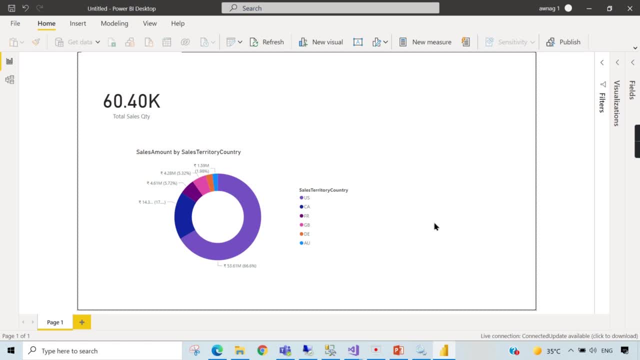 against a database, against a database, and you can compare this results. that is, and you can compare this results. that is, and you can compare this results. that is how you can, how you can, how you can verify it now. this is fine. this is one of verify it now. this is fine. this is one of 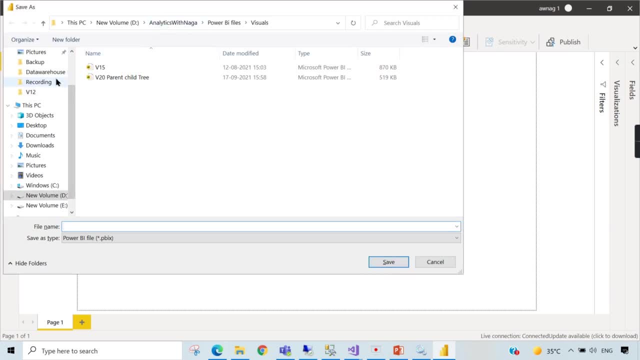 verify it now. this is fine. this is one of the report, the report. the report using um power bi. i mean using um power bi. i mean using um power bi. i mean we can save this one as we can save this one, as we can save this one as power bi awn cube. 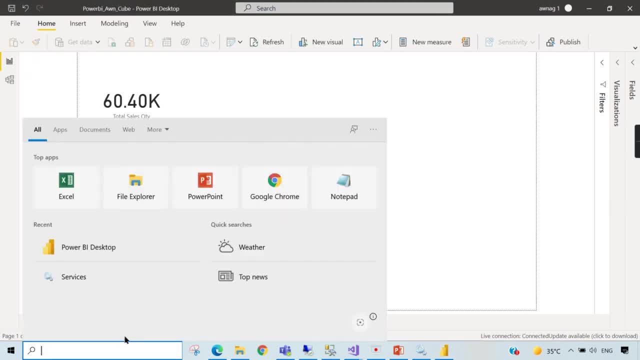 power bi awn cube. power bi awn cube, now, now. now i can also able to create a report from. i can also able to create a report from. i can also able to create a report from: power bi power bi power bi right, using the right, using the. 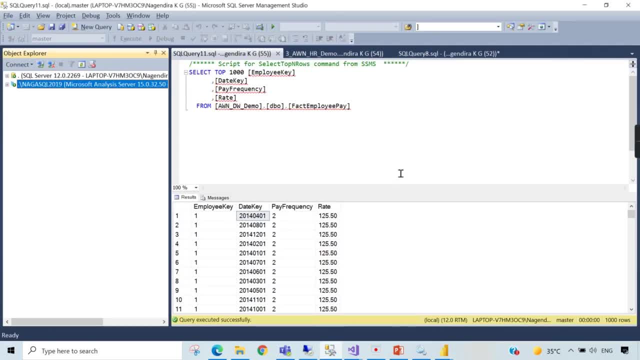 right, using the data varus as well. the code difference is data varus as well. the code difference is data varus as well. the code difference is like like like. all your logics are in a semantic layer. all your logics are in a semantic layer. 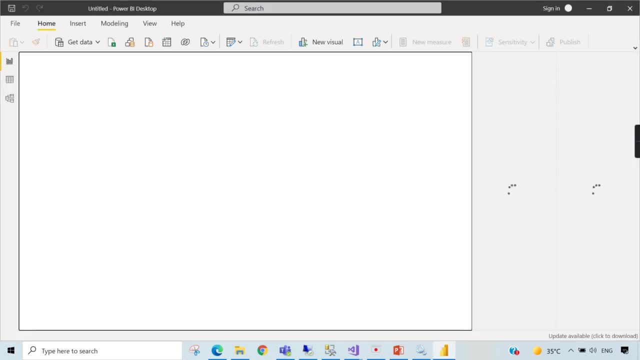 all your logics are in a semantic layer. i will quickly discuss that one. i will quickly discuss that one. i will quickly discuss that one. once we start creating the reports, once we start creating the reports, once we start creating the reports directly from the database as well. 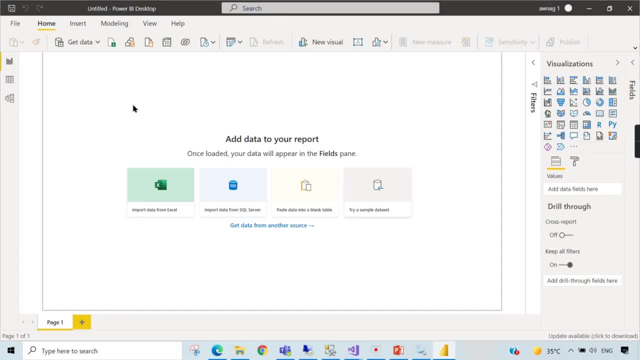 directly from the database as well. directly from the database as well. right, so in this time i will go to right, so in this time i will go to right, so in this time i will go to get data and get data, and get data, and i will get the data from the database. 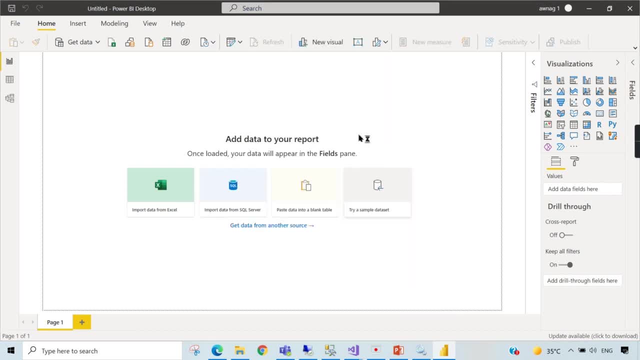 i will get the data from the database. i will get the data from the database now instead of pointing to now. instead of pointing to now, instead of pointing to analyst service, i will choose the analyst service. i will choose the analyst service. i will choose the sql server database. so 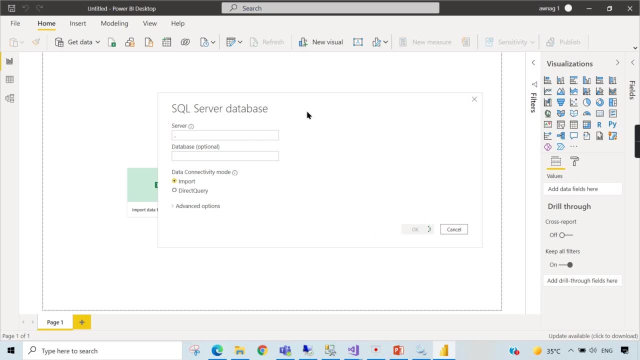 sql server database. so sql server database. so i will press dot here then click on. okay, i will press dot here then click on okay, i will press dot here then click on okay. so dot is my local server in your case. so dot is my local server in your case. 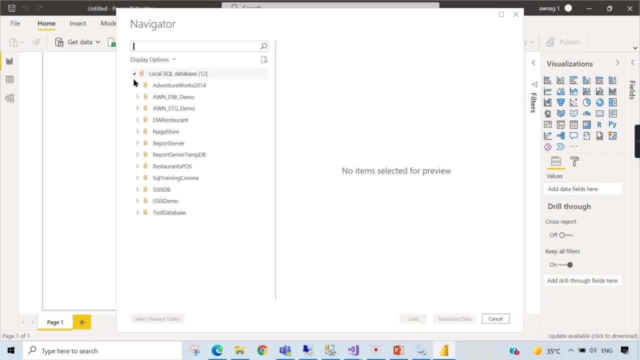 so dot is my local server. in your case, you might, you might, you might need to provide the proper server name. need to provide the proper server name. need to provide the proper server name. clicking on this database and let me clicking on this database, and let me clicking on this database and let me select. 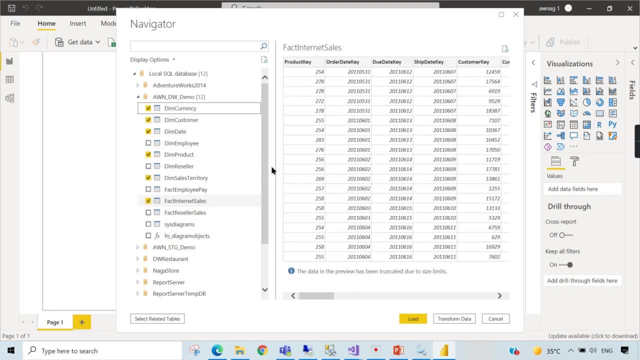 select, select, fact internet sales alone, then i will fact internet sales alone, then i will fact internet sales alone. then i will select related tables, select related tables, select related tables. as the relationship exists, it will, as the relationship exists, it will, as the relationship exists, it will have all the related tables together. 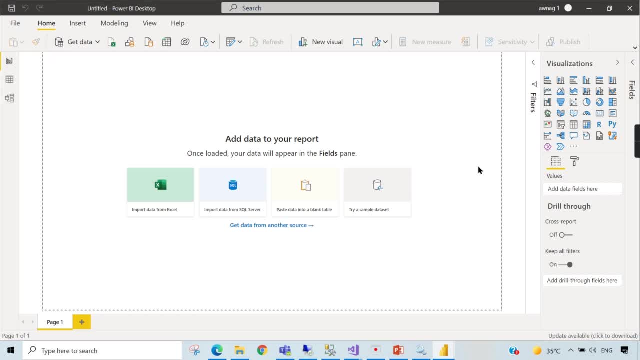 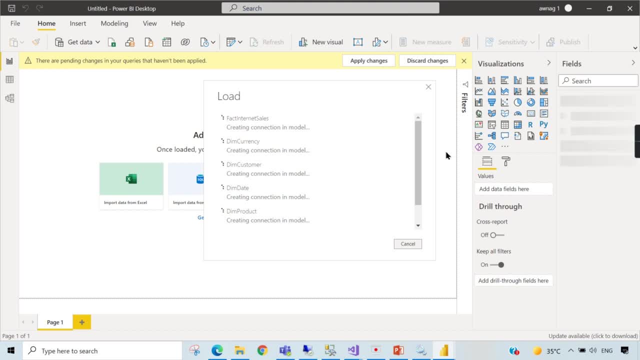 can either they are import mode, that is mode that they are import mode, that is mode that they are import mode, that is mode that is already, is already, is already. if you're not so, if you're not so familiar, if you're not so, if you're not so familiar. 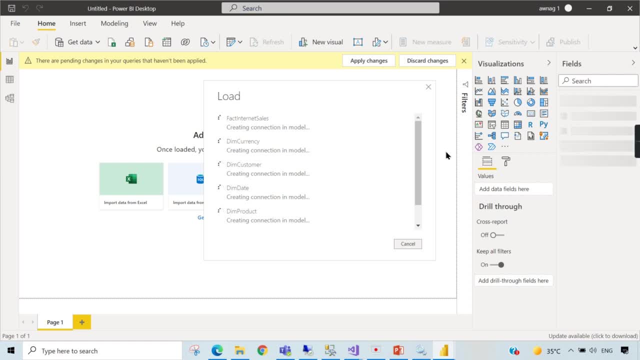 if you're not so, if you're not so familiar with power bi, with power bi, with power bi, i have a complete playlist this channel. i have a complete playlist this channel. i have a complete playlist. this channel main focus on power bi. so you can go and 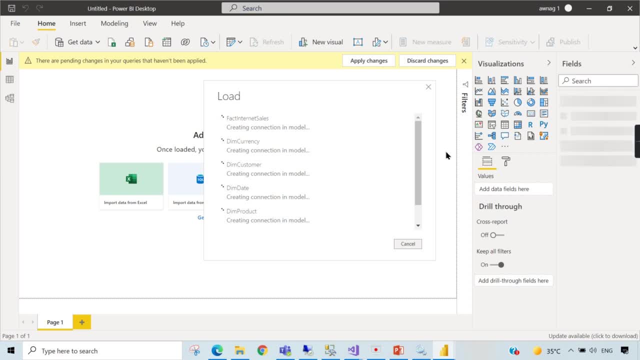 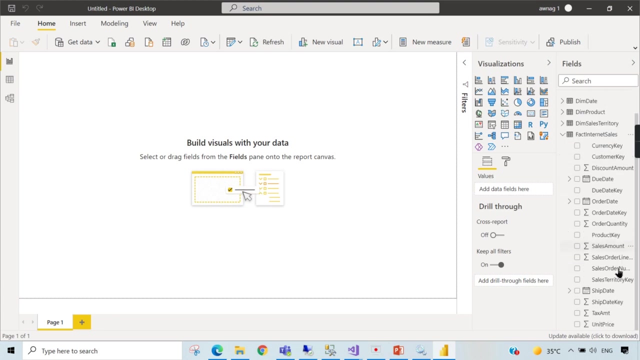 main focus on power bi, so you can go. and main focus on power bi, so you can go and check it out. let's wait for all the tables to load. okay, now, again, i can do the same thing. okay, now, again, i can do the same thing. okay, now again, i can do the same thing over here. 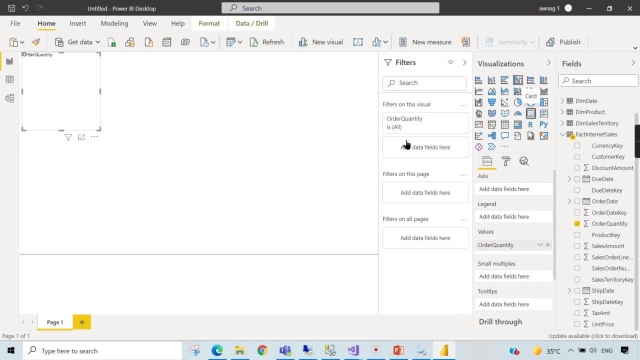 over here. over here, i will use the order quantity, i will use the order quantity, i will use the order quantity and i will have a and i will have a and i will have a data card for it. then i will use the data card for it. then i will use the. 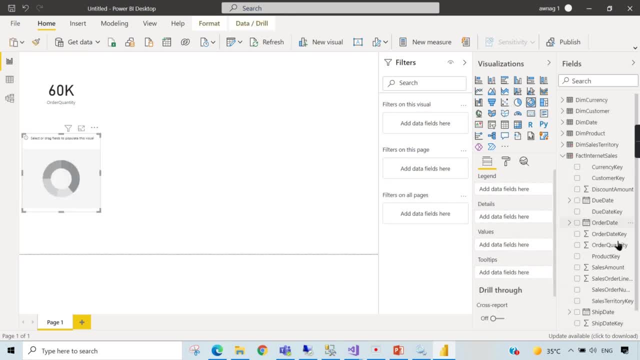 data card for it. then i will use the pie chart for pie chart for pie chart for country-wise sales right over here, for country-wise sales right over here, for country-wise sales right over here, for against a sales amount, and then against a sales amount, and then. 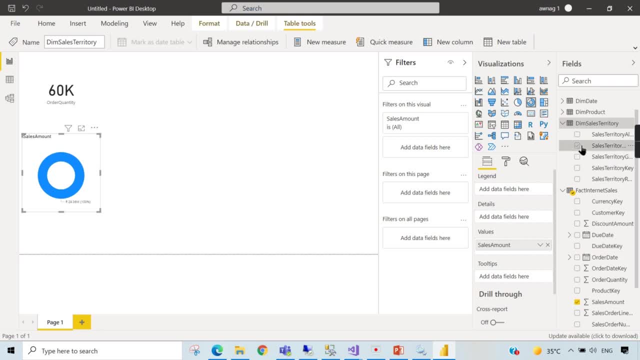 against a sales amount, and then by a country right, so country is over. by a country right so country is over. by a country right so country is over here. there you go. so even this will give me a. there you go, so even this will give me a. 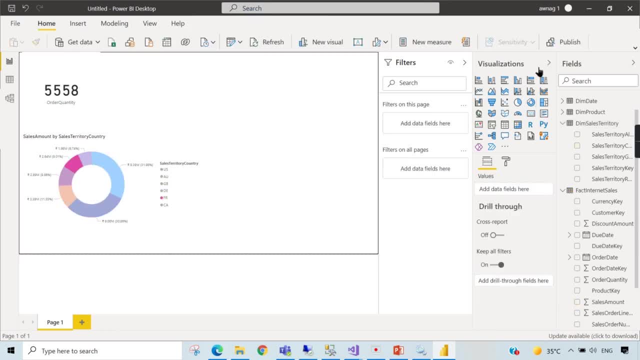 there you go. so even this will give me a same same same. kind of data, everything works fine. kind of data: everything works fine. kind of data: everything works fine. the code difference, the code difference, the code difference. we will try to understand now you get it. we will try to understand now you get it. 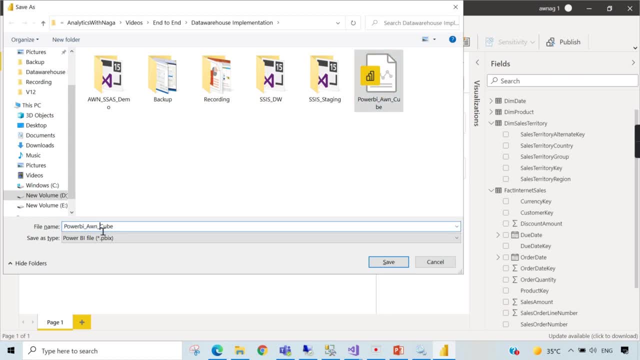 we will try to understand, now you get it, how you different ways, how you different ways, how you different ways. people uh try to connect from people. uh, try to connect from people. uh try to connect from different technologies. right, i mean different technologies. right, i mean different technologies. right, i mean different reporting tools. 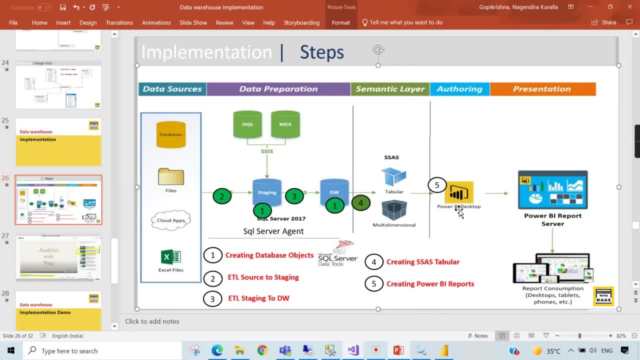 different reporting tools. different reporting tools, even for- instead of power bi. you can even for- instead of power bi. you can even for- instead of power bi. you can use the excel as well, so excel. you can use the excel as well, so excel. you can use the excel as well, so excel. you can electric connect from ssas and then data. 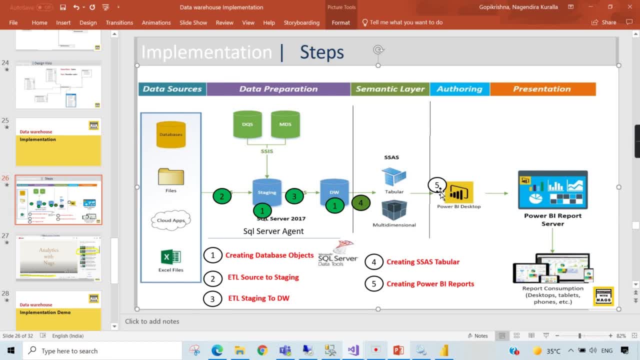 electric connect from ssas and then data electric connect from ssas and then data values as well. you can values as well. you can values as well. you can create reports on top of it. so we are create reports on top of it. so we are create reports on top of it. so we are done with. 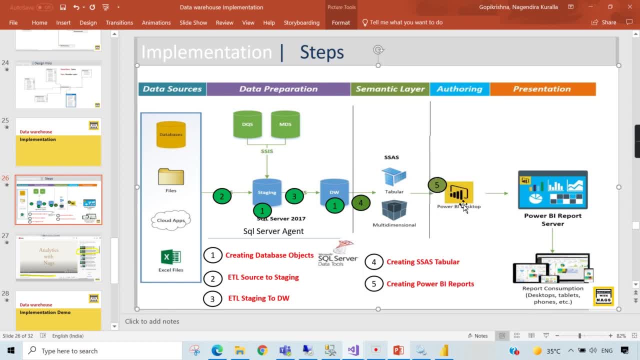 done with. done with this flow, and i want to finally this flow, and i want to finally this flow and i want to finally highlight what is the difference, why we highlight, what is the difference why we highlight, what is the difference why we need to connect to ssas from power bi. 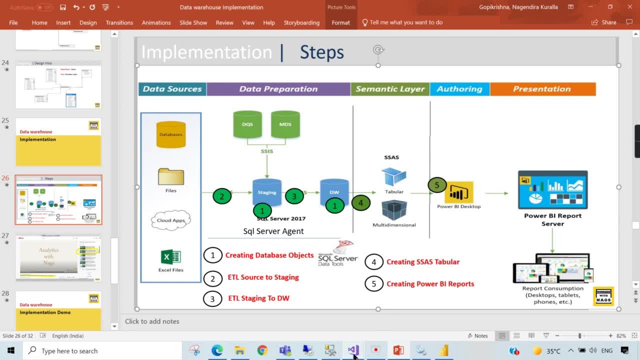 need to connect to ssas from power bi. need to connect to ssas from power bi. or data errors. in what scenarios you or data errors in what scenarios you or data errors in what scenarios you might have noticed in ssas. might have noticed in ssas. 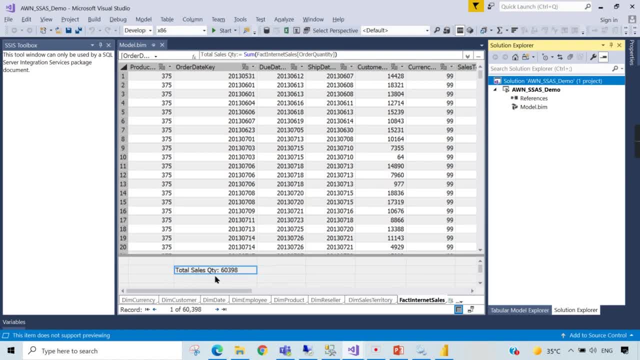 might have noticed in ssas, i have created one of the core measure. i have created one of the core measure. i have created one of the core measure here, here, here. so this particular measure, so this kind of so, this particular measure, so this kind of so, this particular measure, so this kind of logics is a semantic layer, all your. 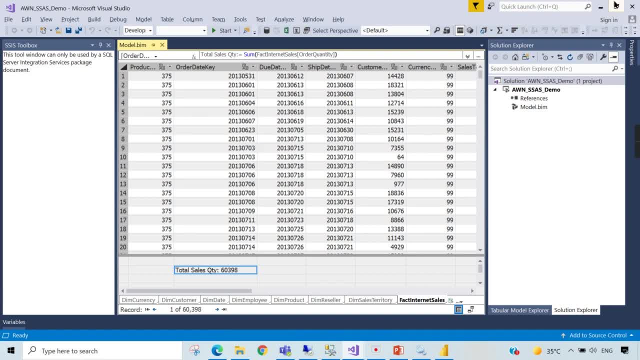 logics is a semantic layer. all your logics is a semantic layer. all your business logics- ytd mtd. business logics- ytd mtd. business logics- ytd mtd. right. everything can be stored in your right. everything can be stored in your. 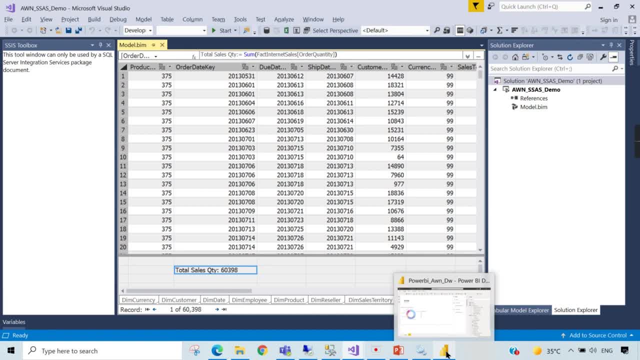 right. everything can be stored in your ssas model. so any reports can consume ssas model. so any reports can consume ssas model. so any reports can consume. so one of the user is utilizing those. so one of the user is utilizing those. so one of the user is utilizing those calculations he can directly connect to. 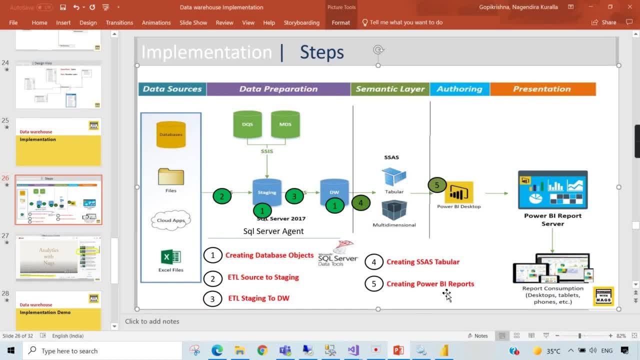 calculations. he can directly connect to calculations. he can directly connect to ssas model. ssas model, ssas model. whereas the when you're trying to connect, whereas the when you're trying to connect, whereas the when you're trying to connect directly from your data arrows. directly from your data arrows. 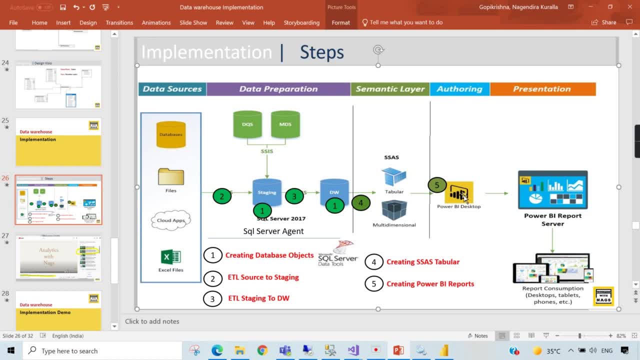 directly from your data arrows some. if one user is want ytd, he has to some. if one user is want ytd, he has to some. if one user is want ytd, he has to write on its own in the power desktop. write on its own in the power desktop. 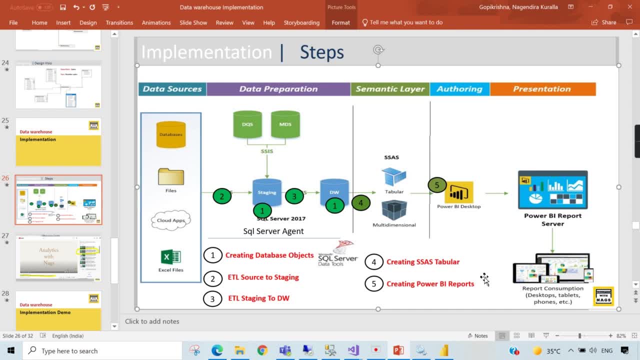 write on its own in the power desktop. another user has to calculate it. another another user has to calculate it. another another user has to calculate it. another user also has to write ytd here. user also has to write ytd here. user also has to write ytd here. those calculations can be stored here. 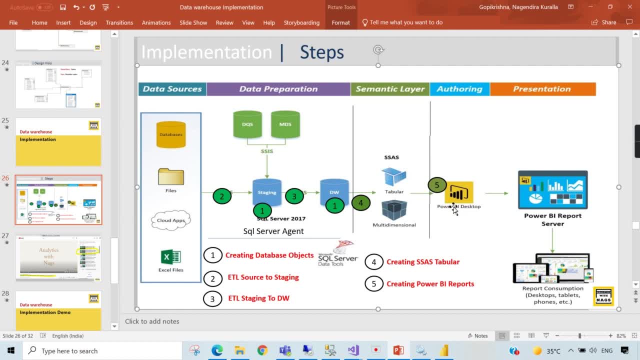 those calculations can be stored here. those calculations can be stored here. typically, ssas tabular is nothing but typically ssas tabular is nothing but typically ssas tabular is nothing but your modeling part of power bi, so you. your modeling part of power bi, so you. 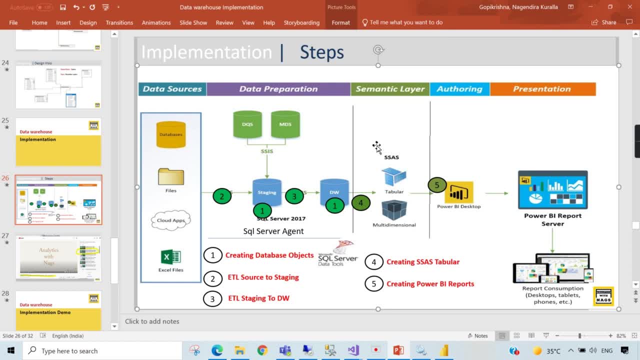 your modeling part of power bi. so you are segregating your modeling part from. are segregating your modeling part from. are segregating your modeling part from power bi and doing it in the another power bi and doing it in the another power bi and doing it in the another layer. 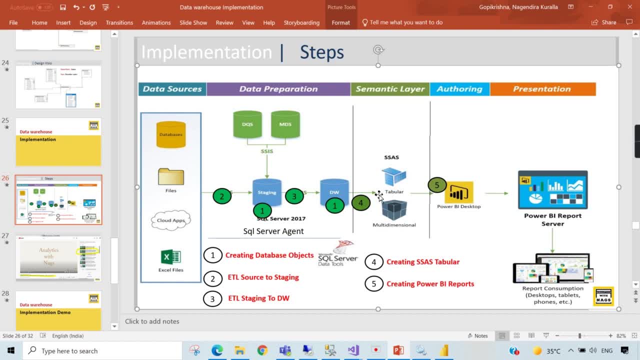 layer, layer. so this is another very big topic. so this is another very big topic. so this is another very big topic. this is only for the on-premises cycle. this is only for the on-premises cycle. this is only for the on-premises cycle. i have explained for. 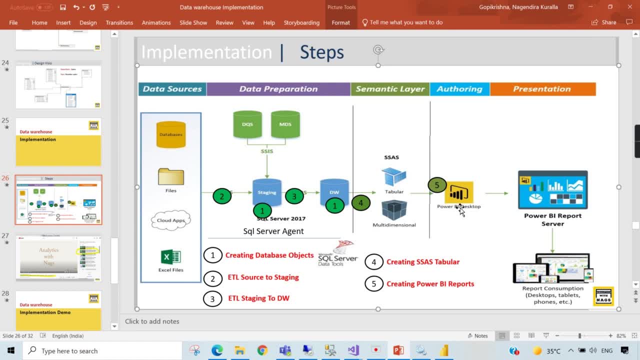 i have explained for. i have explained for: in case of cloud version, you can deploy. in case of cloud version, you can deploy. in case of cloud version, you can deploy the power bi, the power bi, the power bi modeling, and as one of the data set and modeling, and as one of the data set and 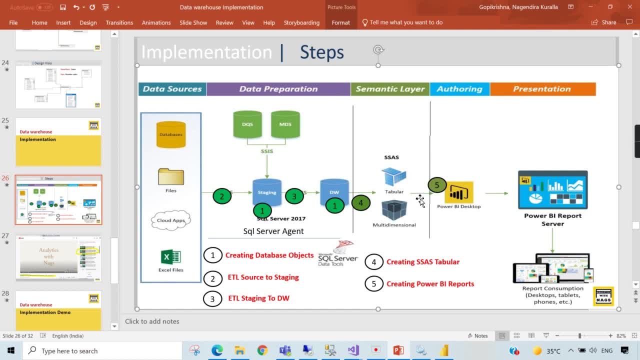 modeling and as one of the data set, and from that data set you can consume it. from that data set, you can consume it. from that data set, you can consume it. that is the workaround. or in case of that is the workaround. or in case of that is the workaround. or, in case of cloud, you can have sql server analysis. 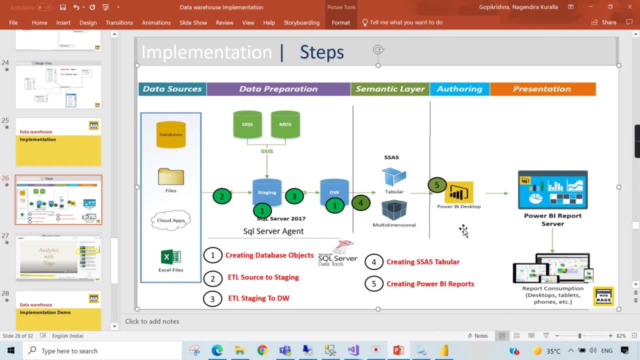 cloud. you can have sql server analysis cloud. you can have sql server analysis, azure analysis service as well, azure analysis service as well, azure analysis service as well. so there are here and there you have. so there are here and there you have. so there are here and there you have some. 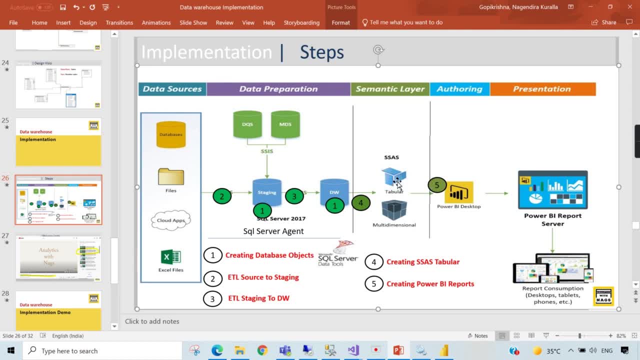 some some advantages disadvantages, but the core advantages disadvantages but the core advantages disadvantages, but the core part is part is part is all your calculations and your modeling, all your calculations and your modeling, all your calculations and your modeling. part can be done only once. part can be done only once. 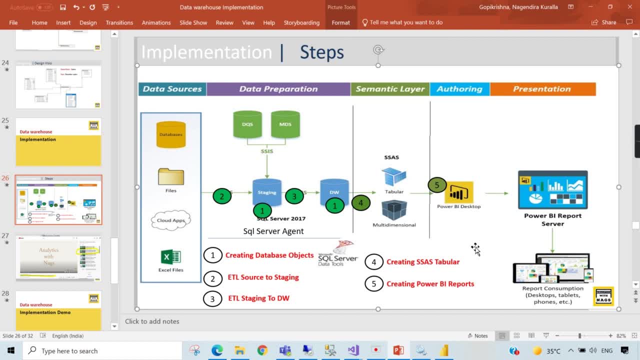 part can be done only once. you no need to repeat those things again. you no need to repeat those things again. you no need to repeat those things again and again, in and again, in and again, in, everywhere in the power bi desktop that is, everywhere in the power bi desktop that is. 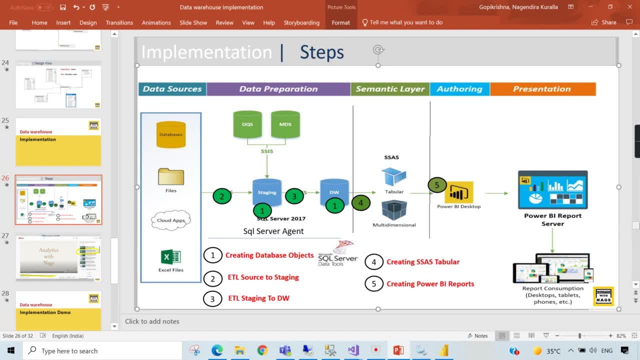 everywhere in the power bi desktop. that is the core difference, the core difference, the core difference. i hope we have completed the entire. i hope we have completed the entire. i hope we have completed the entire session, the entire flow. i have tried my session, the entire flow. i have tried my. 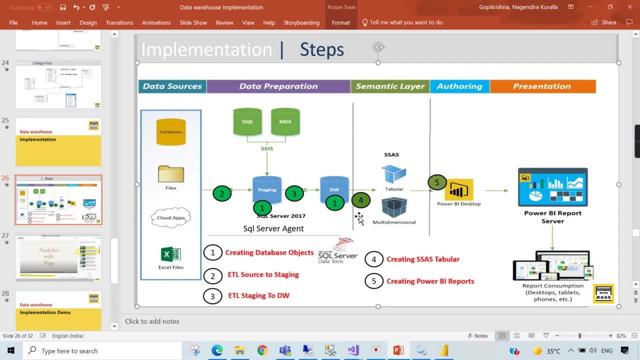 session, the entire flow. i have tried my level best to make you to understand level best, to make you to understand level best, to make you to understand this entire data browsing and this bi, this entire data browsing and this bi, this entire data browsing and this bi implementation. let us quickly see what. 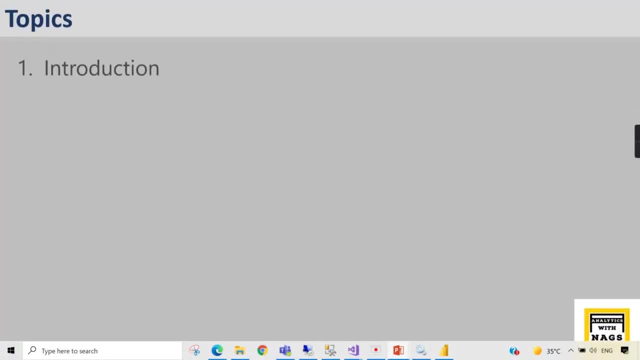 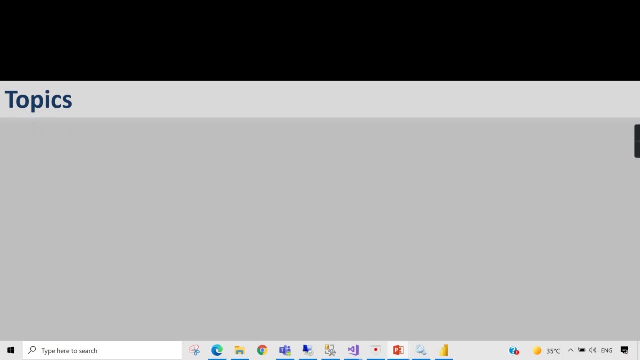 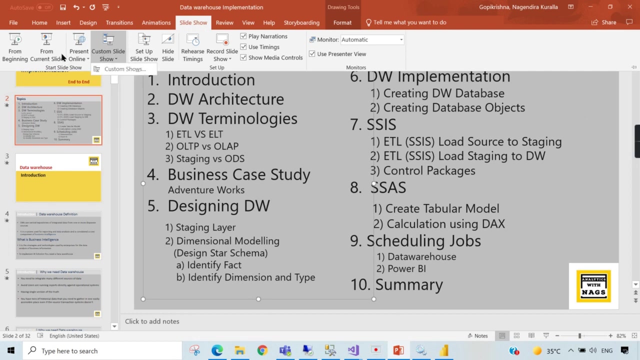 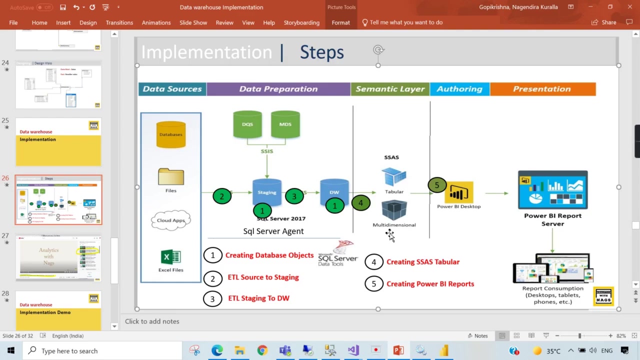 implementation. let us quickly see what implementation. let us quickly see what we have seen so far. we started with the. we have seen so far. we started with the. we have seen so far. we started with the introduction and then we. so this is another very big topic. so this is another very big topic. 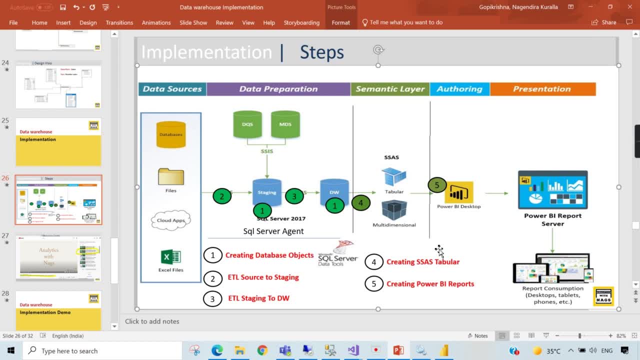 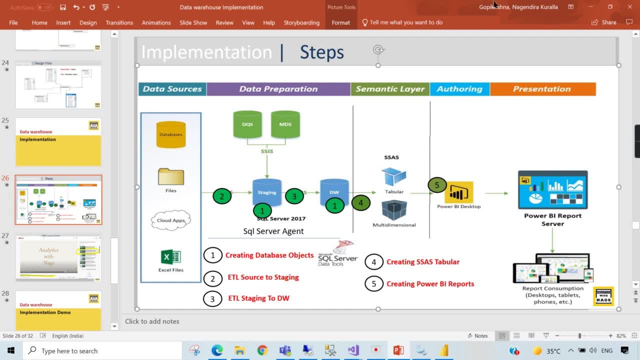 explained for in case of cloud version. explained for: in case of cloud version, you can deploy the power bi. you can deploy the power bi. you can deploy the power bi modeling and as one of the data set and modeling and as one of the data set and modeling and as one of the data set and from that data set you can consume it. 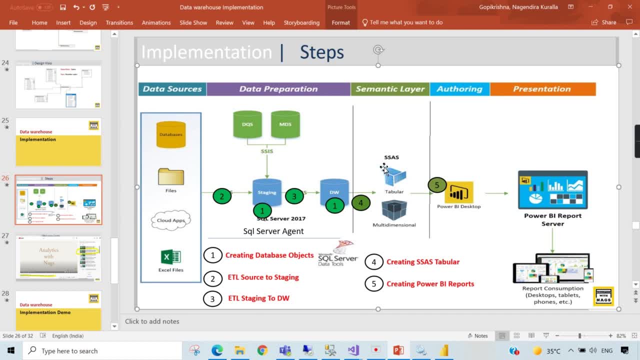 from that data set, you can consume it. from that data set, you can consume it. that is the workaround. or in case of that is the workaround. or in case of that is the workaround. or in case of cloud, you can have sql server analysis. cloud, you can have sql server analysis. 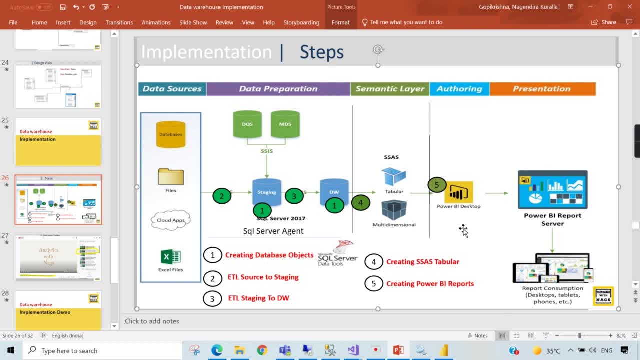 cloud. you can have sql server analysis, azure analysis service as well. so there, azure analysis service as well, so there, azure analysis service as well. so there are here and there. you have some are here and there. you have, some are here and there. you have some advantages, disadvantages, but the core 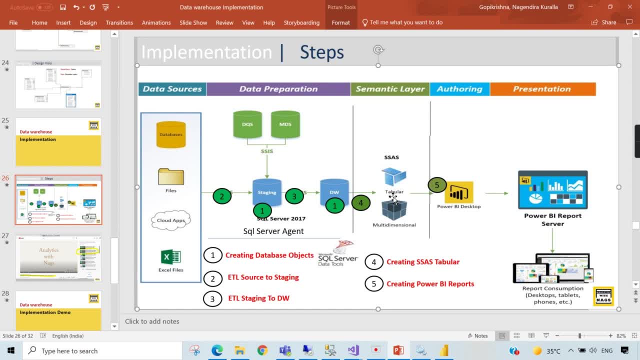 advantages, disadvantages, but the core- advantages, disadvantages, but the core part is all your calculations and your part is all your calculations and your part is all your calculations and your modeling part can be done only once. you modeling part can be done only once. you modeling part can be done only once. you no need to repeat those things again and 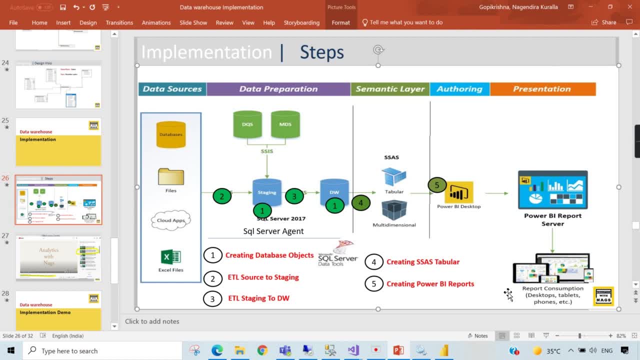 no need to repeat those things again, and no need to repeat those things again and again in every where in the power video, again in every where in the power video, again in every where in the power video. stop, that is the core difference, i hope. stop, that is the core difference, i hope. 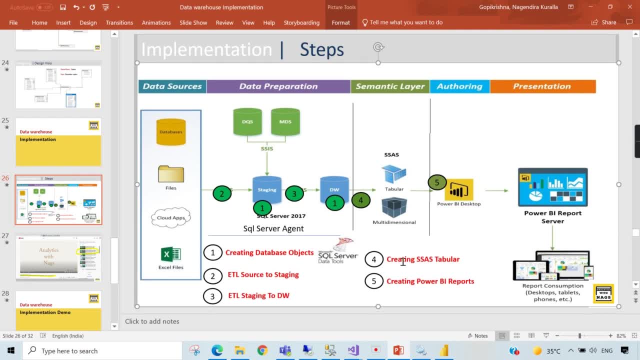 stop. that is the core difference. i hope we have completed the entire. we have completed the entire. we have completed the entire session, the entire flow. i have tried my session, the entire flow. i have tried my session, the entire flow. i have tried my level best to make you to understand. 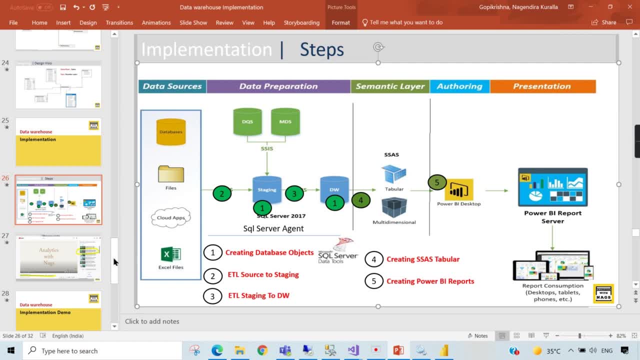 level best to make you to understand, level best to make you to understand this entire data browsing and this bi, this entire data browsing and this bi, this entire data browsing and this bi implementation, implementation, implementation, guys. whatever we have seen today in guys, whatever we have seen today in. 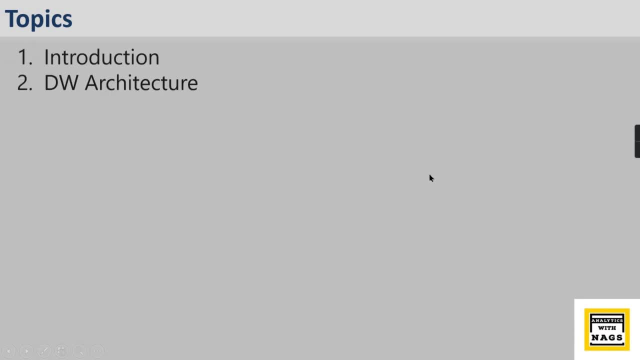 guys, whatever we have seen today in this video, this video, this video, we started with introduction and we started with introduction and we started with introduction and understand the data warehouse, understand the data warehouse, understand the data warehouse architecture- and we have architecture and we have architecture and we have walked through how it can be implemented. 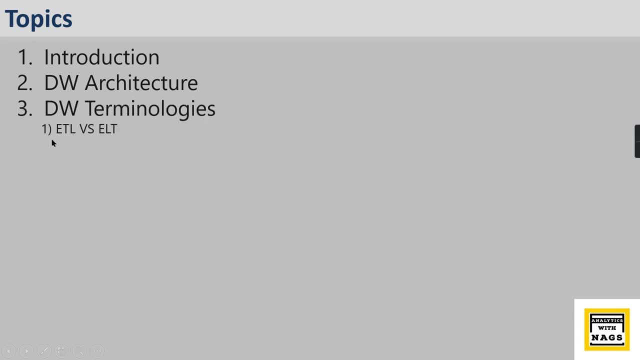 walked through how it can be implemented. walked through how it can be implemented step by step. what is the bi step by step? what is the bi step by step? what is the bi- architecture as well- and terminologies- we architecture as well- and terminologies- we architecture as well, and terminologies we have seen through. 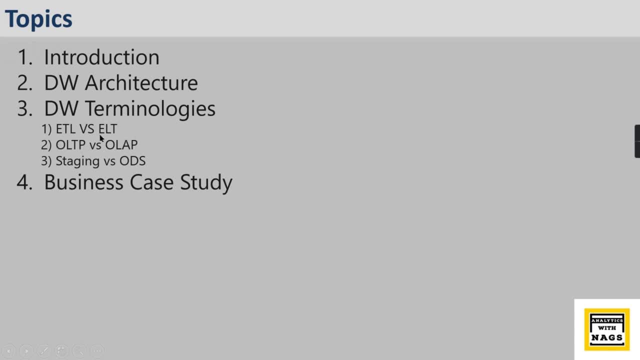 have seen through, have seen through and we have practically seen what is all. and we have practically seen what is all and we have practically seen what is all- app and etl- and we didn't implement at app and etl. and we didn't implement at app and etl and we didn't implement at elt. that is for cloud. 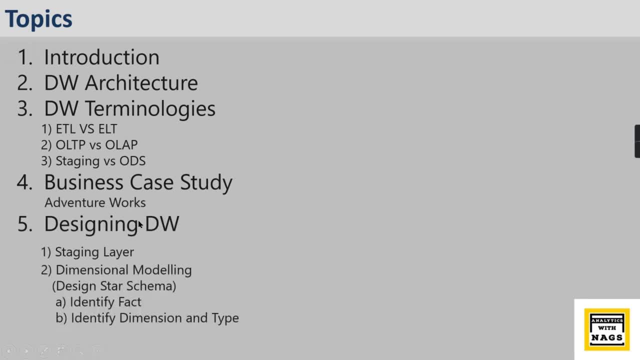 elt that is for cloud, elt, that is for cloud, and we have seen all these things using a and we have seen all these things using a and we have seen all these things using a business case study, business case study, business case study- and we have designed using visio, i mean. 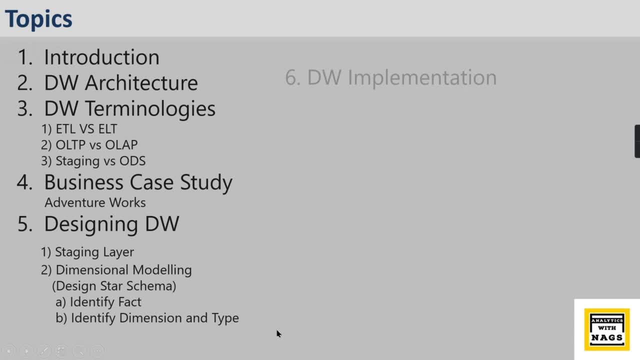 and we have designed using visio. i mean: and we have designed using visio. i mean we have showed how we can design it. we have shown how we can design it. we have shown how we can design it. that is prerequisite for implementation. that is prerequisite for implementation. 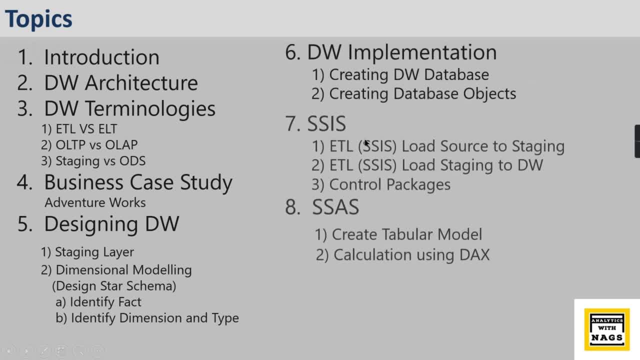 that is prerequisite for implementation. the impractical implementation, we the impractical implementation, we the impractical implementation. we created objects, created objects, created objects and then ssis packages- the controlling, and then ssis packages- the controlling and then ssis packages, the controlling packages, packages, packages and then ssas. we have created tabular. 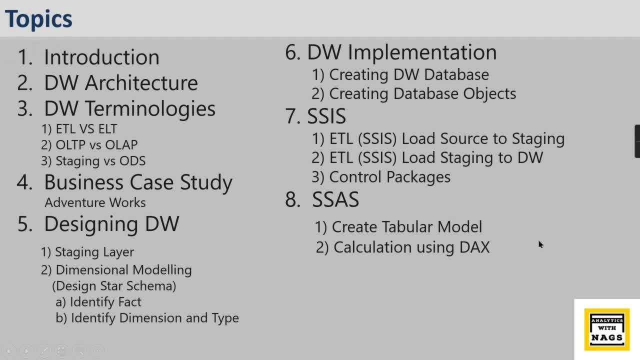 and then ssas. we have created tabular and then ssas, we have created tabular model. simple model, simple model. simple dax queries- a single query. we have dax queries- a single query. we have dax queries- a single query we have created. that is fine for this demo. 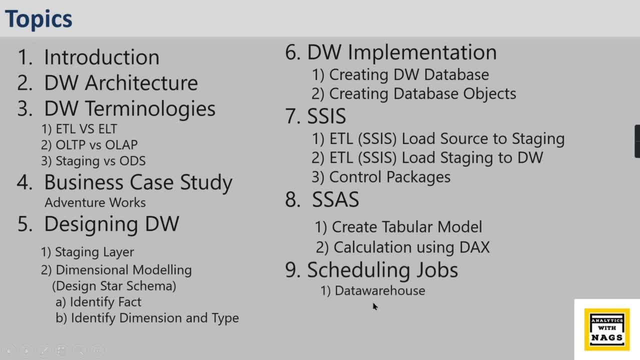 created. that is fine for this demo. created. that is fine for this demo. and then and then and then. you have seen the scheduling and data. you have seen the scheduling and data. you have seen the scheduling and data: browsing scheduling. we have seen browsing scheduling scheduling. we have seen. 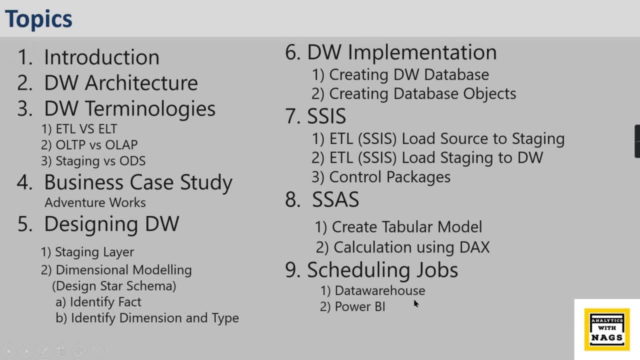 browsing scheduling scheduling. we have seen and power bi scheduling separate. we and power bi scheduling separate. we and power bi scheduling separate. we have never seen it, have never seen it, have never seen it, but it is uh, i explained in the power bi. but it is uh, i explained in the power bi. 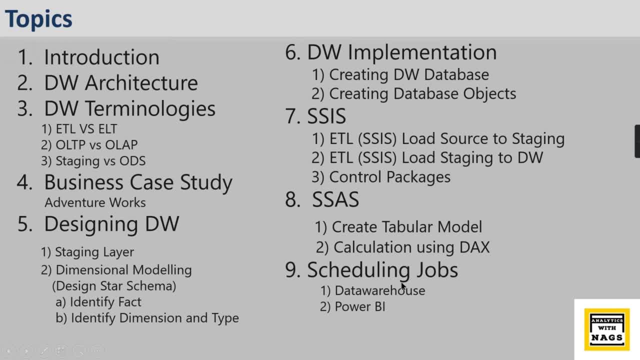 but it is, uh, i explained in the power bi playlist. you go and check it out. playlist. you go and check it out playlist. you go and check it out, so the scheduling from data arrows and so the scheduling from data arrows and so the scheduling from data arrows and power bi is different. say, for example, it: 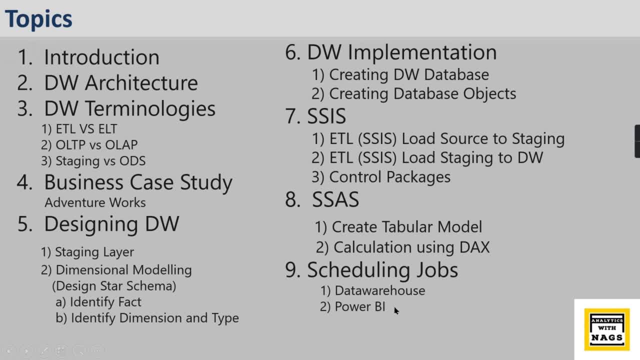 power bi is different. say, for example: it power bi is different. say, for example: it takes two hours to complete, takes two hours to complete, takes two hours to complete. then after that, only you need to schedule, then after that, only you need to schedule, then after that, only you need to schedule it. there is no way to trigger it, right? 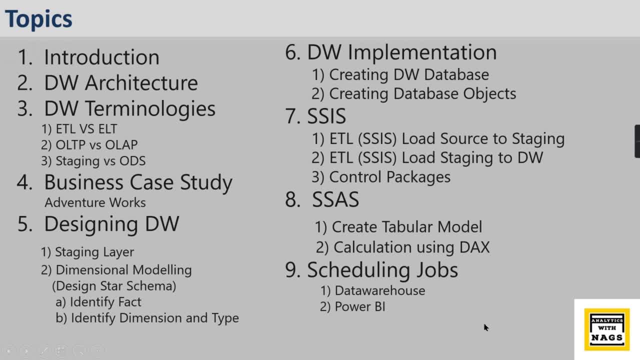 it. there is no way to trigger it right it. there is no way to trigger it right now. there are some other tools we need now. there are some other tools we need now. there are some other tools we need to go for power automate. to go for power automate. 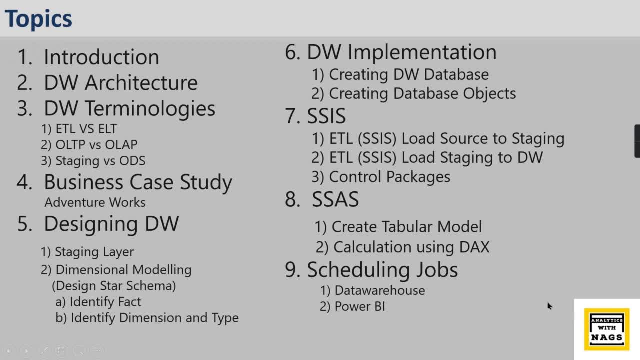 to go for power, automate or some other tools. that is separate, or some other tools. that is separate, or some other tools. that is separate story. i will talk about it story. i will talk about it story. i will talk about it how we can do it. so, but for your, 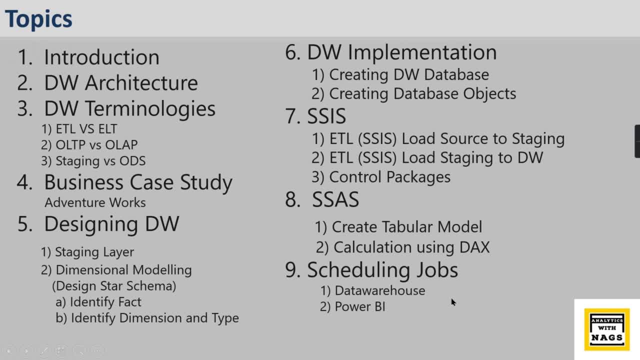 how we can do it so, but for your how we can do it so, but for your, understanding this scheduling, understanding this scheduling, understanding this scheduling between data warehouse and power bi are between data warehouse and power bi, are between data warehouse and power bi are different, different, different even. you can add the cube processing in. 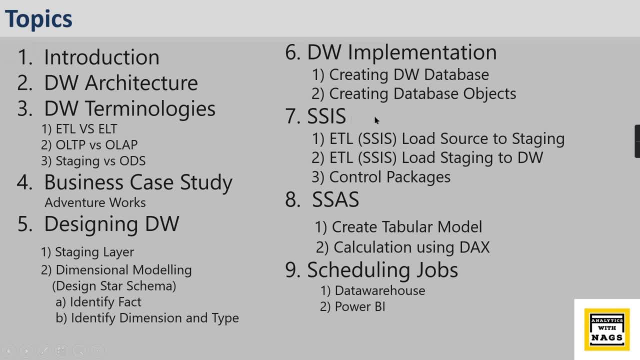 even you can add the cube processing in, even you can add the cube processing in the ssis itself, the ssis itself, the ssis itself, since ssis, ssis concise, since ssis, ssis, concise, since ssis, ssis concise, ssas processing task. right in that you. 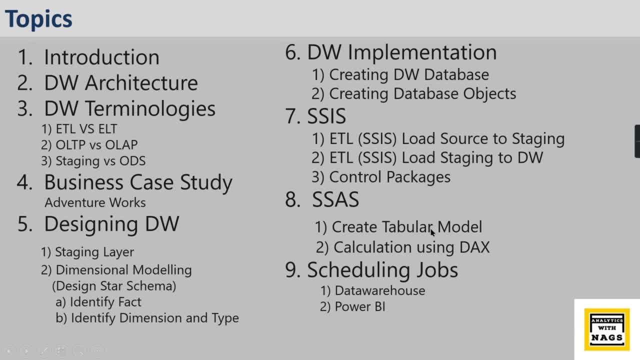 ssas processing task right in that you ssas processing task right in that you can process the cube, can process the cube, can process the cube. so it is part of data warehousing, so it is part of data warehousing, so it is part of data warehousing itself. 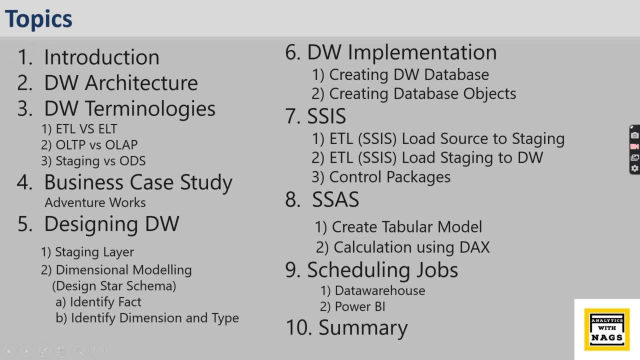 itself itself. now, this is where we are. we are done now. this is where we are. we are done now. this is where we are. we are done with our today's topic. i hope you like with our today's topic. i hope you like with our today's topic. i hope you like this video. if you enjoy this video, give. 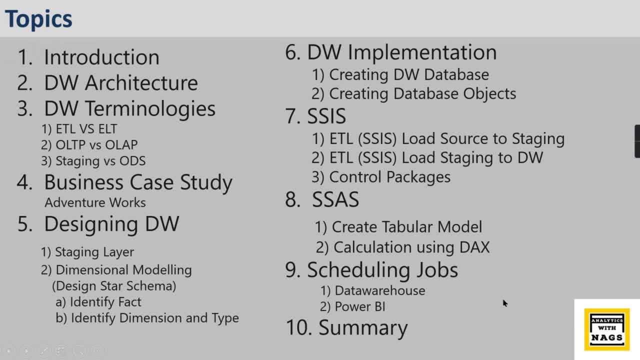 this video. if you enjoy this video, give this video. if you enjoy this video, give a thumbs up, a thumbs up, a thumbs up, share this video with your friends and share this video with your friends. and share this video with your friends and colleagues. colleagues, colleagues, and comment below for queries and do.